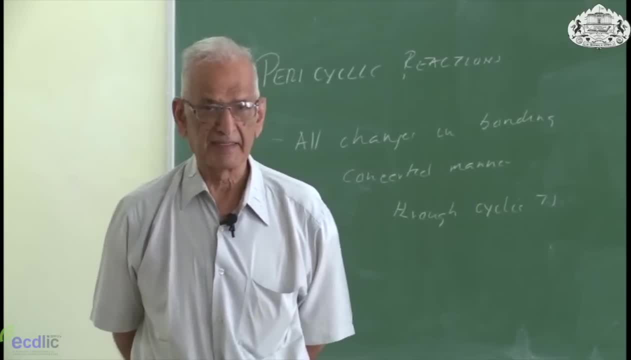 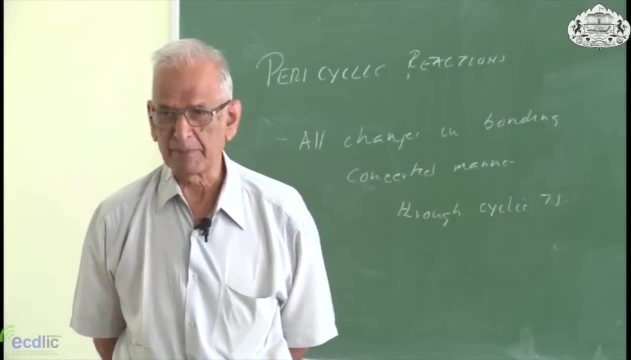 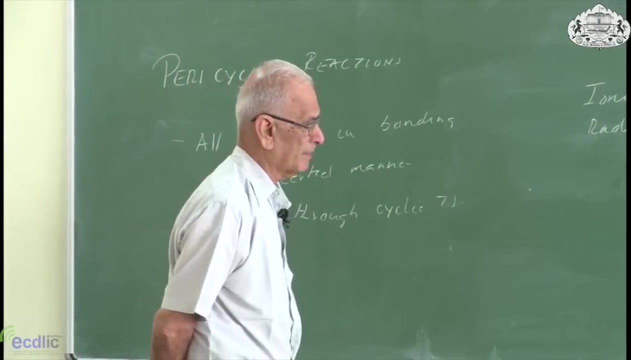 prize. In the talks of penicillin, gap between discovery and prize is almost 30 years. You talk of DNA structure gap between discovery and prize is more than 25 years. So not only a Nobel Prize, but a very short gap between discovery and prize. 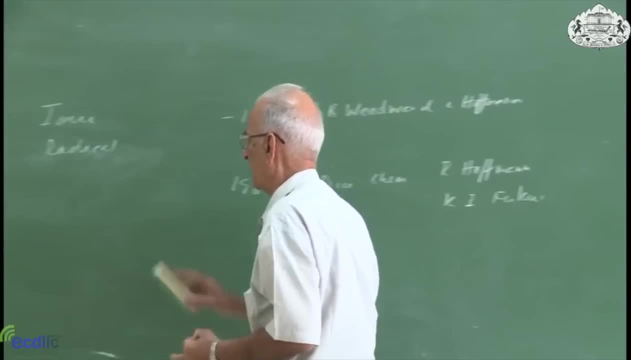 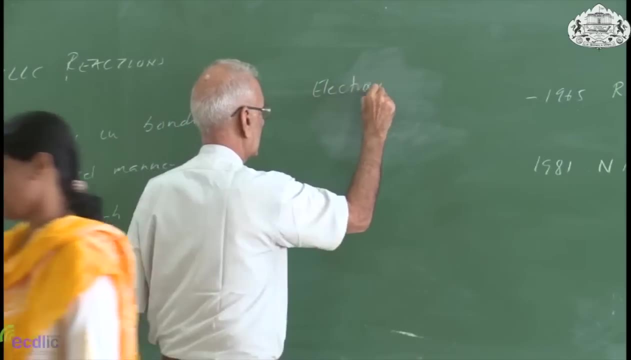 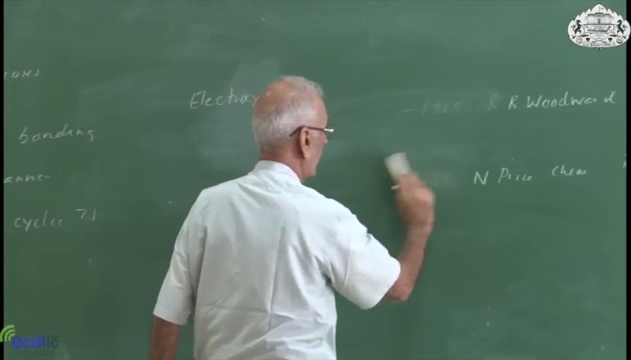 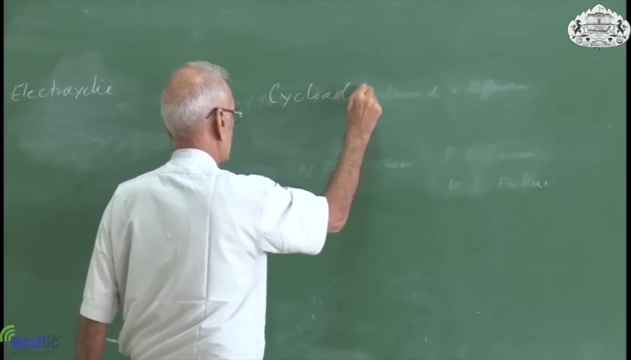 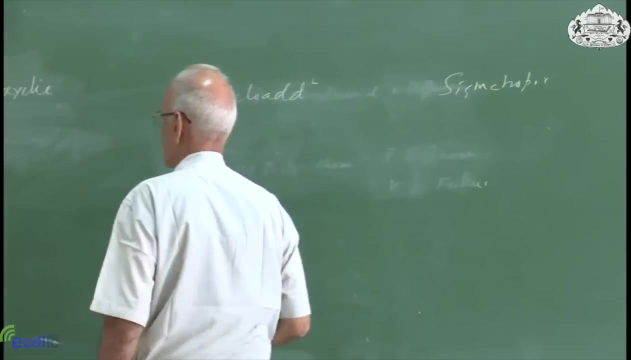 Pericyclic reactions can be categorized into three types. First type is cycloaddition-sigmatаюсь. cycloaddition of different types is cycloбоids. There is there is a cyclo transition, often named as scole. 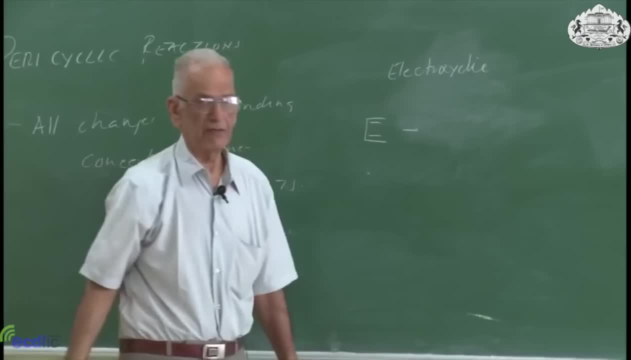 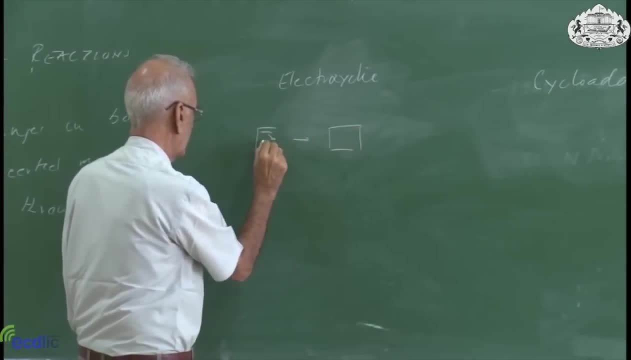 There is really foreshadowingment, So Maar, but the idea is not 1.2.There is some time there will maybe stay 3, but 3아, It can take 5 to 6 years. conversion of butadiene to cyclobutene. If I push the arrows only to make it more clear. 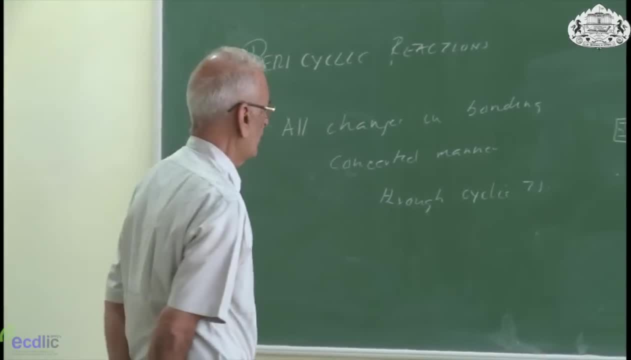 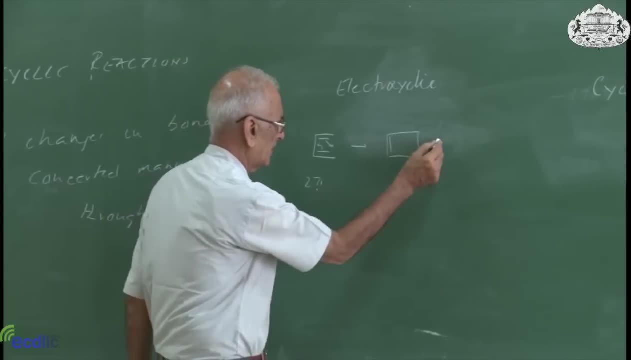 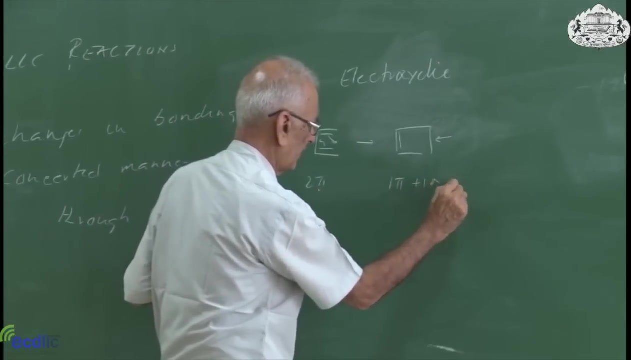 that is the kind of change that we are talking about. If I look at left hand side, we have two pi bonds in the product. we have made a new sigma bond, So there is one pi bond, one sigma bond and a ring If we go from left to right. 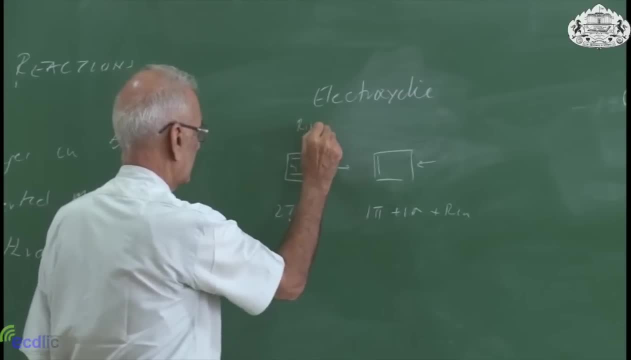 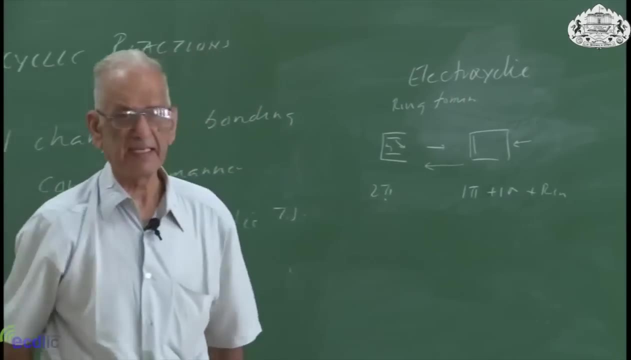 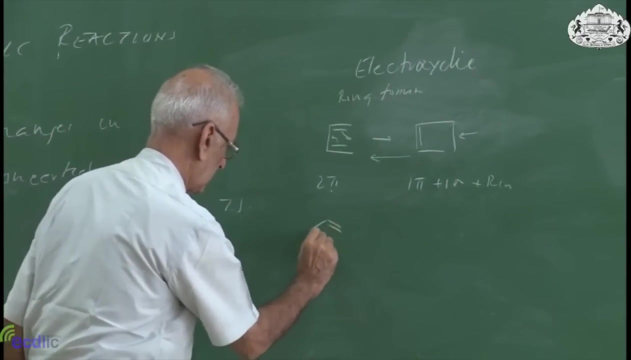 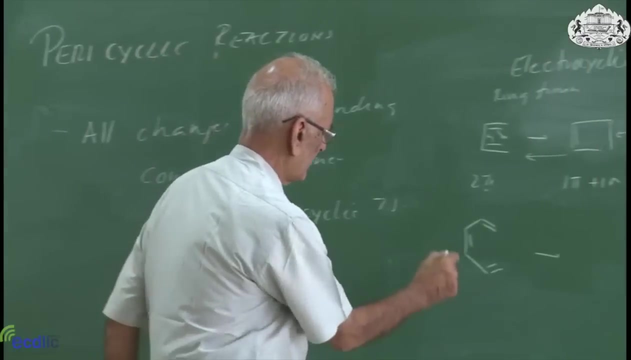 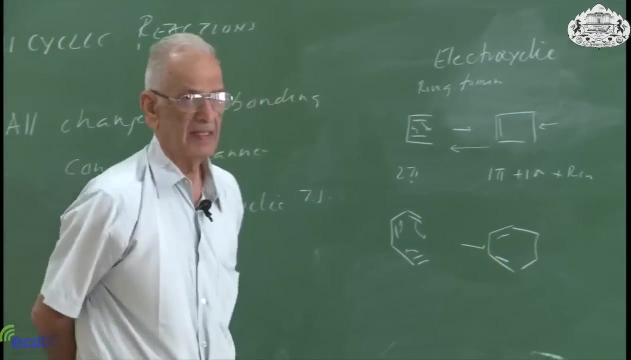 we call this as a ring forming reaction. If you go from right to left, it is obviously a ring opening reaction. That would be another reaction, Another example of this hexatriene getting converted to cyclohexadiene, If I look on. 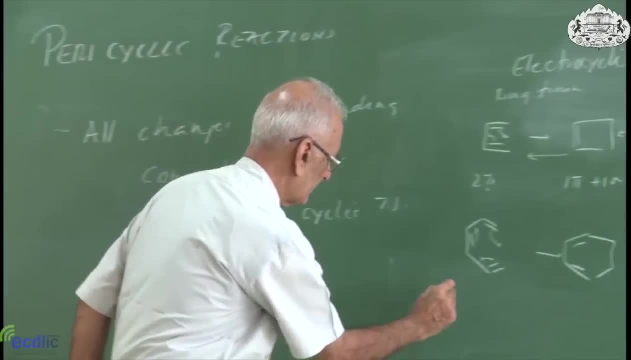 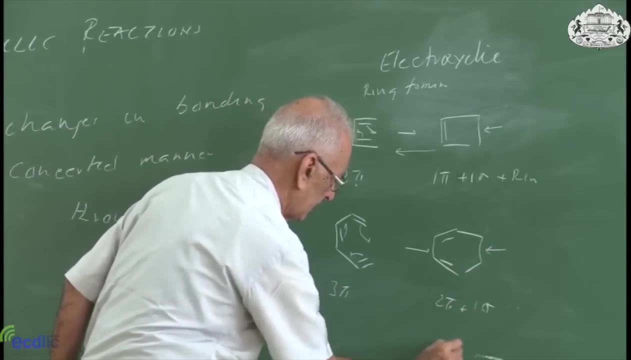 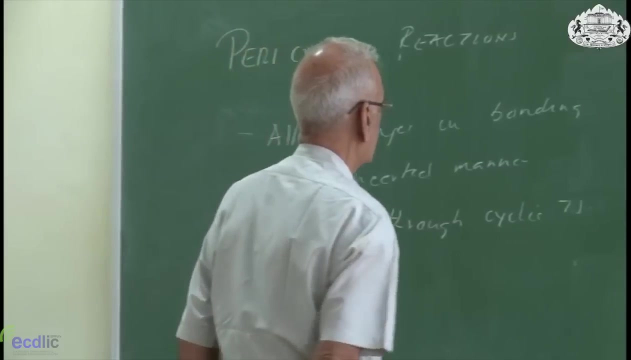 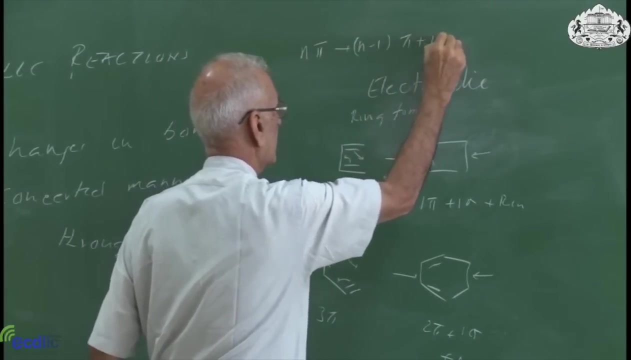 the left hand side I have three pi bonds. If I look in the product I have two pi bonds, I have made one sigma bond and I made a ring. So in an electrocyclic reaction what we are Putting is we are going from n pi bonds to n minus 1 pi bonds plus a sigma bond plus 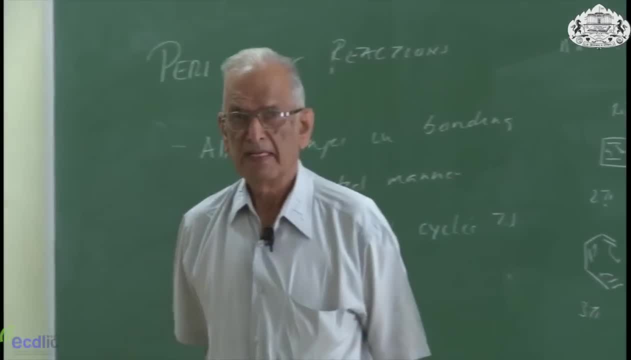 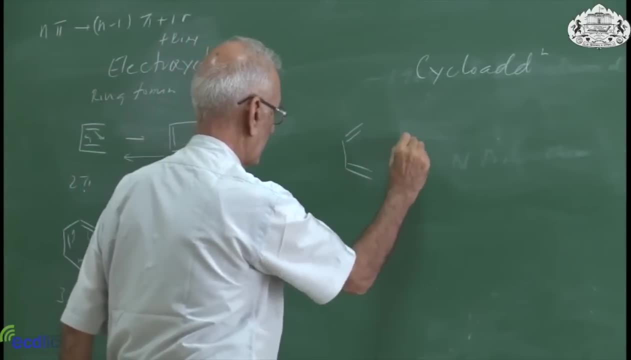 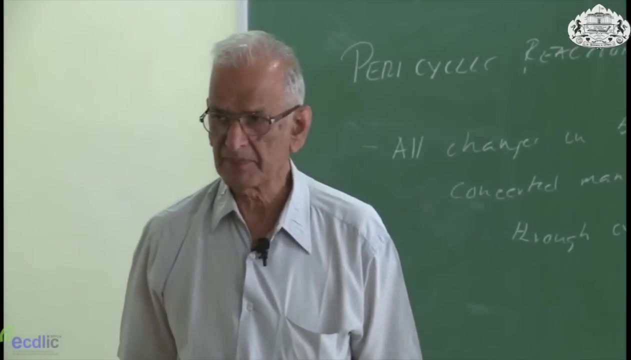 a ring In our next group of reaction, the cyclo addition. that is a very famous reaction. What is this very famous reaction? Diels-Alder, Diels-Alder, Diels-Alder, Diels-Alder, Diels-Alder. 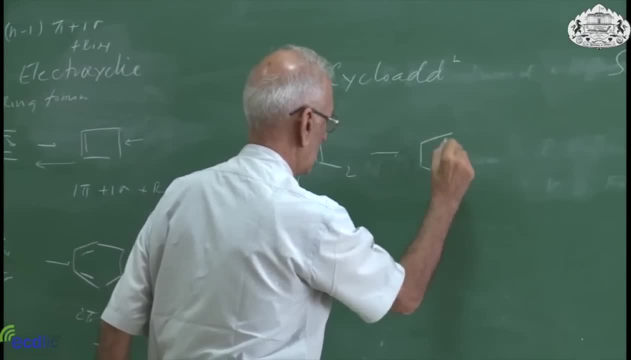 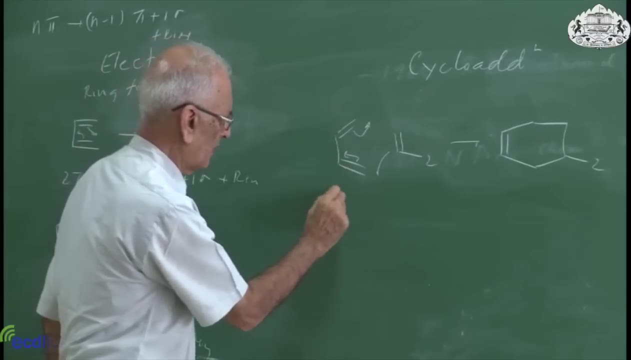 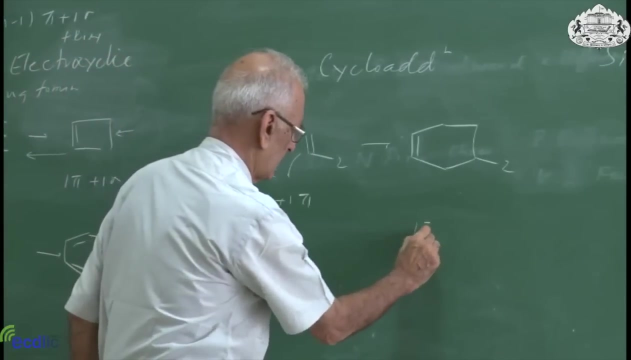 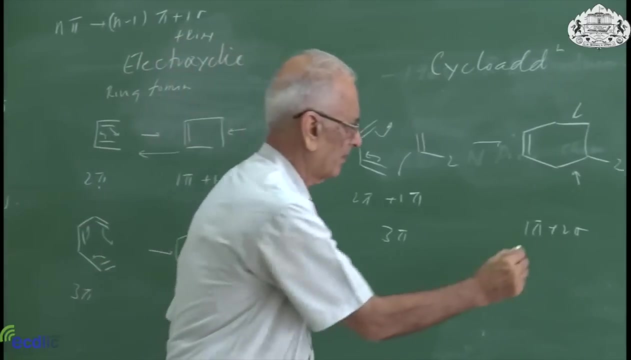 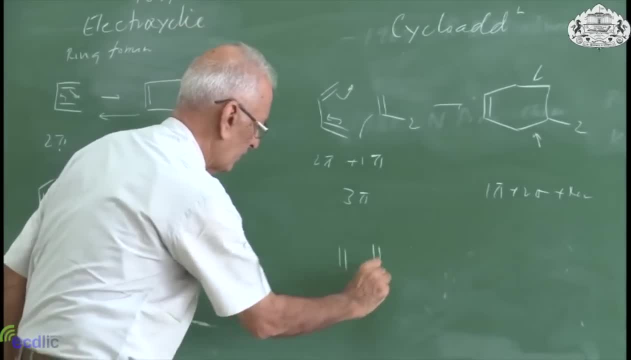 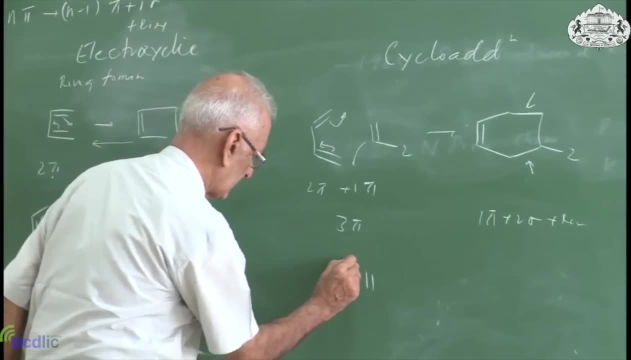 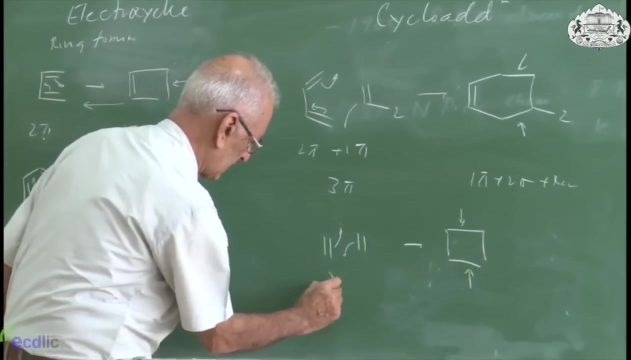 ring. Another example of this: a ring. In the next group of reactions we are going to look into the cyclo addition. In the next group of reactions we are going to look into the cyclo addition would be the reaction of two, two molecules of ethylene to give you cyclobutane, So on. 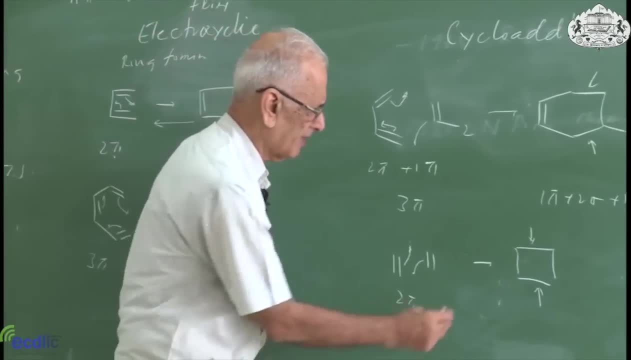 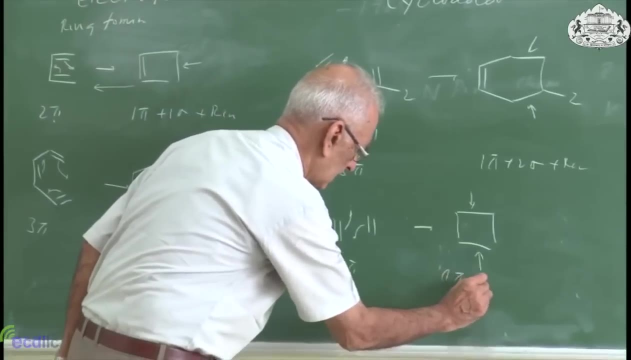 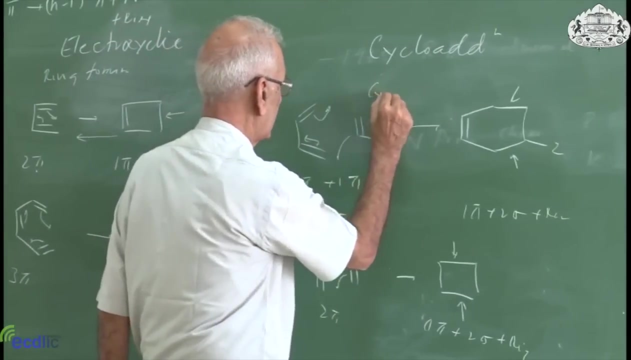 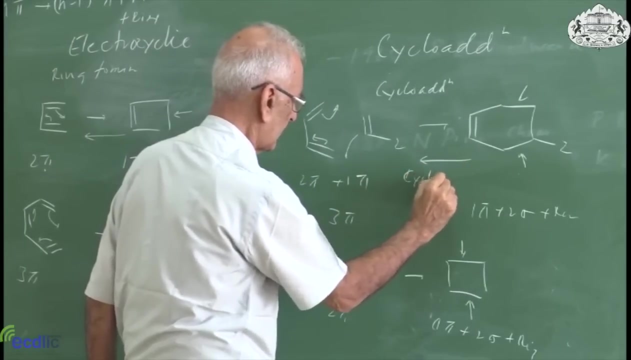 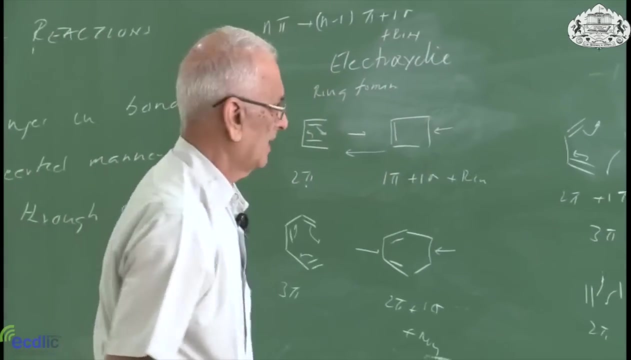 the left hand side. one plus one pi bond total two pi bonds. we have made two sigma bonds plus a ring. If I go from left to right I call it as a cyclo addition. If I go from right to left, this is a cyclo reversion. So in a cyclo addition I am going from n. 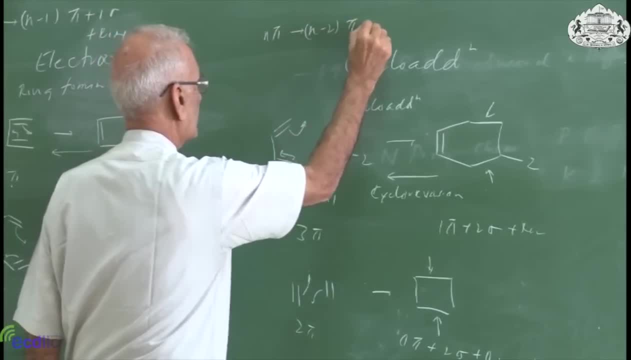 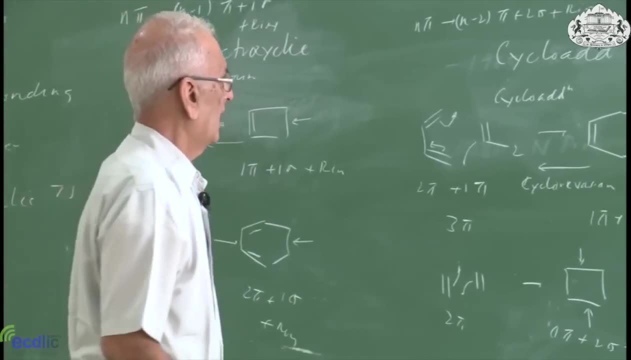 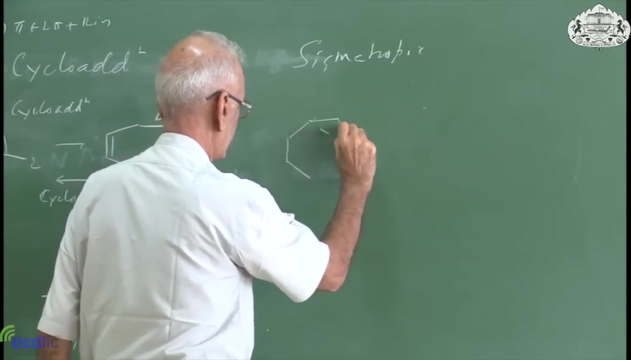 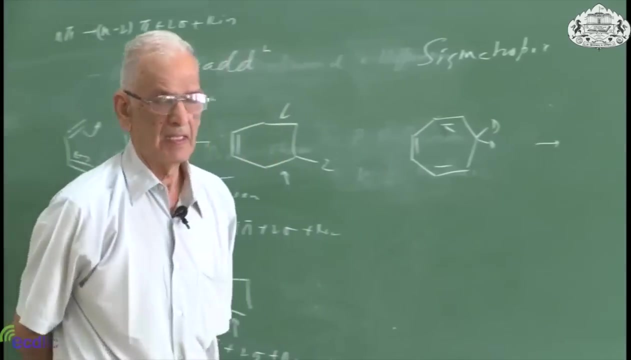 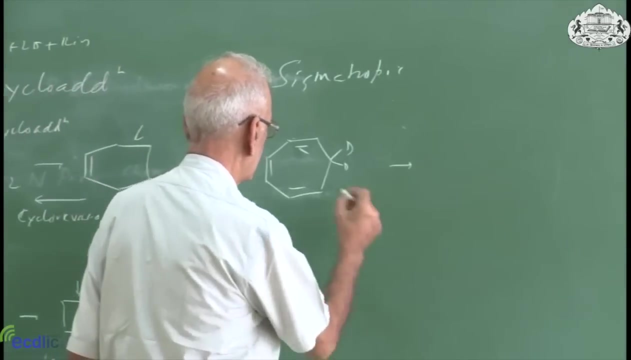 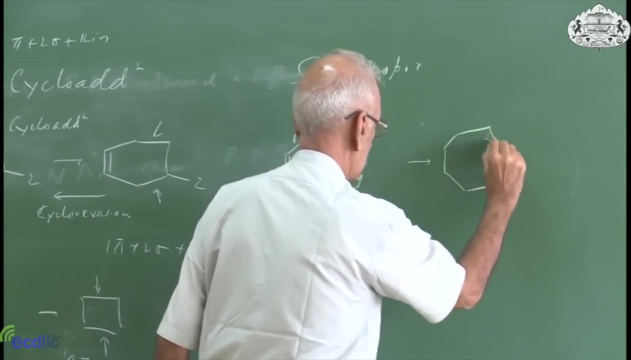 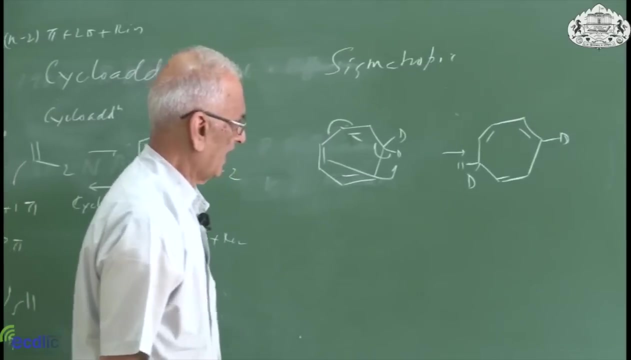 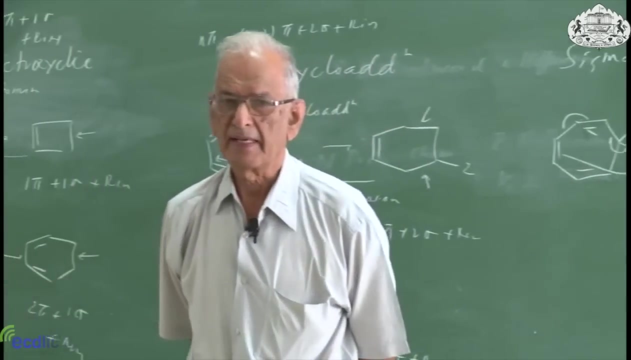 pi to n minus 2 pi. My third type of reaction is a sigmatropic reaction. I look at this deuterated cyclohepatrine. What have I done? I have broken the sigma bond at one place and formed the new sigma bond at a different place. Why have I shown? this arrow, It must involve a cyclic transition state. If it does not involve a cyclic transition, it is not going to be a pericyclic reaction. So number of double bonds: three pi one ring, three pi one ring In an electro cyclic will go from n pi to n minus 1 pi In cyclo addition. you go from n pi to n minus 2 pi In a sigmatropic, no change in number of double bonds, even an in number of ways. Another example of the sigmatropic reaction is this: Let us look on the left hand side: total 4 pi bonds in the product: 1, 2,, 3, 4,. 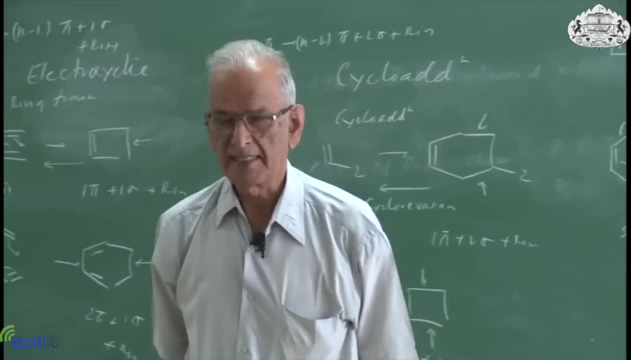 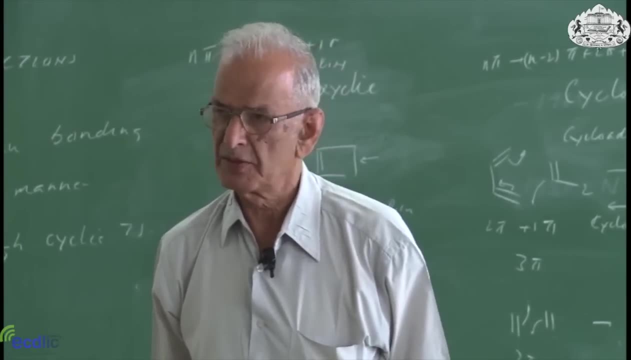 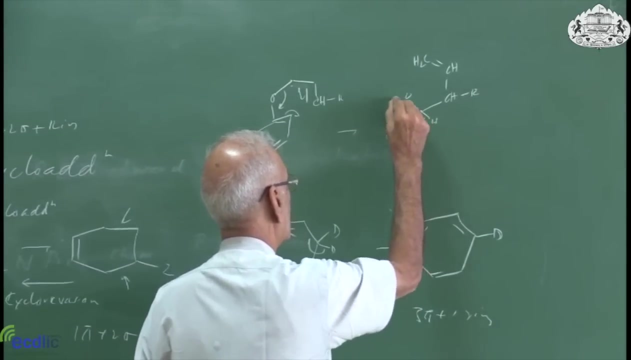 pi bonds. Starting material: 1 ring 4 pi bonds. product has got 1 ring 4 pi bonds. no change in number of double bonds, no change in number of ring. What is the last step of this reaction? Compound becomes aromatic. 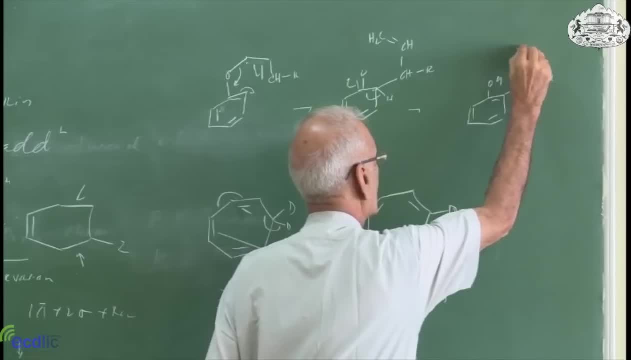 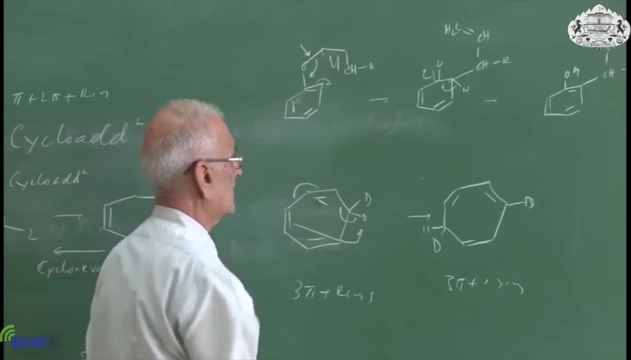 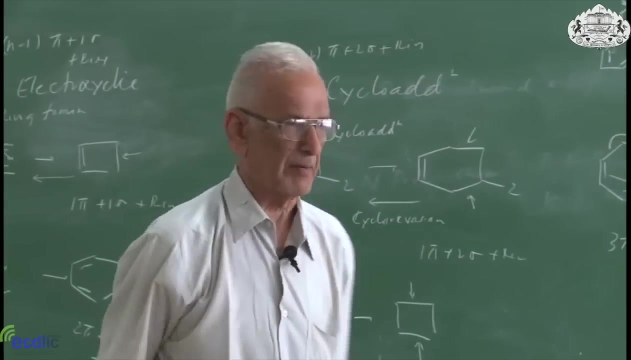 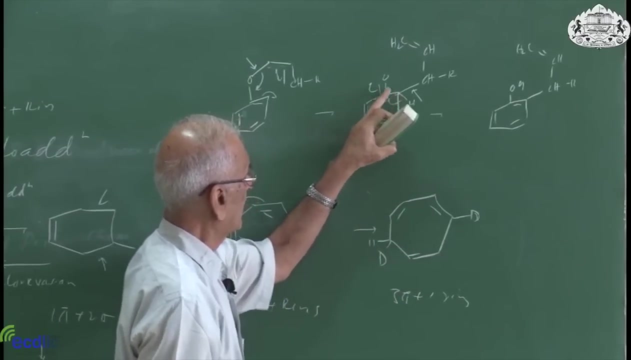 Compound becomes aromatic. What have we done in the first step? We have broken the sigma bond at this place. We have formed a new sigma bond at a different place. If I look at this step, I have broken the sigma bond, this sigma bond, I have formed the new sigma bond here. This step is not. 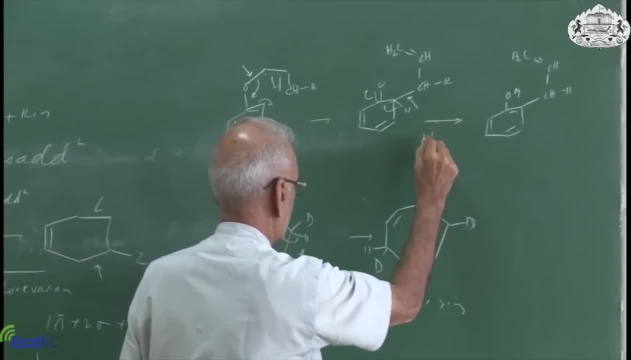 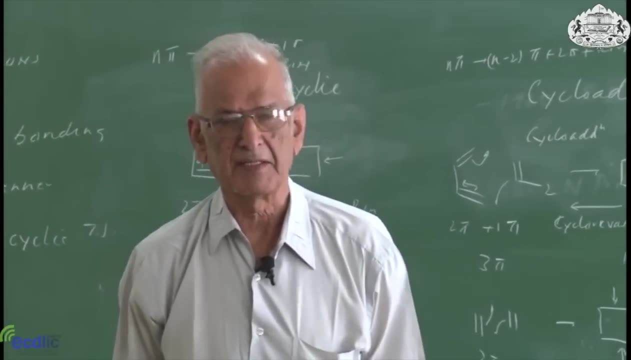 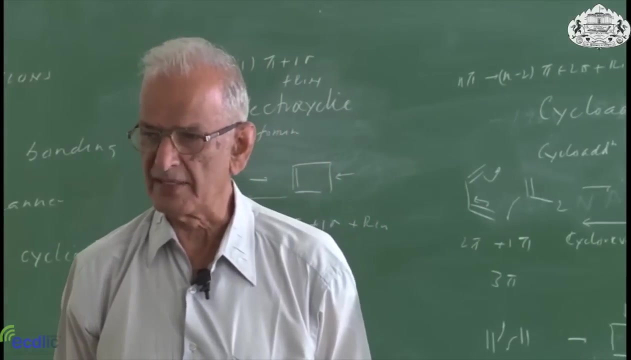 called as a pericyclic reaction because it is atmospheric. This is called acid catalyzed And, as we will see, when we give the features of a pericyclic reaction, we say that in a pericyclic reaction there is no significant role for acid role-base. So the first step, 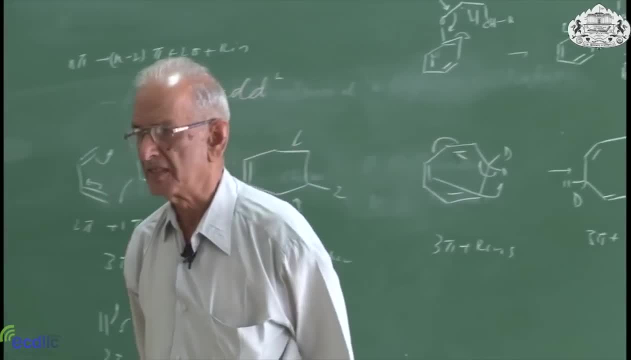 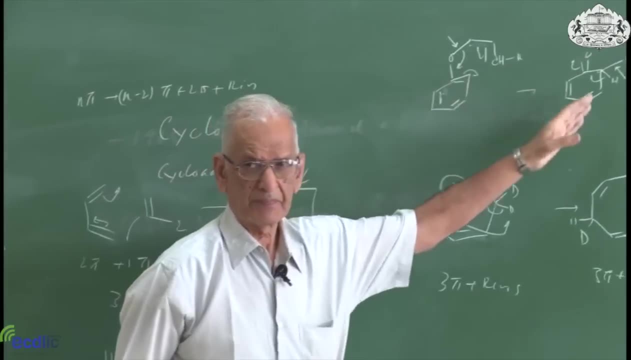 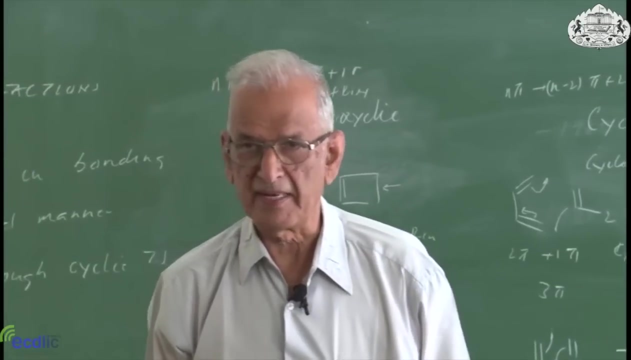 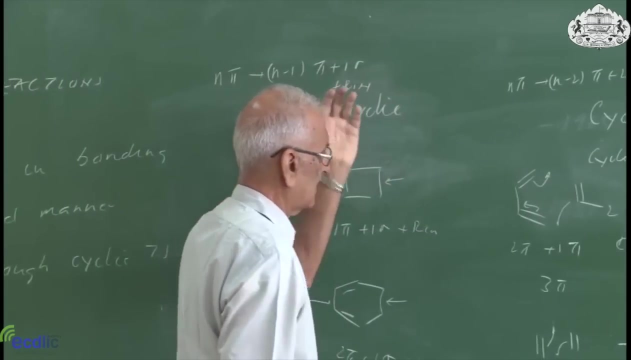 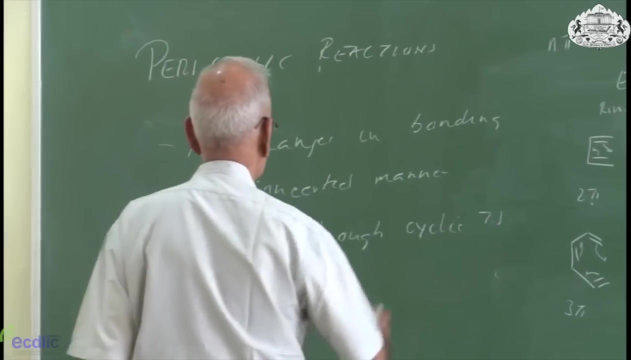 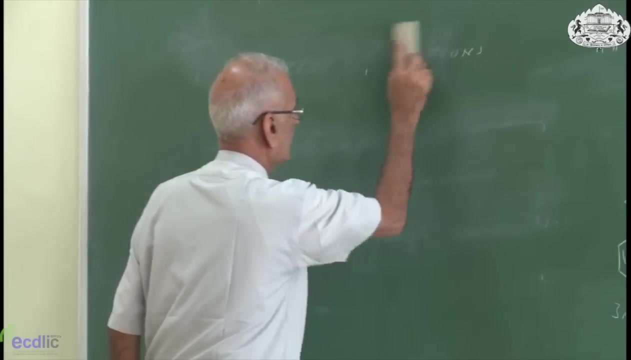 is pericyclic. the second step, aromatization, is not a pericyclic reaction. What is this very famous reaction? This is the Claisen rearrangement. So we have given our classification: electro cyclic, cycloaddition, sigmatropic. Now we are looking at our next, that is, what are the features? 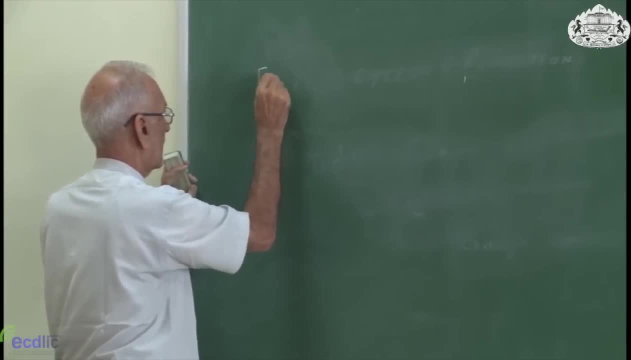 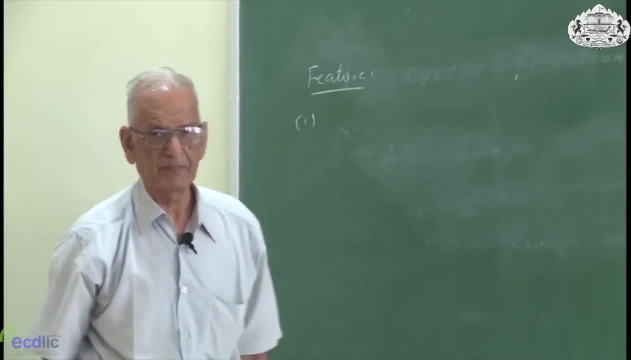 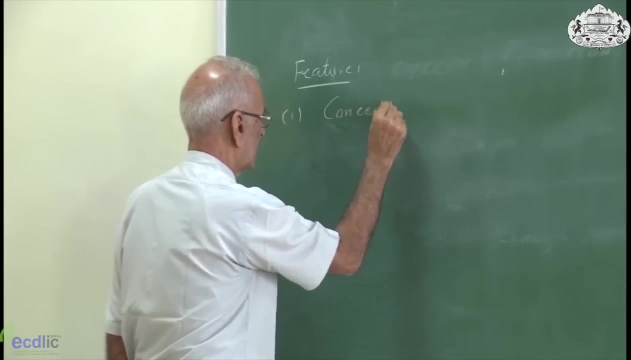 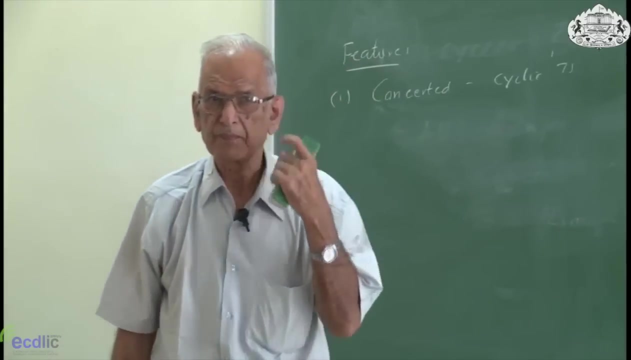 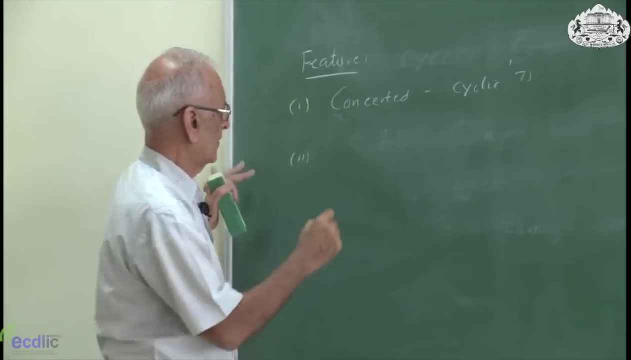 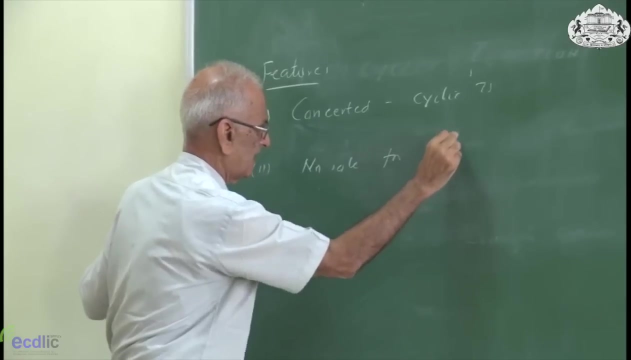 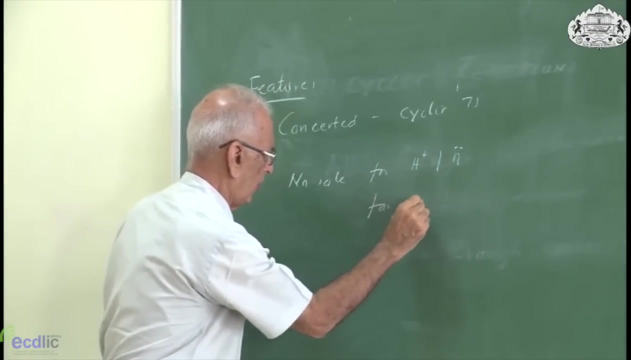 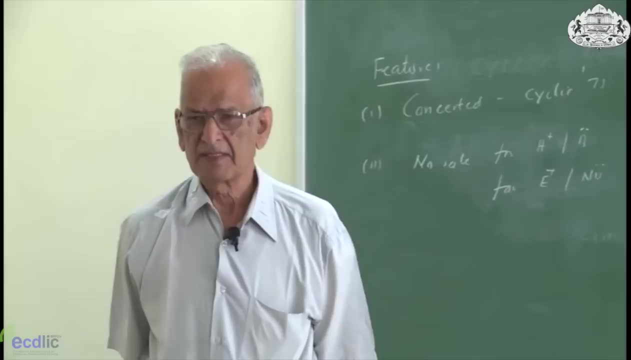 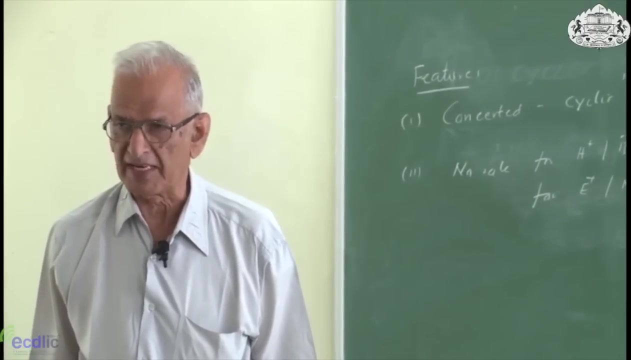 of a pericyclic reaction. Obviously, feature number one: it must be concerted and it must involve cyclic transitions. No Number two: no role for acid or base, no role for electrophiles or nucleophile. These features obviously differentiate a pericyclic reaction from an ionic reaction. 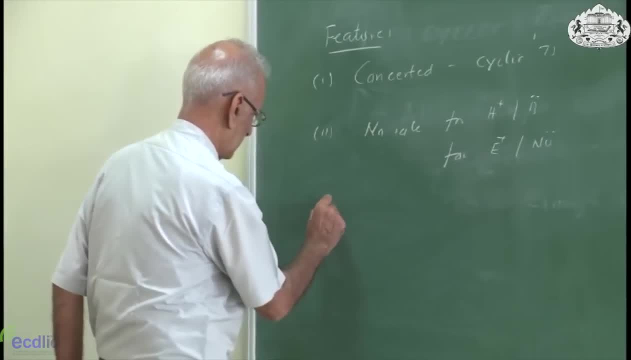 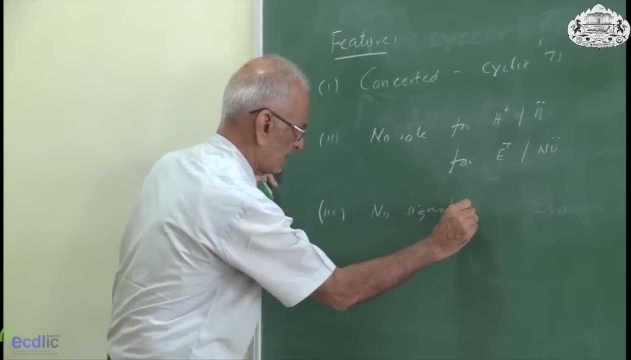 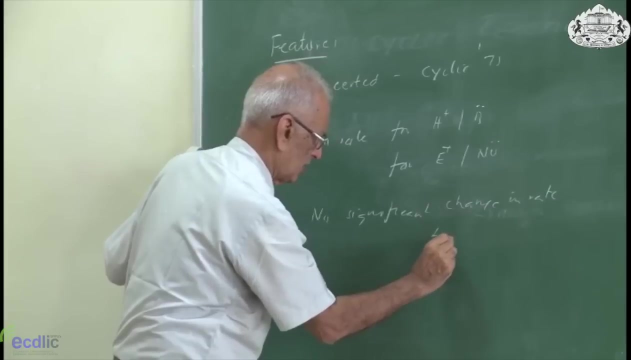 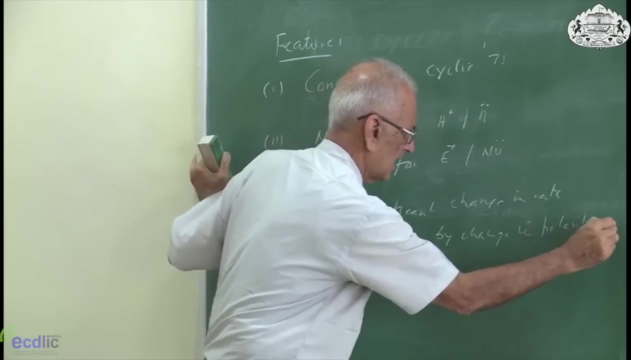 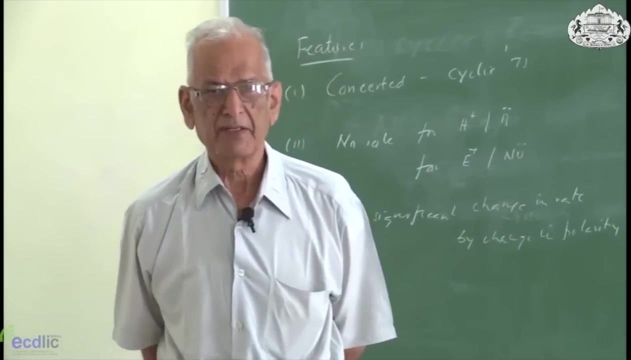 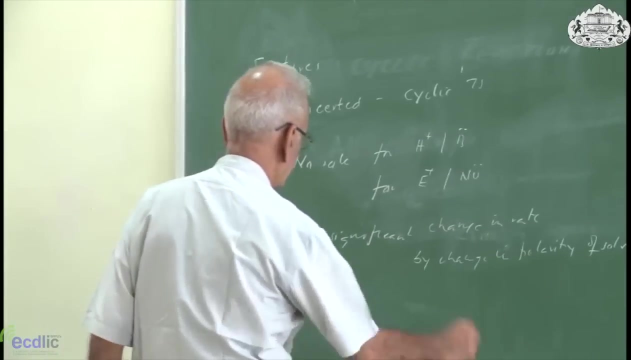 No significant change in rate by change in polarity of solvent. As you are well aware, if it is polychromic freezing then the polarity is not very important, but it is very important it is ionic. when I change the solvent make it more polar, reaction rate increases No. 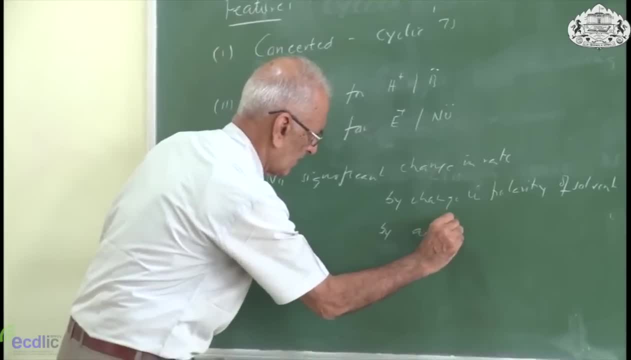 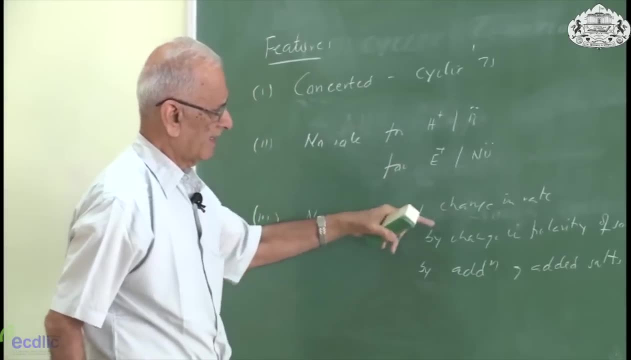 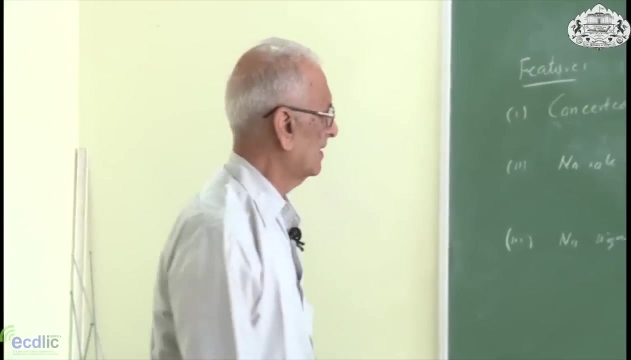 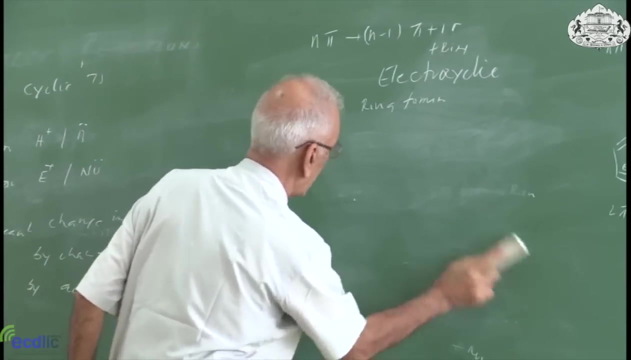 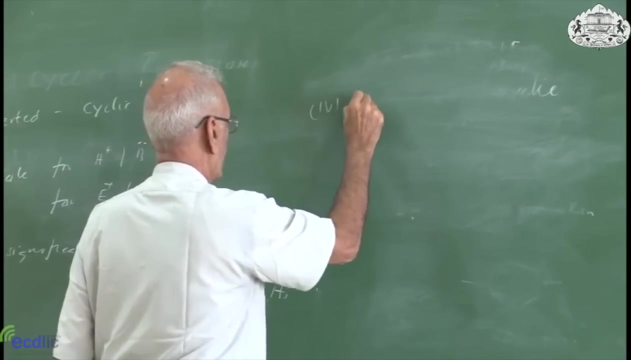 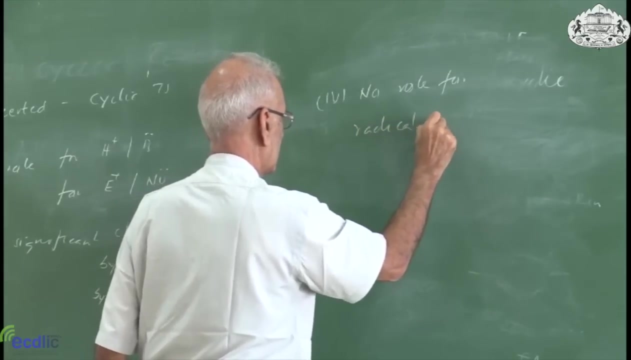 change in rate by addition of added salts. So, once again, that is a feature which differentiates pericyclic from ionic reaction. What is the feature that will differentiate pericyclic from radical reaction? No role for radical initiators. I put it in. 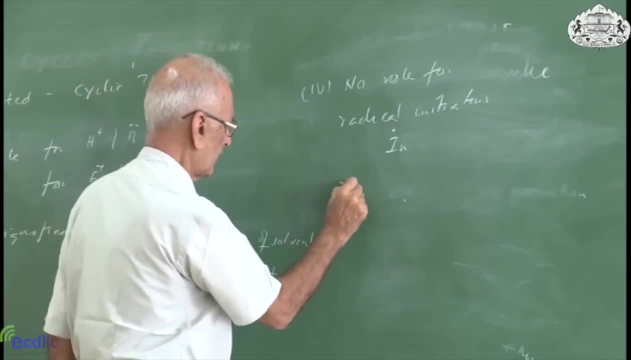 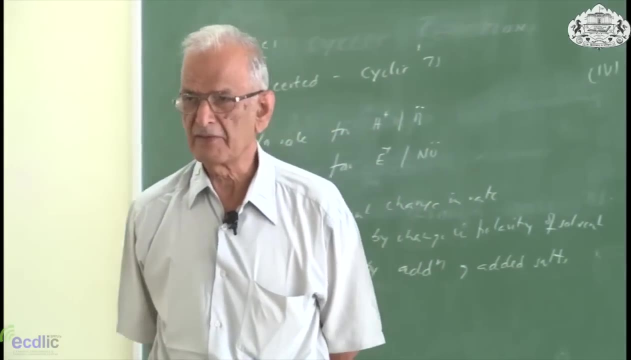 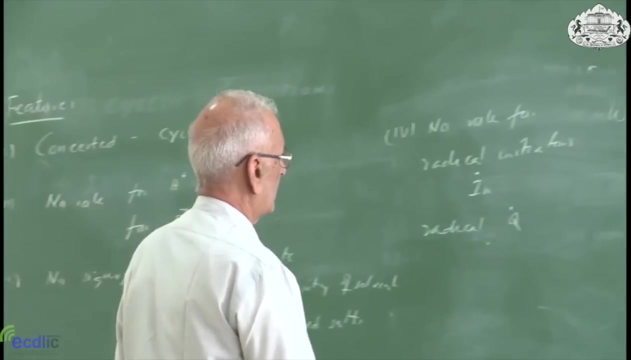 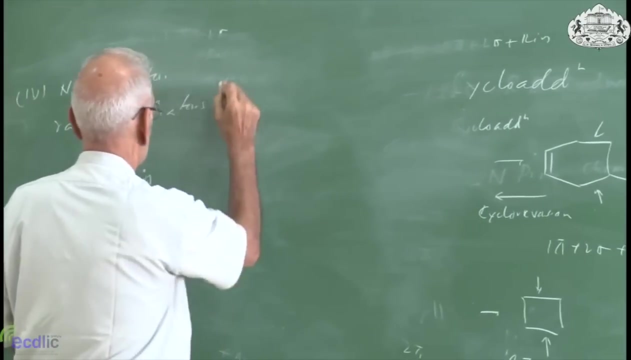 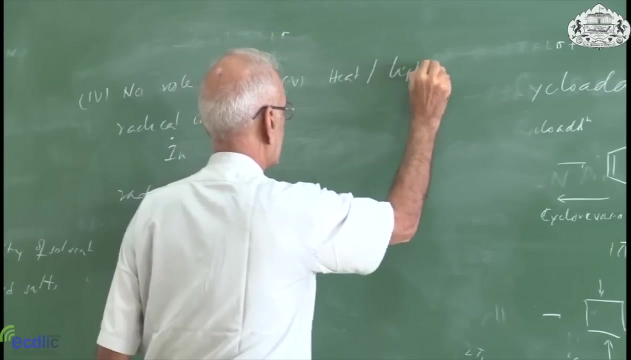 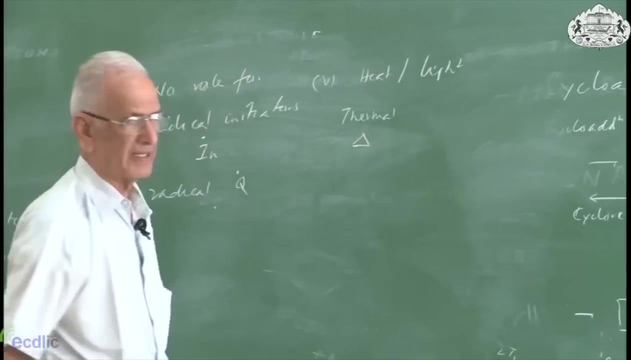 like this radical initiator or radical quencher. Obviously, this differentiates a pericyclic reaction from a radical reaction. Reaction is carried out either with heat or light. When we do it with heat, we call it as a thermal reaction and we show it as a. 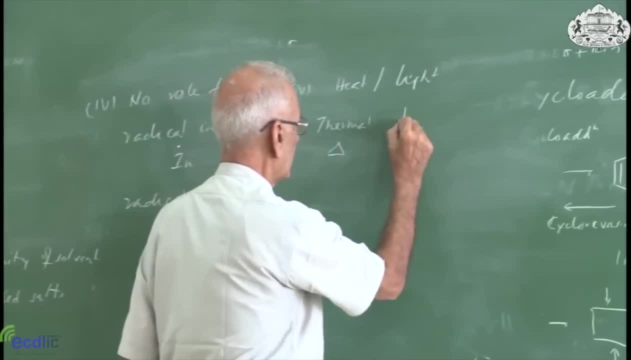 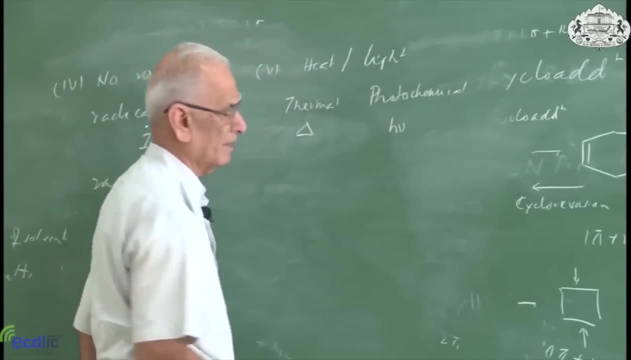 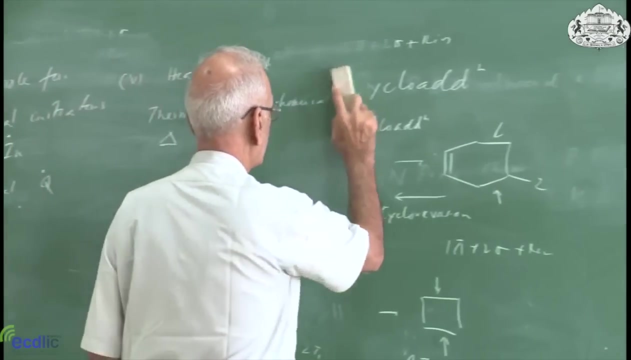 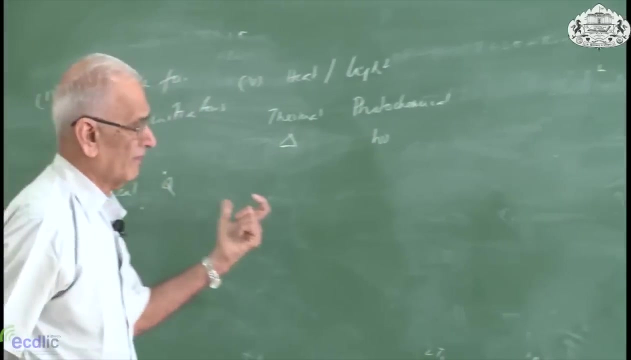 triangle. When we call it, do it with light, we call it as a photochemical reaction and show it by the symbol h nu. The important aspect of this is the reaction rate, is not the difference between two. When I do this, if I do it with heat, I get one stereochemical. 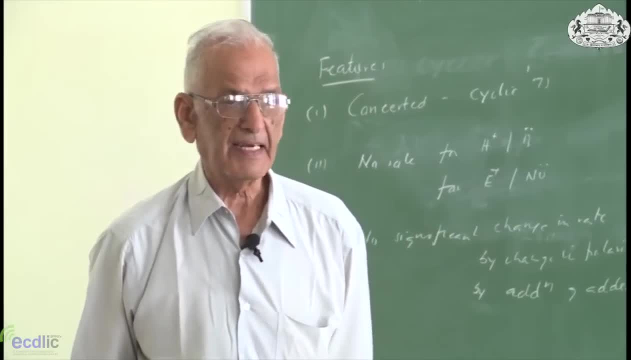 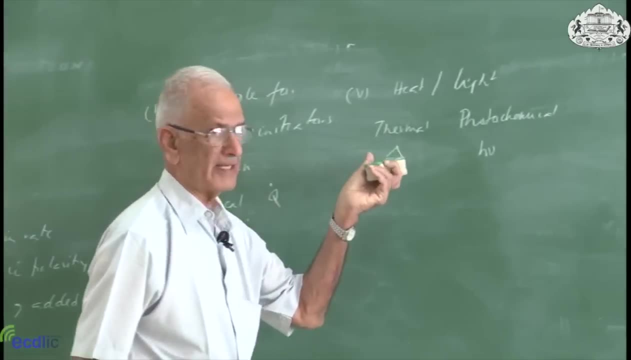 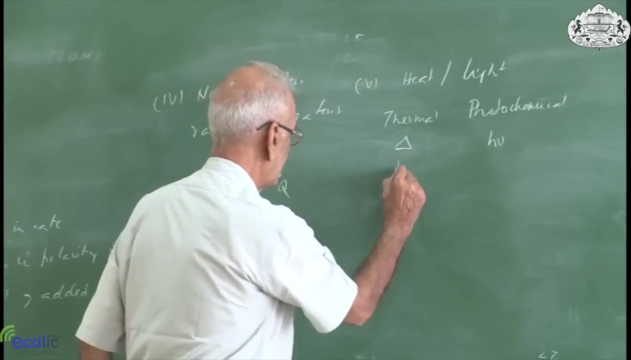 result. If I do it with light, I get a different stereochemical result. Therefore, it is not that this is only supplying energy. there is an important difference between these two. When I do it with heat, reaction takes place from vibrationally excited material, and when it is heated, the reaction takes place from the energy field which is sent. When I do it with heat, it is a different result. Then, when I do this, the heat is怎么样, which is not a material. in any case, the energy is separated from the material, for the same. 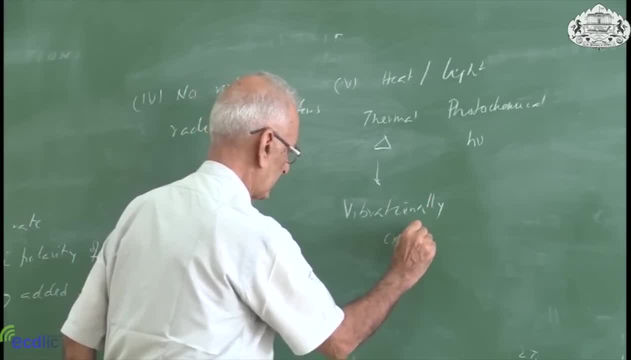 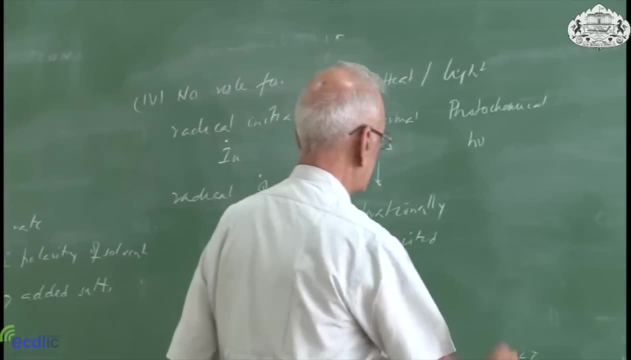 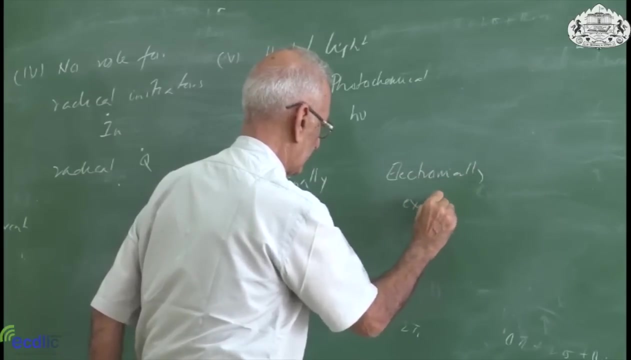 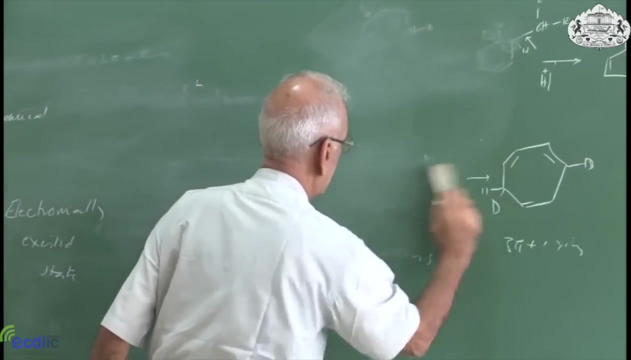 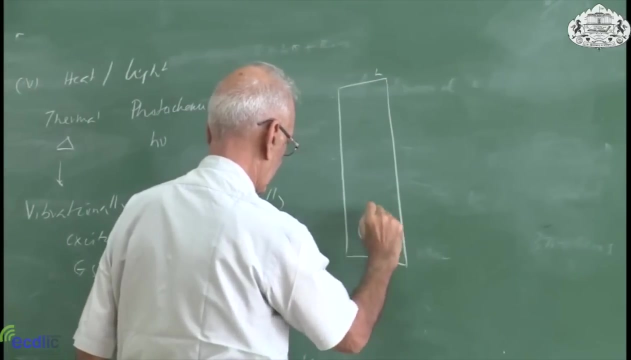 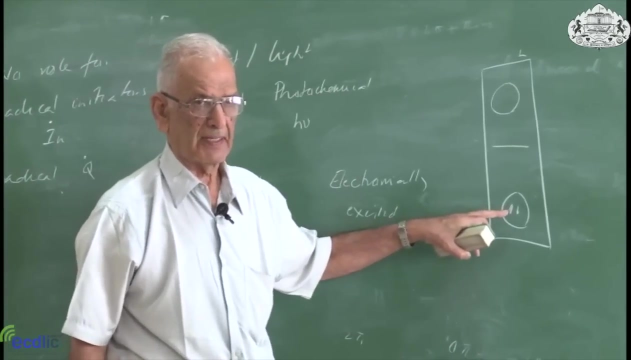 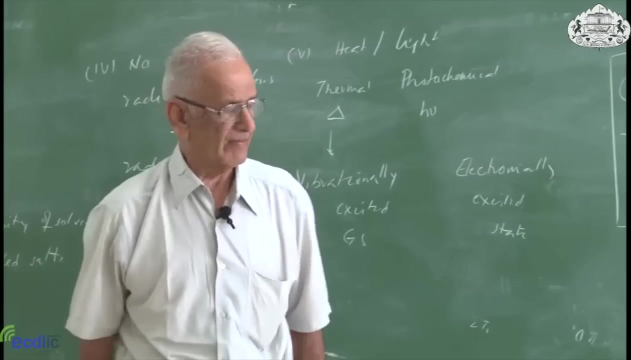 When I do it with light, reaction takes place from an electronically excited state. Let us clarify what exactly we mean by this. This is your bonding orbital and that is your anti-bonding orbital. So in a thermal reaction we have electrons only in bonding orbitals we do not have any. 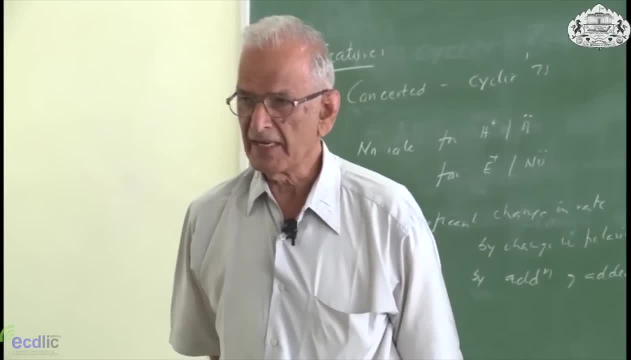 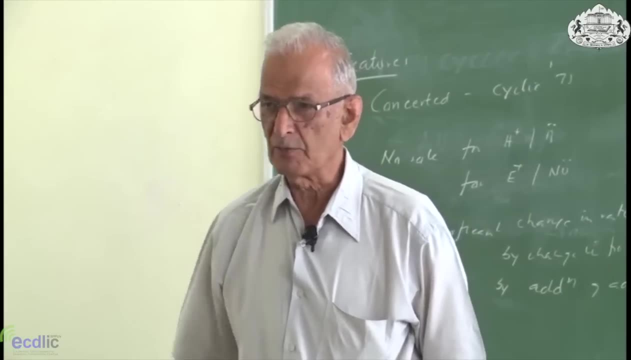 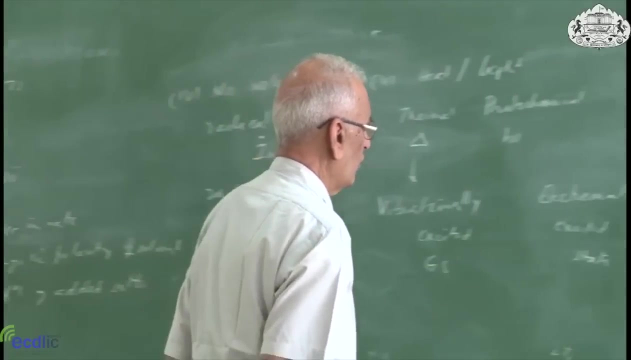 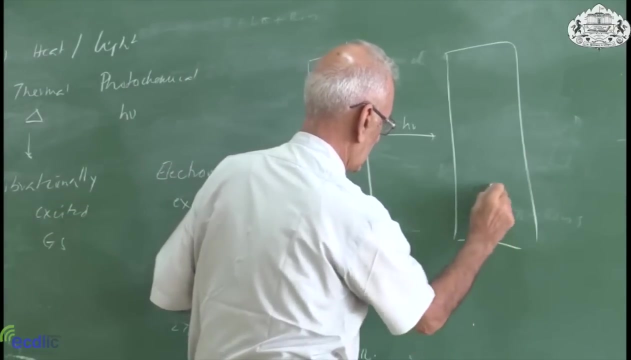 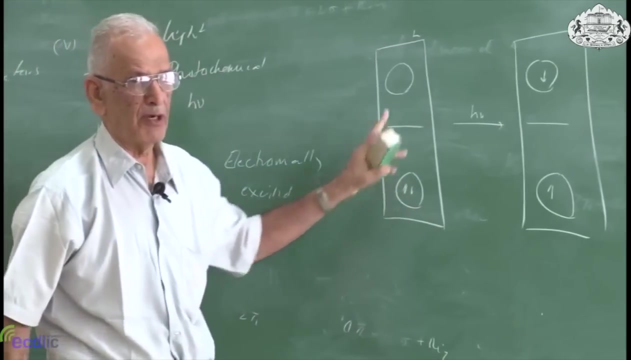 electrons in bonding orbitals We give energy that still remain only in the bonding orbitals, supplying energy to go from ground state to excited state, but which is still in bonding orbitals. When I do a photochemical reaction, electron goes from bonding orbital to anti-bonding orbital. 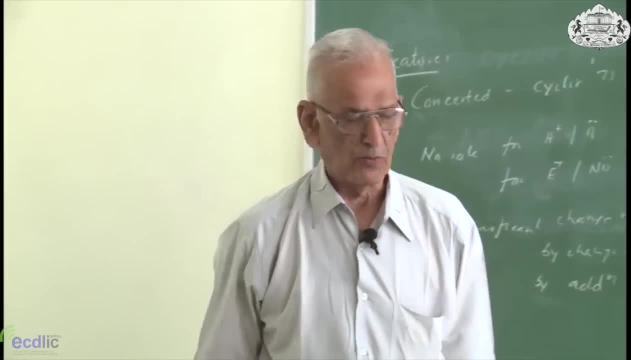 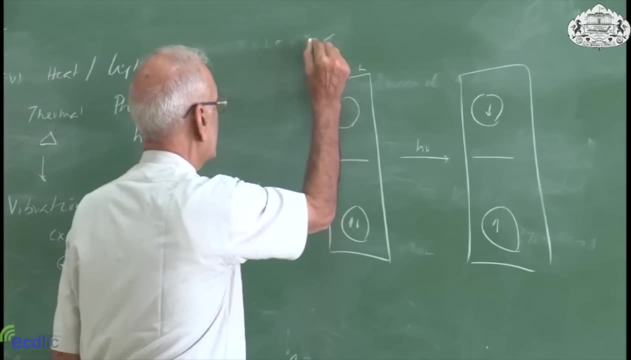 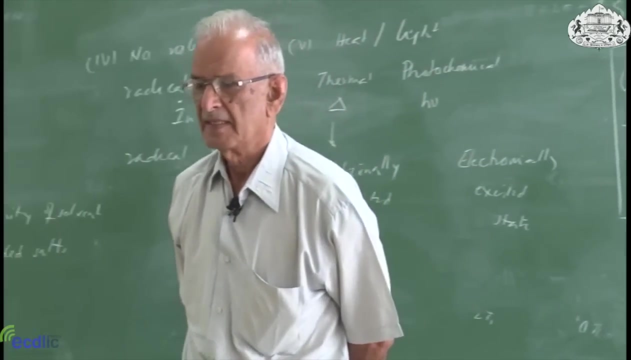 Earlier, the anti-bonding orbital was vacant, So electron has been transferred from bonding orbital to anti-bonding orbital. This is called as the ground state singlet. This is excited singlet. Electron has gone from bonding orbital to anti-bonding orbital. 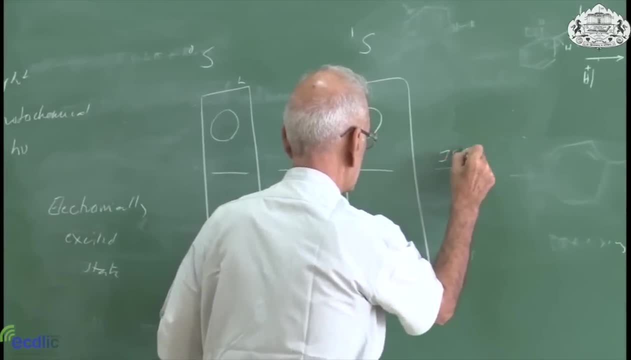 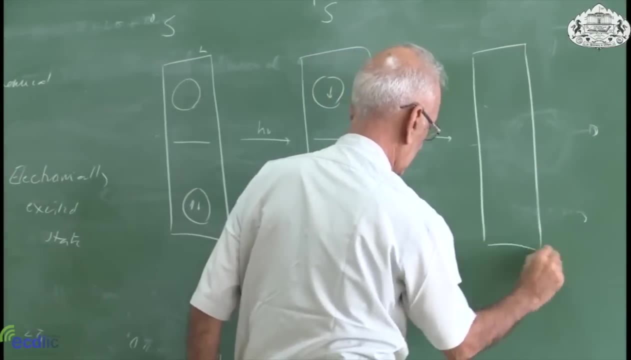 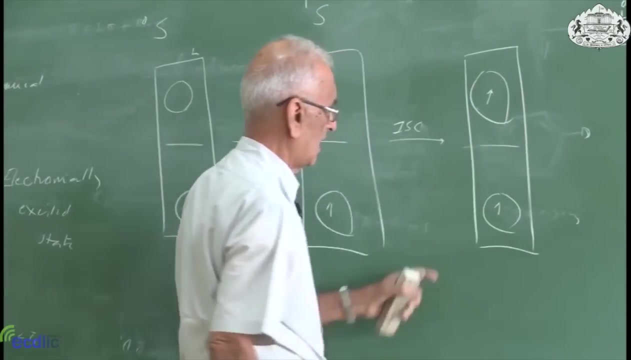 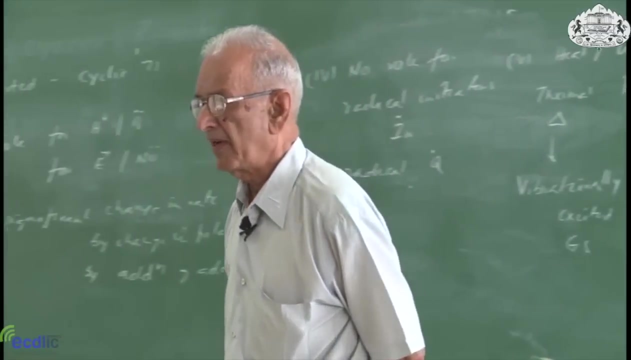 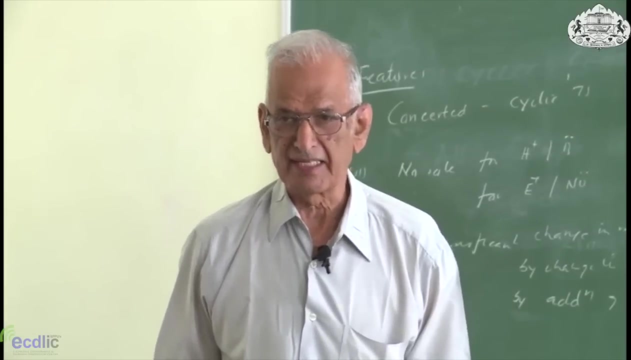 Then we have a process which we call as inter system crossing. What have we done now? We have changed the spin of this electrons. The Frank Kondal principle says that when I excite a molecule there is no change in spin but in the inter system crossing, the spin of 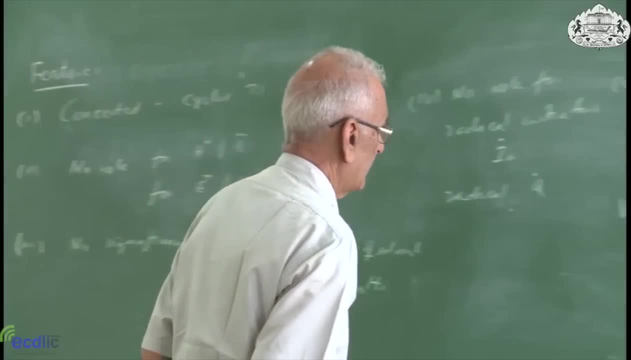 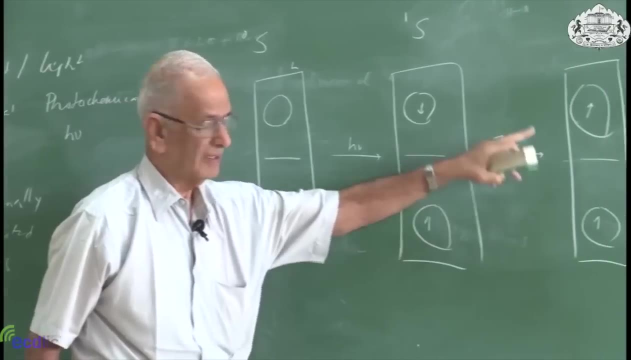 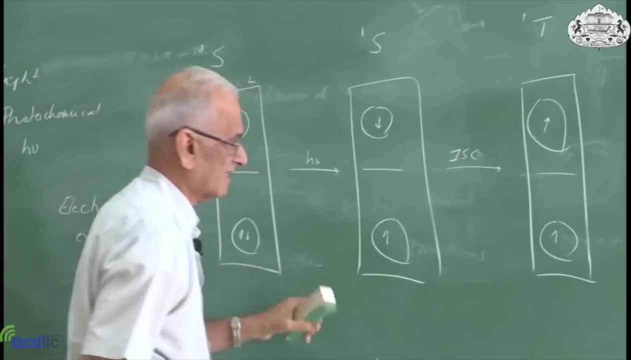 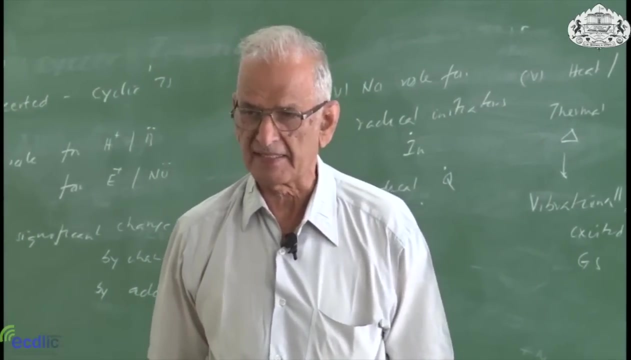 the electron becomes different. In this case both electrons have opposite spins. Here both electrons have the same spin. So we call this as a triplet excited state. Triplet excited states have long term spin. Triplet excited states have longer life time than singlet excited states. Why In singlet? when this electron comes back, it goes directly into ground state. But for this first spin inversion has to take place, and only then it can go to ground state. Therefore triplet excited states have longer life than singlet excited. Please note when I say longer life. 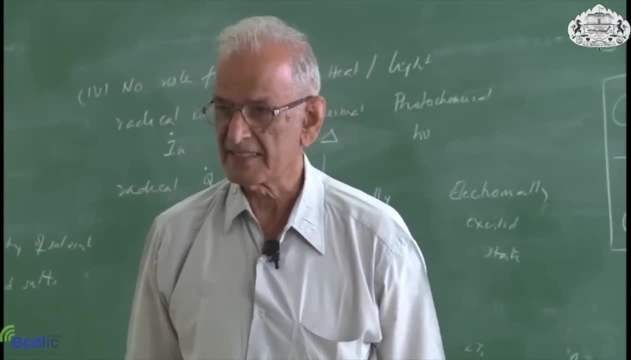 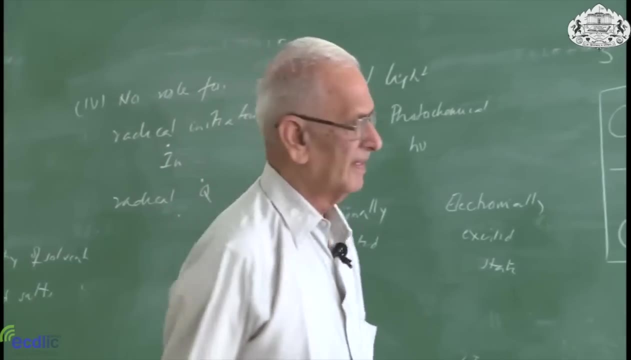 we are talking of triplet excited states. Triplet excited states have longer life than singlet excited states. So triplet excited. 10 raise to 6, 10 raise to 9 seconds. 10 raise to 6 to 10 raise to minus 9 seconds. So usually 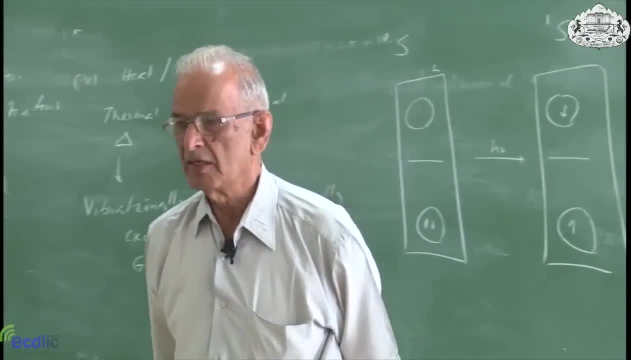 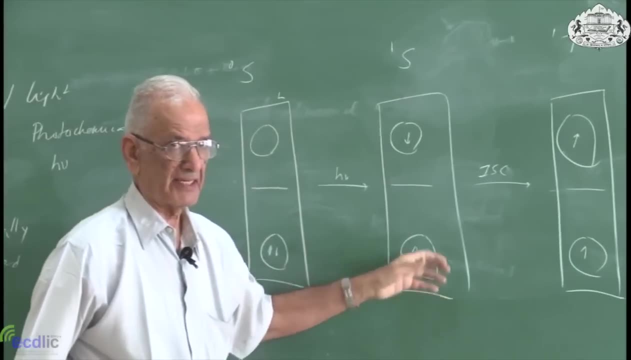 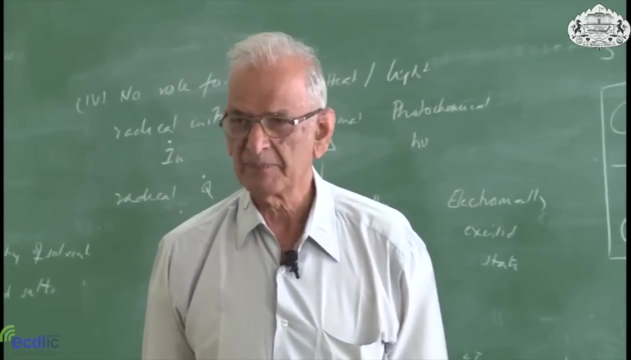 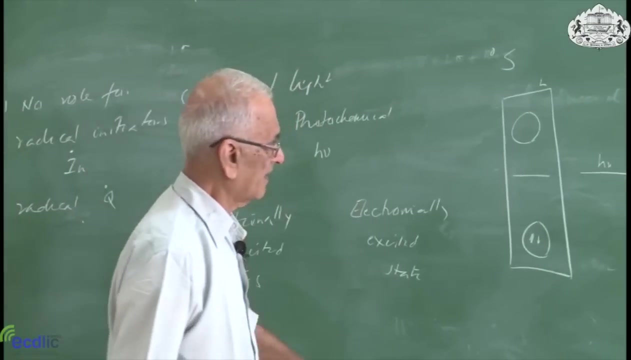 photochemical reactions take place from the longer lived triplet excited state and it does not mean that photochemical reaction does not take place from singlet excited state, but because singlet excited states are shorter lived, most often reaction takes place from a triplet excited. So the difference in stereochemical result is in thermal reaction. we are looking 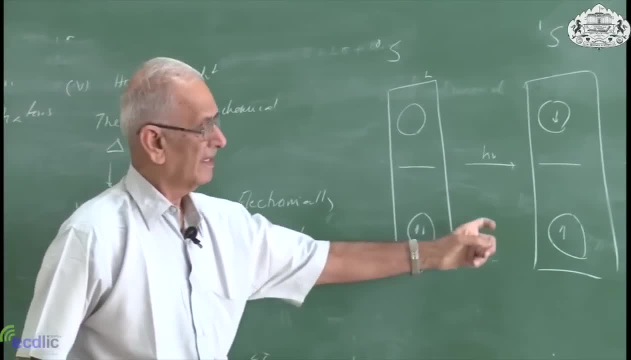 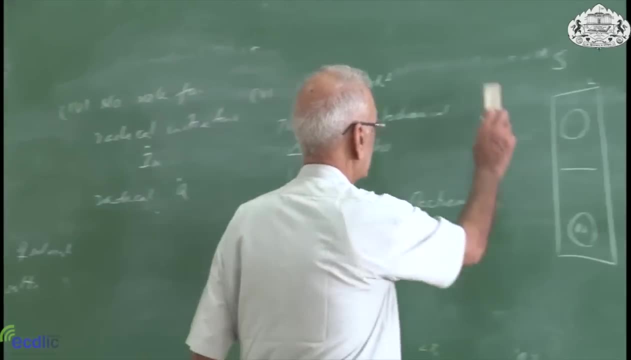 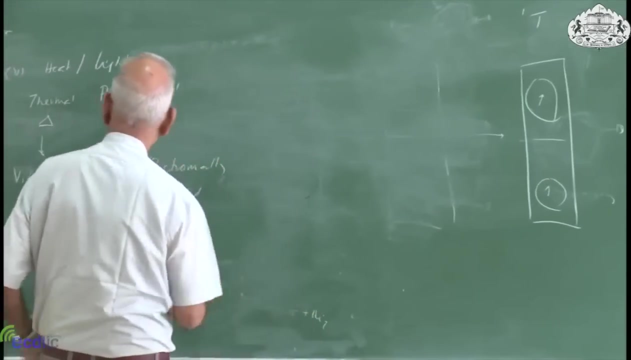 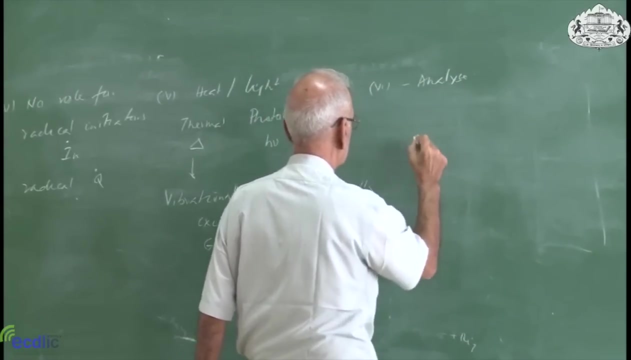 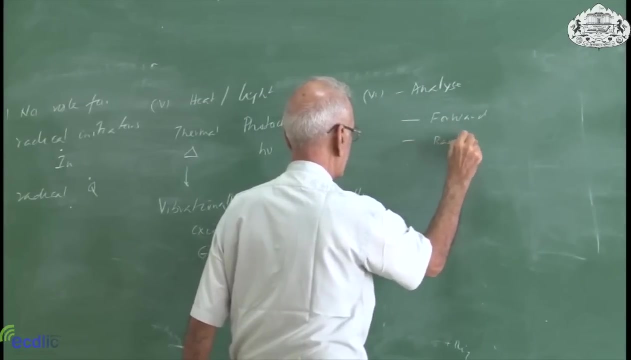 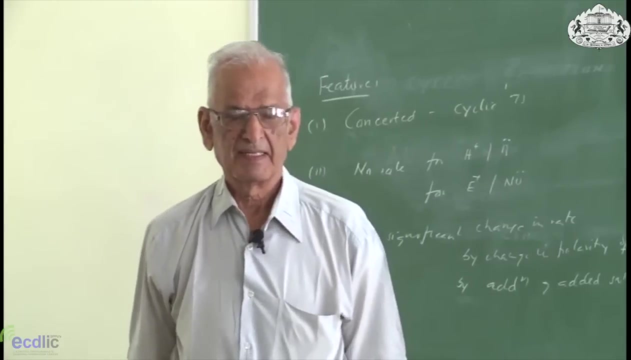 only at electrons in bonding orbitals in photochemical reaction. we are looking at electrons in anti-bonding orbitals. Thank you, We can analyze a pericyclic reaction by looking at forward reaction or by looking at back reaction. This is what is called as the principle of microscopic reversibility, If you know. 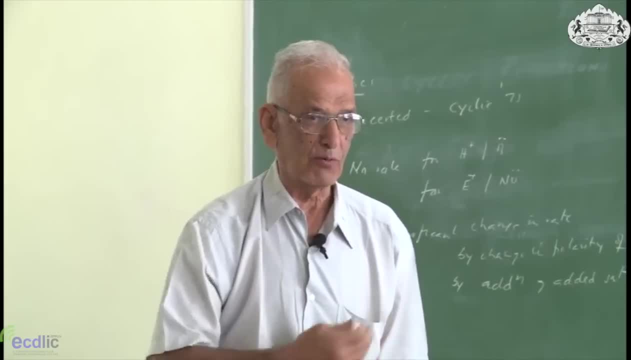 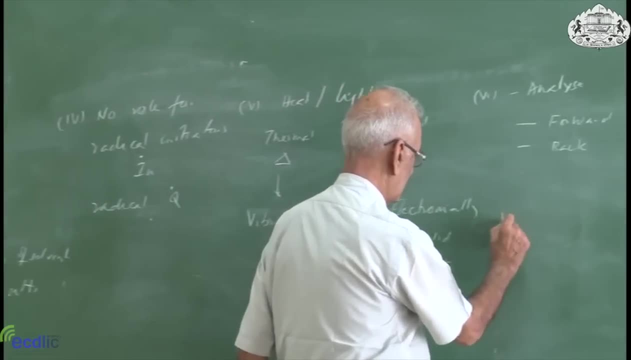 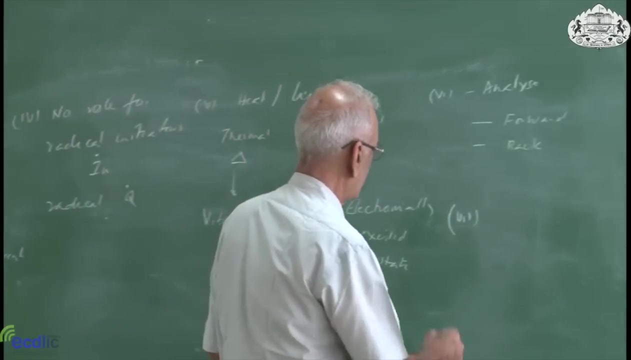 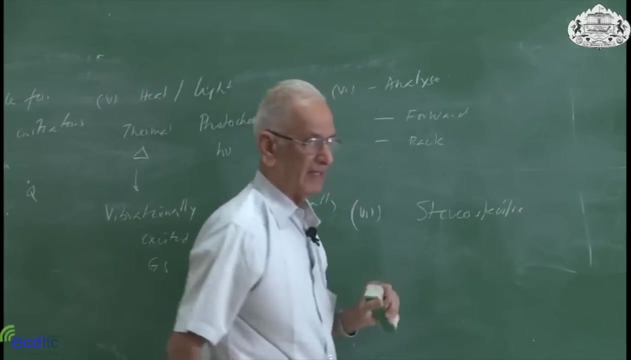 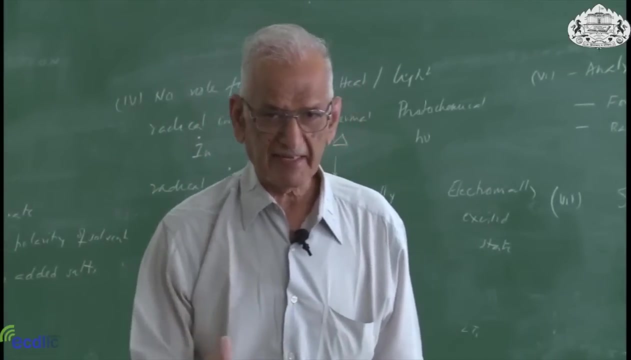 the way to go from Pune to Mumbai. obviously you know the road to come from Mumbai to Pune. that is the picture that we see. The seventh important feature is pericyclic reactions are usually stereospecific. Let me immediately add: ionic reactions can also be stereospecific. radical reactions can also. 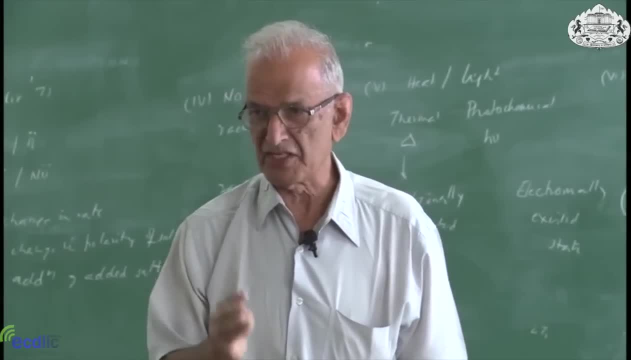 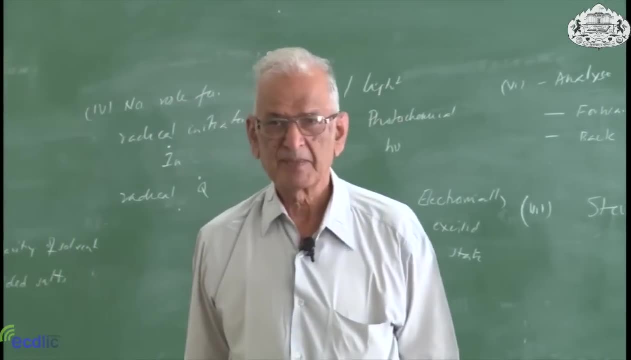 be stereospecific. So stereospecific does not differ, So stereospecific does not differ, So stereospecific does not differ. Now I want to differentiate this. What is an example of an ionic reaction which is stereospecific? Your SN2 reaction reaction. 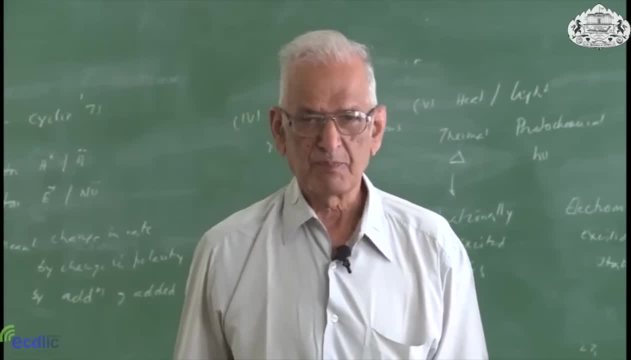 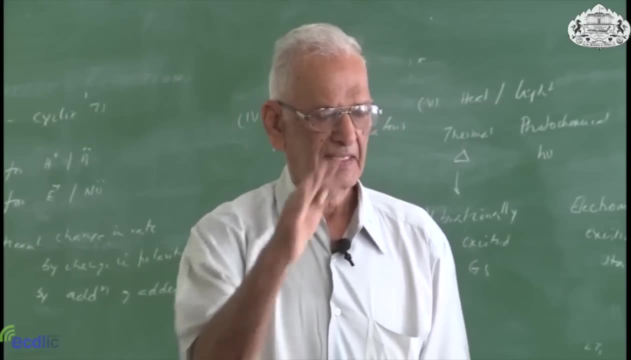 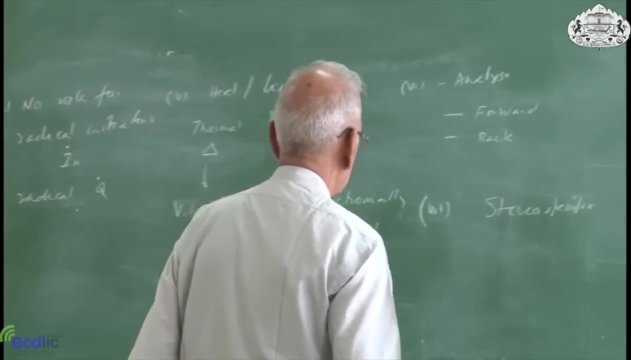 takes place to give you inversion of configuration. You talk of elimination. we talk of an ETU elimination. trans geometry will give you sorry. electro compound will give you trans geometry. Tiro compound will give you size geometry, Alright. So stereospecific kynanaut t motivates the radioactive� alum in 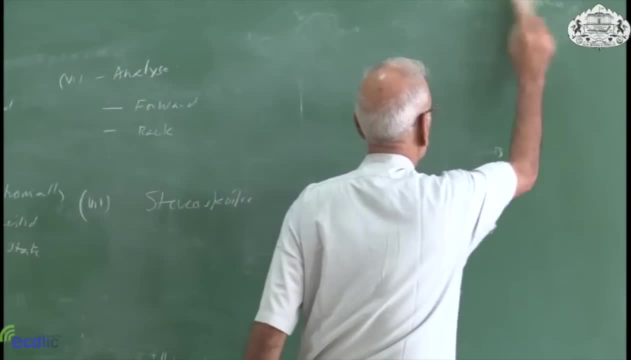 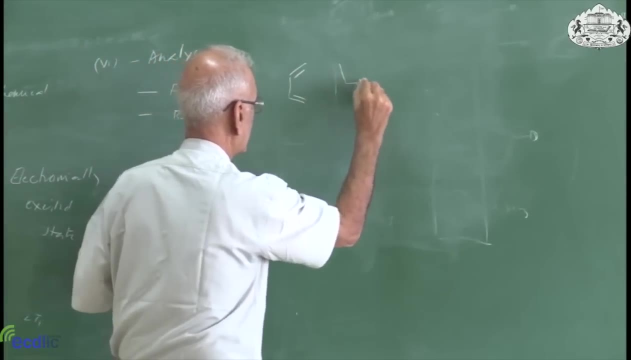 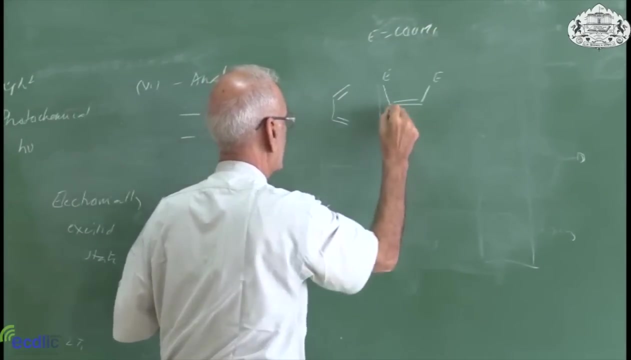 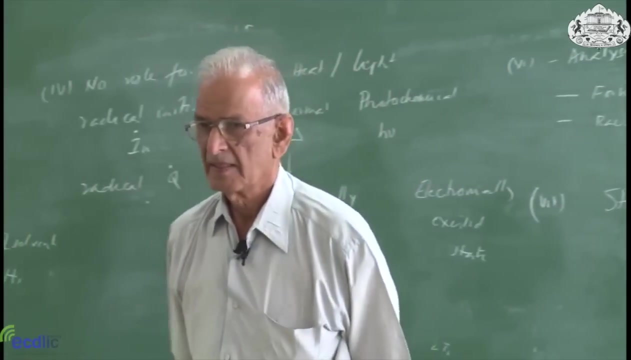 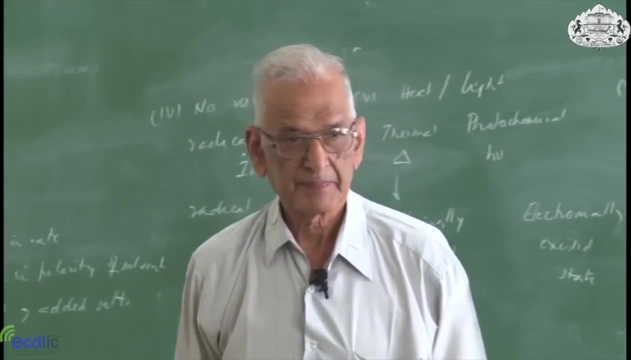 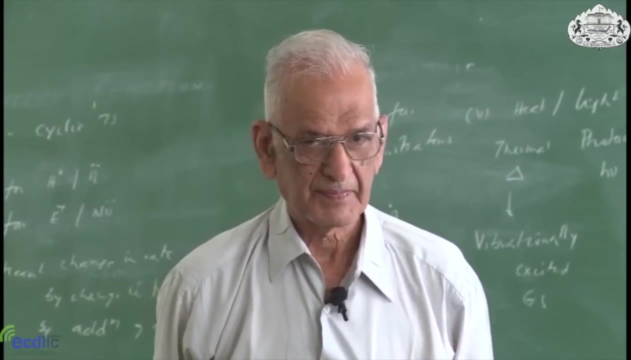 can get for ionic, you can get for radical, you also get for pericyclic. Let us clarify exactly what we mean by stereospecific. That is your ester. E stands for ester. What will you call this ester? What name will you give to this ester? 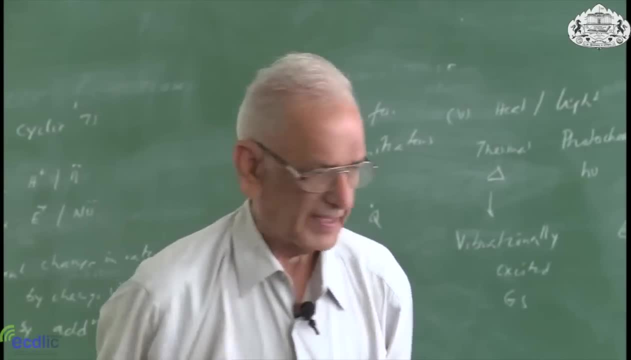 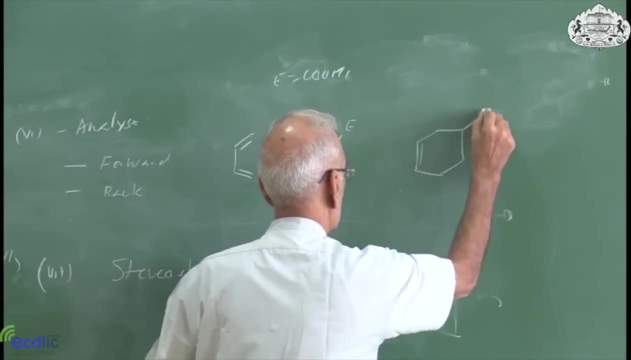 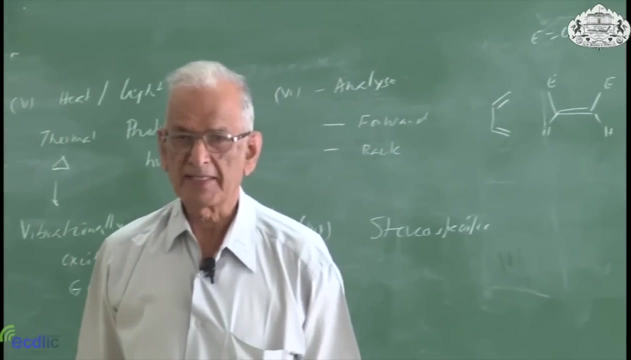 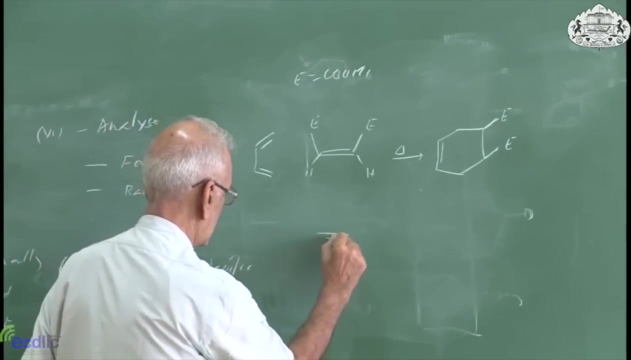 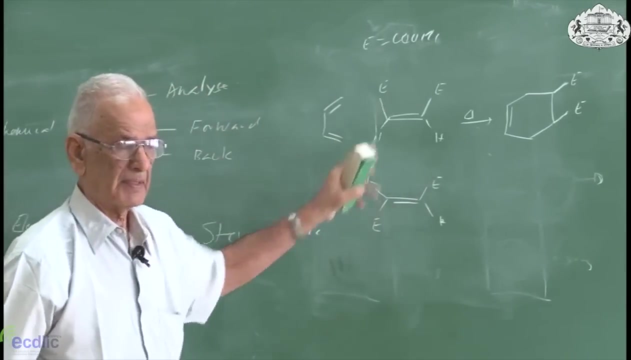 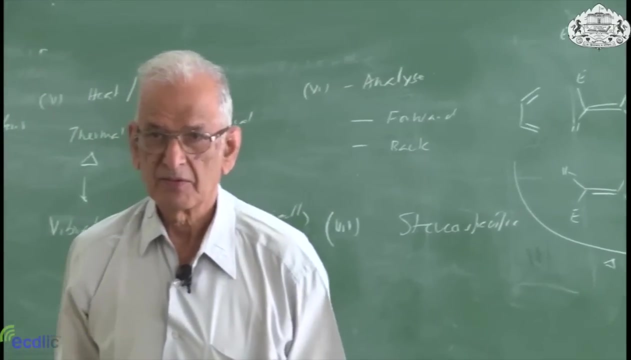 This is the ester of maleic acid. When I use this ester of maleic acid- this is the ester- I get product in which both ester groups are cis. If, instead of using maleic acid, I use what is this acid now, Fumaric acid, I use the ester of fumaric acid and I get 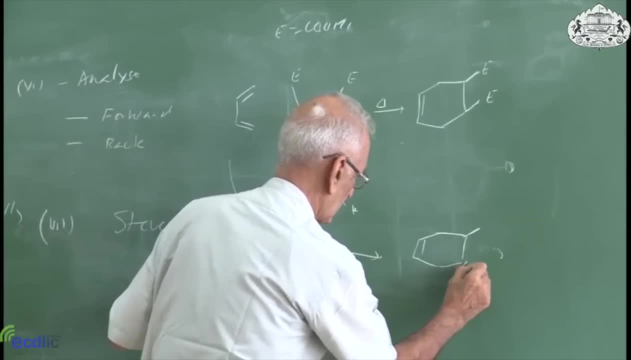 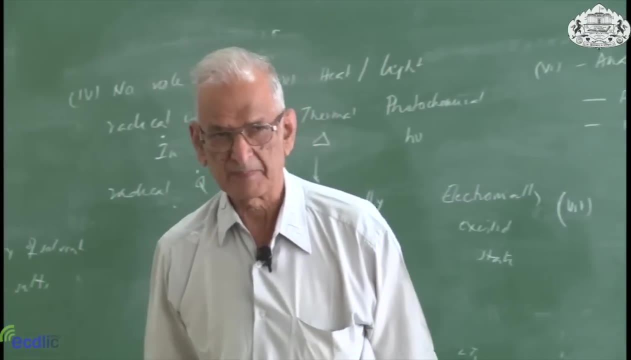 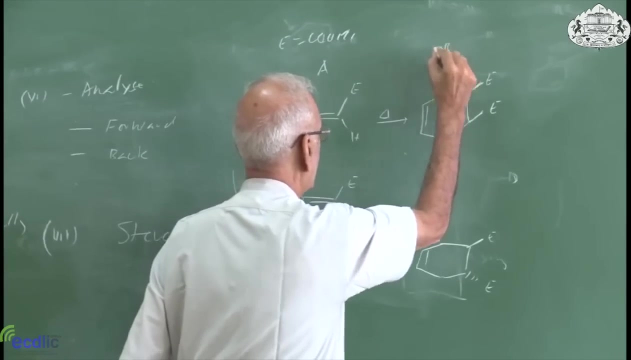 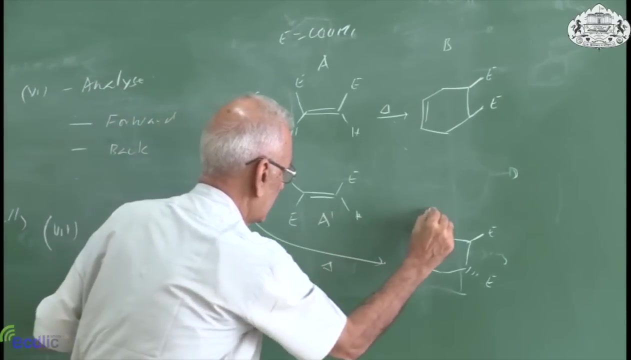 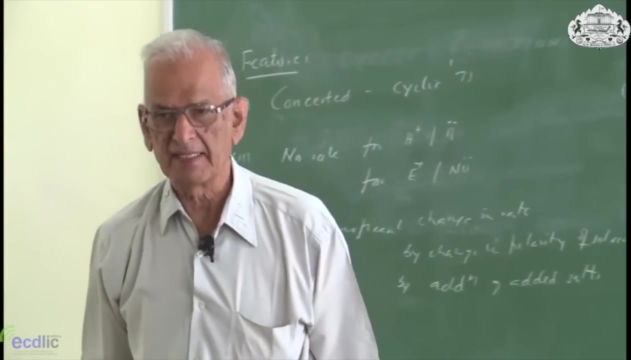 both ester groups are cis, The product will now have both ester groups cis. Starting material A gives me product B. Starting material A- dashed- gives me product B- dashed. Two different isomers of starting material give me two different isomers of the product that is then called. 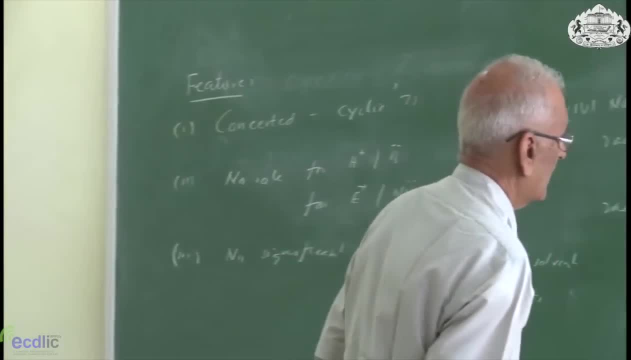 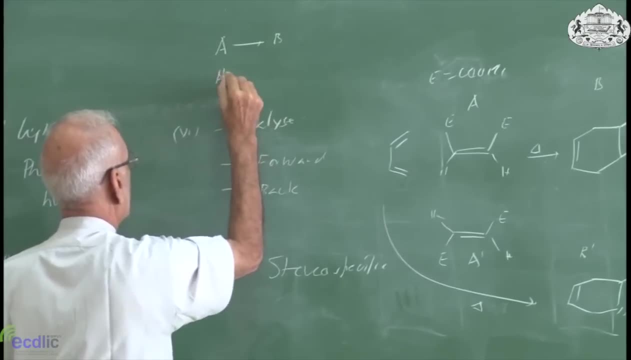 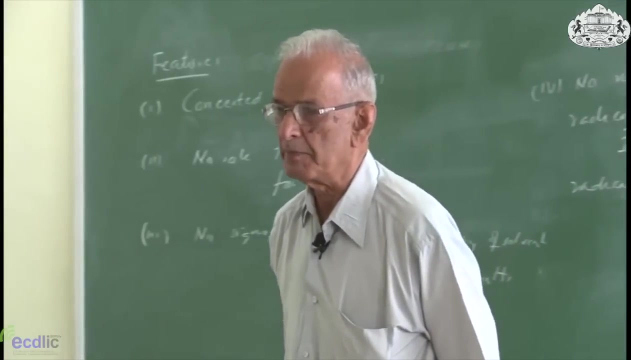 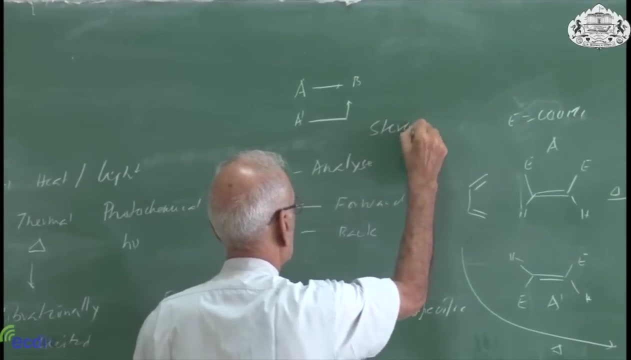 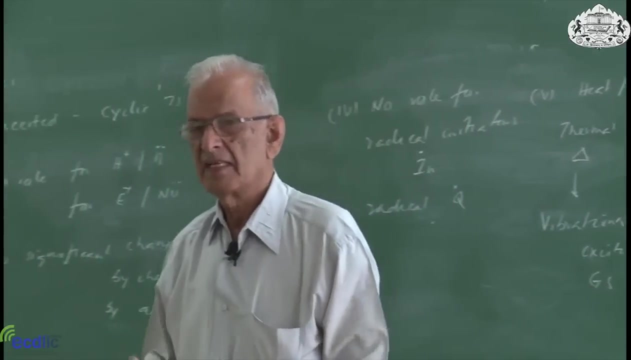 as a stereospecifically. If I have a reaction like this: A gives me B, A dashed, also gives me B, even though there is another isomer B dashed, then we call this reaction as stereoselective. So in a stereospecific reaction isomer A must give you product B, isomer A dashed must. 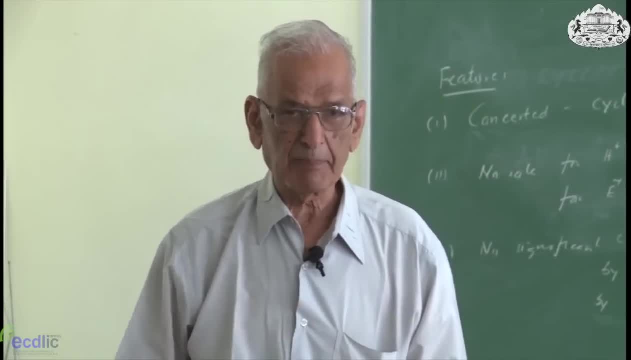 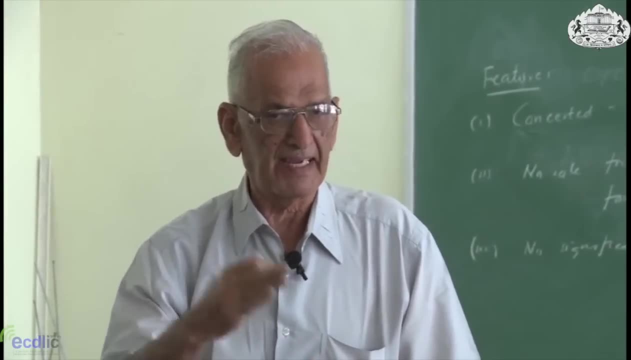 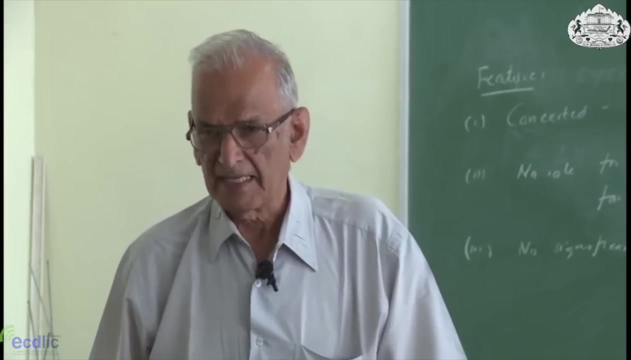 give you different product: B dashed, If it is 100 percent, we say it is 100 percent B, then stereospecific. If first reaction gives you 90 percent A, 10 percent B, second reaction gives you 90 percent B, B dashed, 10 percent B, then we say it is 90 percent stereospecific. 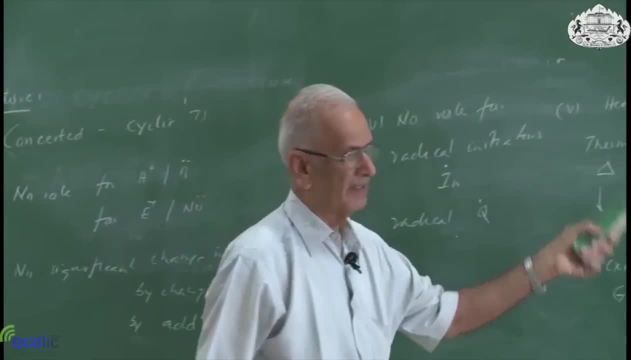 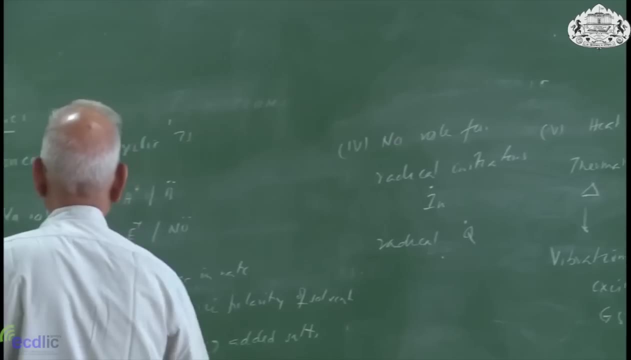 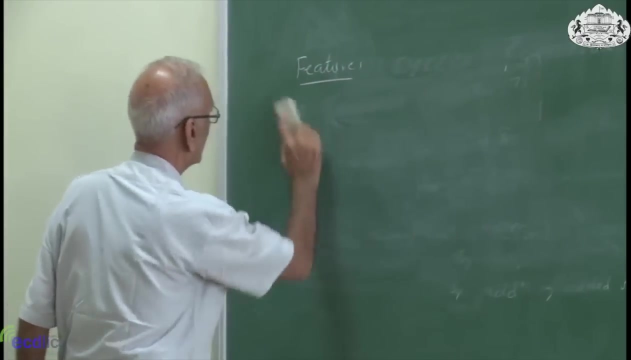 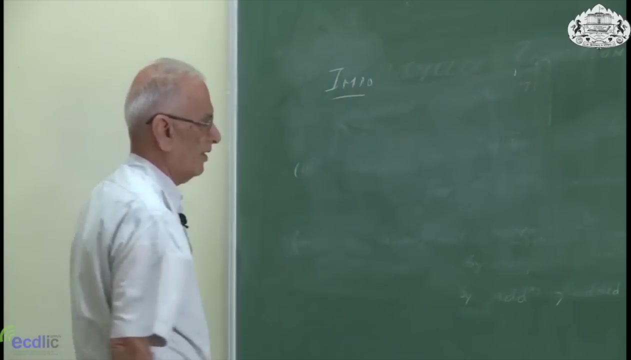 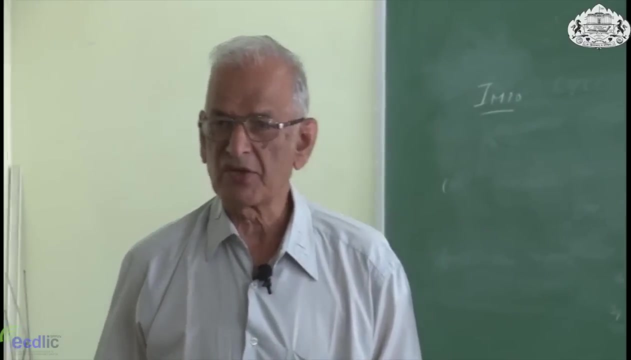 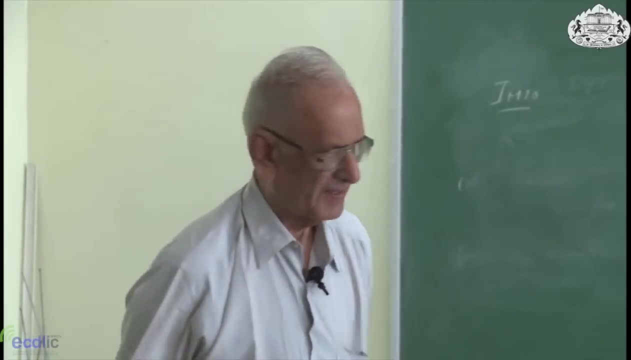 So we have listed the features of a pericyclic reaction. Thank you. Why are pericyclic reactions important? What is the importance of a pericyclic reaction? After all, organic chemistry is the chemistry of carbon-carbon bond formation. So in all of this, we are having carbon-carbon bond formation. 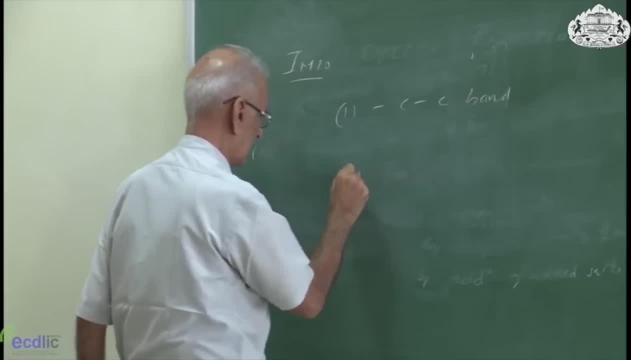 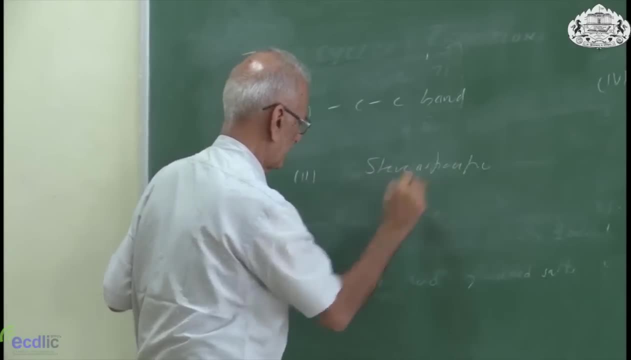 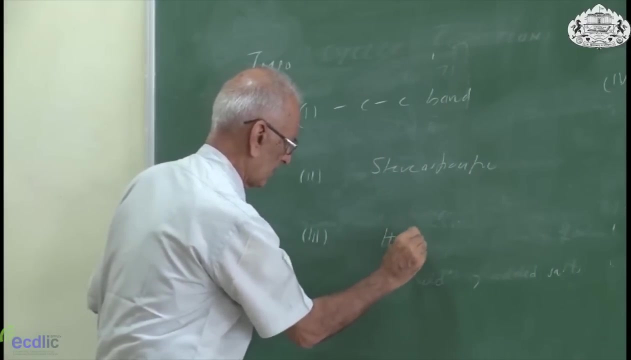 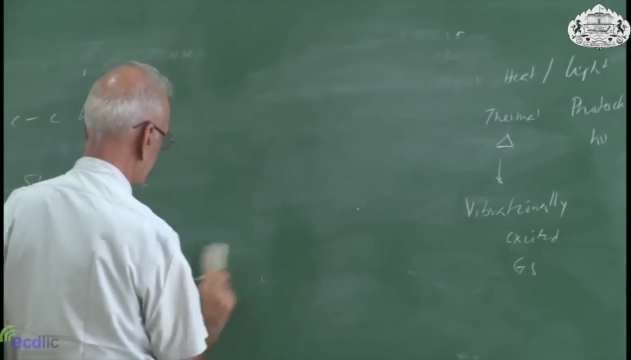 Number 2- reaction is stereospecific. number 3- reaction takes place in high heat. Why does the reaction take place in high heat? If I am looking at an ionic reaction, if today we have met a agua ionizing reaction, you can say two aging reactions we call regime 1-. 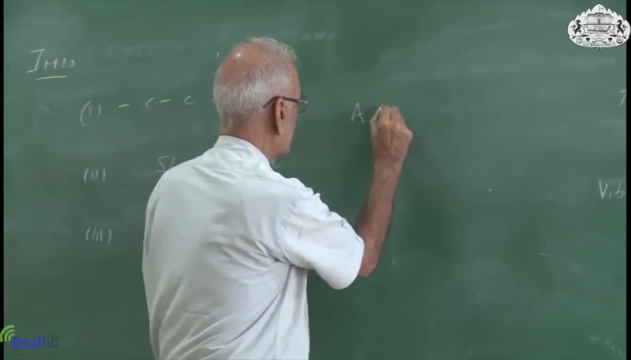 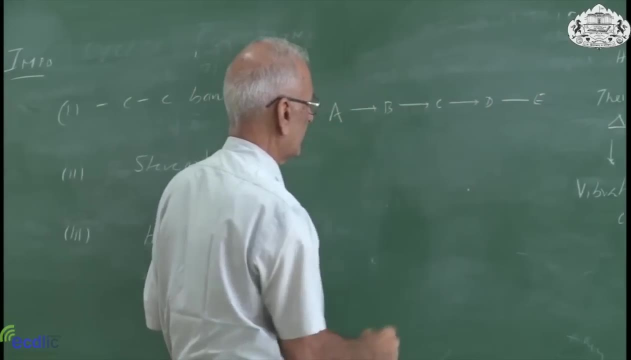 position, reaction: we are simply looking different reaction cause and AL 1, reaction 2 and so on, for reasons of four domestic: A gives me B, B goes to C, C goes to D, D goes to E, Then B will give me some intermediate. 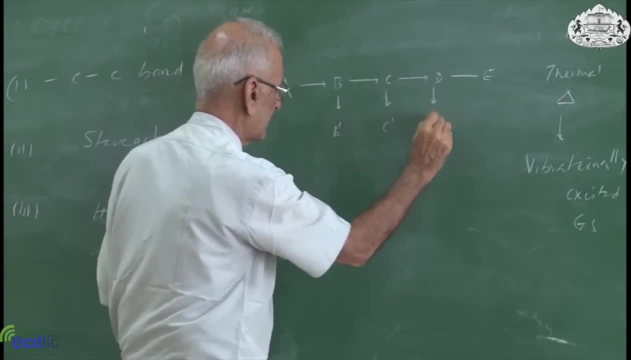 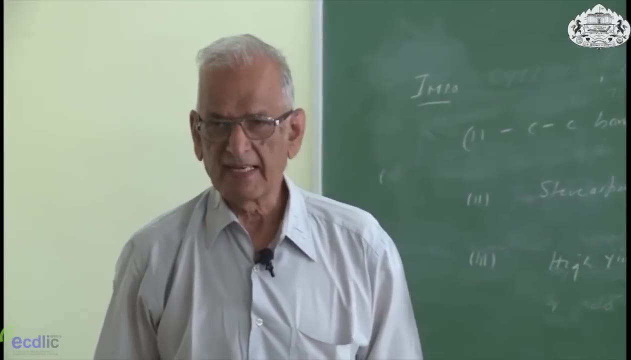 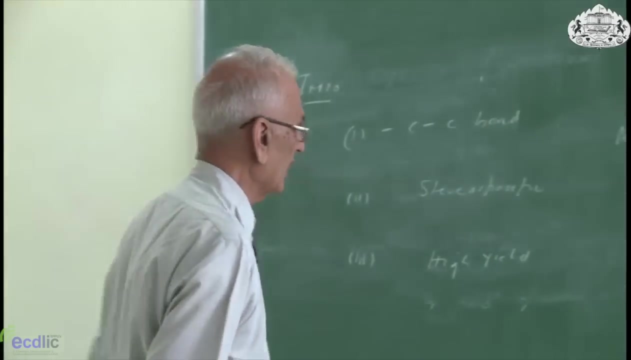 some impurity of B dash, C will give me impurity of C dash, D will give me impurity of D dash. So, besides E, I will get B dash, C, dash, D dash. therefore you will have low yield. 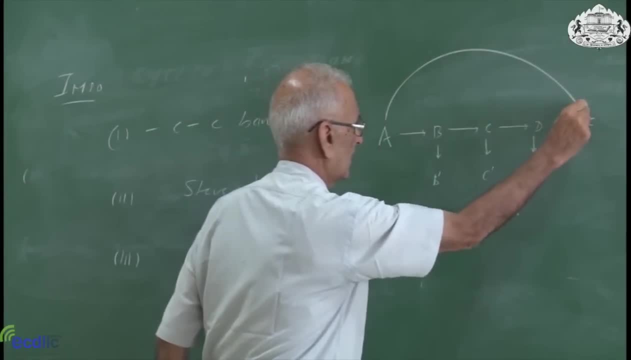 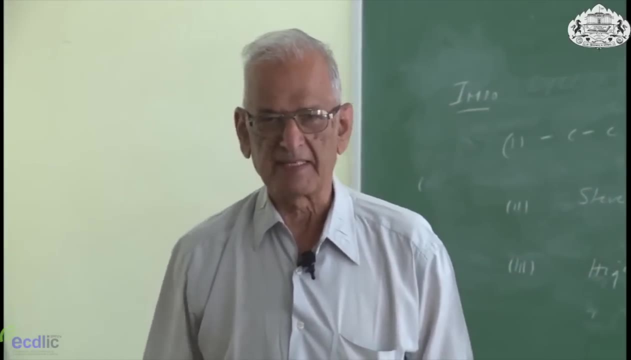 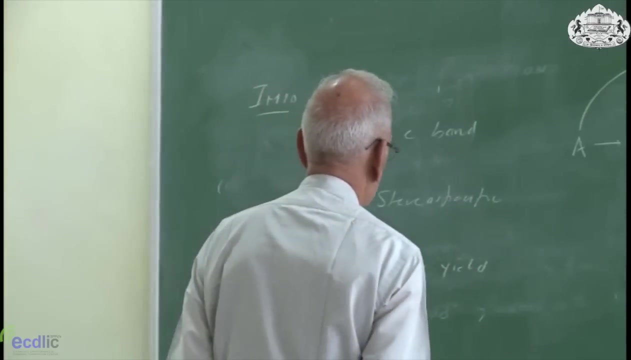 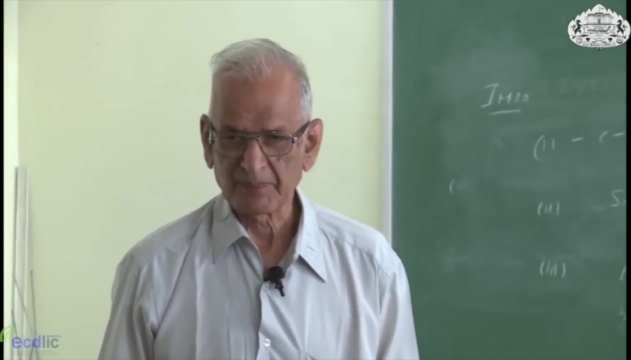 but in a pericyclic reaction no intermediates are involved. you directly go from A to E, no intermediate either. there will be A and E, but nothing else. you send a small child from Pune to Delhi, then what is your problem? You tell the child. 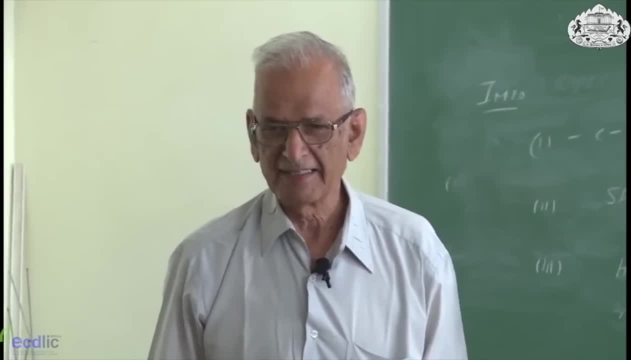 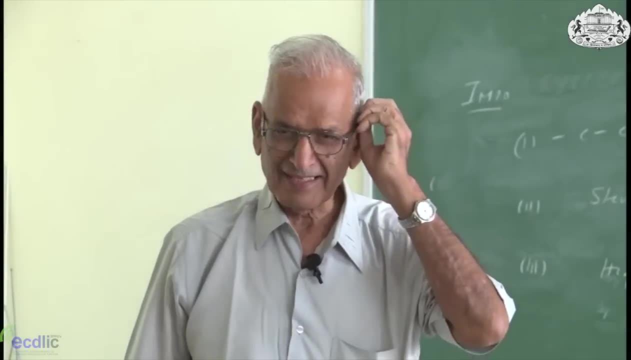 it will take long time. this thing, that thing do not get down anywhere. but child does not have understanding of what is long time. After two hours he thinks it is a very long time and station will come and he will get down and then of course parents will be in great. 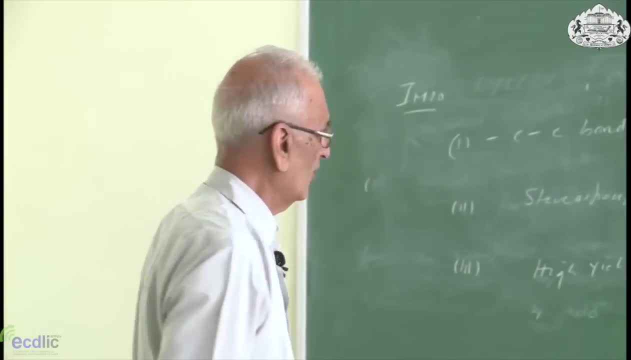 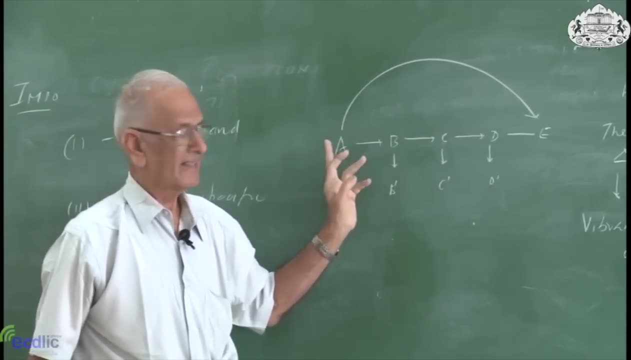 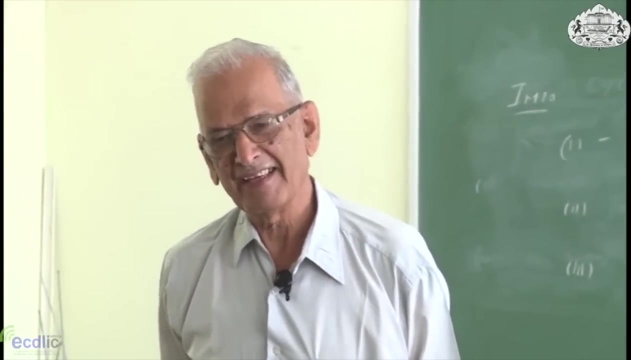 difficulty. He can get down at any station. So what do wise parents do? Send him only by air, He can go up, get down. get up in Pune, he can get down, only in Delhi. So no problem, You put him in the aeroplane at A, somebody picks him up at Delhi, no chance. 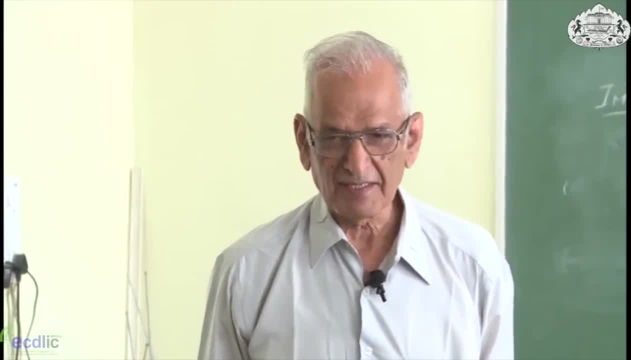 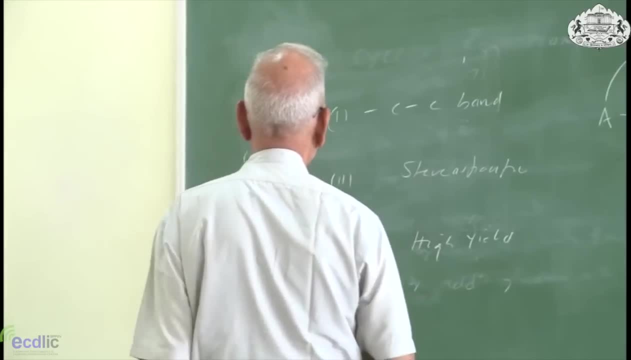 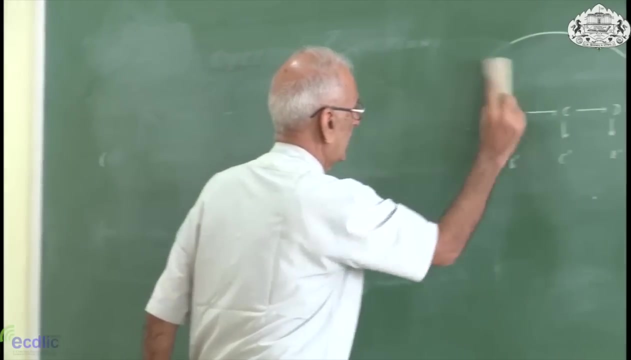 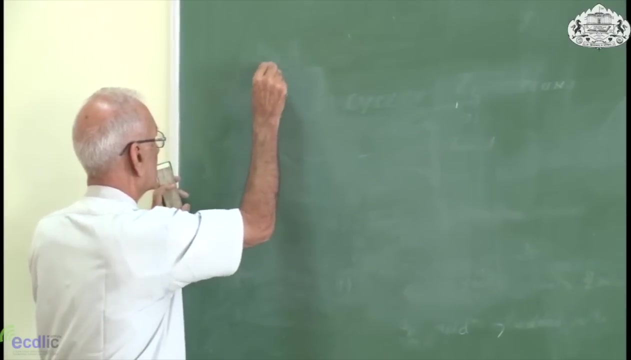 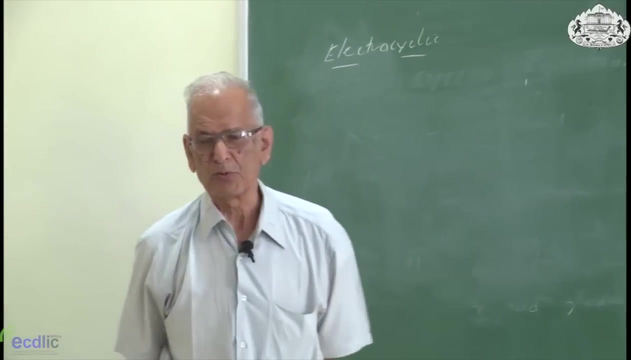 of making a mistake. So high yield because there is no intermediate In ionic and radical there are several intermediate. Now we are going to look at our first class of pericyclic reaction and that is your electrocyclic reaction. 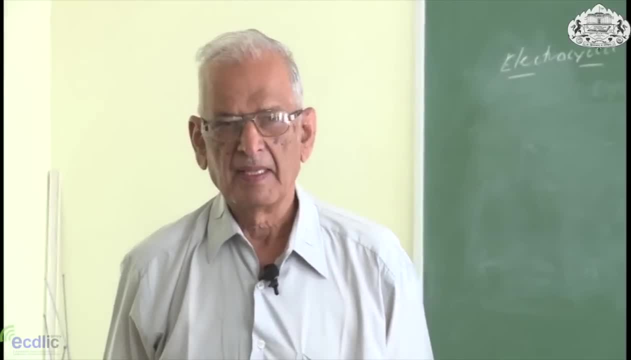 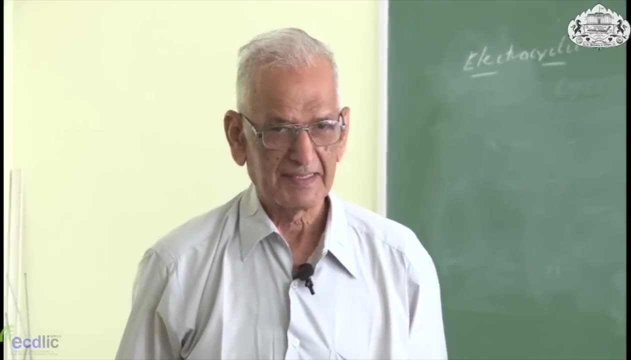 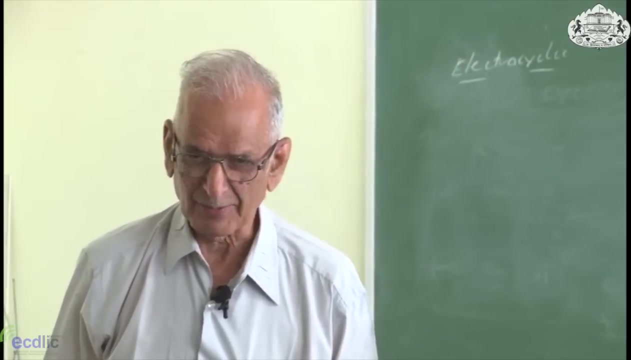 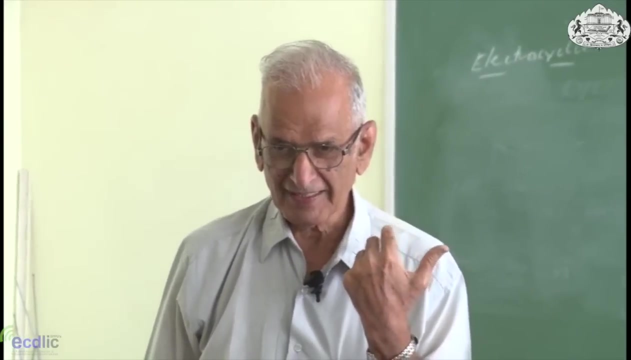 Ok, Now I am going to emphasize two rules. Number one is: class should not have me talking and you listening, or you sleeping, also All right. What I want is you should ask. So if you have a doubt, do not keep your mouth closed, immediately ask. 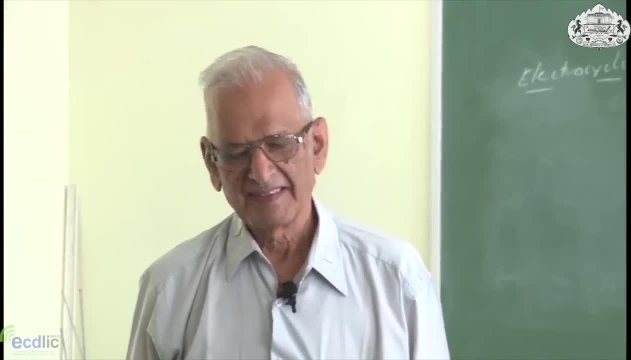 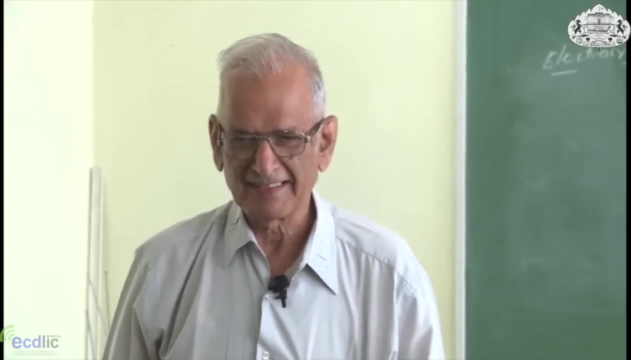 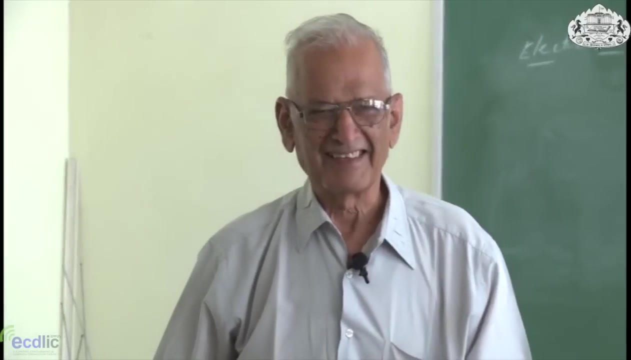 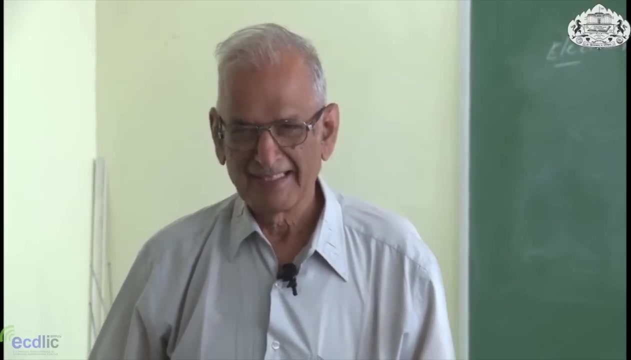 Ok, I know that when I was a student, I also did not ask, But now the days are different and it is time you asked. In spite of this, I know you are not going to ask, So what is the alternative? I am going to ask lots of things and my request is you try to answer. 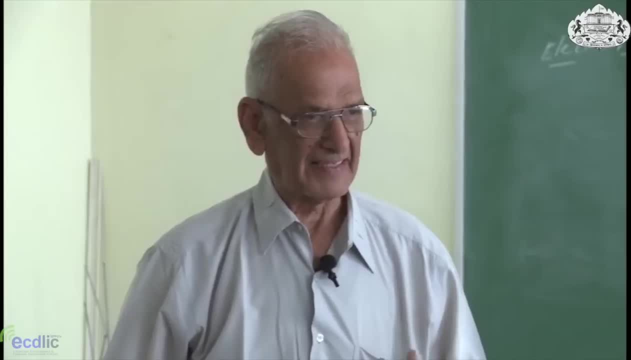 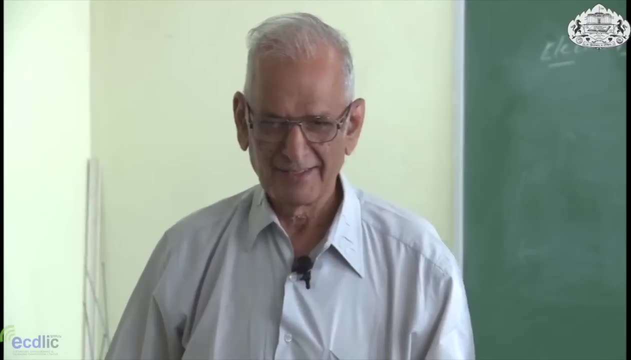 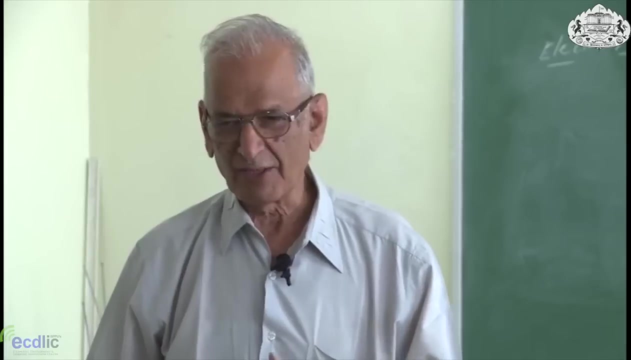 Does not matter if it is right or wrong. Ok, In fact, wrong answer teaches you many more things than the right answer. So I am going to ask you lot of questions and I want you to try- Do not be afraid- What is our usual. 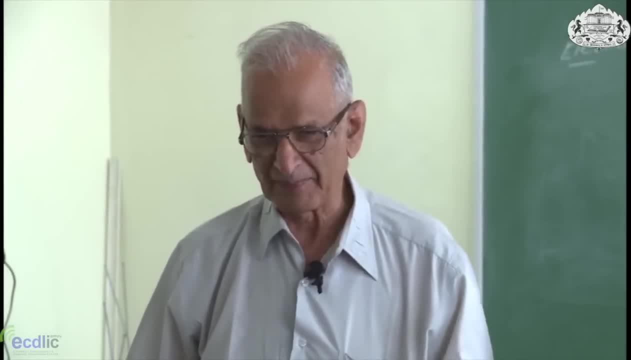 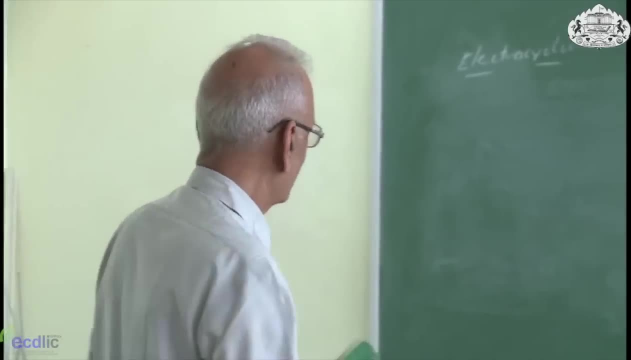 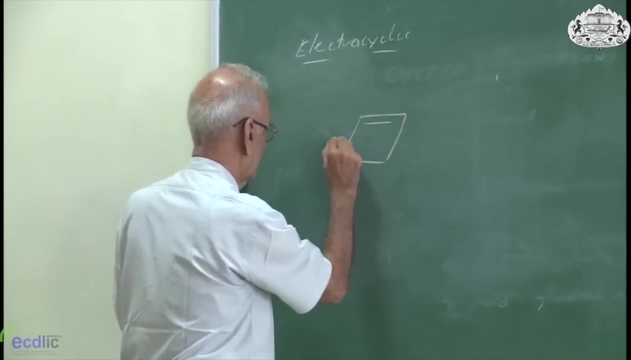 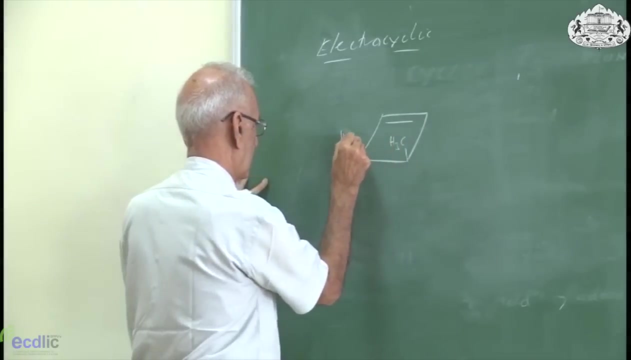 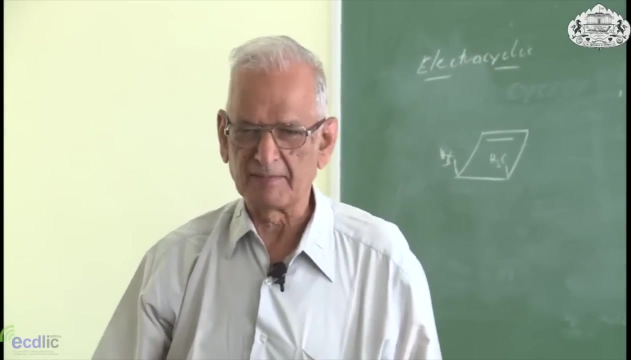 fear, If I do not answer, all my friends will think that I do not know anything. Forget it, Your friends also do not know many things, So there should be no barrier in this. All right, Well, let us start with our first question: What is the systematic name for this component? 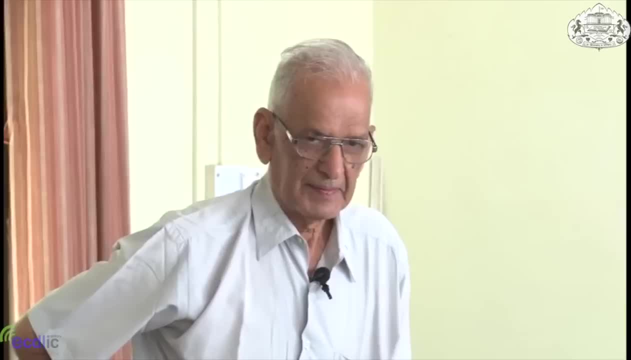 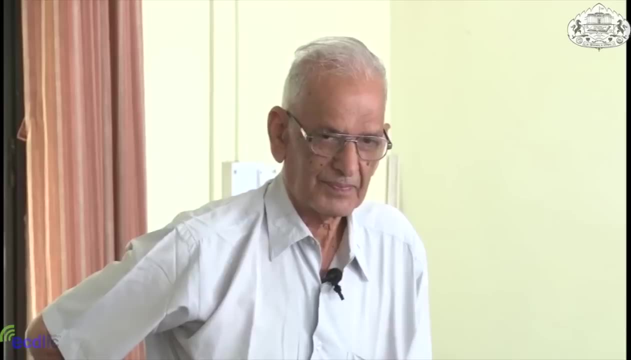 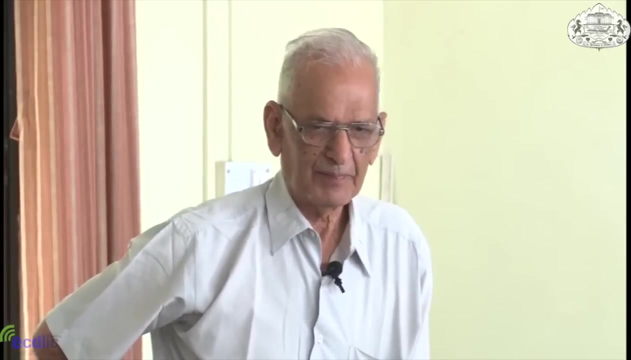 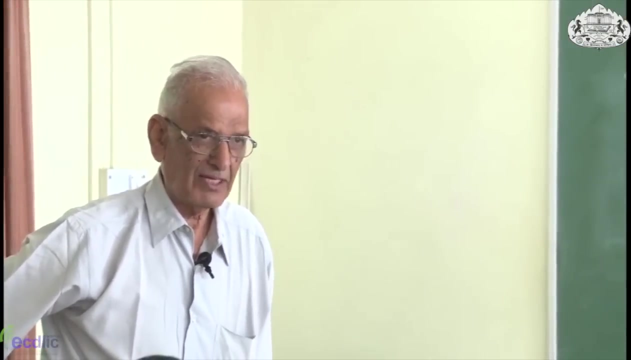 1. 1. 1. 1. 1.. What is the first thing you will see? Ring is four membered, so cyclo butane. then there is a double bond, so cyclo butane. Then what is next step? It has two metals, so you must give the position of the metals. So that is the question: from where should I start the numbering? 3, 4 dimethyl. 3, 4 dimethyl cyclo butane- why 3, 4?? Double bond must have smallest number. so 3, 4 dimethyl cyclo butane. Is that enough, or I must add something else: cis. So we are looking at cis: 3, 4 dimethyl cyclo butane. What are we going to do? 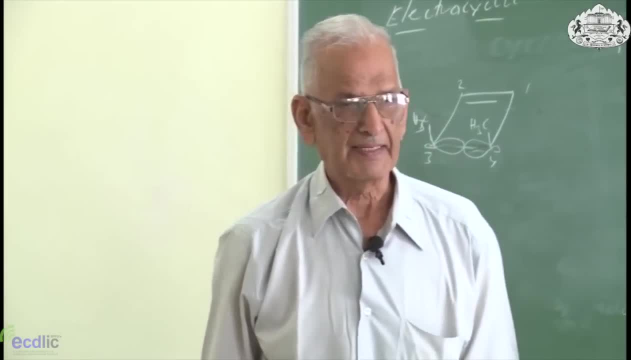 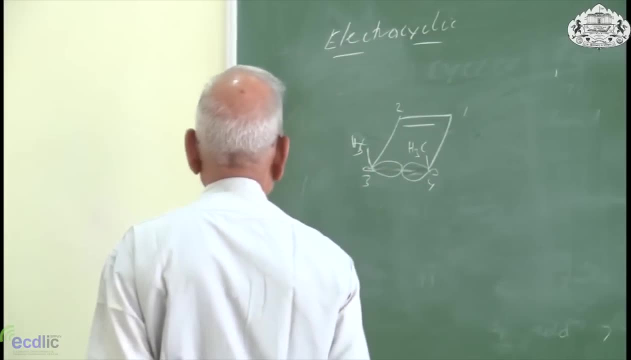 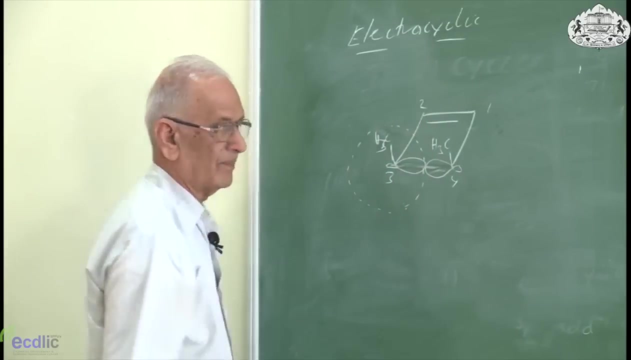 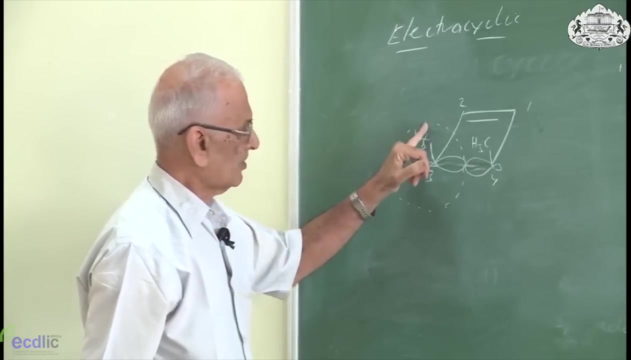 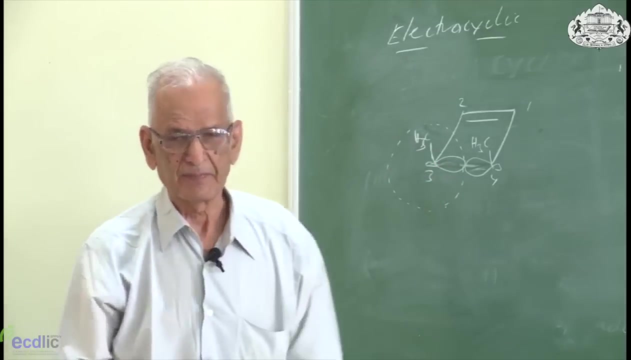 We are going to break this sigma bond and convert this cyclo butane into butadiene. So you imagine that this is a watch. Okay, All right. What is this position? the watch 12, position 3, position 6, position 9, position everything. 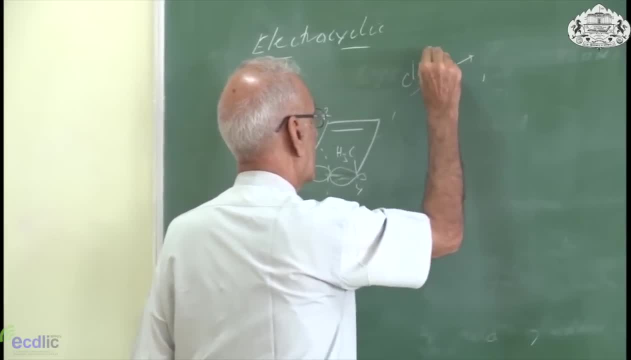 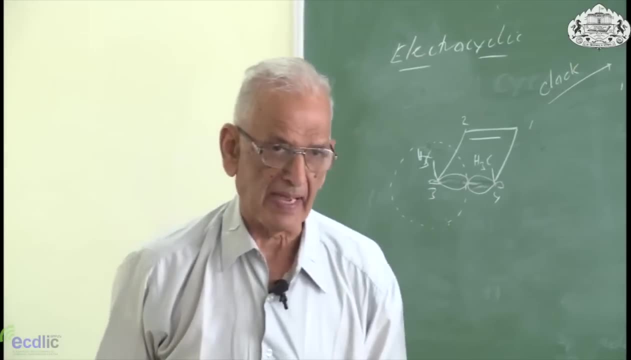 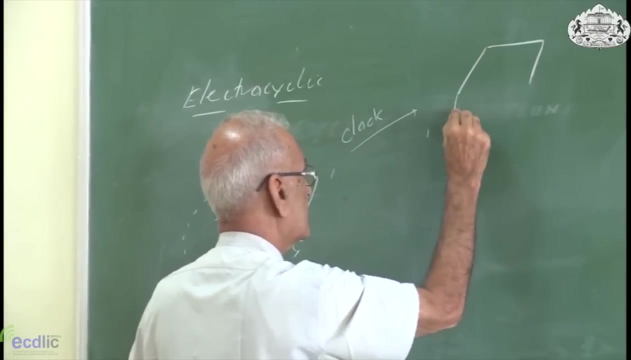 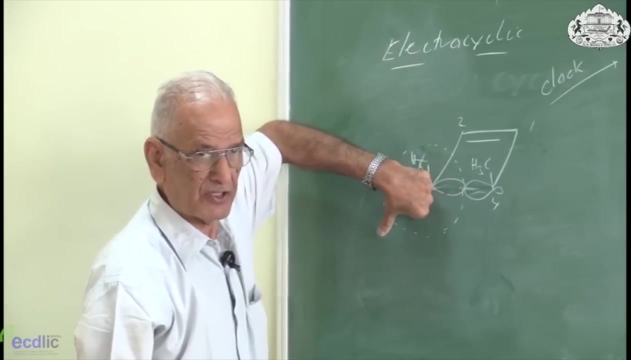 So we are going to open this orbital in a clockwise manner. So I am going to take this orbital from 3 position to 6 position. When I take this orbital from 3 position to 6 position, what will happen to this methyl group? where will it go? 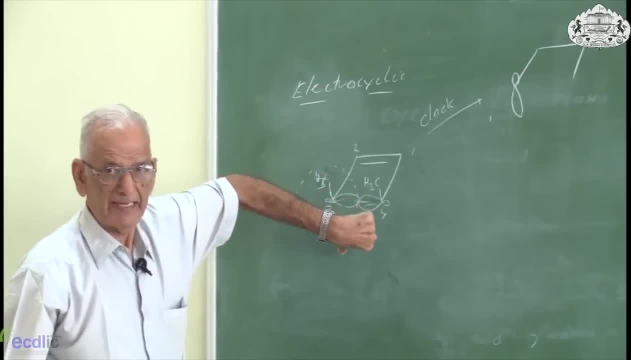 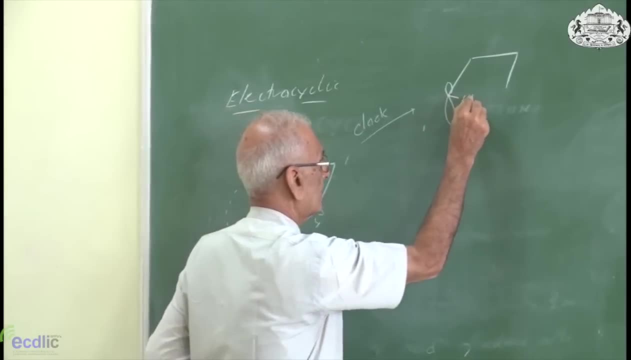 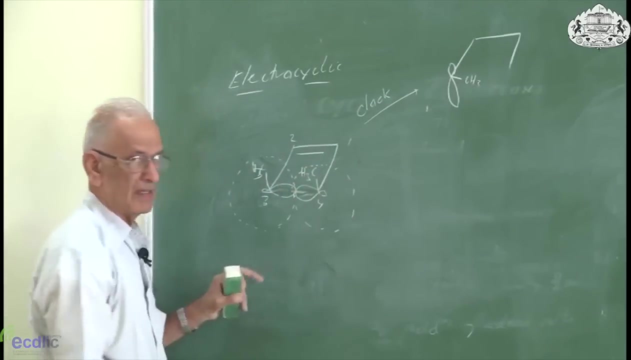 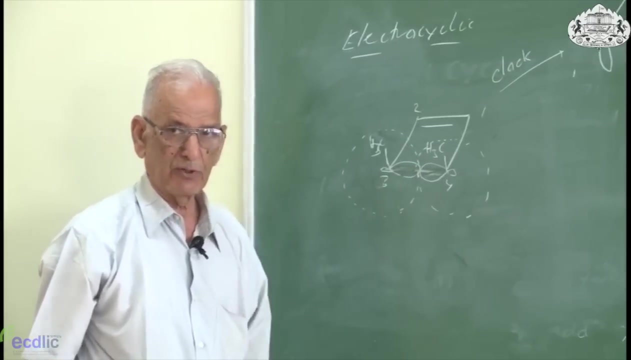 It will go inside. Metal group will come inside. Now you look at this. watch, Where is this orbital? This orbital is here. I have taken this. It is here. orbital is at the 9 position. We are going to take it to 12 position When I take this. 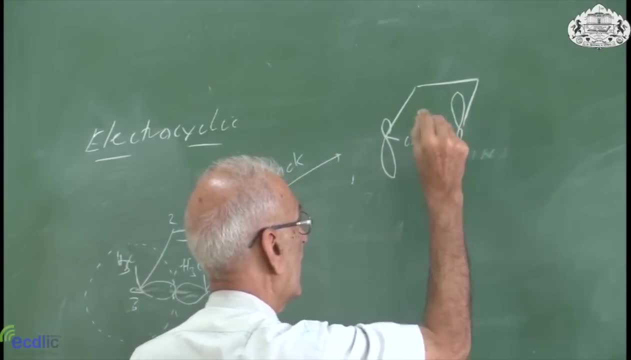 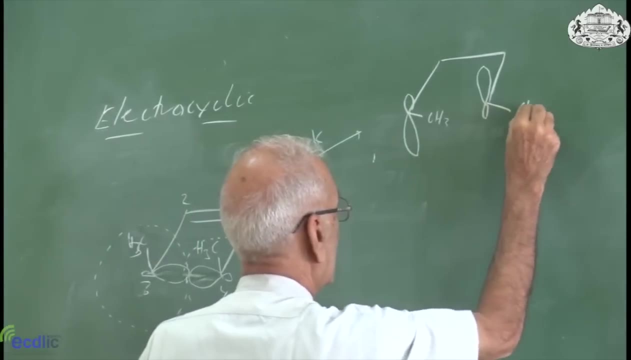 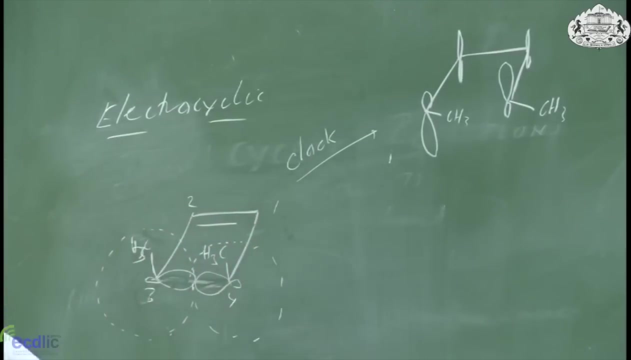 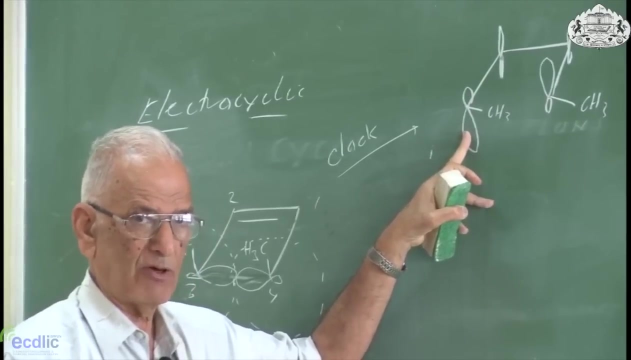 orbital to 12 position. where will the methyl group go Outside? Now, what is this? This is your p orbitals of the double bond. Now what we want to do, What type of orbital is this? sp 3 orbital? We are going to convert this sp 3 orbital into p orbital. 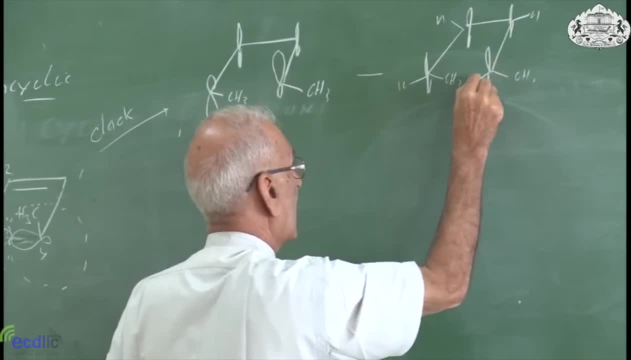 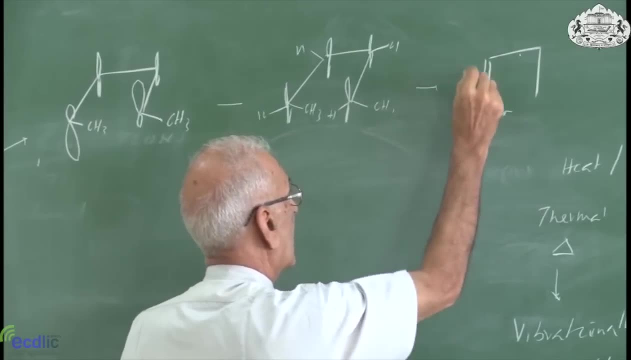 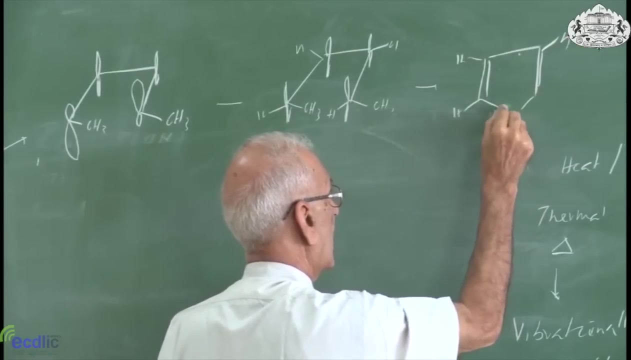 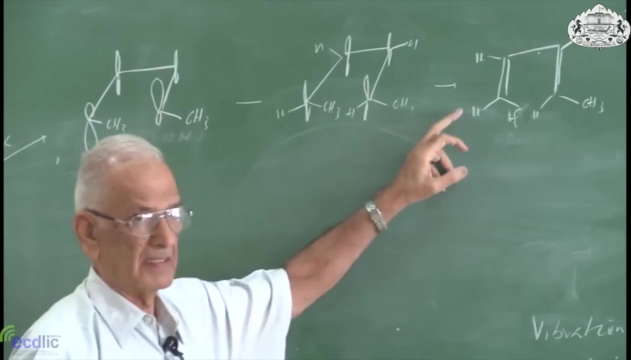 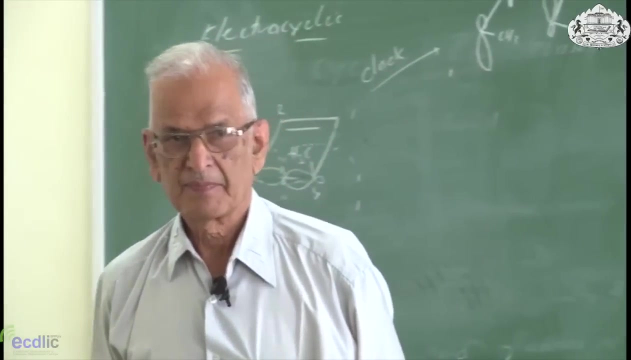 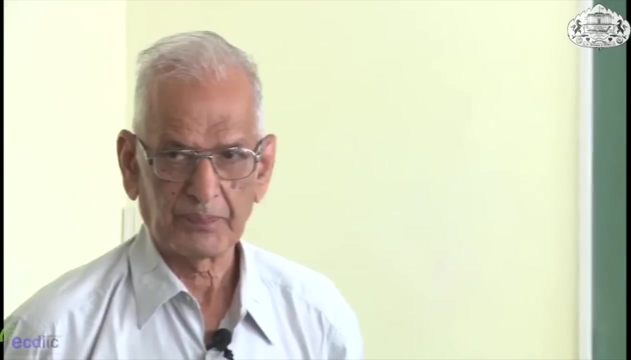 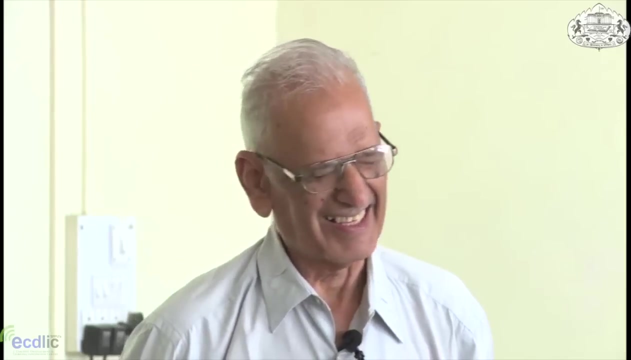 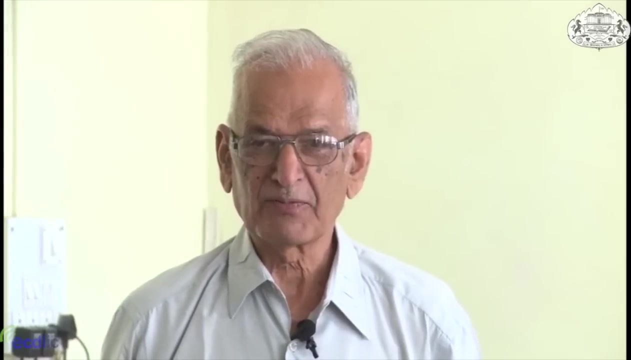 And therefore that is your product. What do we see? This double bond is cis, this double bond is sp. Now, what is this trans? Give a systematic name to this compound. That is not a systematic name. When you make nomenclature, you must first decide which. 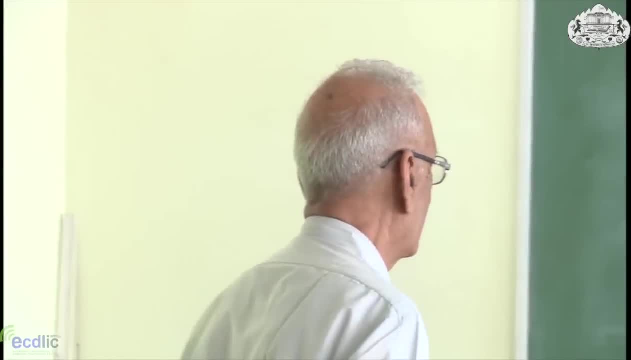 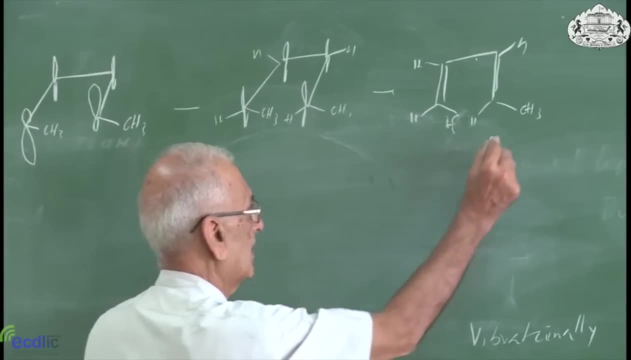 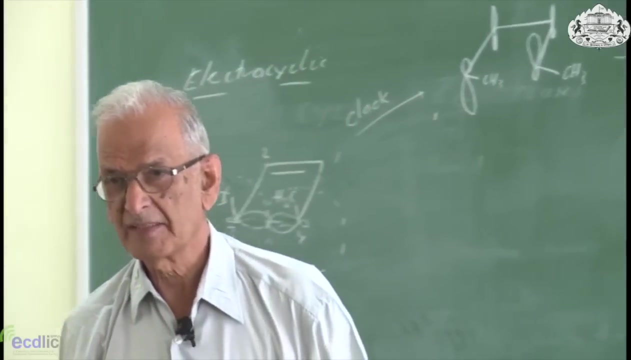 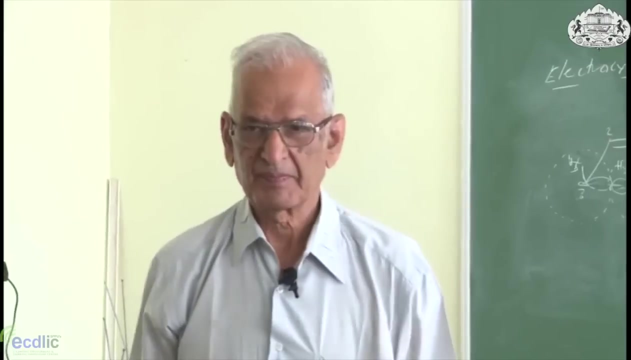 is the longest carbon chain. Okay, Okay, So you should start from either this metal or that metal. So what is the product? 2, 4 hexadeye. but you want to make it complete: Trans 2 cis, 4 hexadeye. 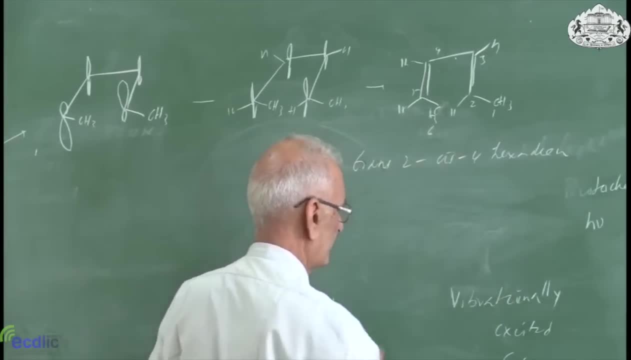 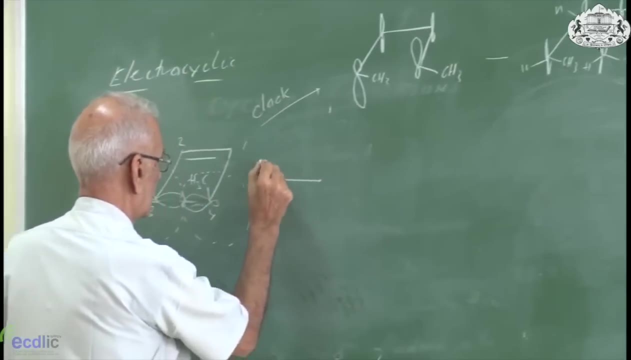 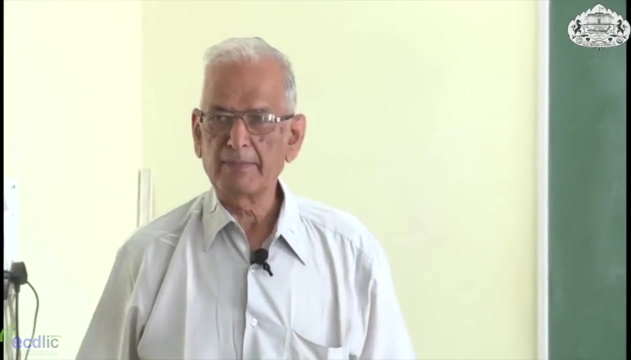 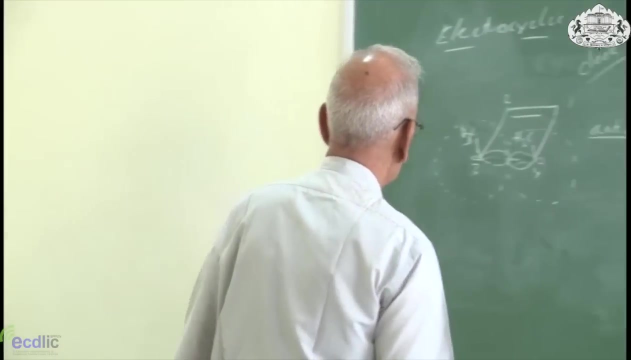 Okay, Now, in my next operation, I am going to move these orbitals in anti-clockwise manner. If I am going to move these orbital in anti-clockwise manner, where should this orbital move? This orbital must not be move. This is an antilockwise manner. Where should this orbital move? Where? 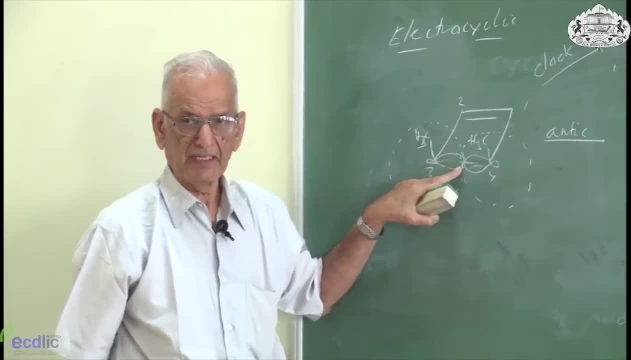 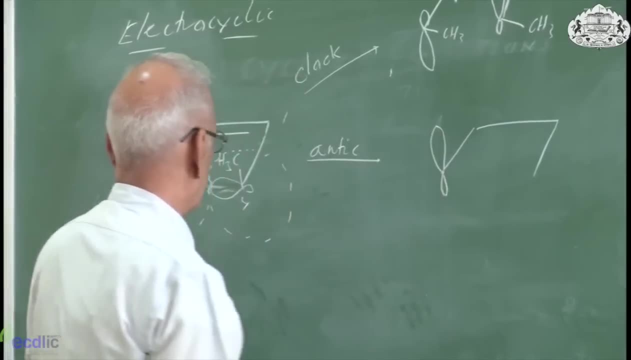 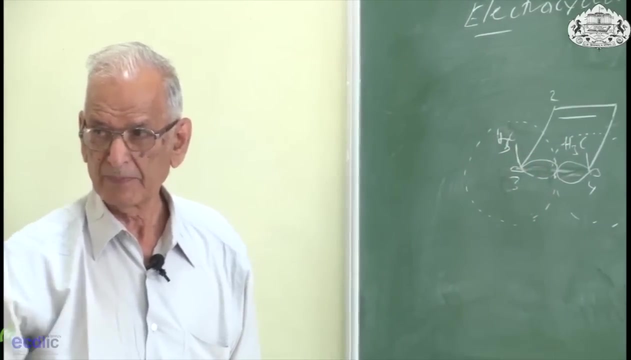 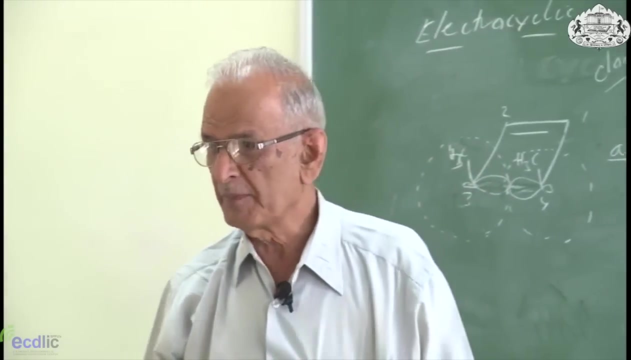 it will go From 3 position. it must go to 12 position. When it goes to 12 position, what will happen to the methyl group? Where will it go? Outside or inside? Outside, No, old people cannot hear properly, alright, and I am a very old person, So speak little bit. 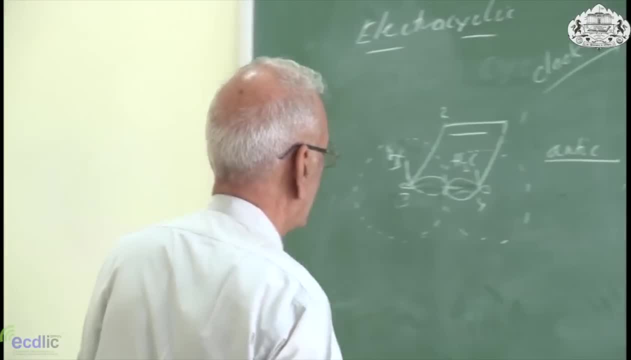 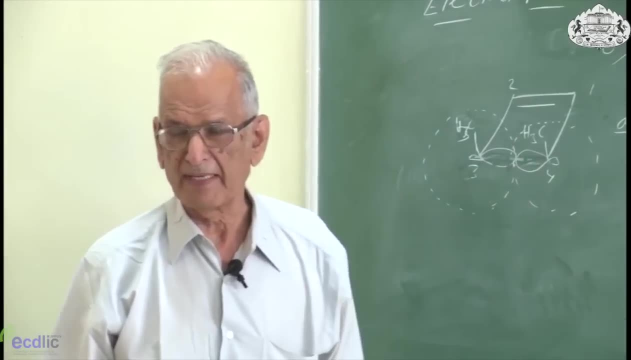 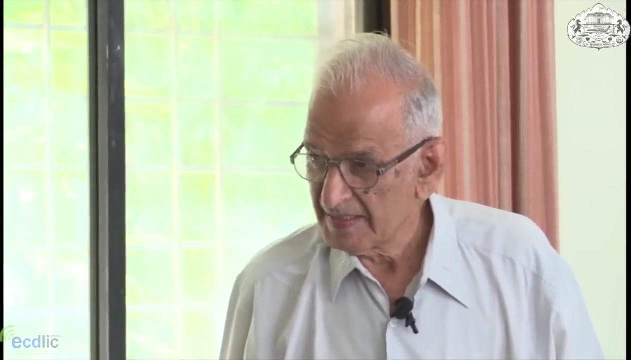 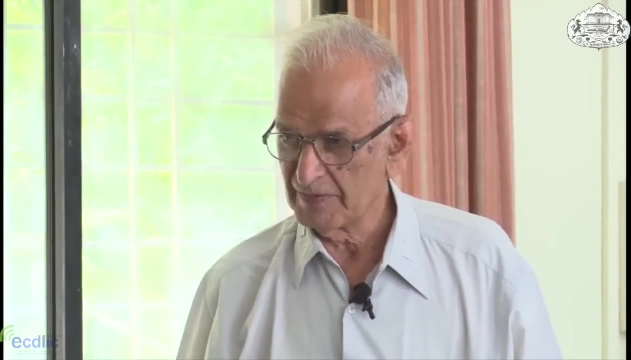 loudly. ok, Now this is also going to move in anti-clockwise manner. Yes, please, where will that orbital go? Where will the orbital go? Methyl group will go inside. Orbital should go from 9 position to 6 position. 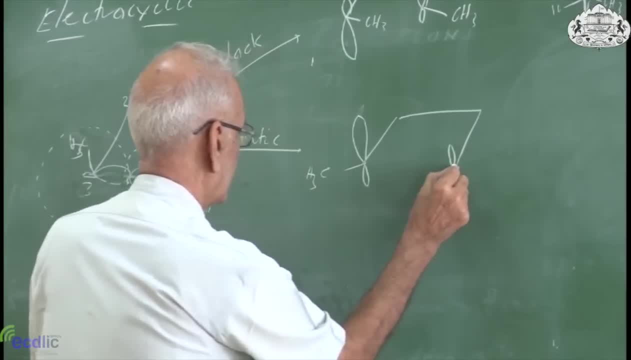 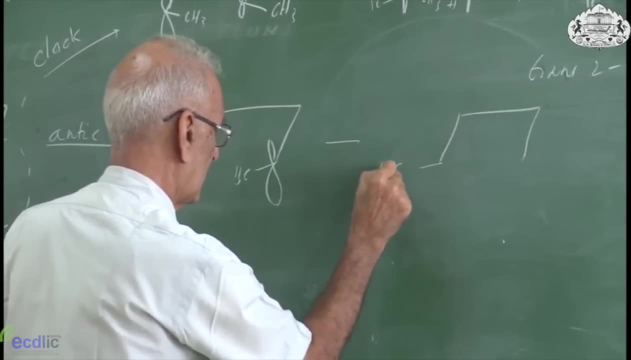 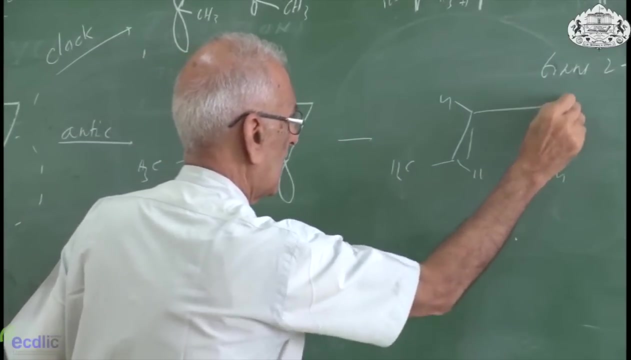 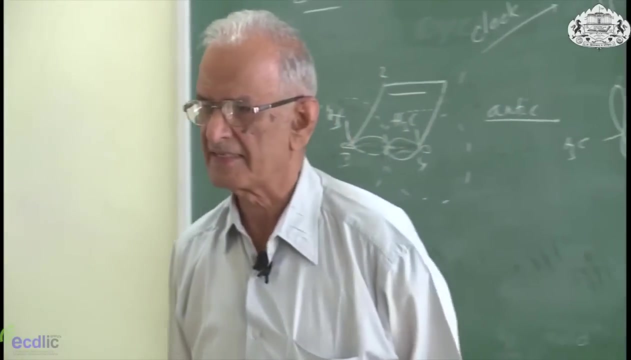 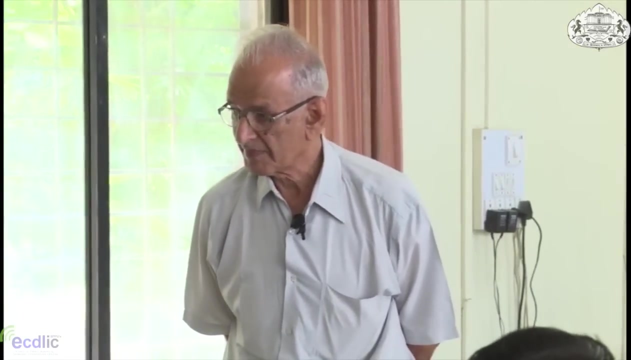 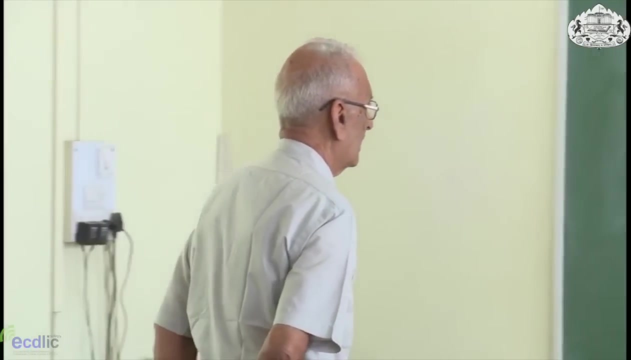 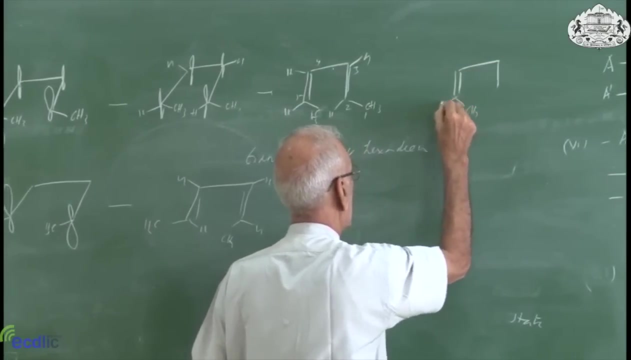 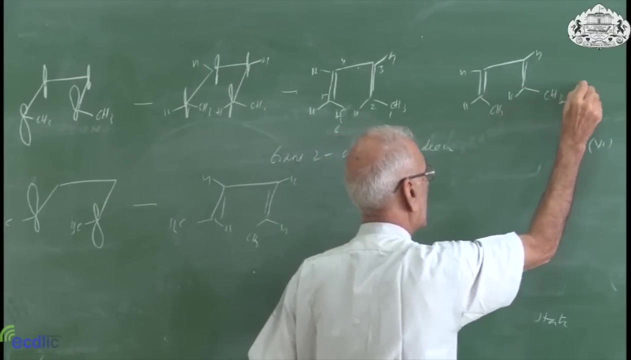 And methyl group will go inside. Therefore, after I complete the process now, this double bond is trans, that double bond is cis. Are the two compounds same or different? Same, Same. I start the numbering from this side. it will become the same. ok, In my starting. 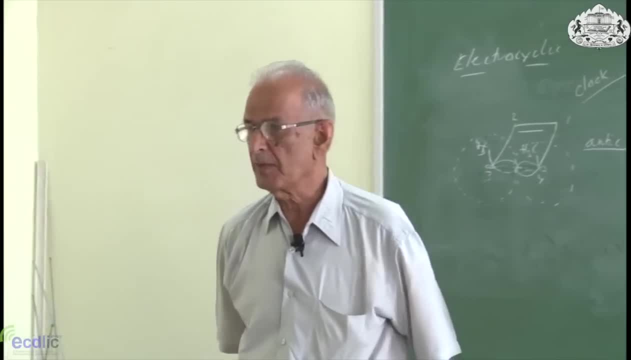 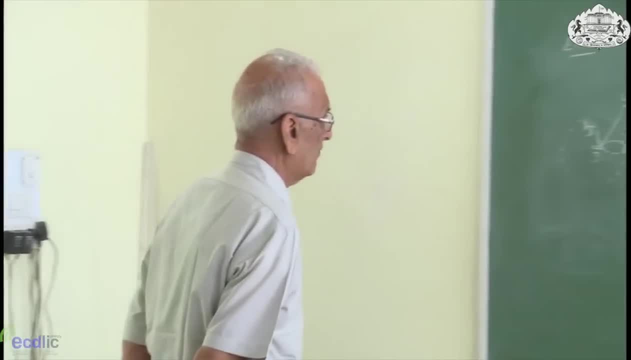 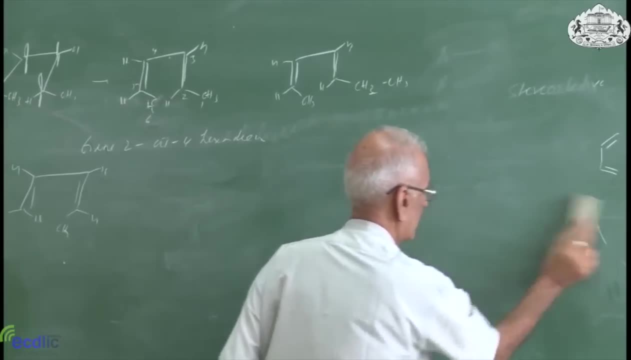 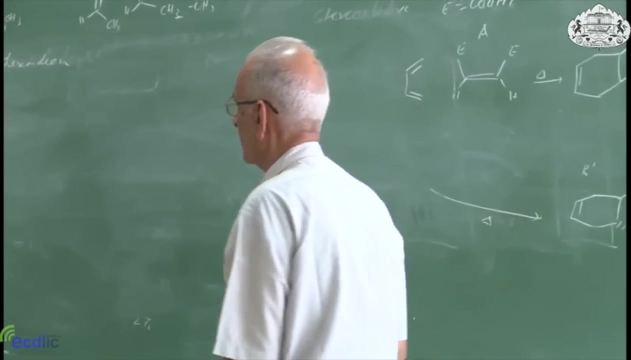 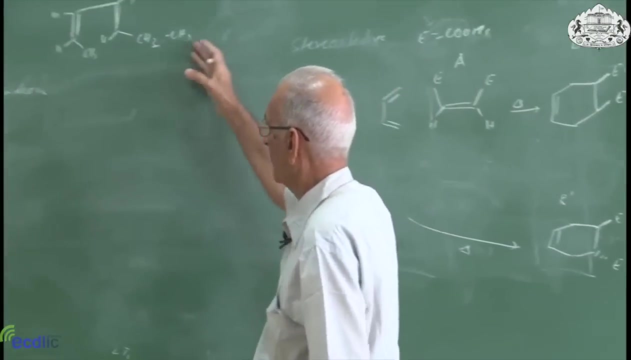 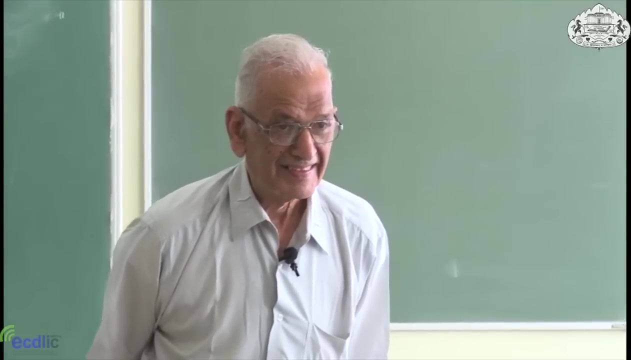 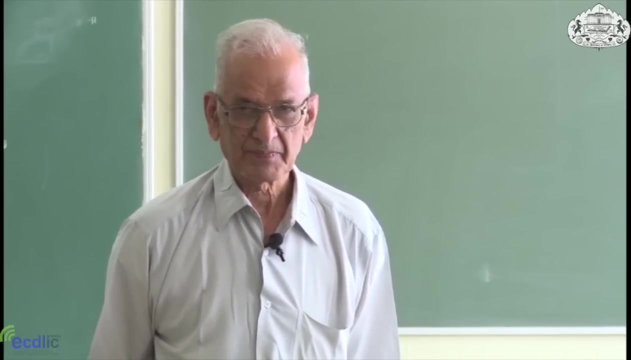 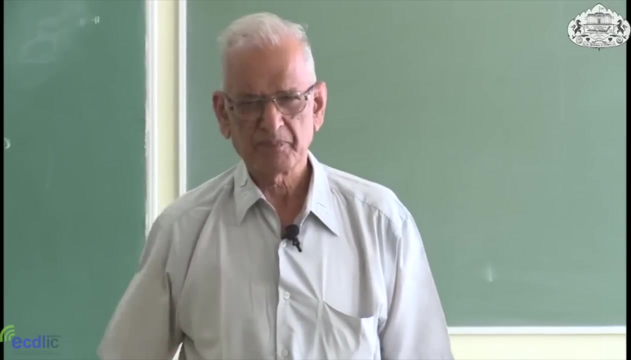 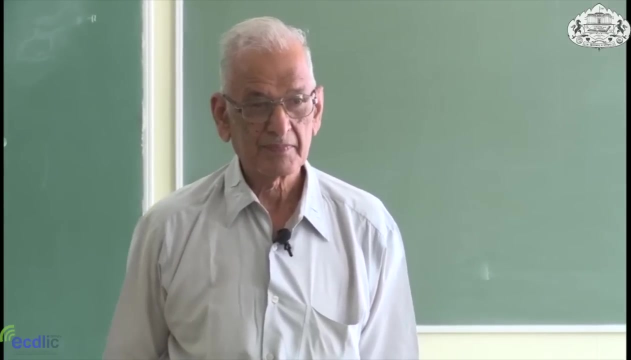 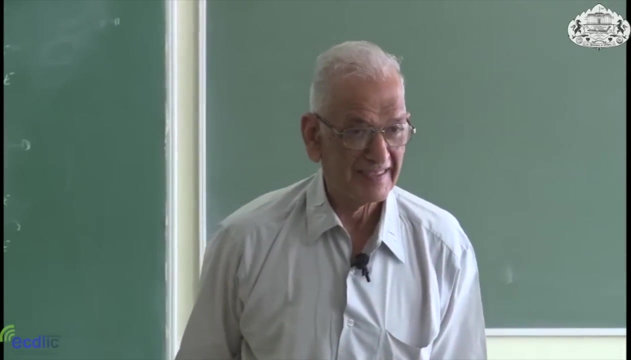 Yes, Yes, Yes, Now I have taken one methyl group and one methyl group. What is the systematic name you will give to this compound? Where should I start numbering? from here or from here? From here? Yes, From where should I start the numbering? will you start from methyl group or ethyl group? 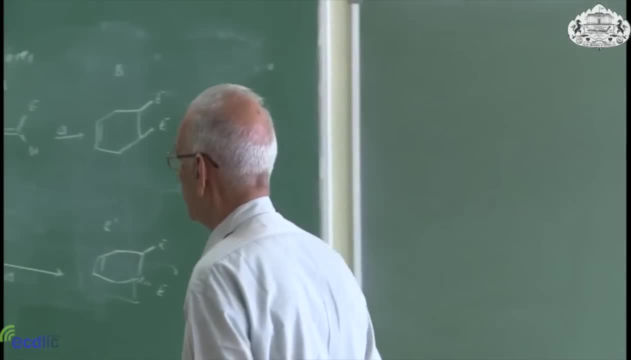 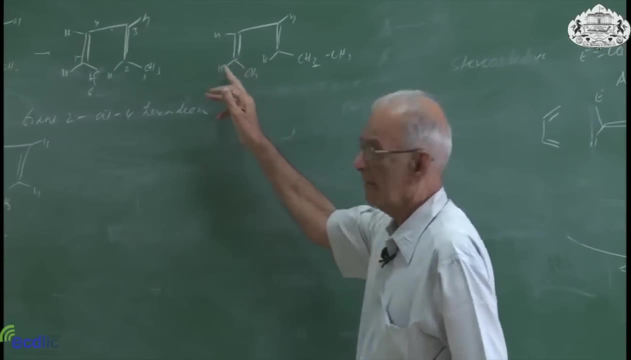 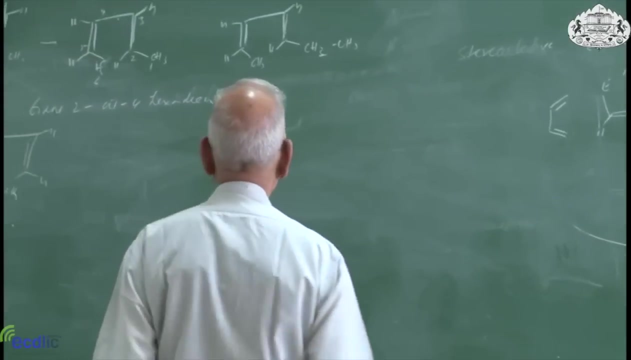 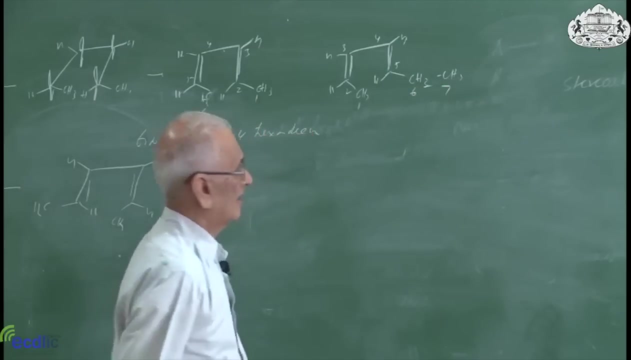 If I start from ethyl, what will happen? 1,, 2, 3: double bond is at 3 position. if I start from here, double bond is at 2 position. Therefore I must start the numbering from the methyl group. So now it is a 2,, 5 heptadi. 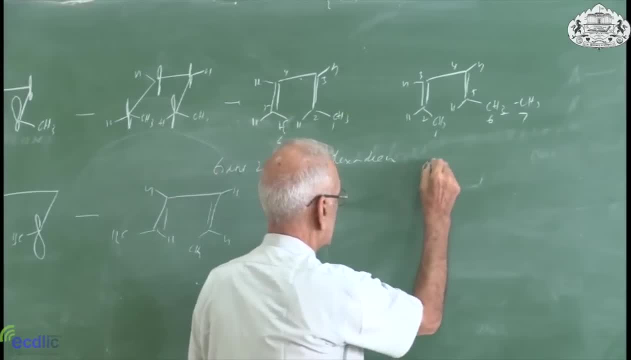 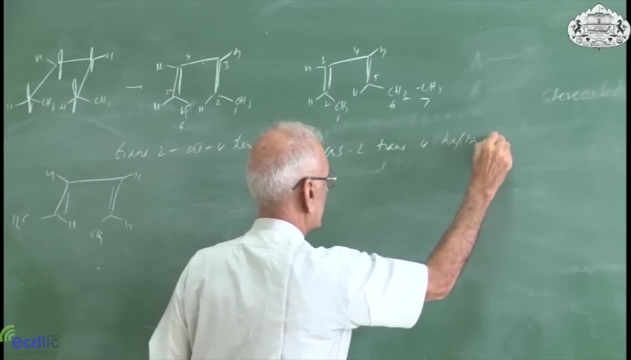 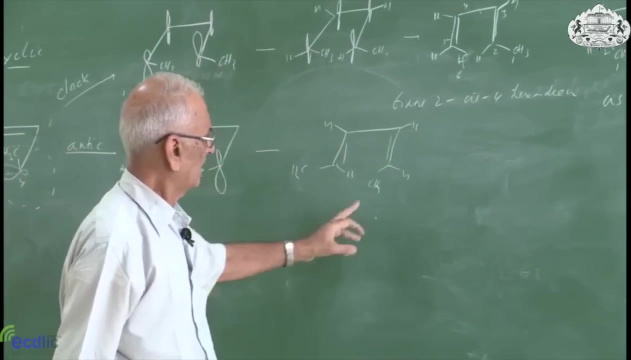 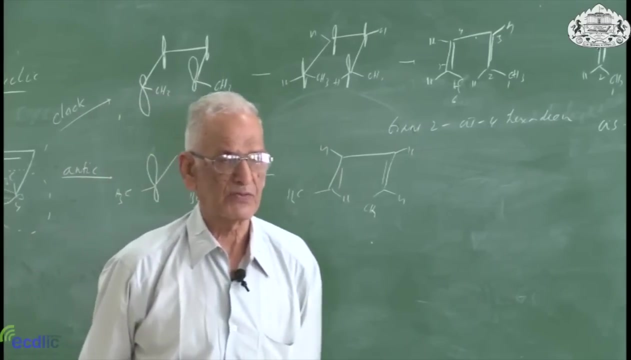 And now there is no ambiguity: cis 2 trans 4 heptadi In this process. now what will happen? Numbering will start from here, So that will be trans 2 cis 4 heptadi. So if the substituents 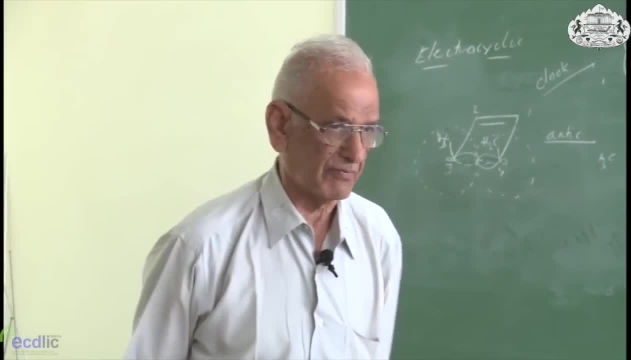 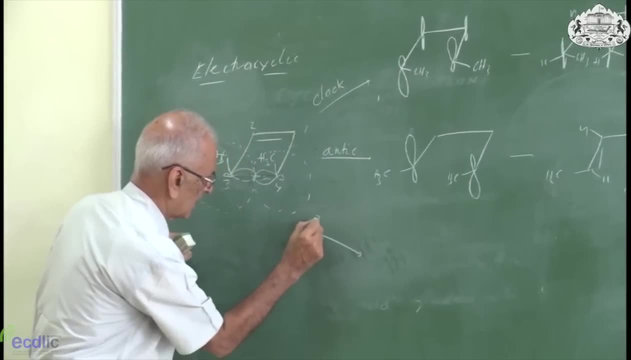 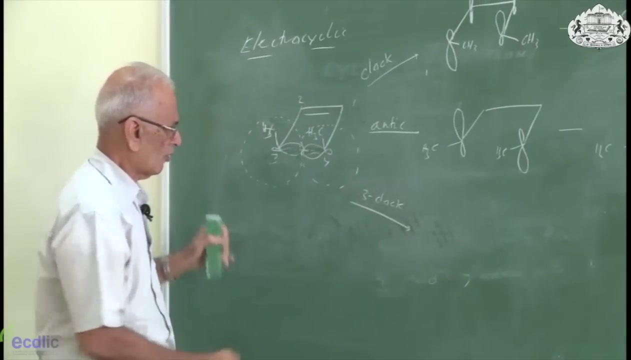 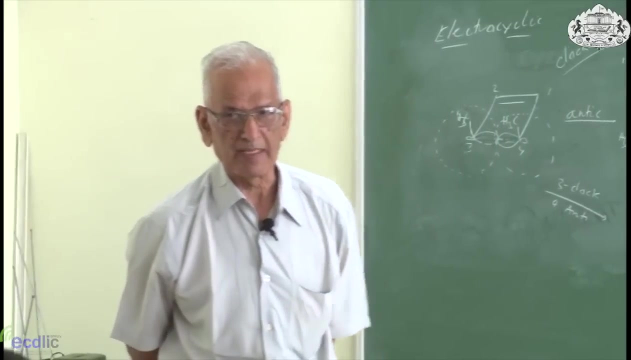 are different. So two processes will give me different products. Orbital number 3 is moving clockwise. Orbital number 4 is moving anticlockwise. Where will that orbital 3 go? It will go in the same direction. 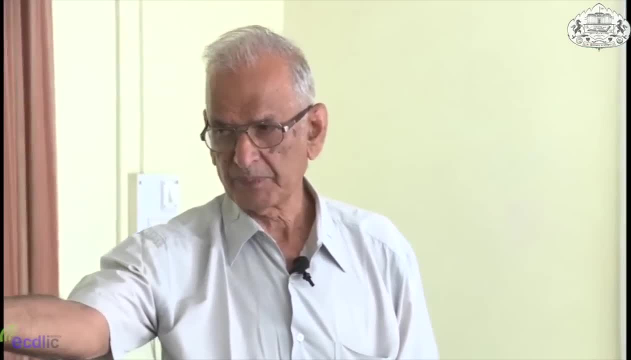 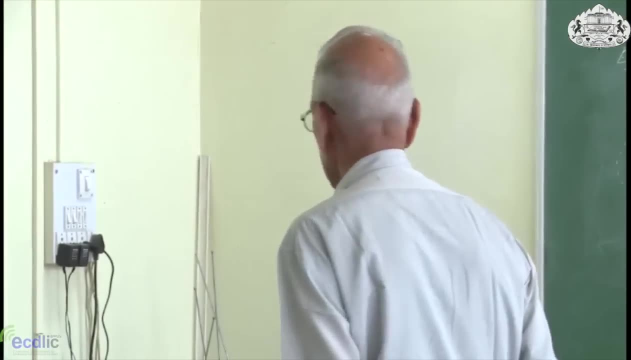 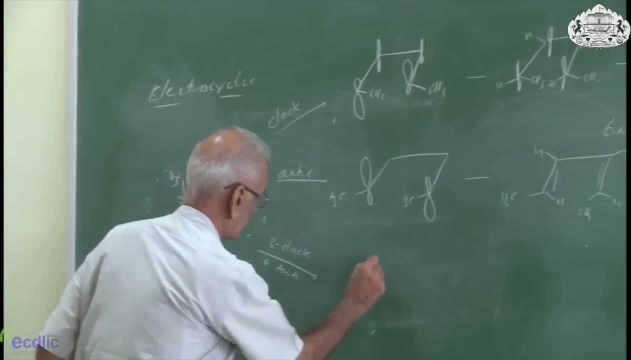 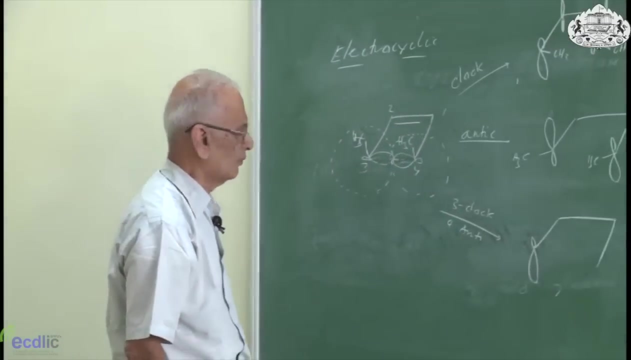 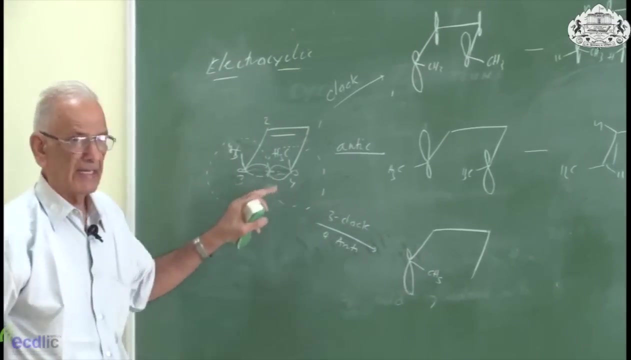 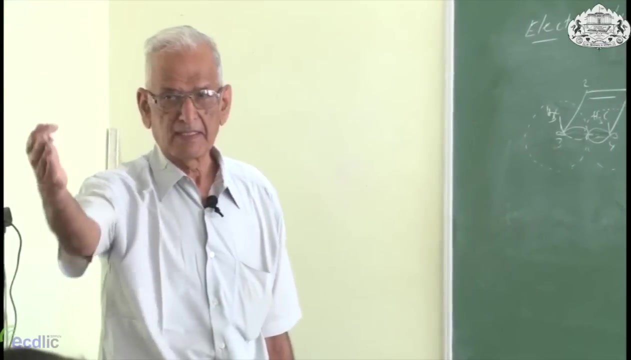 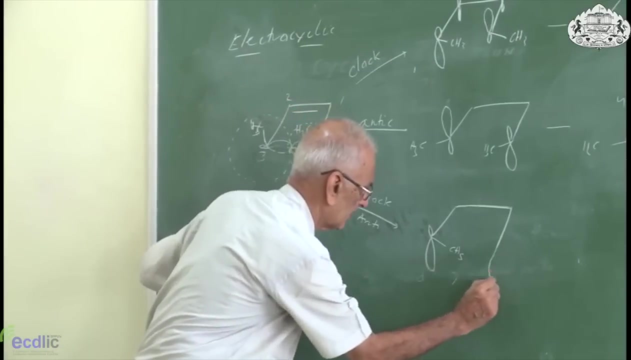 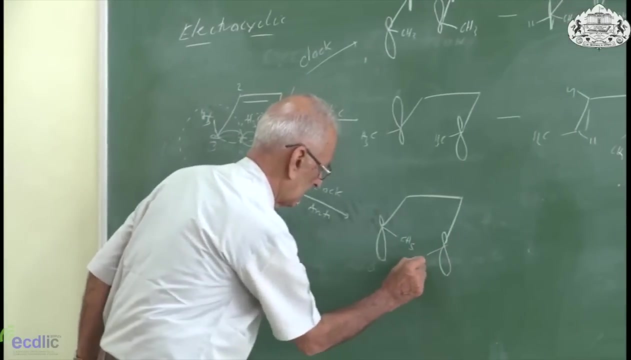 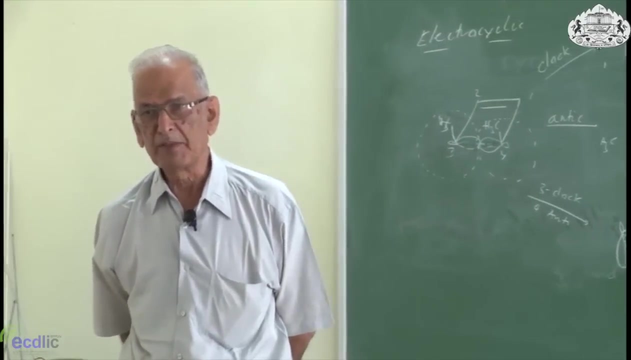 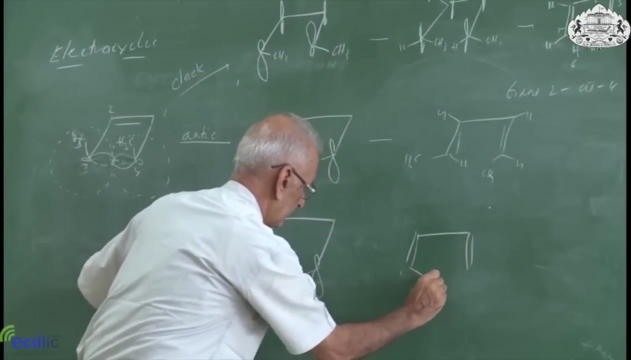 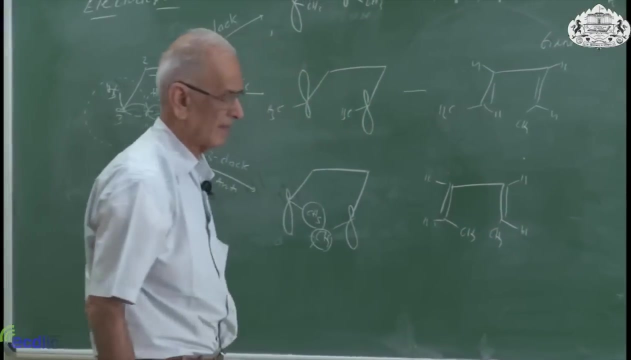 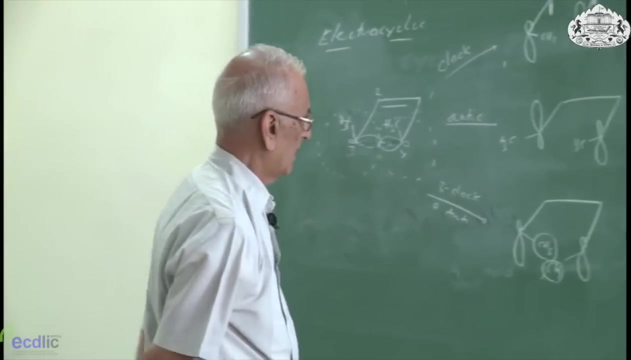 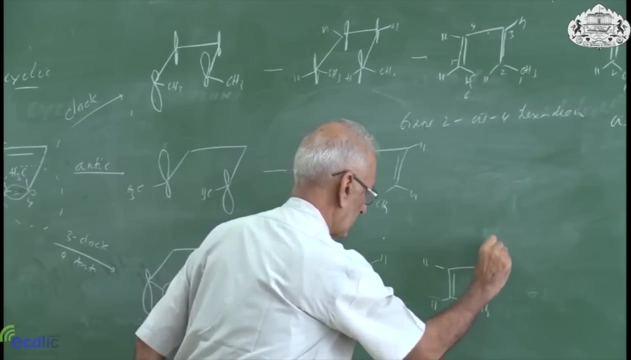 promote. the 부 Orbital at 4 position is going to move anticlockwise. Miss where will that orbital go? It will go to 6 position, 6 position. So compound is cis-cis-hexadi. 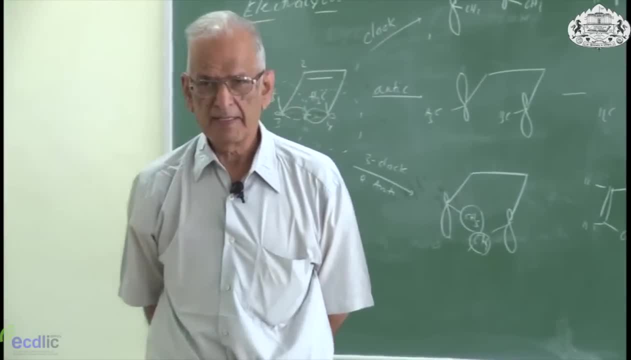 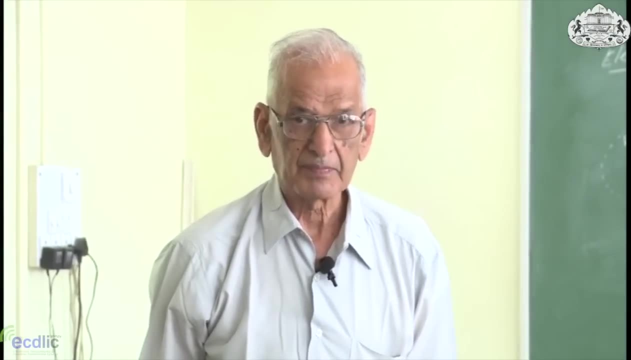 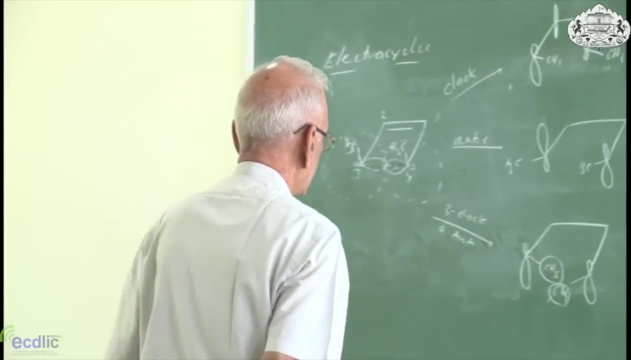 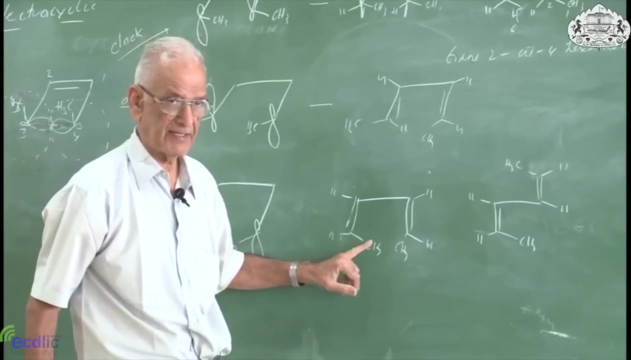 What are these two? Are they configuration isomers? are they conformational isomers? are they totally different? They are conformational isomers. What have I done? I have simply rotated around this bond. So in transition state, there is lot of problem. 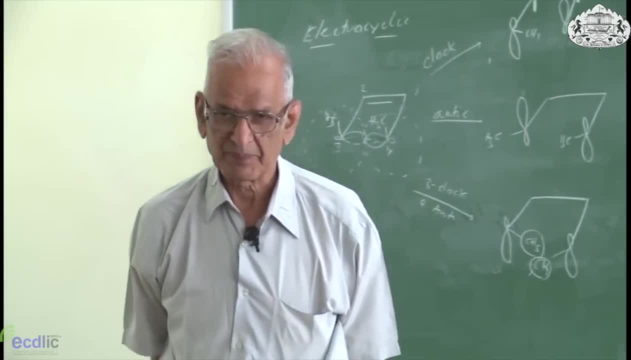 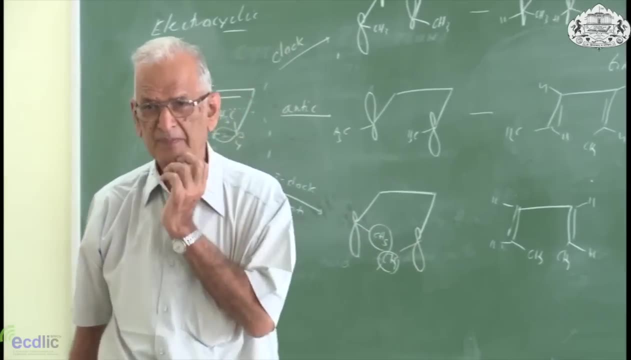 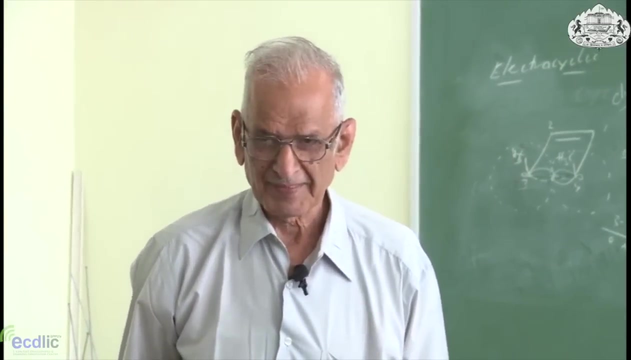 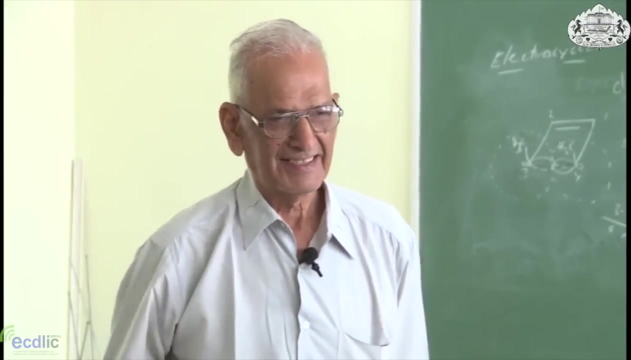 After transition state, There is no problem. This is like what happens in India. you stand at the bus stop till the bus comes. line is very good, and moment the bus comes, everybody goes out. push, push, push, push. good Indian. 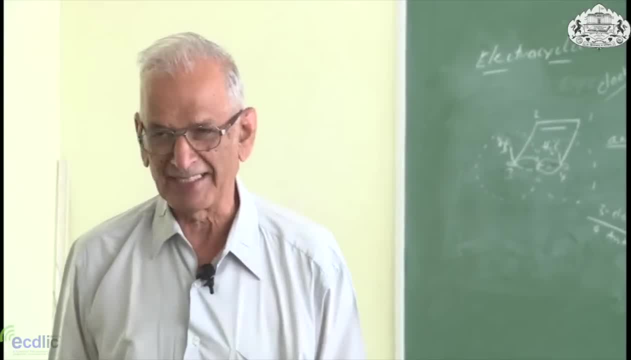 should push. If he is goes in straight line, he will push. If he goes in straight line, he will push. If he goes in straight line, something is wrong with him. I push. what about you? You push or not? 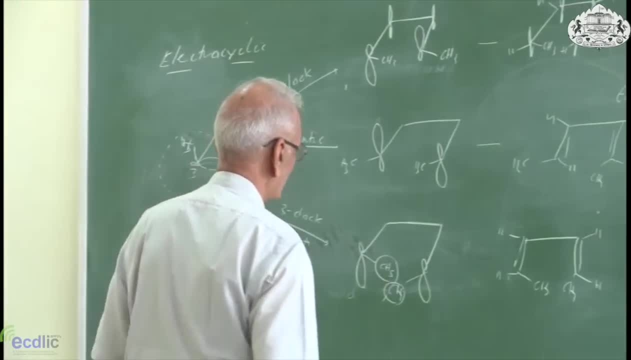 You obviously push All right, So. but afterwards, what do you see? Everybody gets position, everybody gets place, but at the door, push All right. So that is typical of our… All right, Thank you, Thank you. 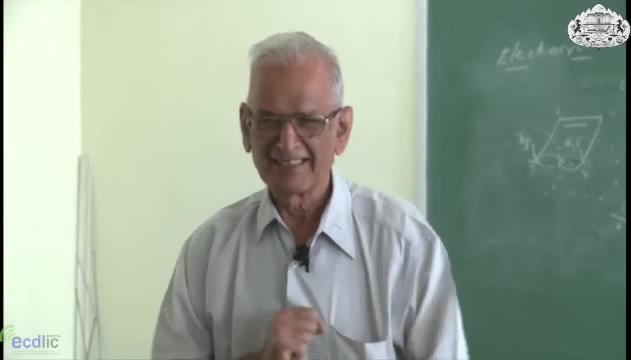 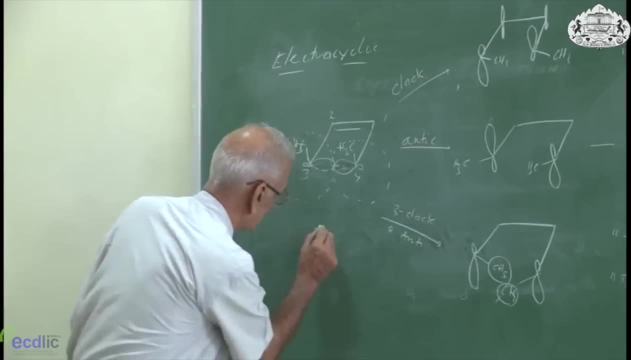 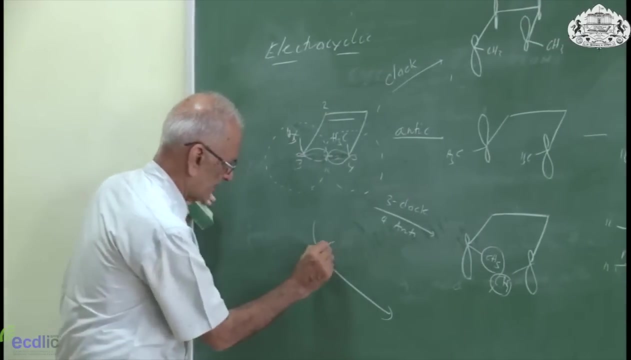 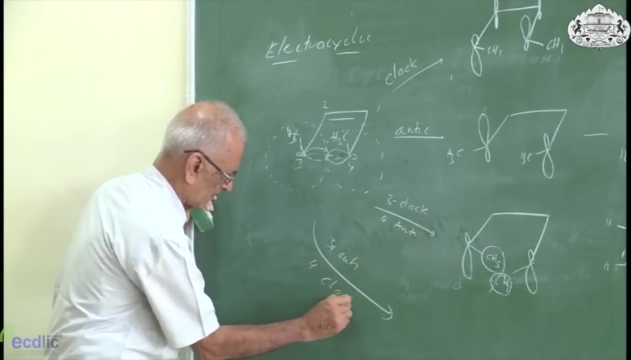 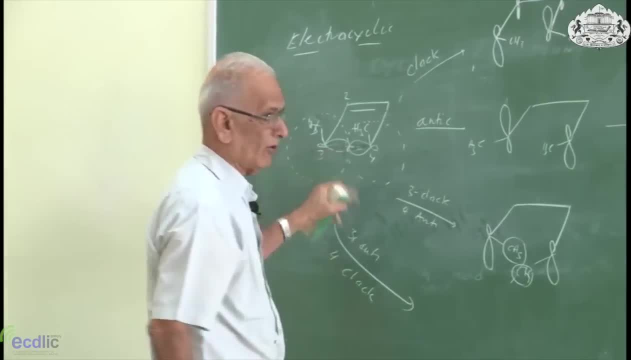 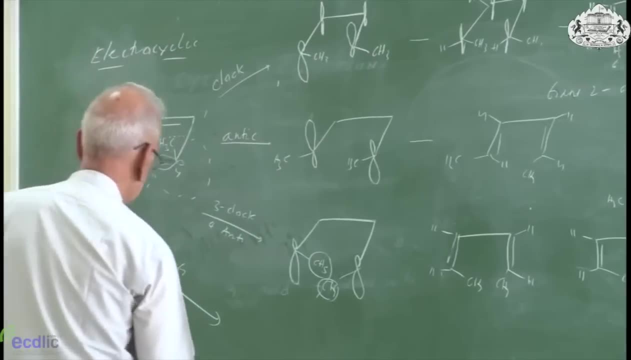 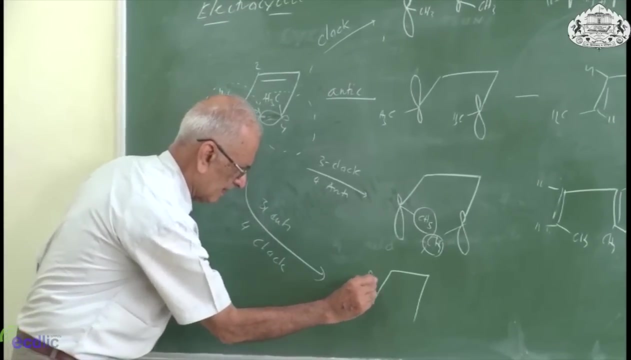 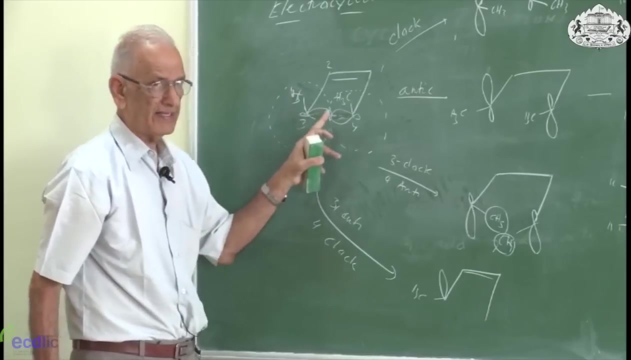 So three moves anticlockwise means where should that three orbital go? Q, L position, Where will the methyl group go? Outside, Outside, Outside, Outside. 4 is going to move clock wise. So from 9 position it will go to 12 position and your 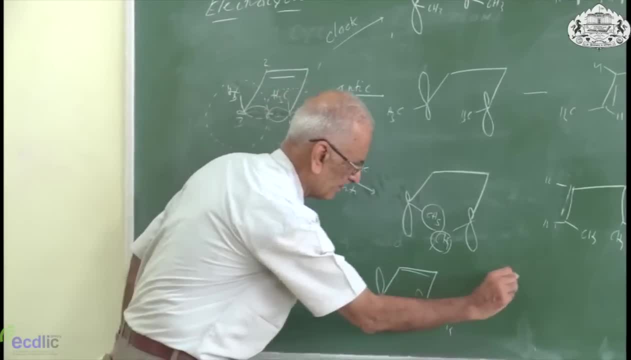 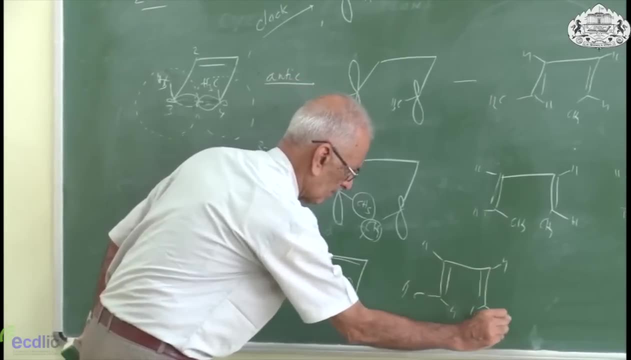 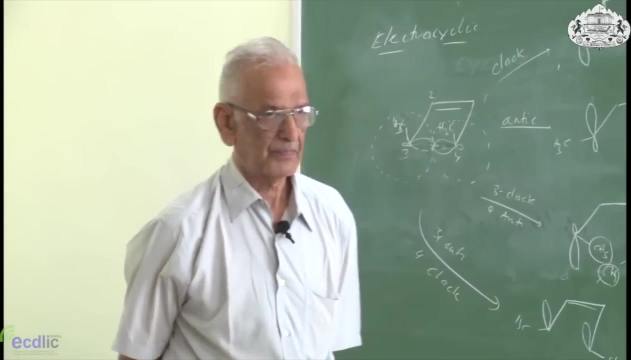 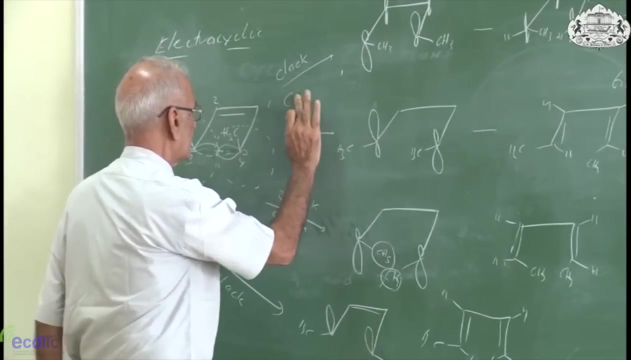 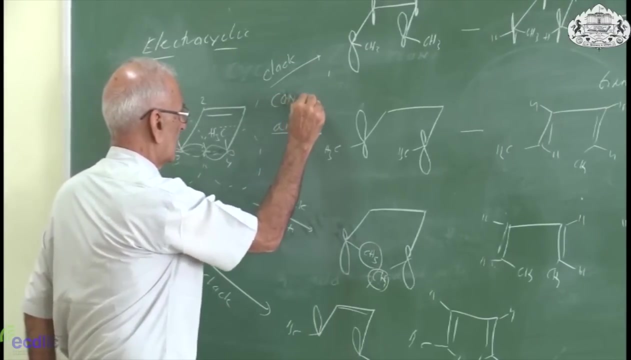 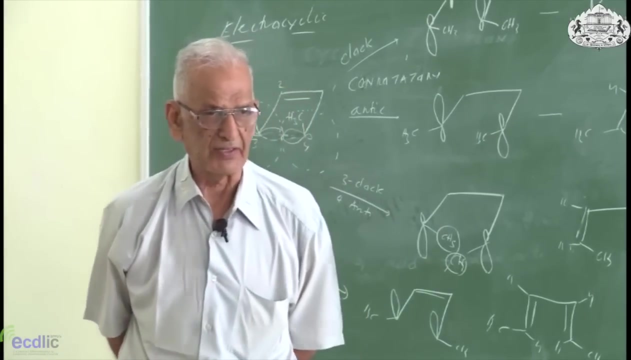 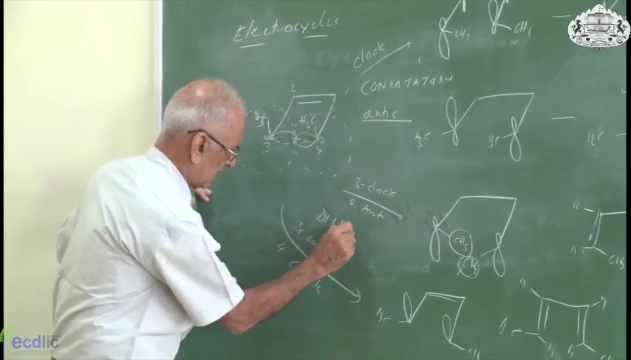 methyl group will again go outside. So this will give you trans, trans product. So when Woodward and Hoffman introduced this, if both move clock wise or both move anti clock wise, they called it con rotatory. If one moves clock wise, one moves anti clock wise. they 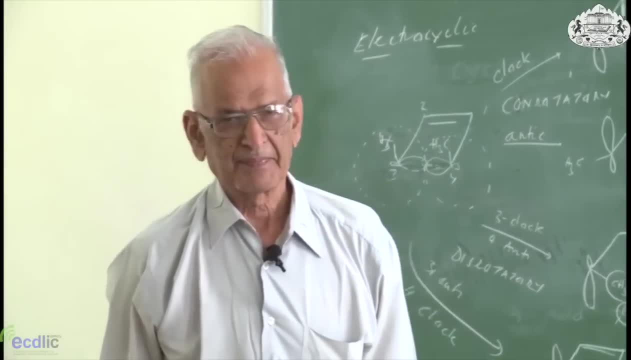 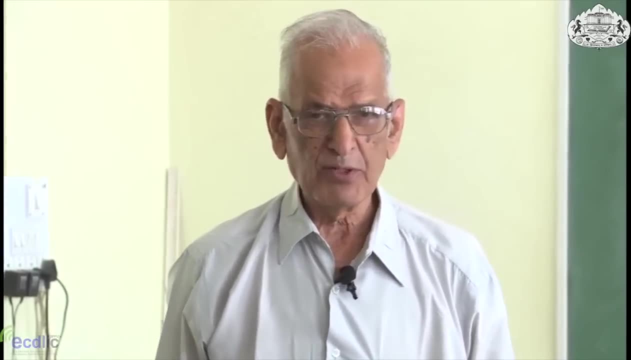 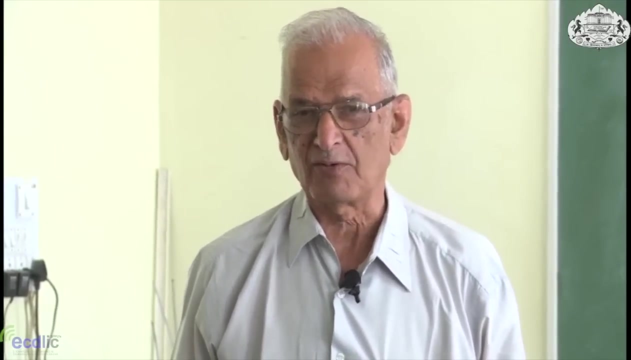 called it dis rotatory. When they introduced this word they said: everybody will know what is clock wise, what is anti clock wise. And after few years American children now do not know- at least till few years back they did not know- what is clock wise or anti clock wise, because they were not using this. 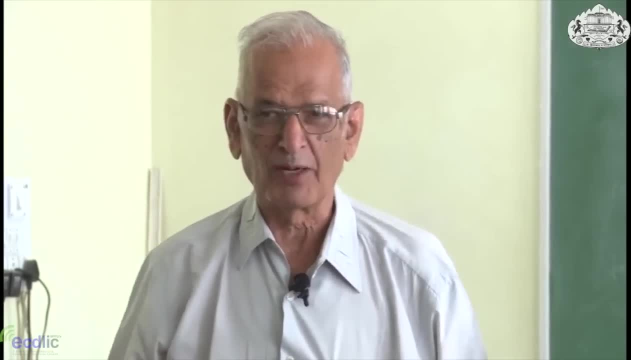 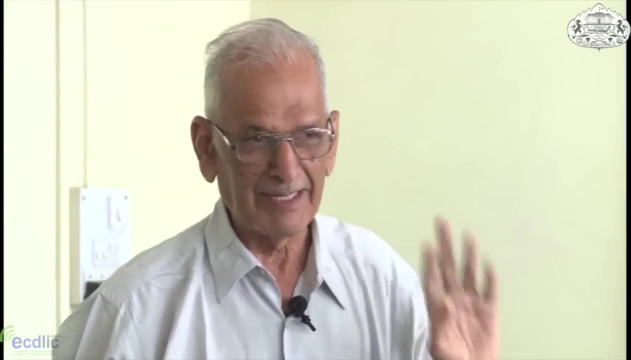 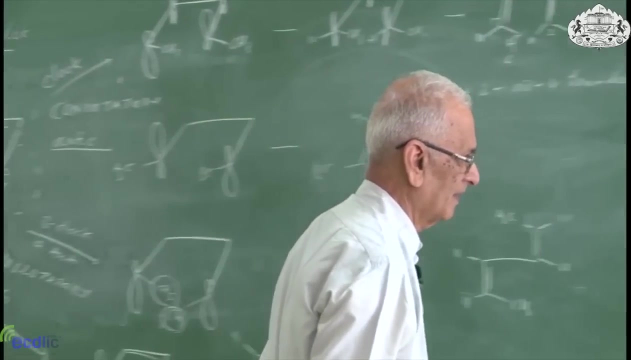 type of watch. They were using digital, So they do not know what is clock wise, what is anti clock wise. All Indian children know what is clock wise or anti clock wise Moment. the lecture knows. everybody knows what is clock wise, So we have the advantage over. 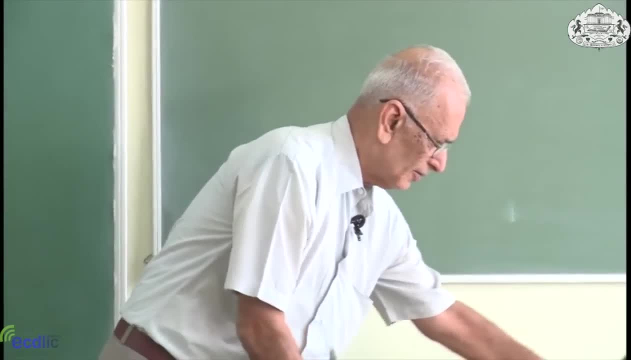 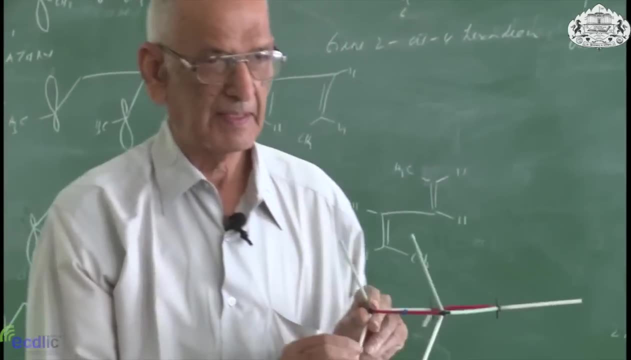 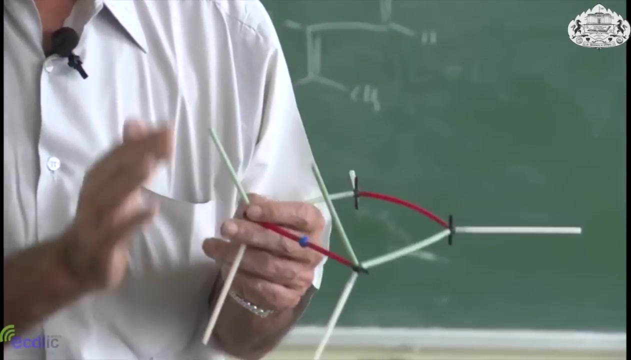 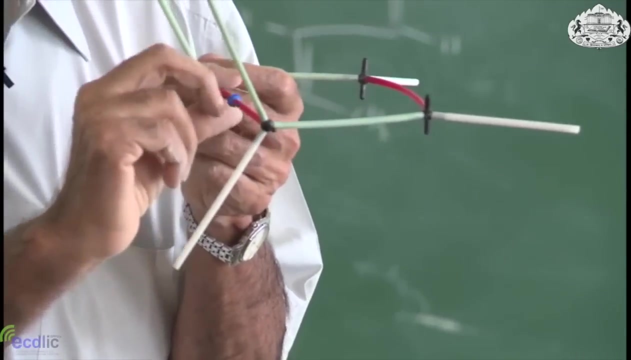 there. All right, So we did this on the blackboard. Now we are going to do this with the model. All right, Greens are metal groups, Whites are hydrogens. That red is a double bond and this is the orbital that we are going to open. All right, This is your carbon number three. this is: 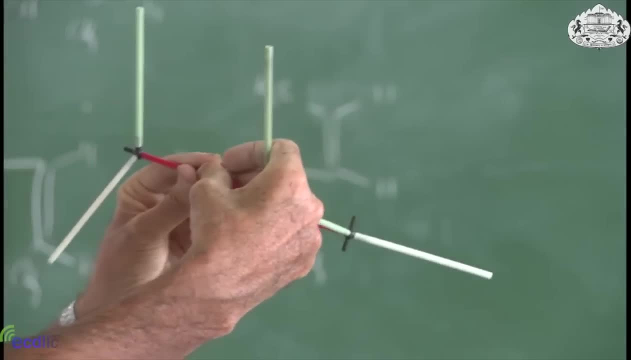 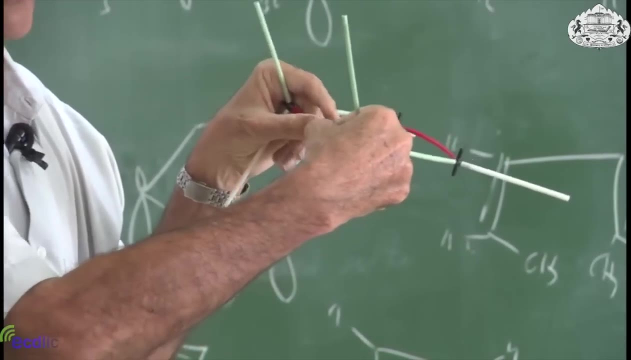 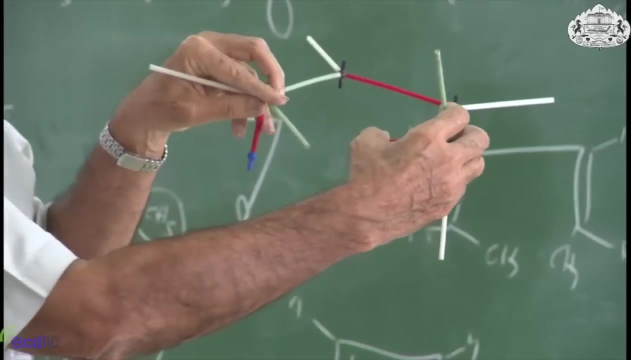 your carbon number four. Three moves, Three moves. Three moves clock wise. All right, Three moves, clock wise. So from three position it goes to six position. Where is the methyl group? Methyl group is inside. From nine position. 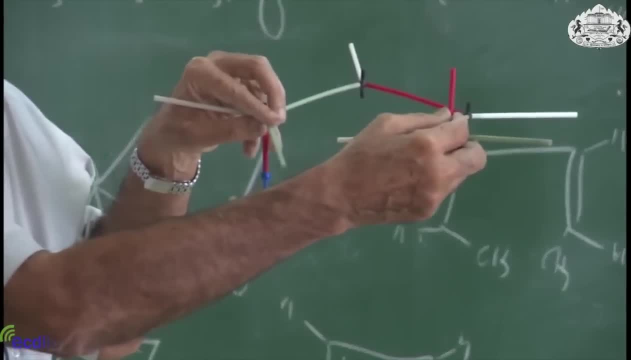 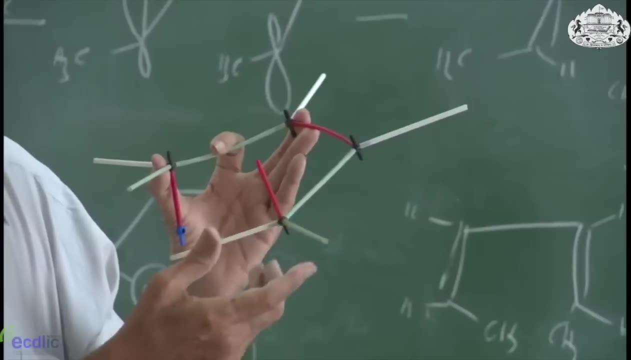 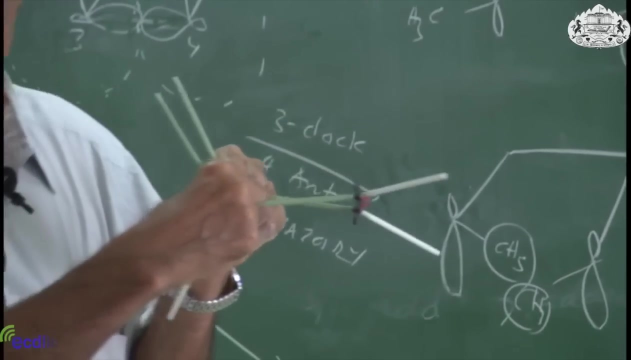 it goes to twelve position. Where is the methyl group? Methyl group goes outside. What is the product? This double bond is cis, that double bond is trans, Everything. All right, Now let us do the other one. Move both in anti clock wise manner. So from three position: 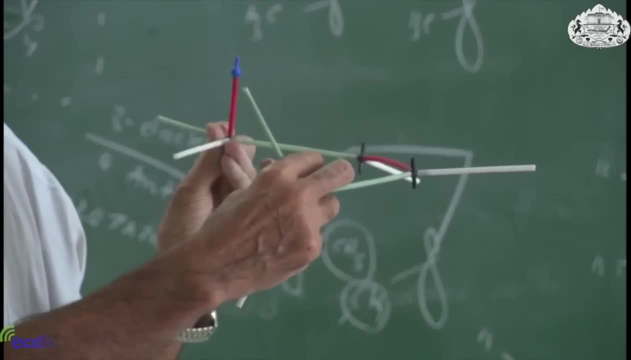 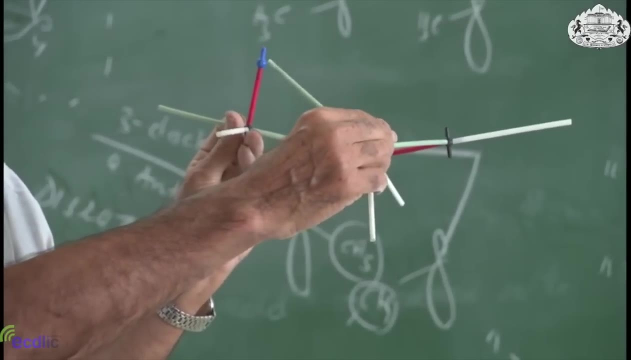 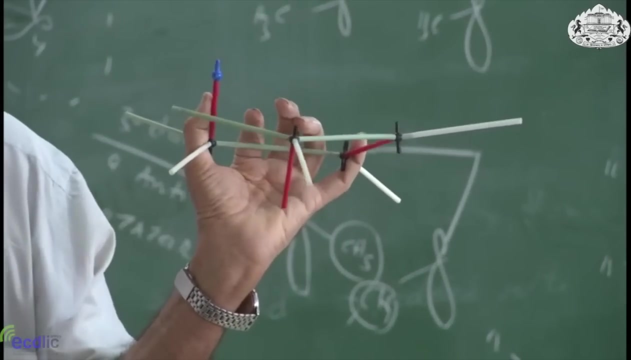 it goes to twelve position. where is the methyl group? go Outside This orbital from nine position. anti clock wise, it should go to six position. Methyl group goes inside. Now. this double bond is trans, that double bond is cis. All right. 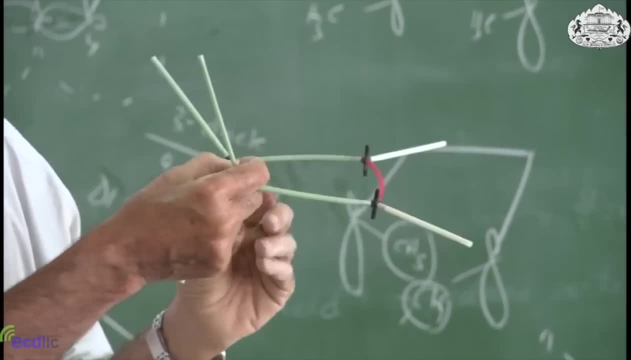 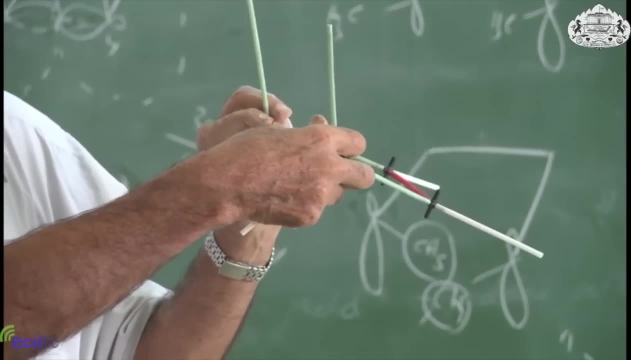 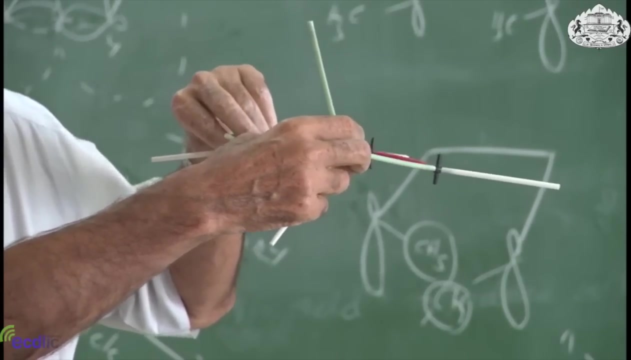 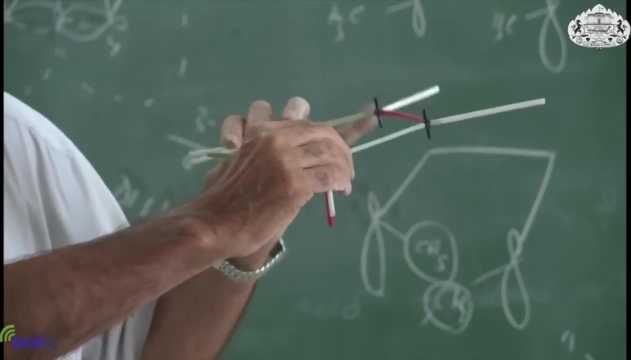 Now we are moving 3 in clockwise manner. So from 3 position it goes to 6 position- methyl group goes inside. This is now going from 9 position anticlockwise. it is going to 6 position- methyl group goes inside. This is now single bond. If I do, this problem is: 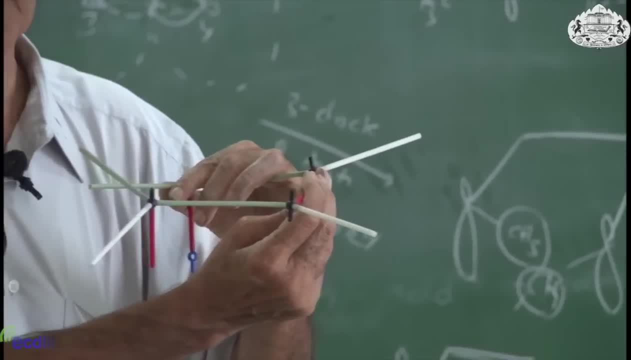 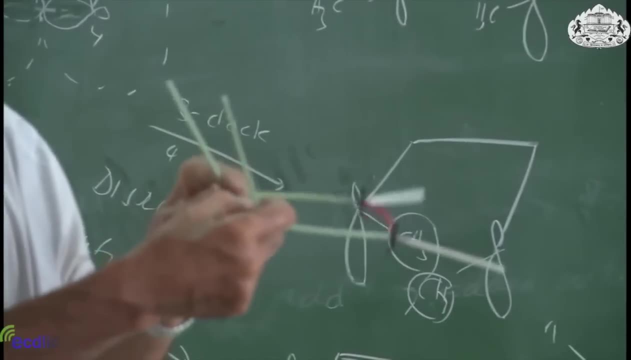 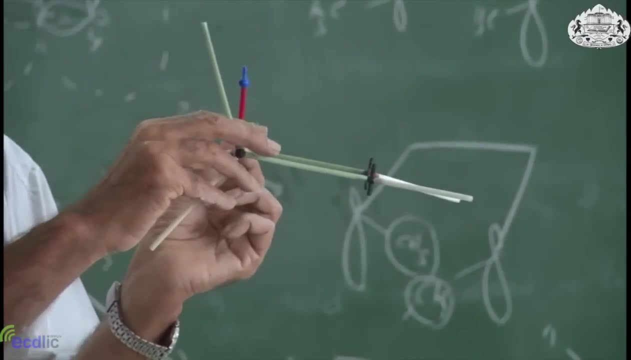 not serious, but in the transition state problem is very serious. Lets do the last one. 3 is going to move anticlockwise, So from 3 position it goes to 12 position. and this is going to move clockwise, So from 90 it goes to 90.. 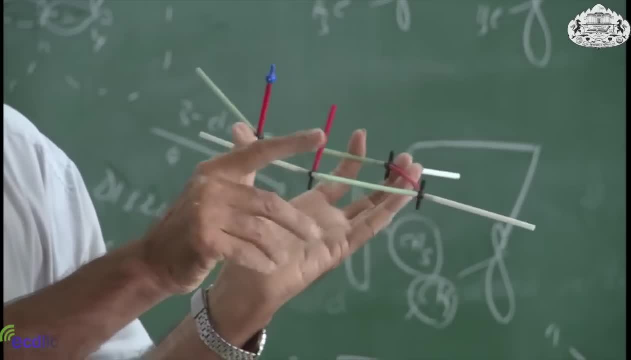 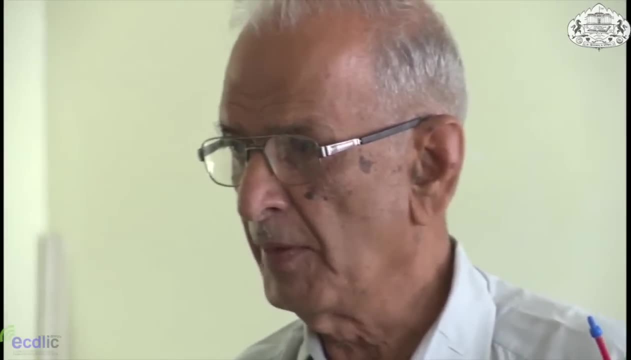 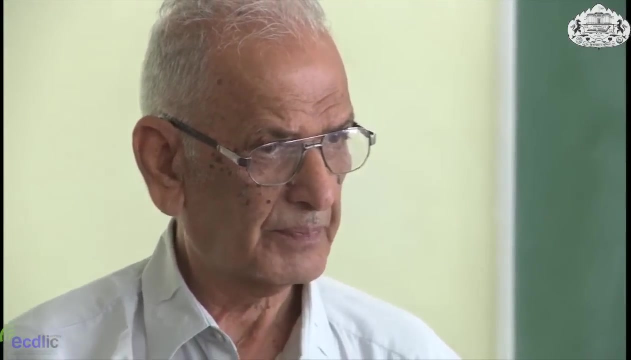 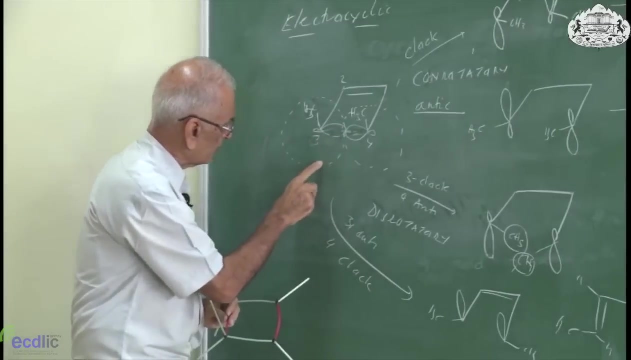 position, it goes to 12 position. So both metals are outside, both double bonds are trans, No problem, Everything clear, Everybody is. everything clear, No difficulty at all. I have, Why did we move this from 3 position to 6 position? Why not 9 position? Why not? 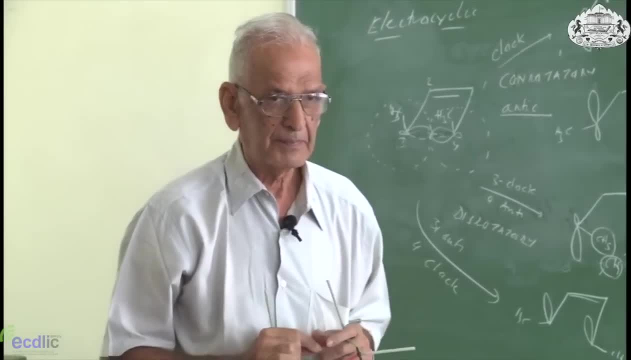 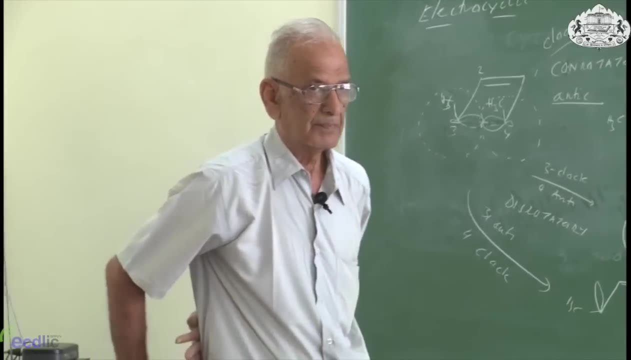 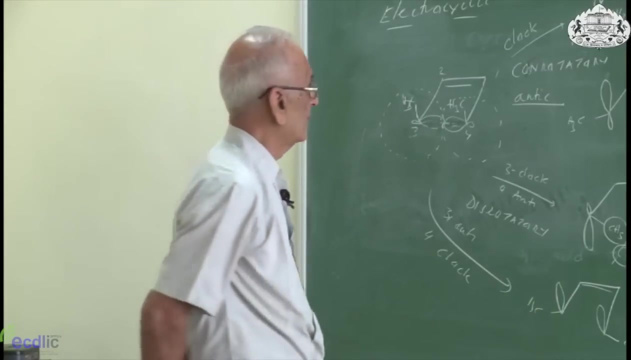 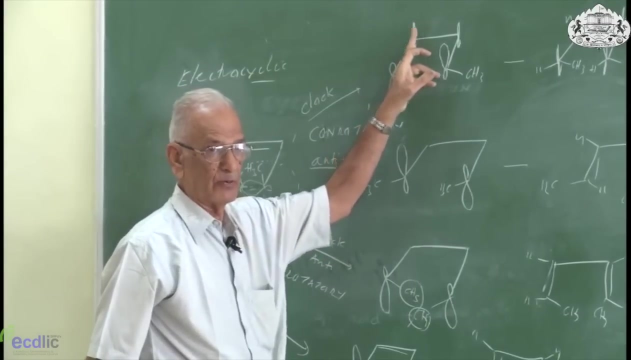 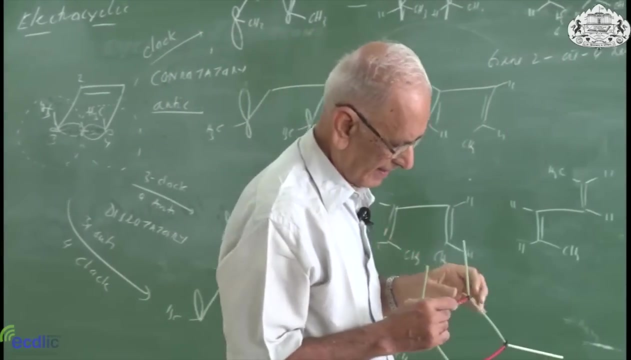 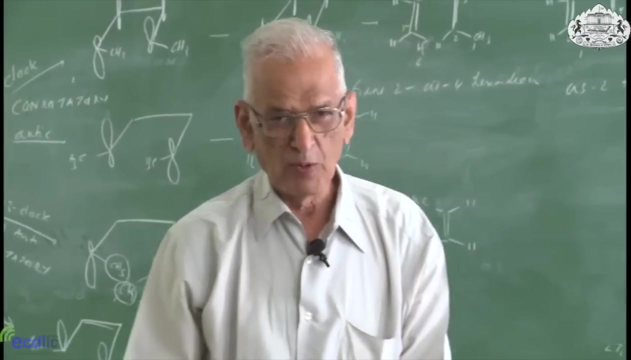 7 position. What did we say? This orbital is to be made into p orbital, So it must be parallel to this. So I can only move it to 6 position or to 12 position. Long back there used to be the people used to ask in the old days in Greece, everybody. 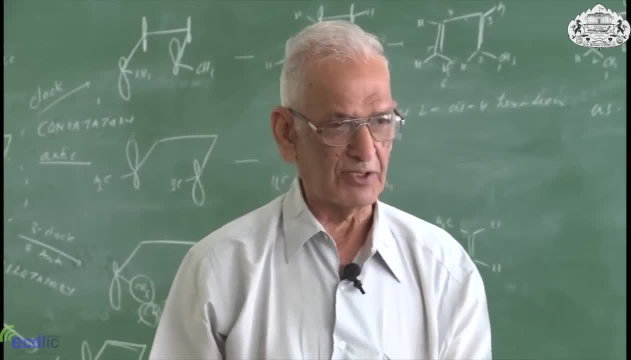 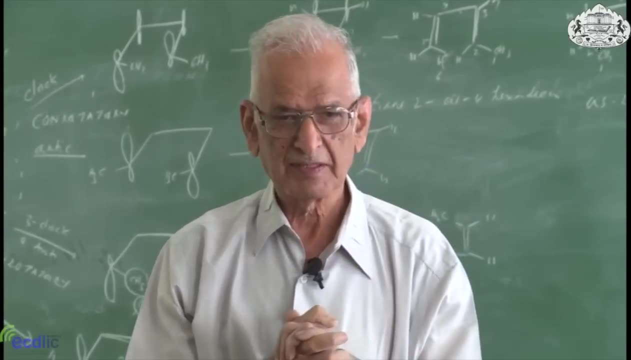 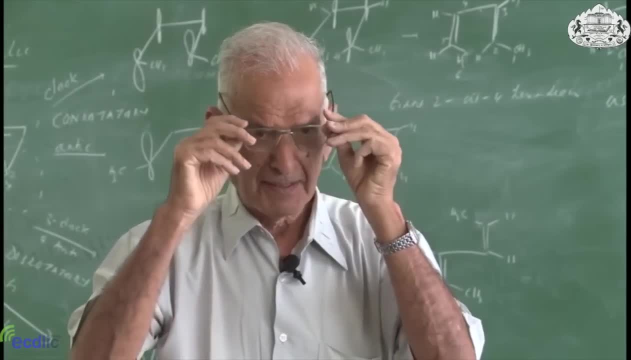 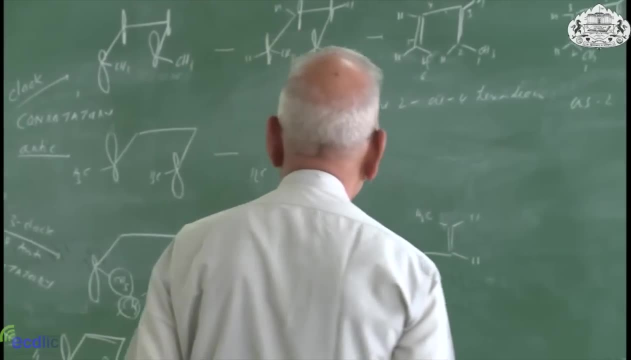 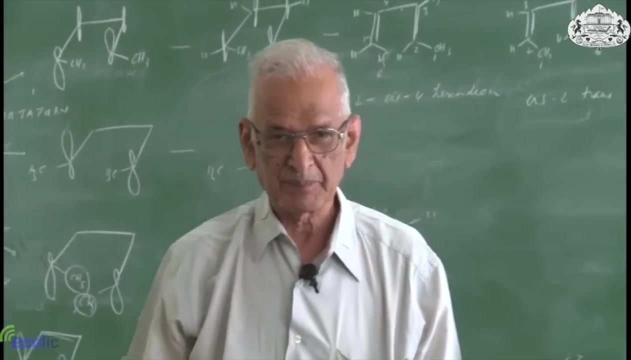 knew that when you become old, you will have to wear spectacles. So if your ears were here or somewhere here, you would have problem. So that is the proof that God is there. God also knew that organic chemist will have problem. So that is the second proof that God is there. 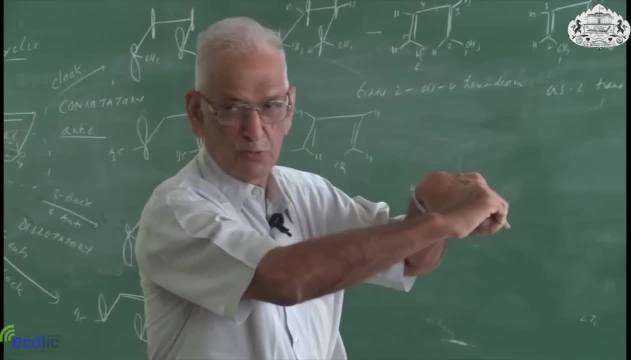 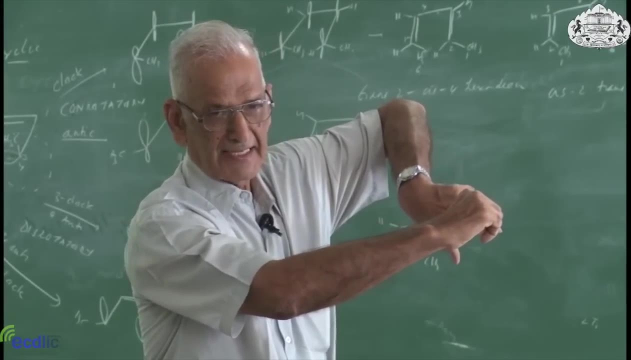 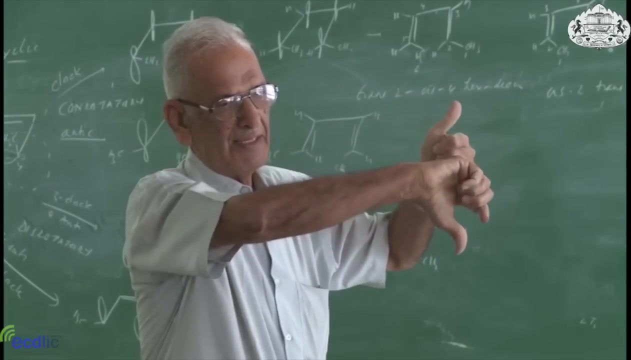 That is your orbital, which you are going to open. That is your two metal groups. So move it to 6 position. what happens? Methyl group goes inside. Move this to 12 position. methyl group goes outside. Move it anti-clockwise. this is inside, that is outside. Move this clockwise methyl group. 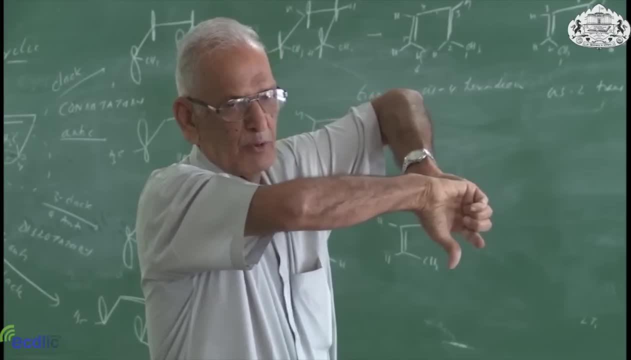 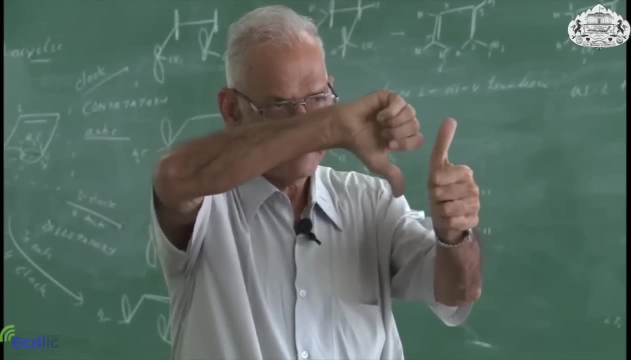 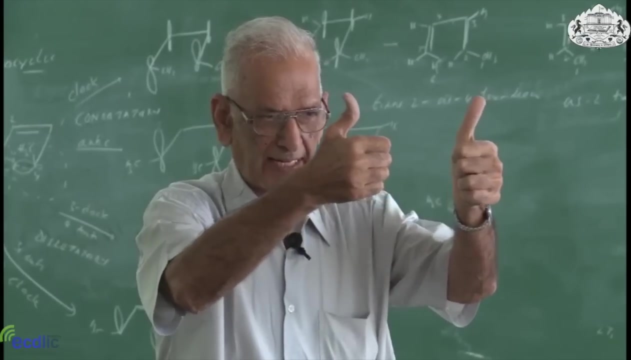 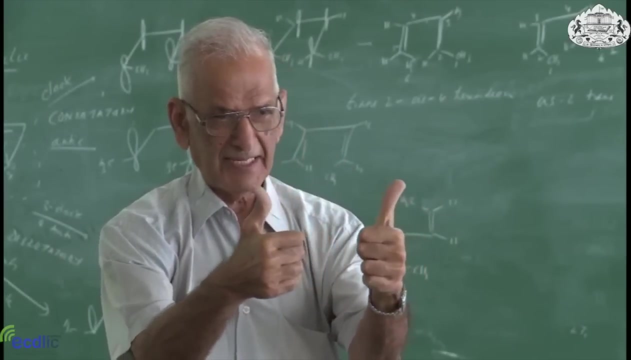 goes inside. Move this anti-clockwise. both are inside. Do it opposite, both are outside. So what have you to remember? In corn rotatory, one thumb is up, one thumb is down. In disc rotatory, both are up or both are down. So how do you remember? Disc rotatory means you. 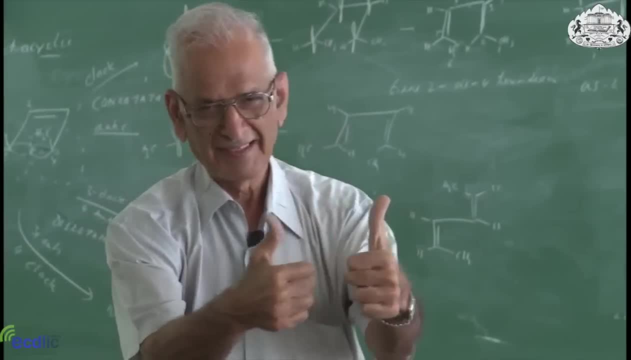 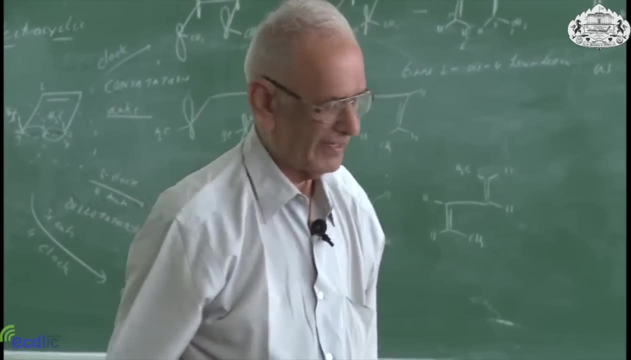 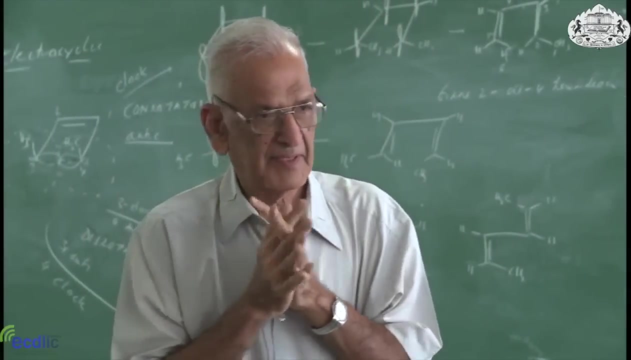 think of thumbs up. You think thumbs up or no. So that is your disc rotatory. It is a thumbs up or a thumbs down. In corn rotatory one is up, one is down. What are the salient features of what we have spoken? Number one: pericyclic reactions. 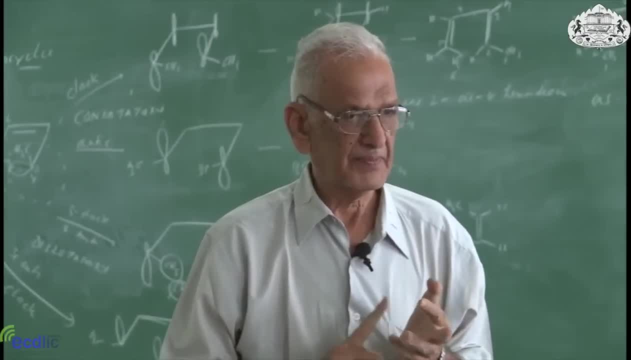 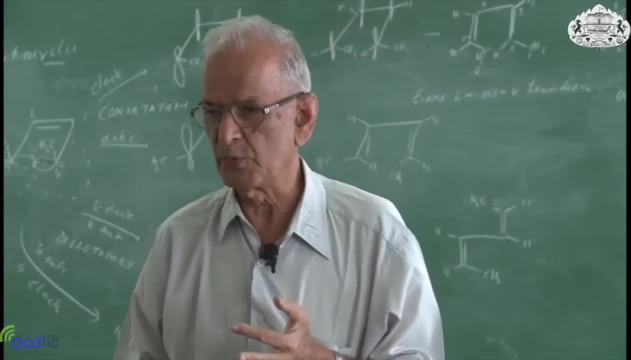 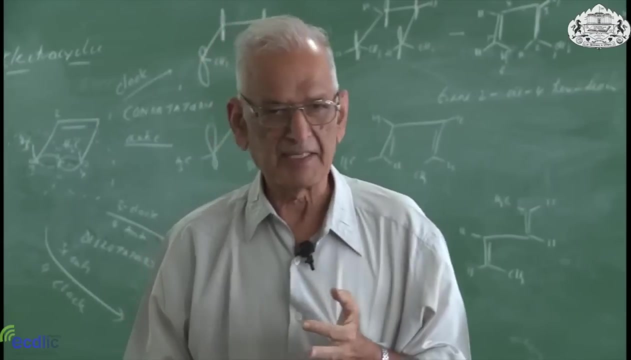 are of three types: electrocyclic, cycloaddition and sigmatropic. In an electrocyclic, you go from n? pi to n minus 1 pi. In a cycloaddition, you go from n pi to n minus 2 pi. In a sigmatropic, 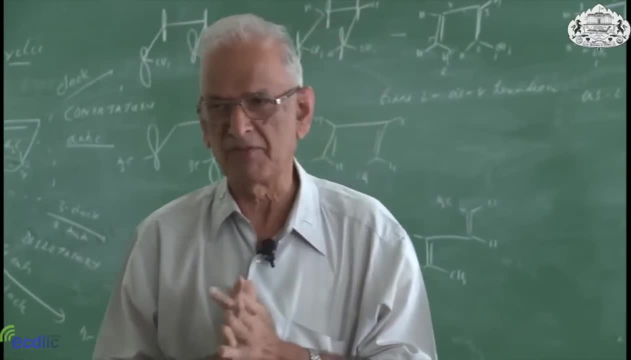 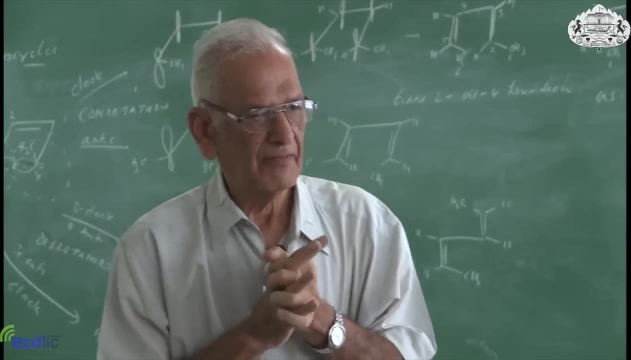 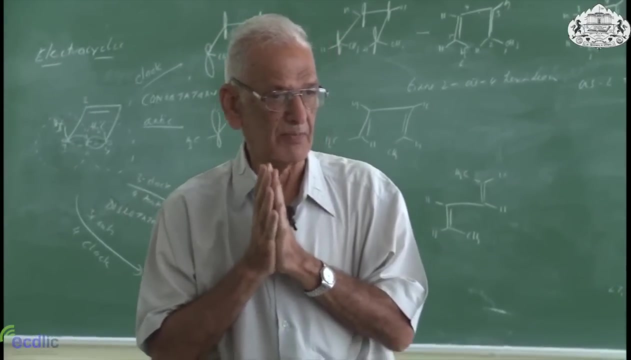 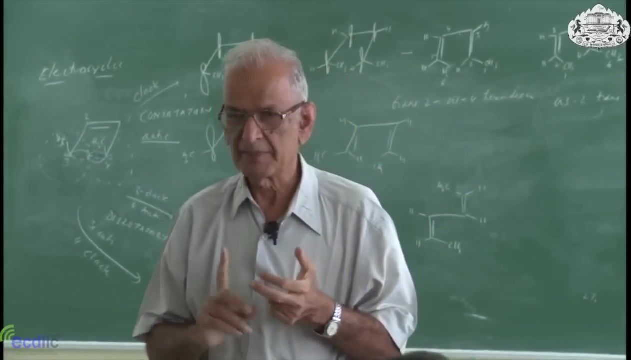 you go from n? pi to n pi: No change in number of double bonds, no change in number of double bonds. Then we gave the features of the pericyclic reaction, Then we emphasized what is the importance of pericyclic reaction. You get carbon-carbon bond formation, you get stereospecific 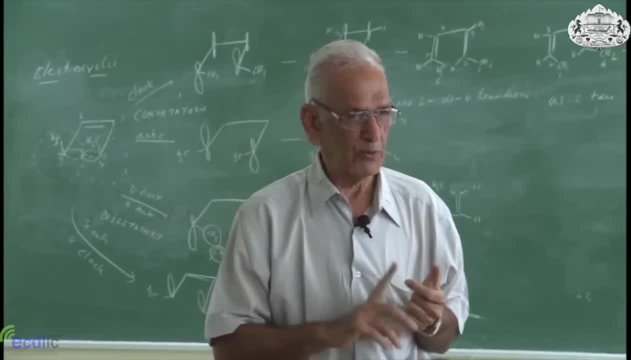 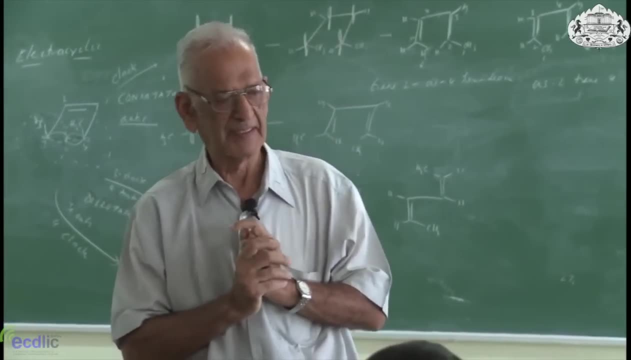 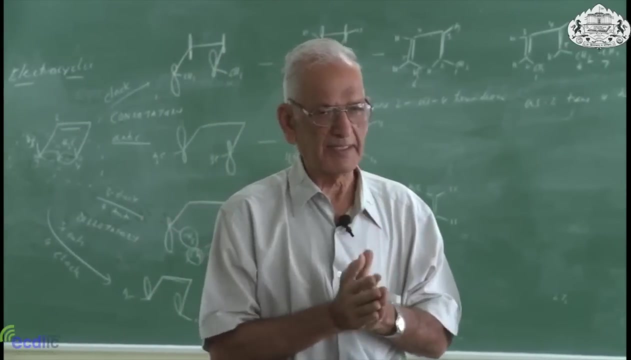 you get high yield. Today, if you want to synthesize any big molecule, usually there will be at least two or three pericyclic reactions. Then we looked at electrocyclic, And when we looked at electrocyclic we have corn rotatory. 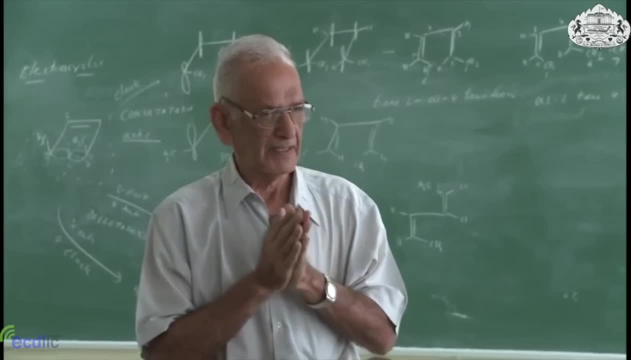 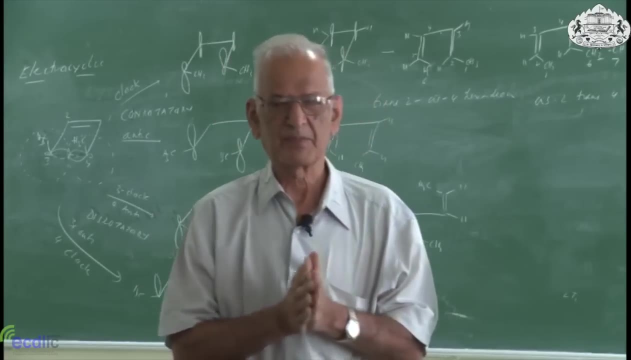 In corn rotatory you move both orbitals, either clockwise or both orbitals anticlockwise. In a disc rotatory you move both orbitals, either clockwise or both orbitals anticlockwise. In a disc rotatory you move one in clockwise manner, one in anticlockwise manner. So corn. 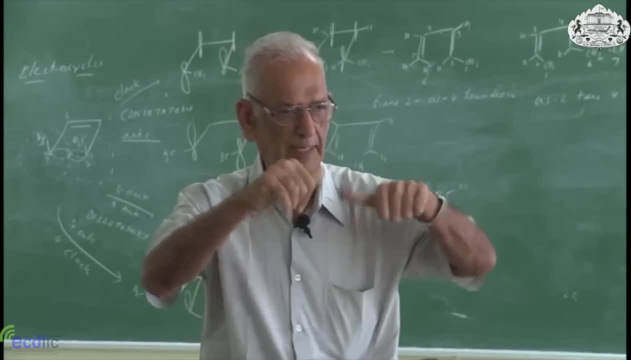 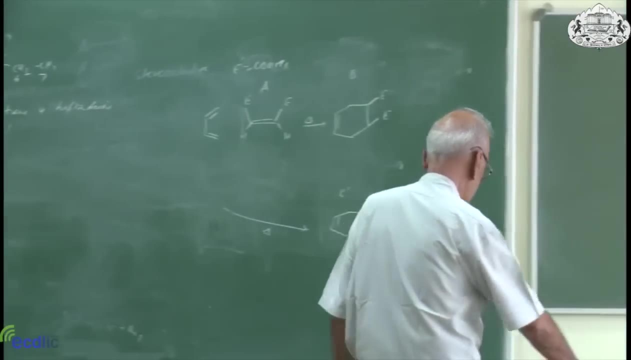 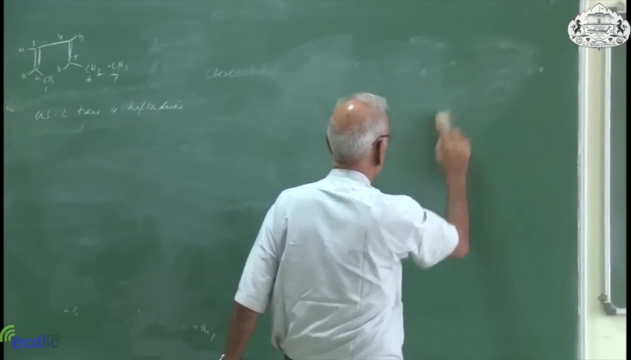 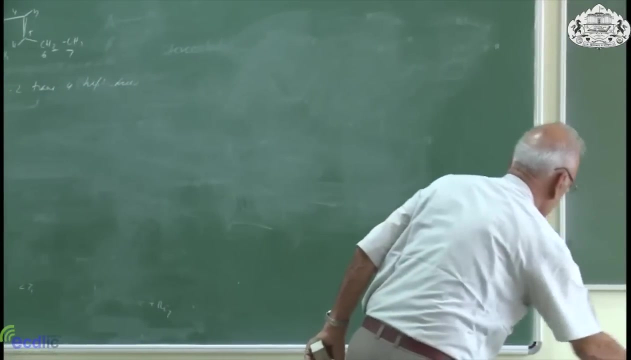 rotatory thumbs are up In disc rotatory, both up or both down. That is the features that we looked at. What was the important contribution? These things were known. If I take a system which has four electrons, this is a four electron system Which are: 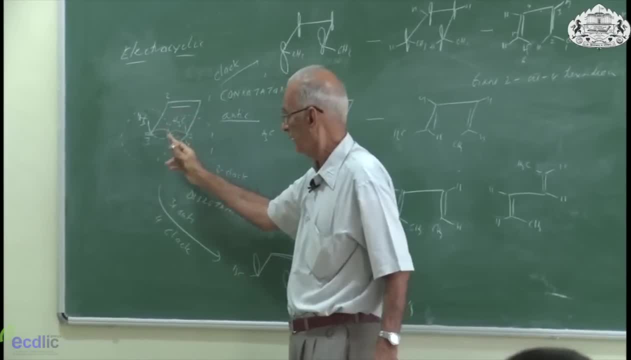 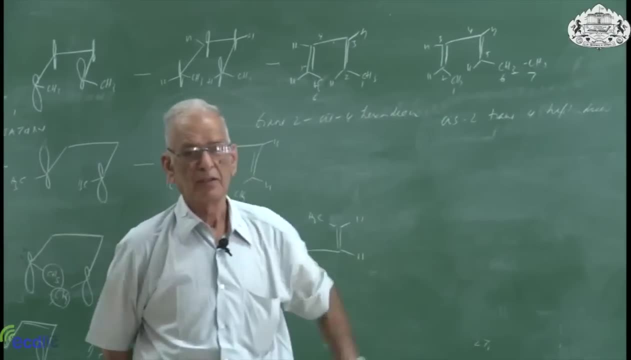 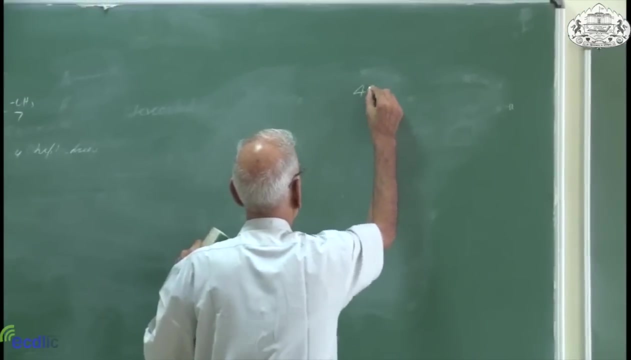 the four electrons: Two electrons of the double bond, two electrons of the single bond. In the product, your four electrons are the four electrons of the two double bonds. When you do- sorry, Yes, When you do- the reaction with four electrons, two electrons will cumulate. For example, 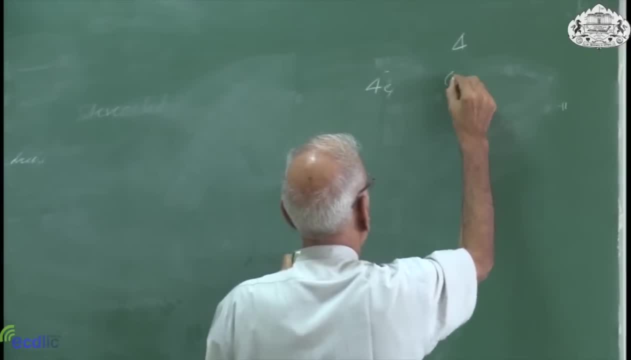 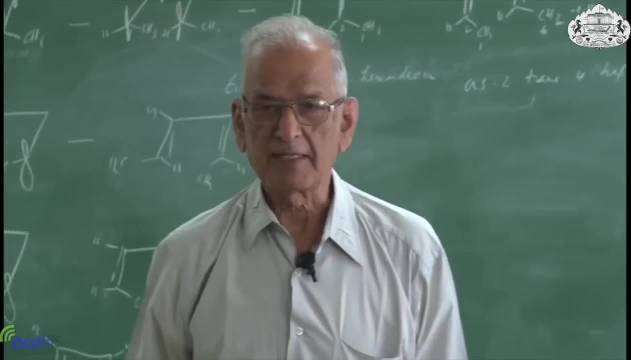 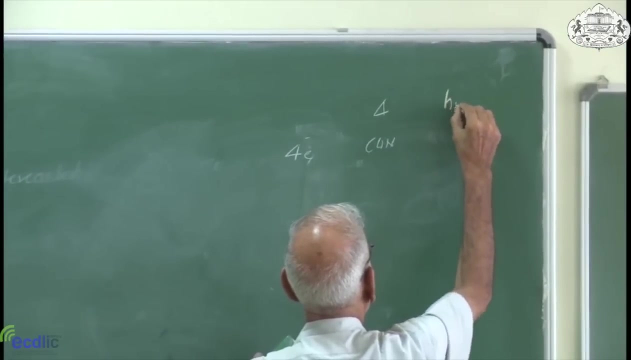 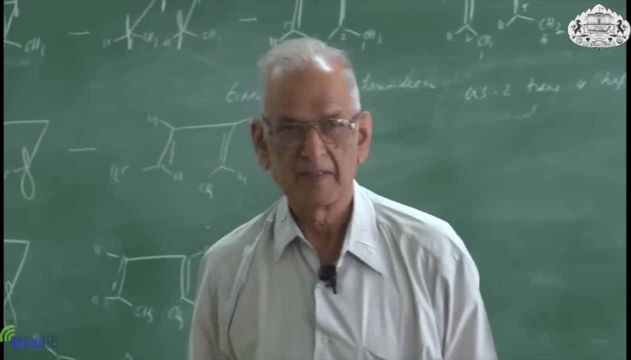 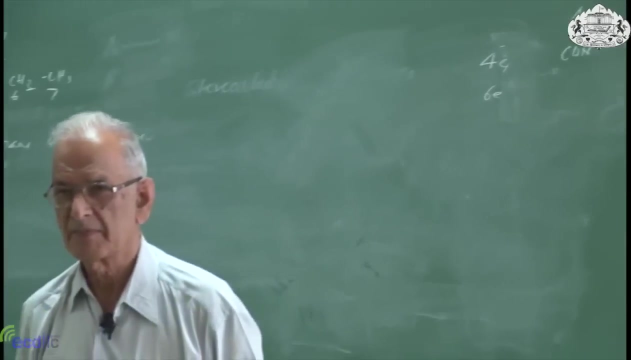 Here, say this protocol: We have one electron, two electrons, two electrons of the single bond electrons. after looking at lots of reactions you find that product is convoluted. If I do it photochemical, the product is dis-rotated. When I do it with six electrons, the thermal, 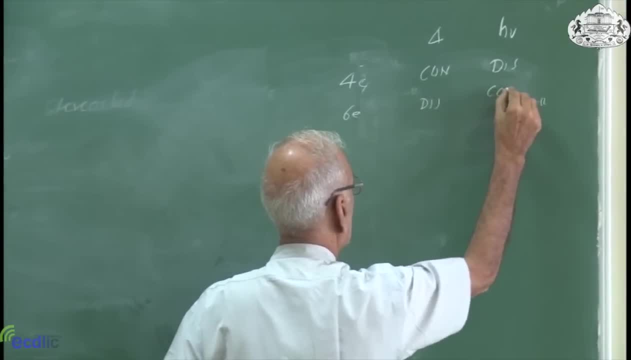 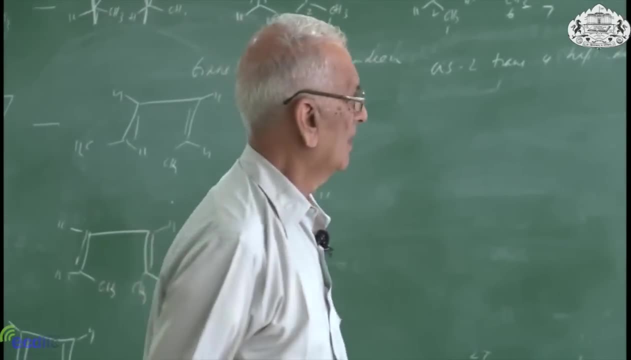 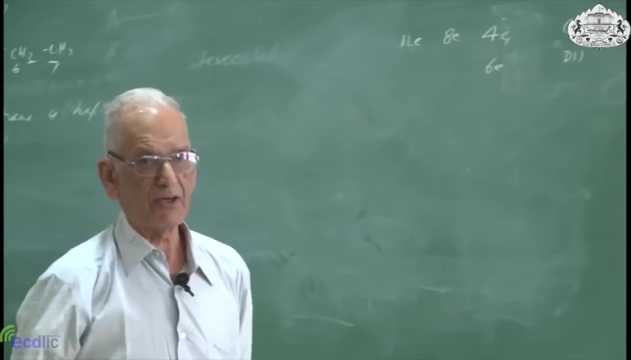 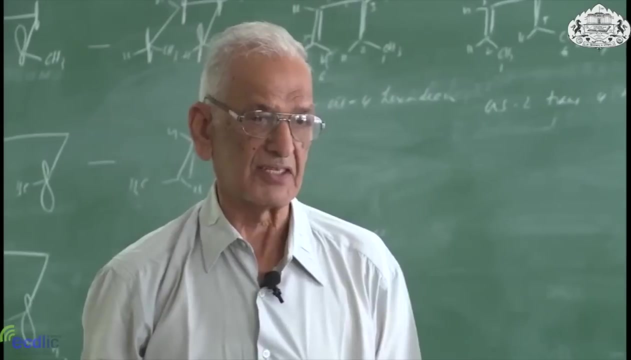 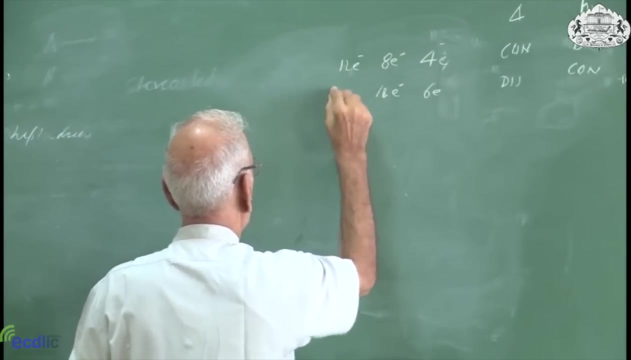 reaction is dis-rotatory, the photochemical reaction is convoluted. If I use eight-electron system or twelve-electron system, thermal reaction is convoluted. photochemical reaction is dis-rotated. Ten electrons or fourteen electrons: thermal reaction is dis-rotatory. 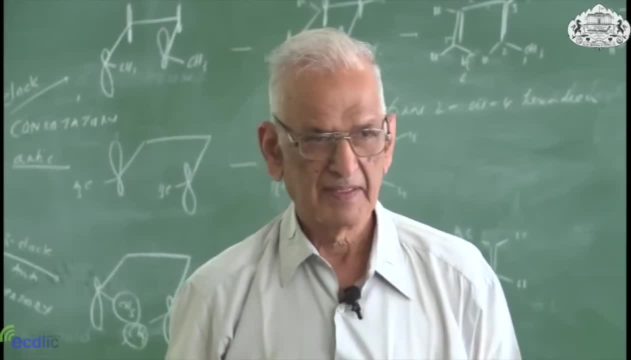 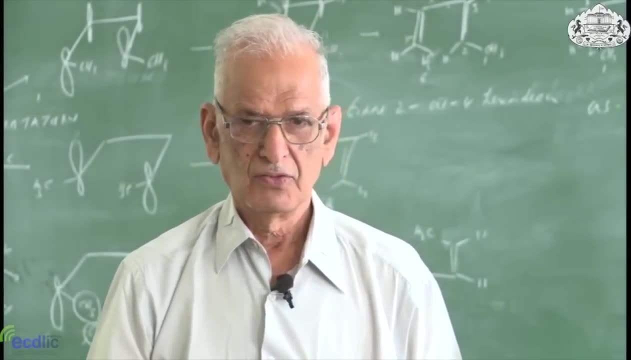 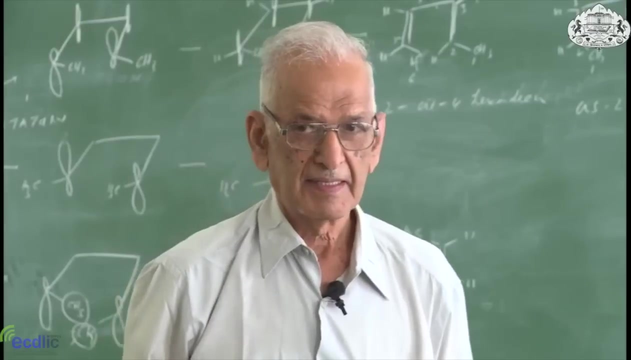 photochemical reaction is convoluted. Four-electron system behaves in one way. four n plus 2 behaves in different way, which is the very famous rule that links to this Huckel's rule. What is that? Huckel's rule A closed. 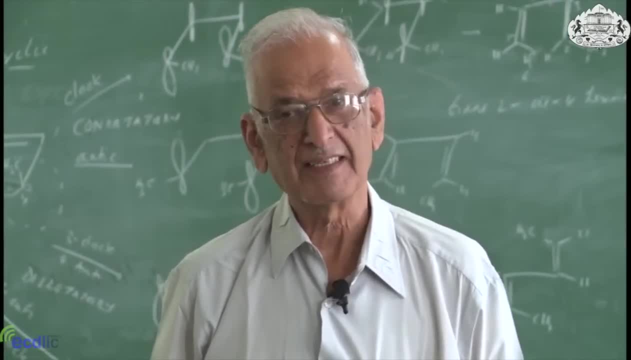 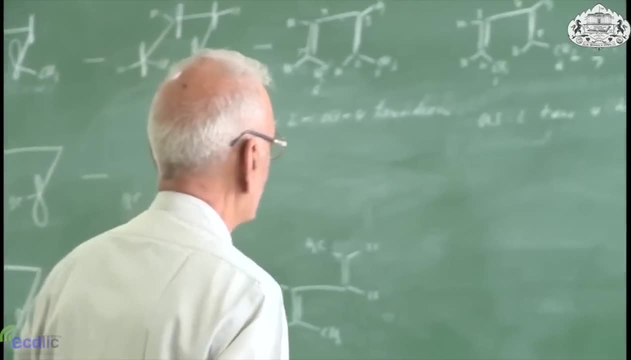 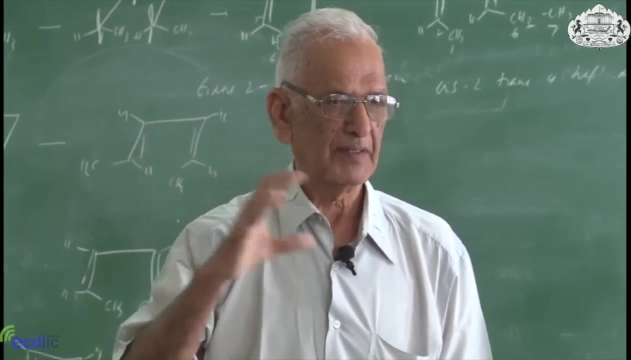 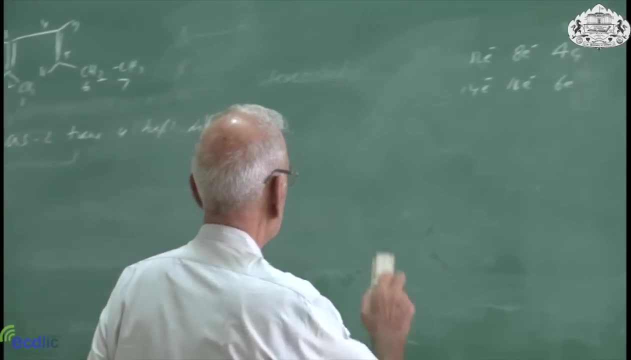 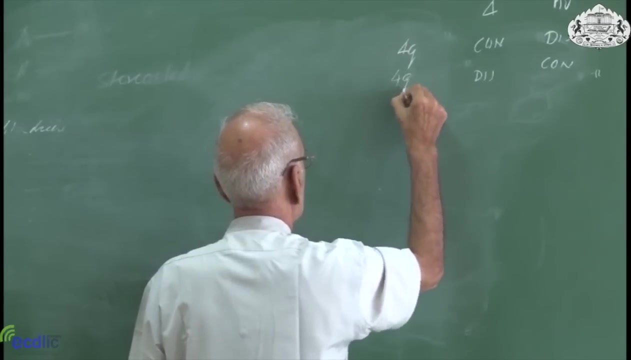 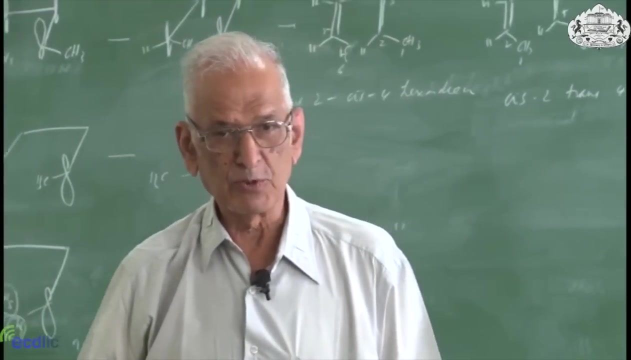 cyclic system with four n plus 2 pi electrons is aromatic, and if it has four n, it is anti-aromatic. So once you correlate with this, it seems to follow some logic. Four is anti-aromatic, six is aromatic. So we now say it like this: Why are we using q? We do not want to confuse. 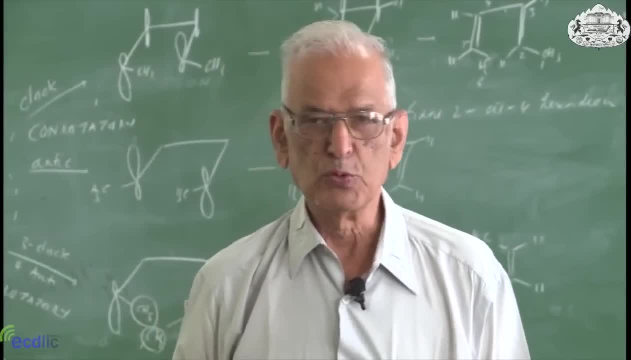 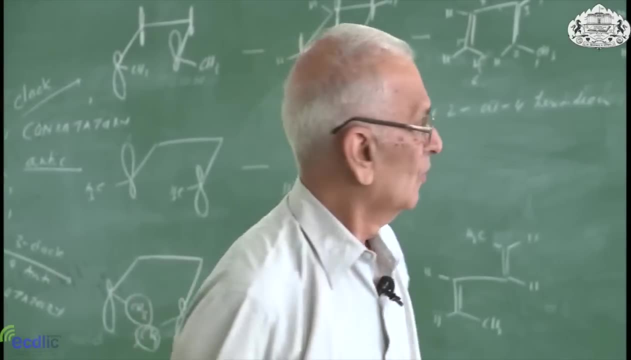 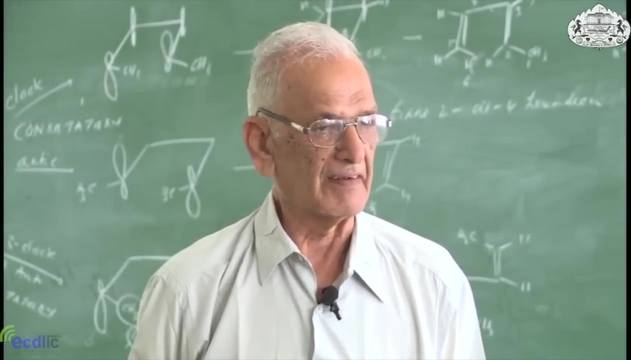 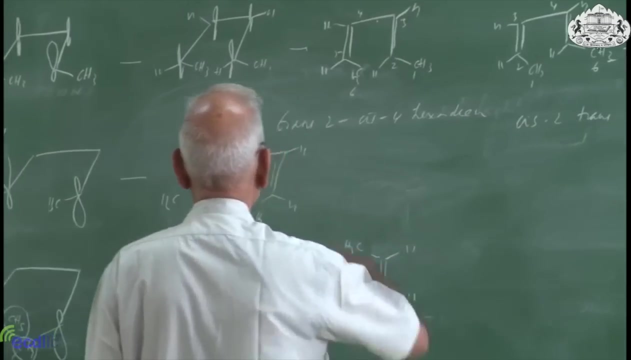 it with the Huckel's rule. So four q- the thermal reaction is convoluted, photochemical reaction is dis-rotated. Four q plus 2, picture is opposite: Thermal reaction is dis-rotated, photochemical reaction is convoluted. So that is the picture that you see. 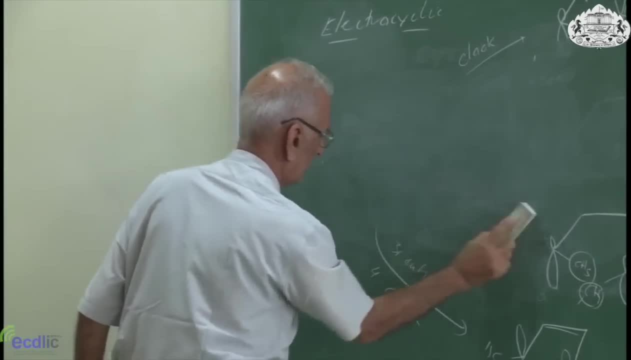 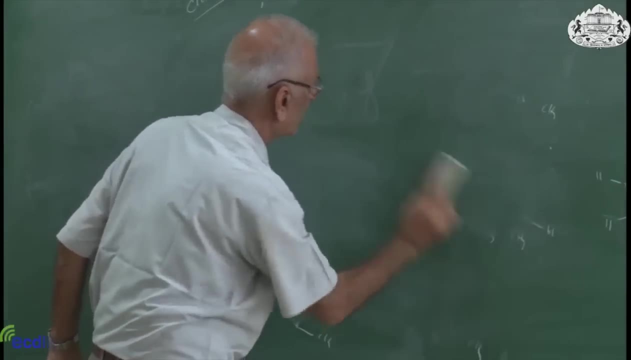 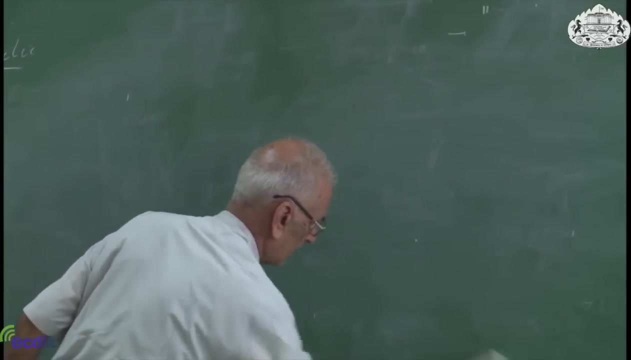 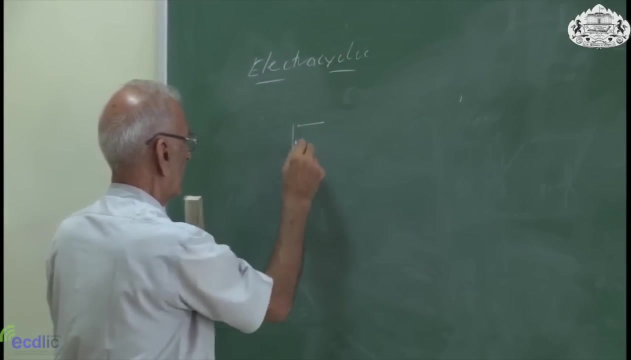 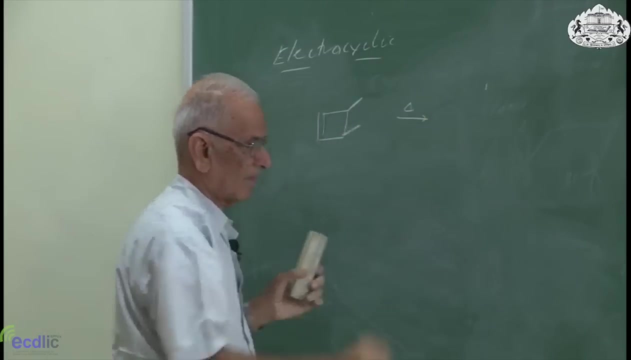 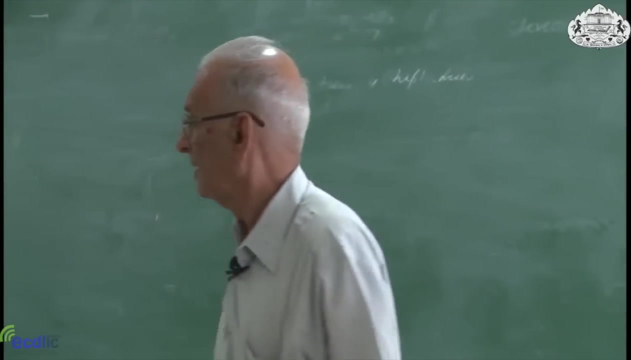 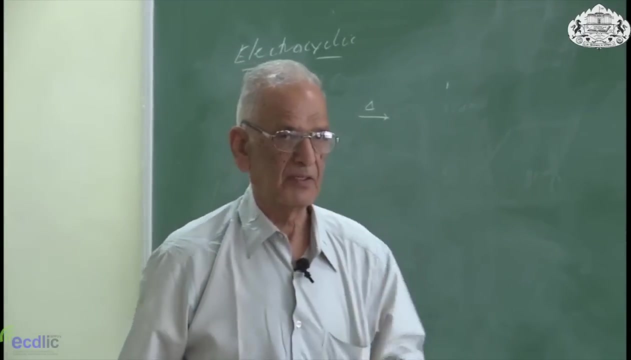 verändertion Huckel's rule. Sorry, ix, you heat it. How many electrons? 2 electrons here, 2 electrons here. So it is a 4 Q system. 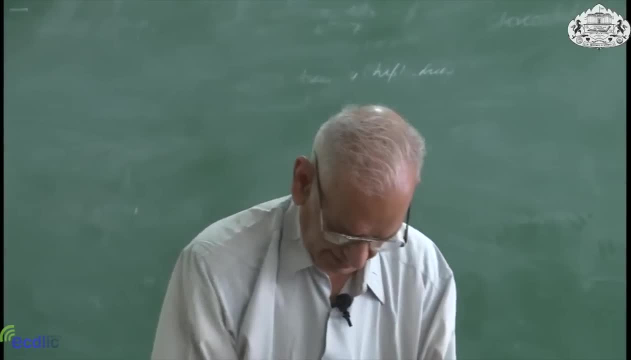 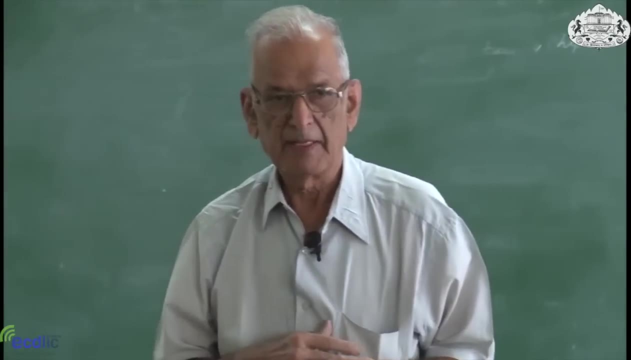 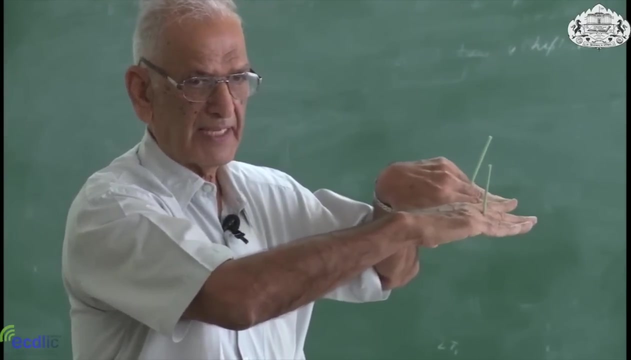 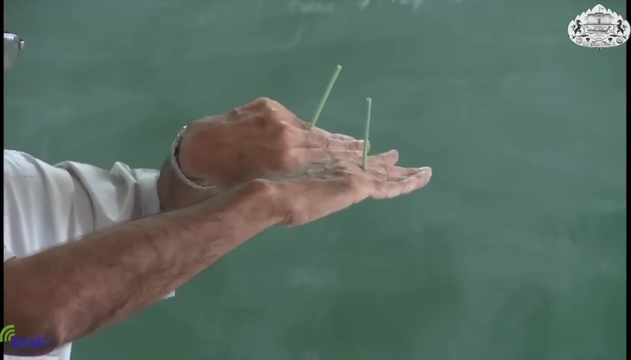 Therefore, reaction should be convoluted. So, in order that we do not make any confusion, let us see this. What are these two? These are your methyl groups, and your thumbs are moving opposite direction, sorry, in clockwise direction, both clockwise or both anticlockwise. 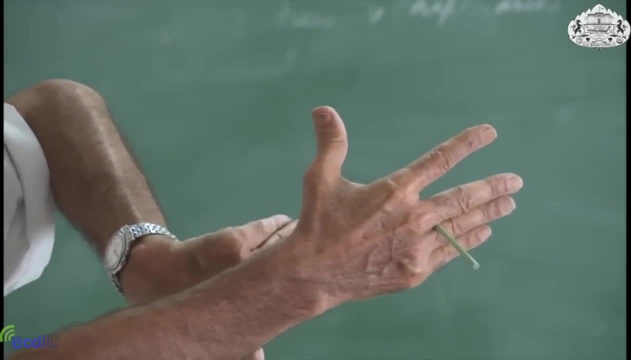 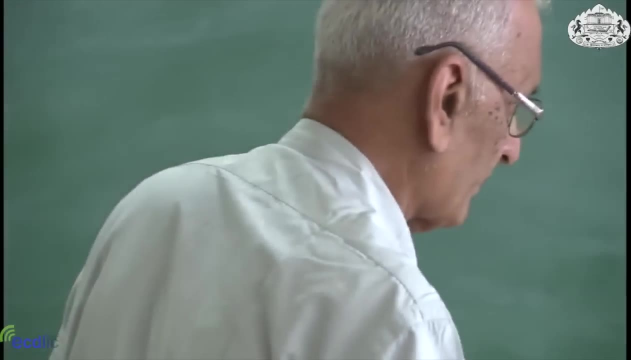 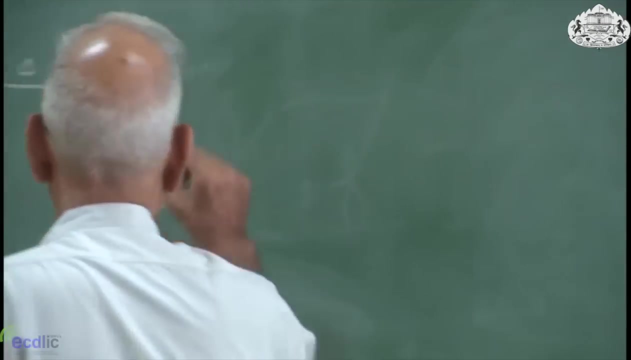 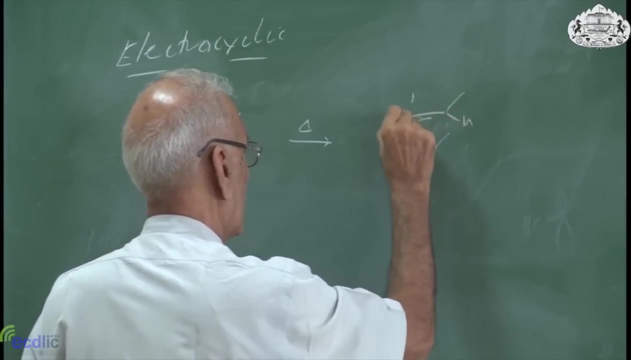 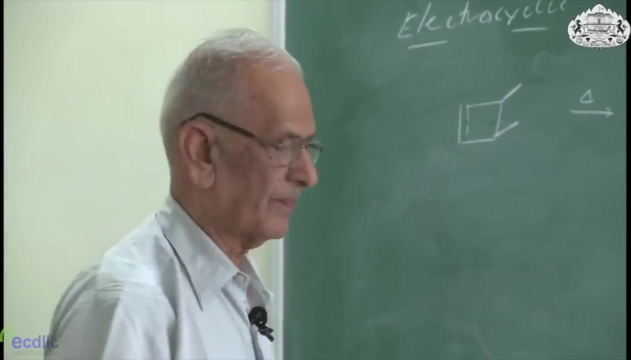 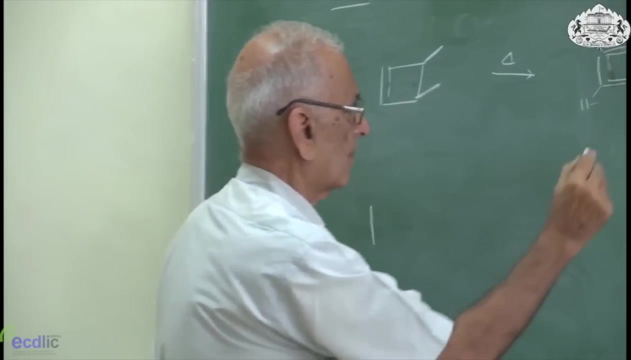 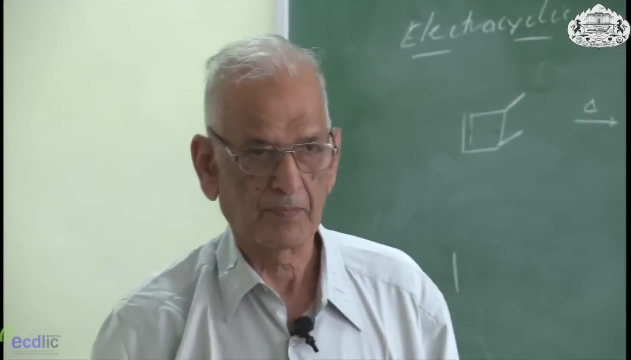 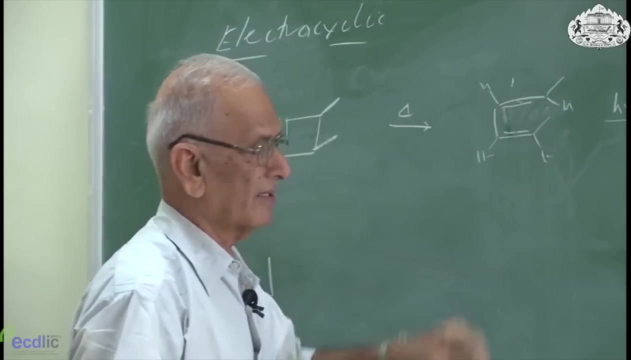 So clockwise, clockwise. So what will happen? One methyl group will be outside, one methyl group will be inside. One double bond trans, one double bond cis. How many electrons involved? 2 electrons, So it is a 2 electrons here. 2 electrons. 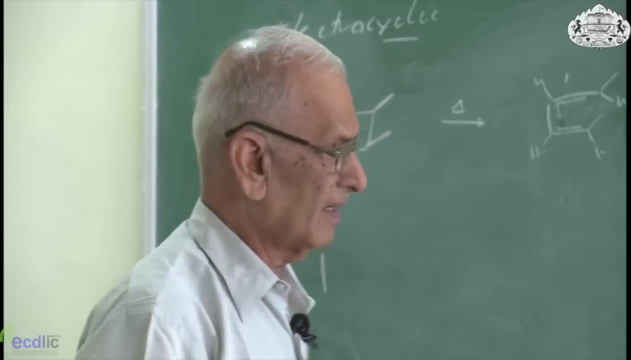 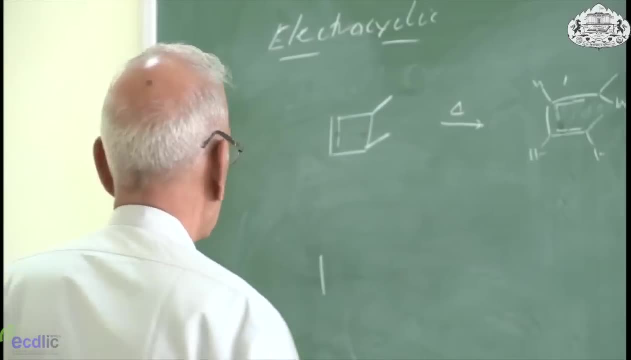 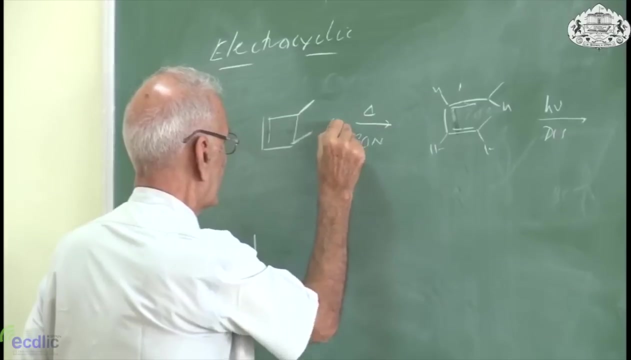 here. So it is a 4 electron system. All right, 4 electron system. What does our rule tell us? The photochemical reaction is going to be dis-rotated. 4 electron thermal reaction, 4 electron photochemical reaction is going. 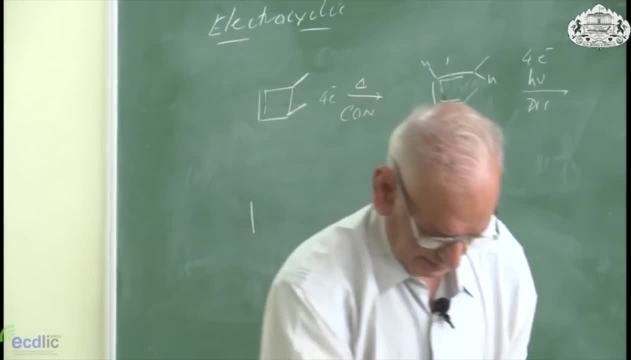 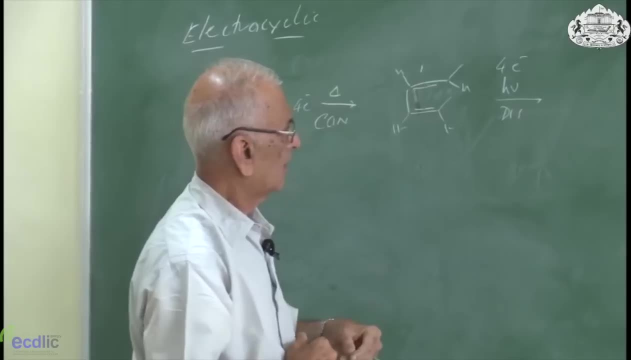 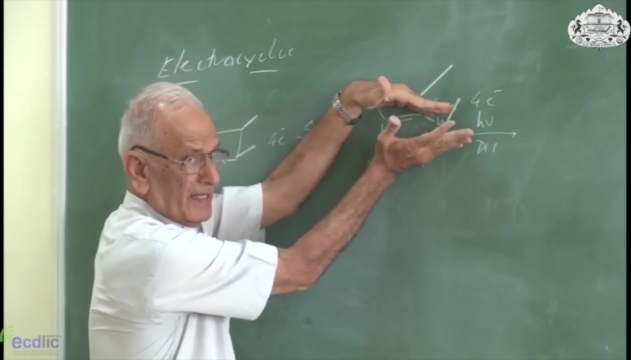 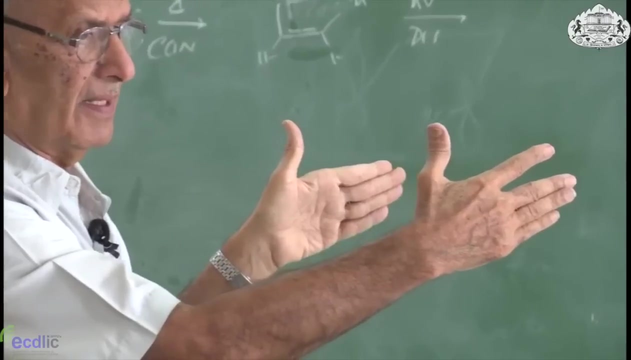 to be dis-rotated, All right. So how are we going to look at this? One methyl group is outside and this methyl group is inside. That is the picture that you have Now. dis-rotated means thumb should move in. 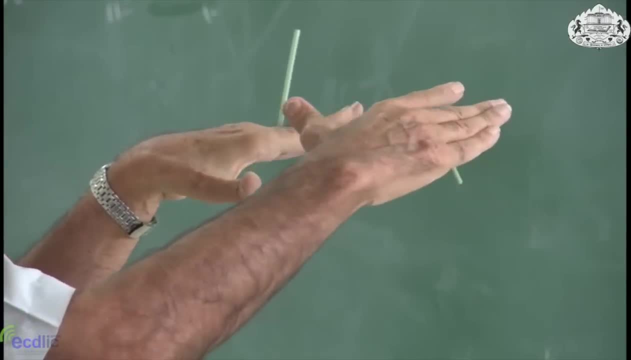 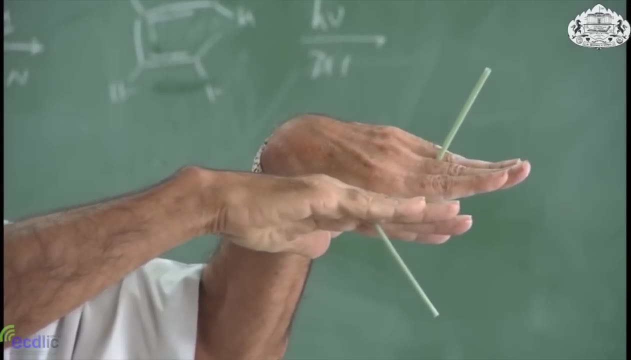 opposite direction. So this is moving clockwise, This will move anticlockwise, So your product will have one methyl group up, one methyl group down. So this is the picture that you have. If I do the opposite, result will be this one is down, this one is up, but n result. 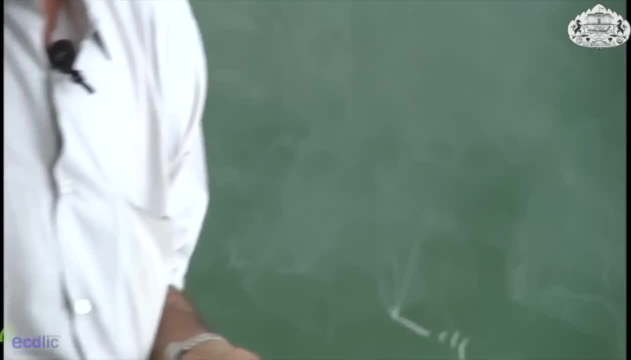 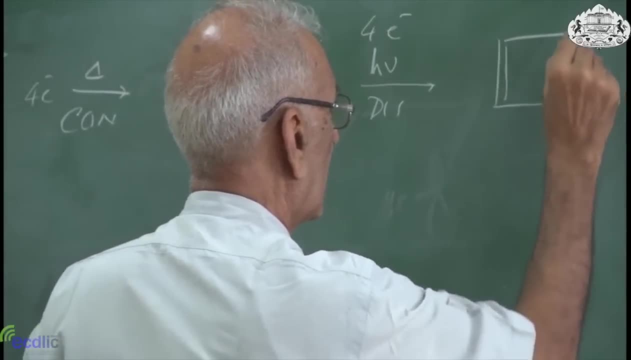 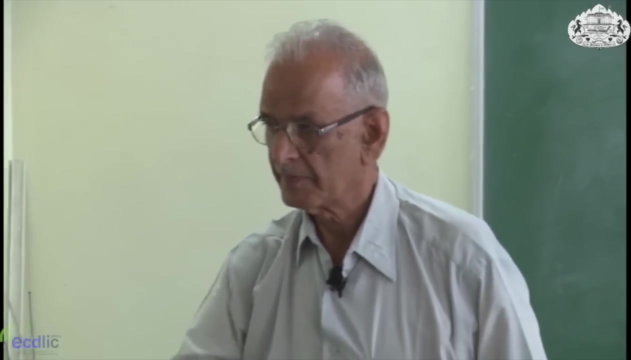 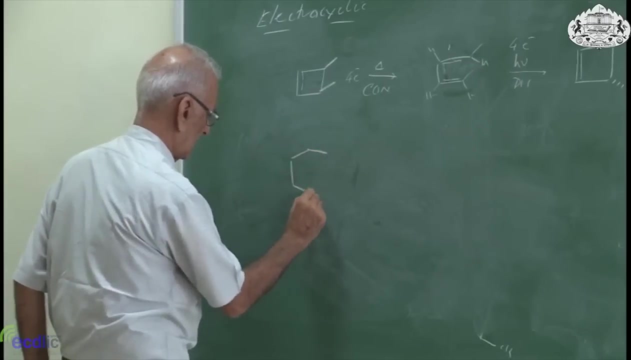 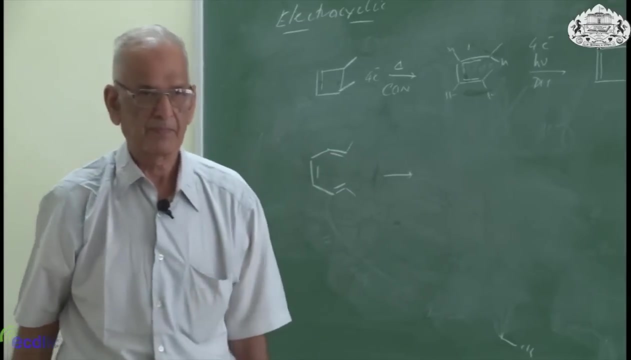 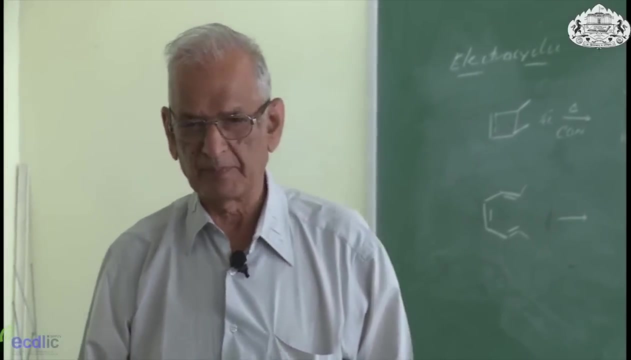 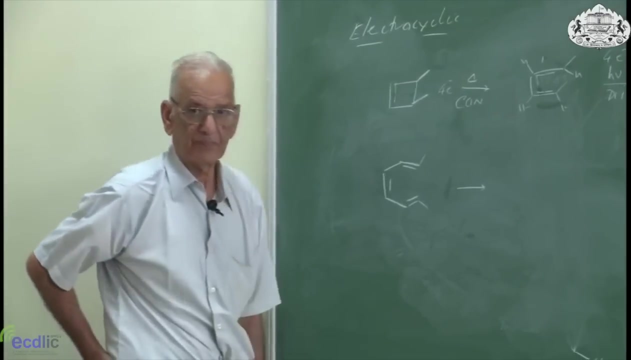 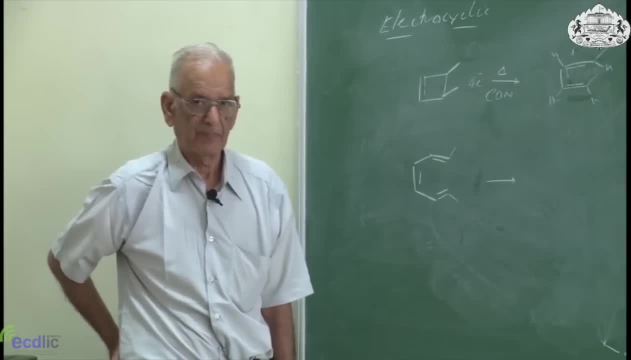 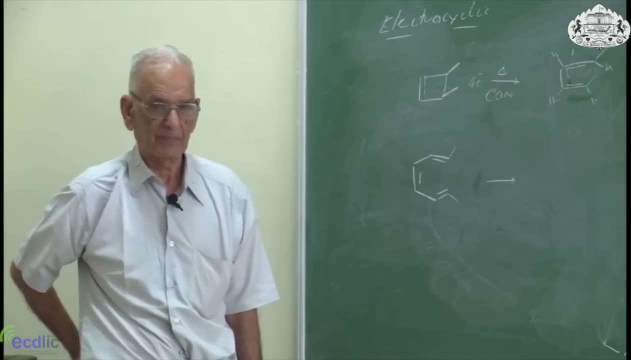 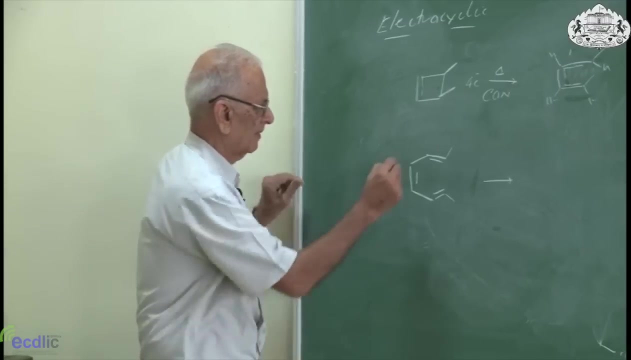 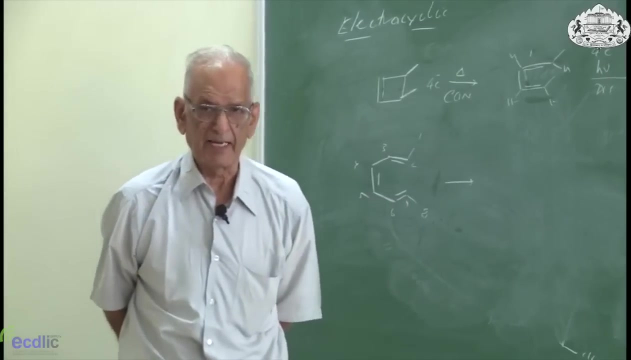 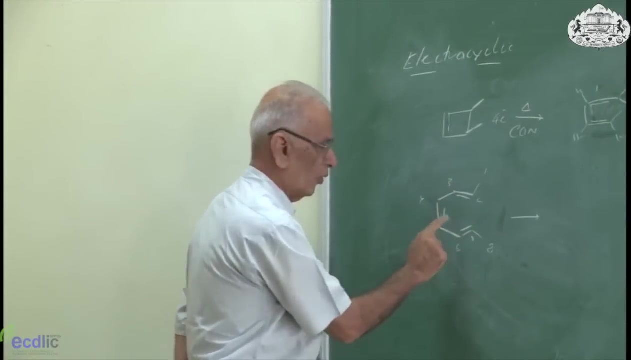 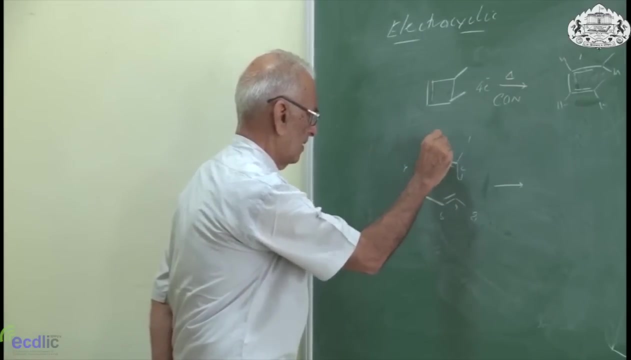 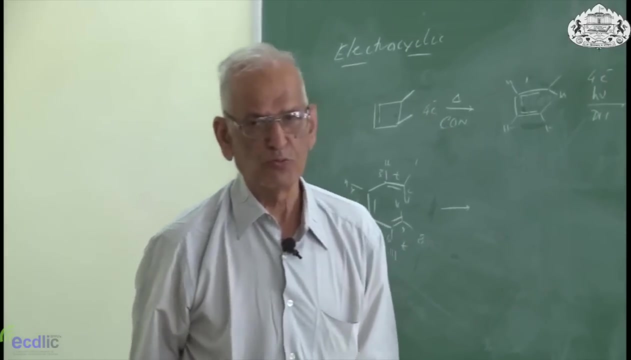 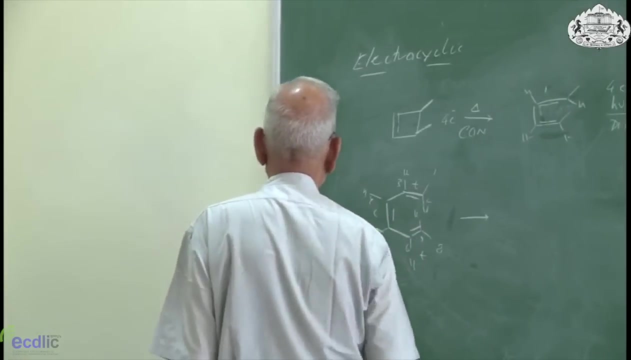 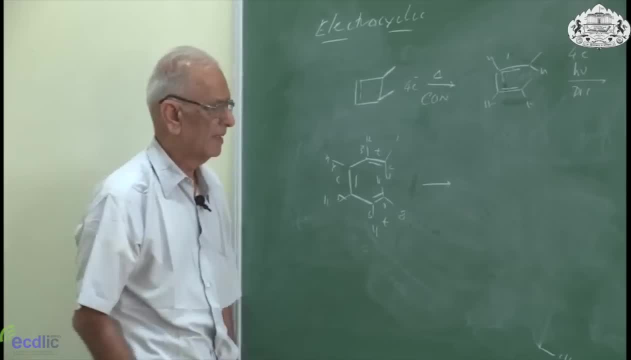 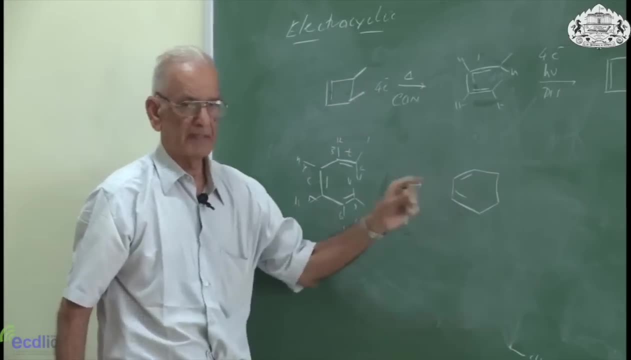 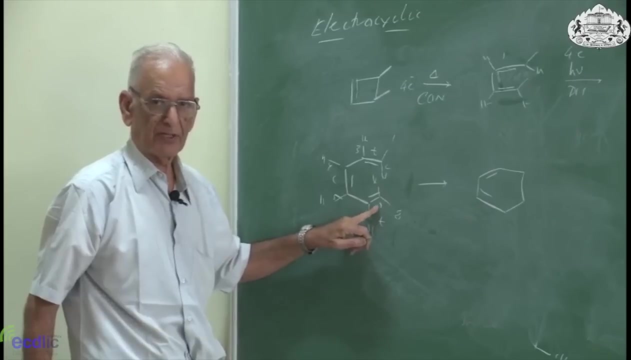 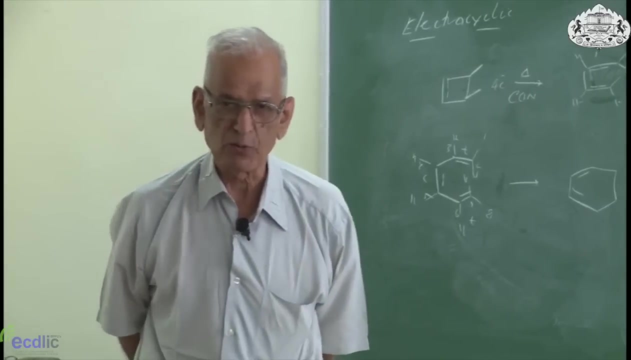 tri. That is essentially a double bond. The product is cyclic with two double bonds. How many electrons? 6 pi electrons or 3 pi bonds. product gives 2 pi bonds. so it is a electro cyclic reaction: N pi going to N minus 1 pi. 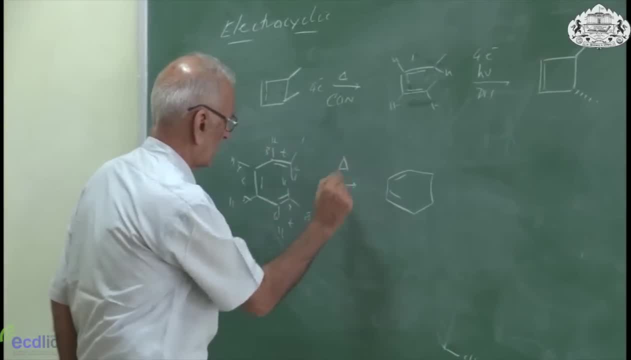 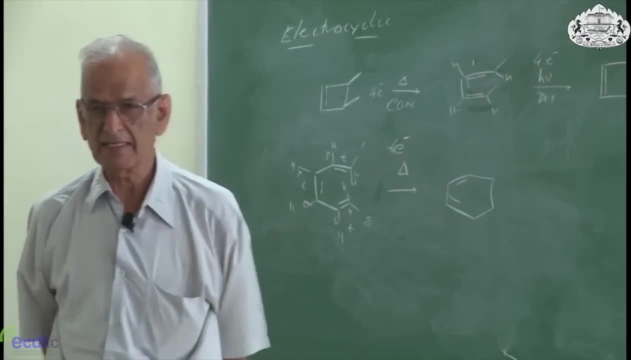 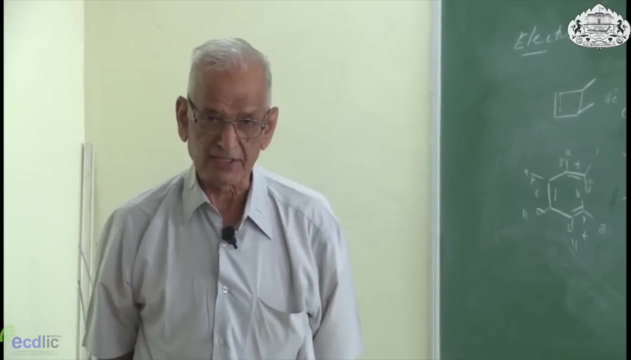 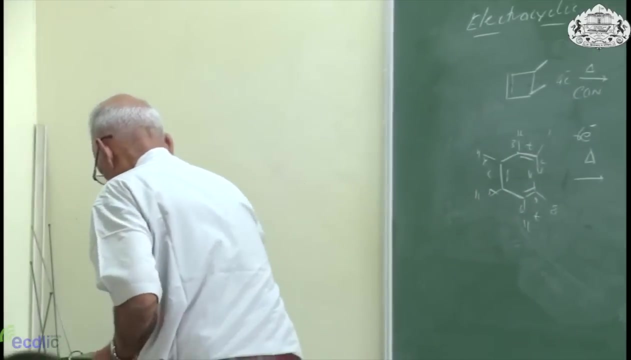 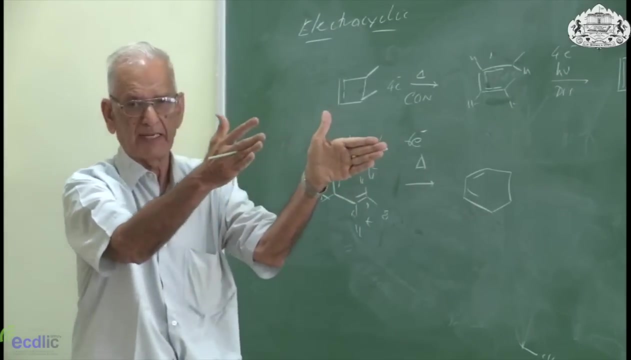 Alright, Now six: electron thermal reaction. what does our rule tell us? Six electron thermal reaction is going to be dis-rotatory. So how are my methyl groups? One methyl? both the methyl groups are outside. Dis-rotatory means thumb should move in opposite direction. This is 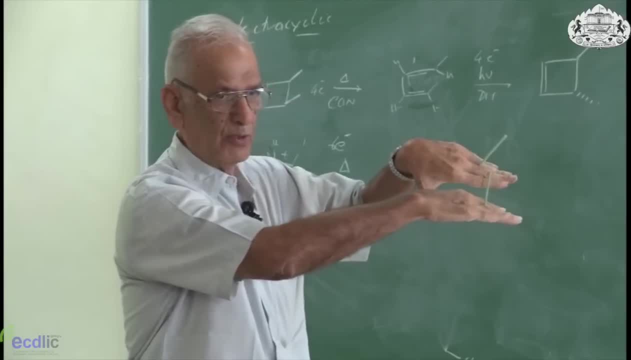 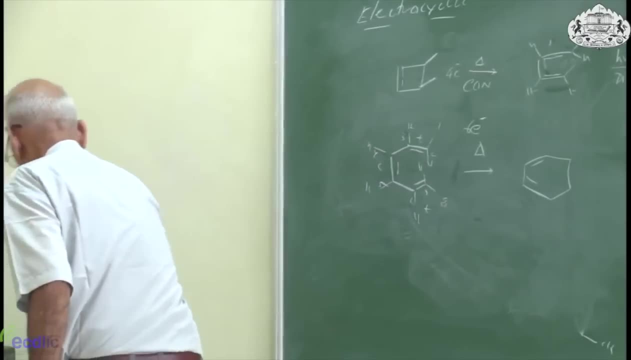 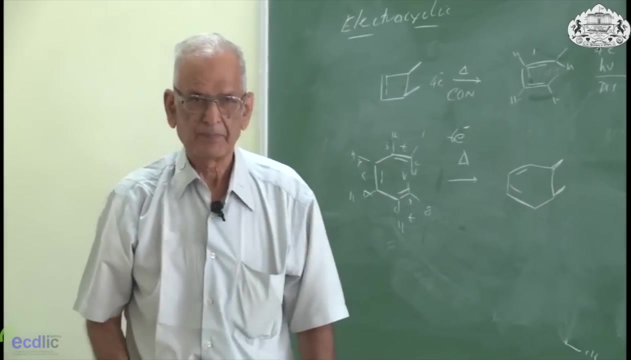 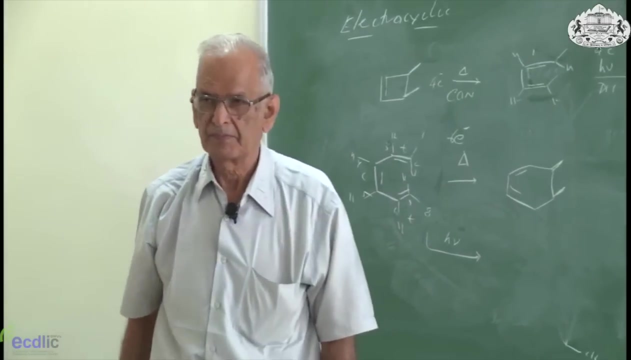 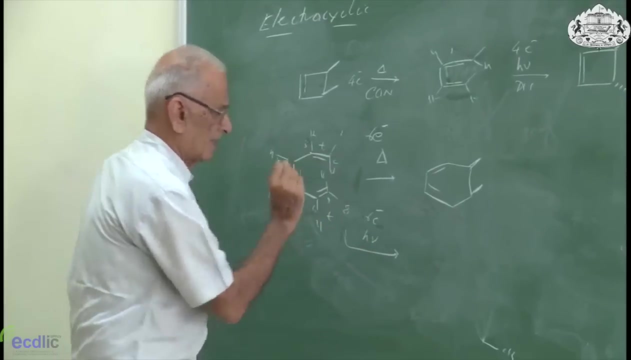 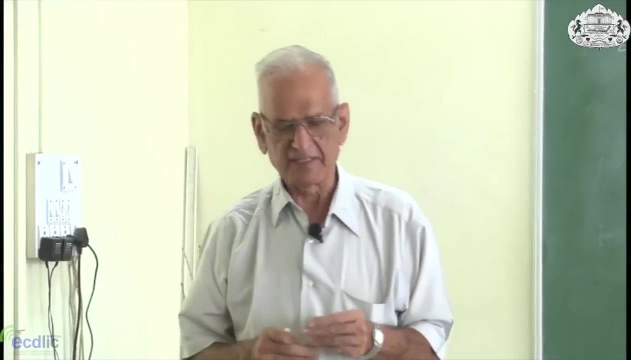 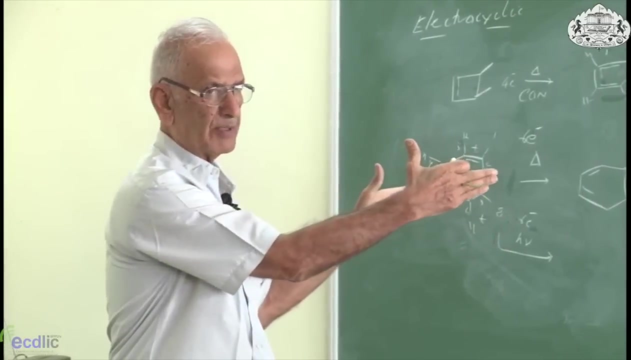 clockwise. this is anti-clockwise. So product is going to be cis. Okay, Six electron photochemical reaction. It must be conroutine, Conroutine, Conrotatory, correct. So your two methyl groups are outside. Conrotatory means thumbs. 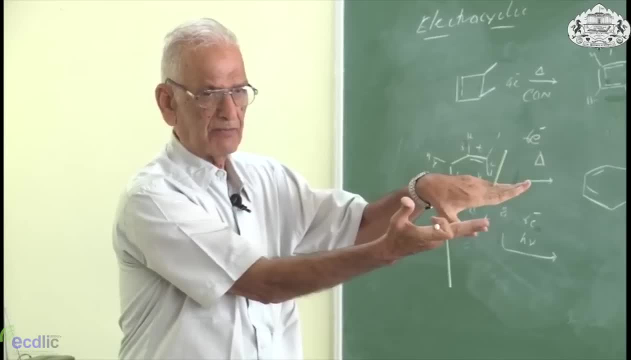 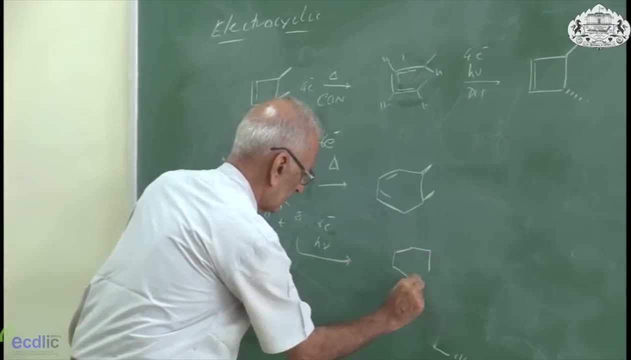 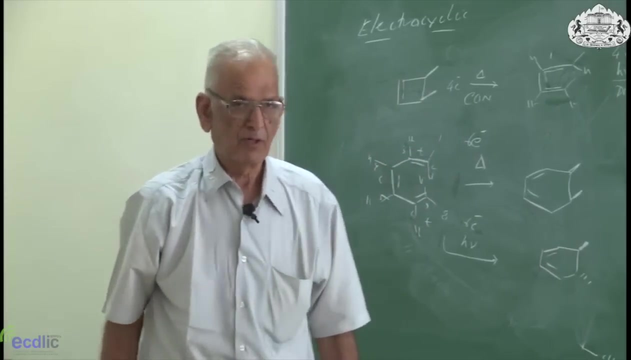 must move in the same direction. So one product will be one methyl group will be above, one methyl group will be below. What are we seeing? Thermal reaction has given. So this is the conrotatory- Conrotatory. 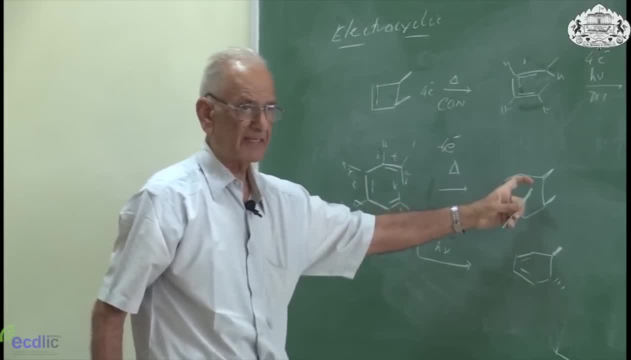 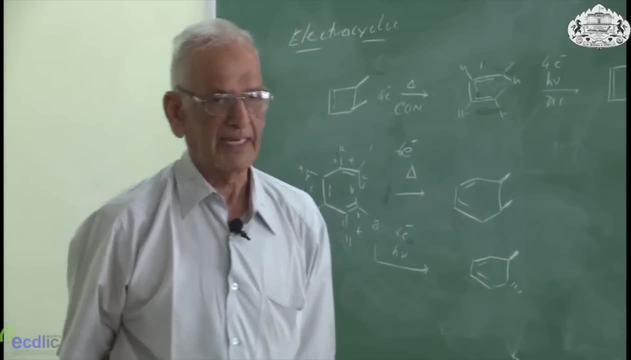 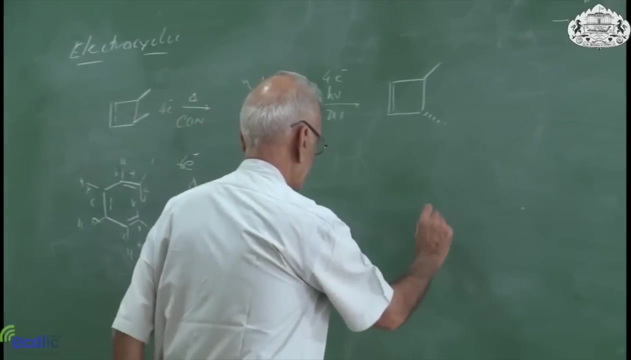 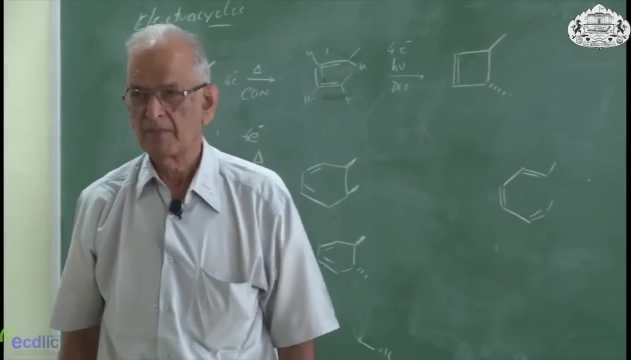 Conrotatory, Conrotatory Whether the Henkel reaction has given cis product". Yes, Photochemical reaction has given transics product. So when I do with photochemistry I get different results. What will I call this compound? 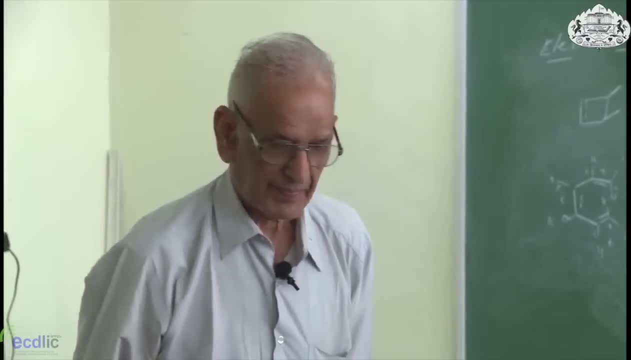 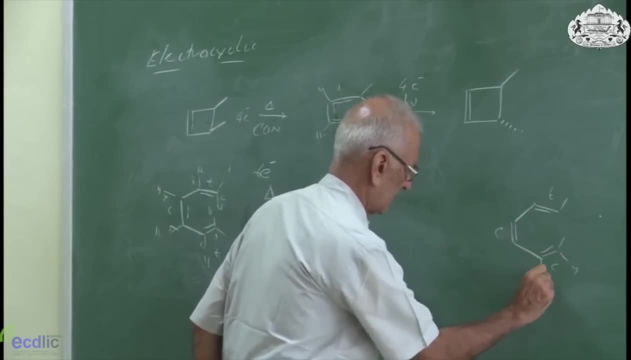 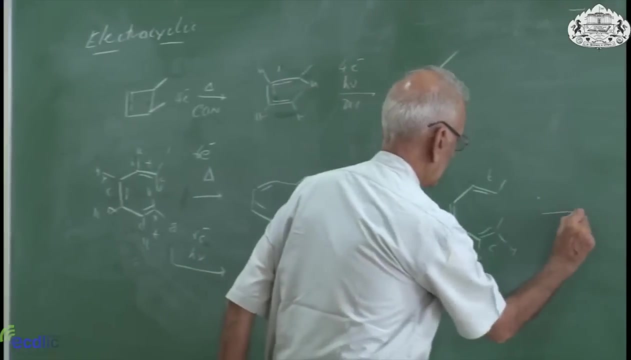 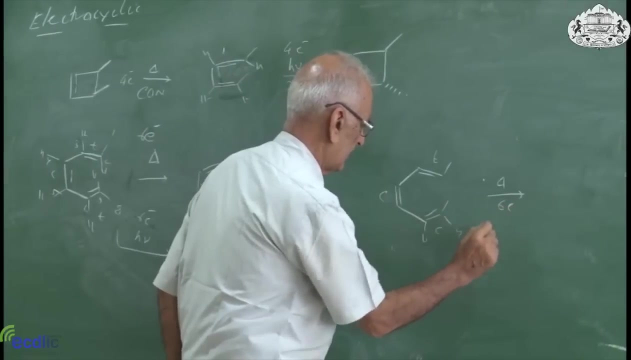 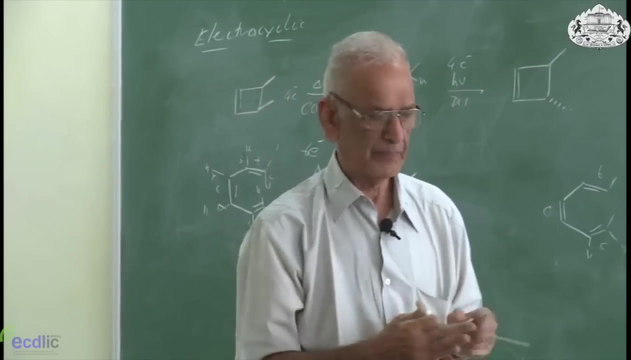 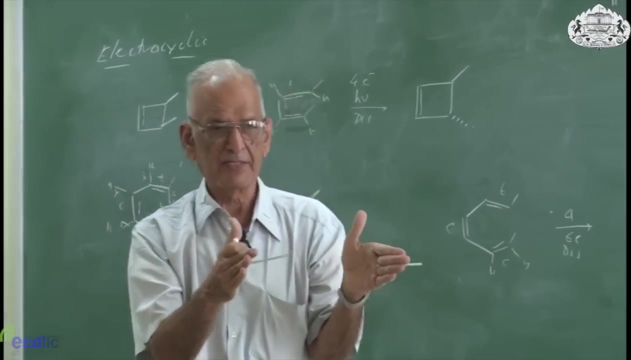 Bp, Bp, Trans, cis, cis, all right. Thermal reaction: 6 electrons: 6 electron thermal reaction is going to be dis-rotate. So one metal group is outside, one metal group is inside- Dis-rotate. 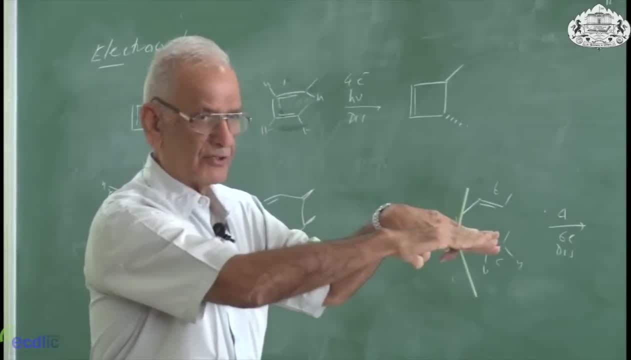 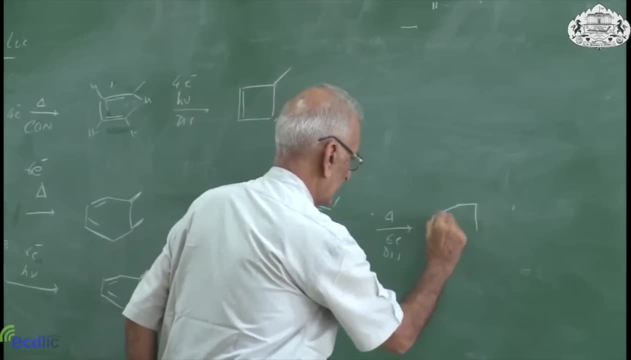 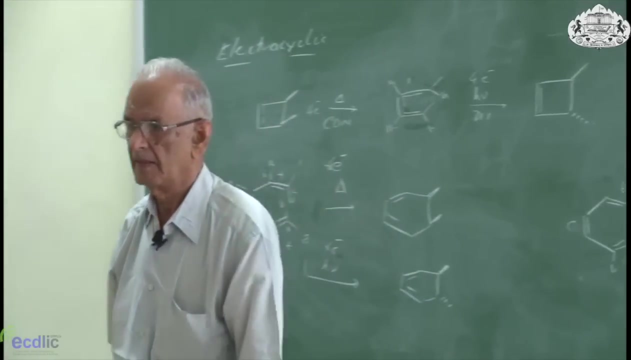 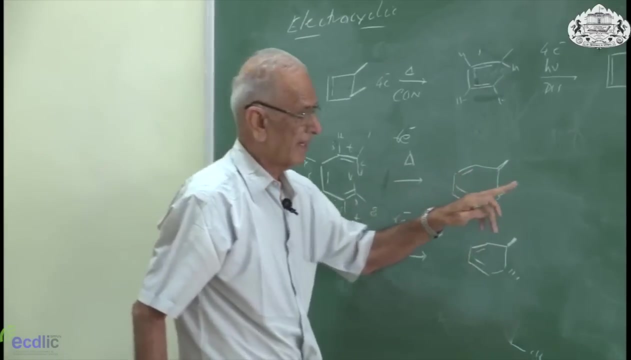 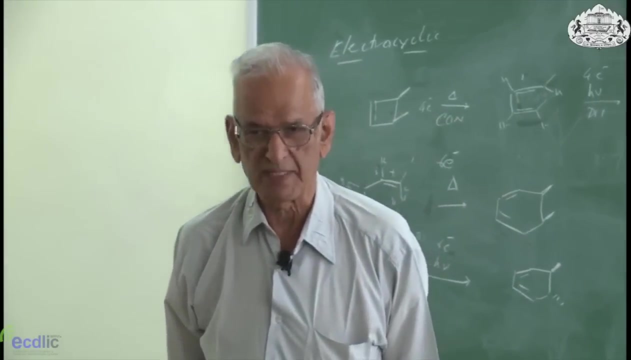 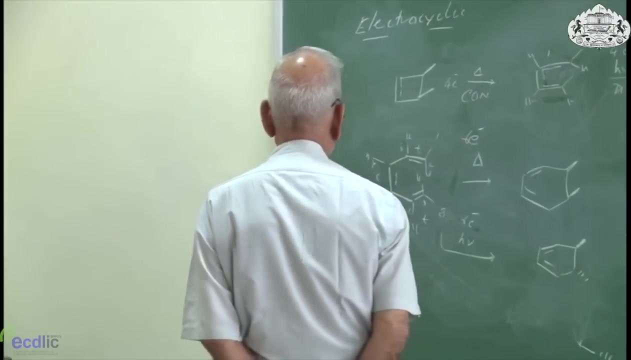 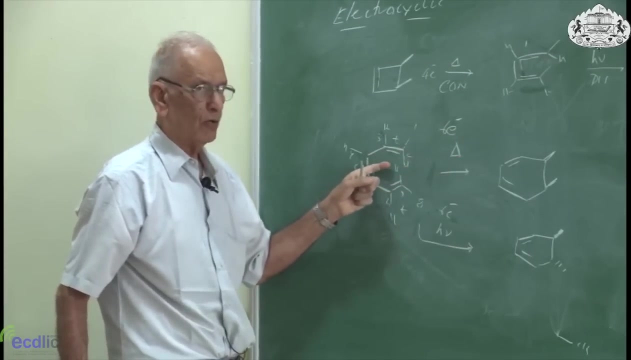 means thumbs must move in opposite direction, So product will be one metal group up, one metal group down. Isomer A gave me product B. Isomer A- dash- gave me product B- dash. Reaction is stereospecific. Now we have the next question In this reaction. what happened? Open chain compound gave me. 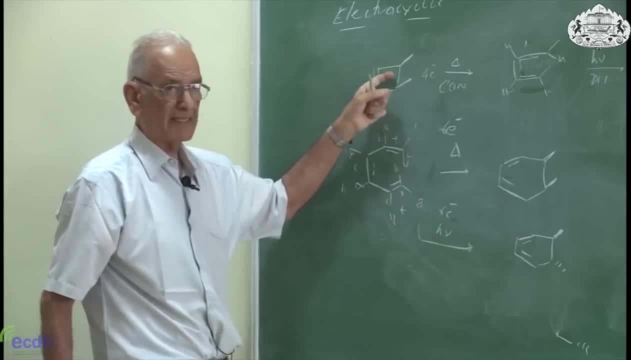 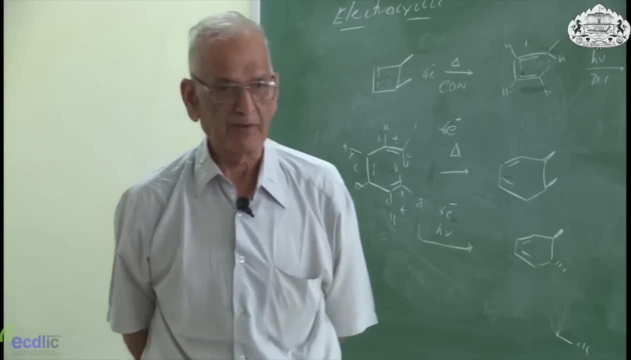 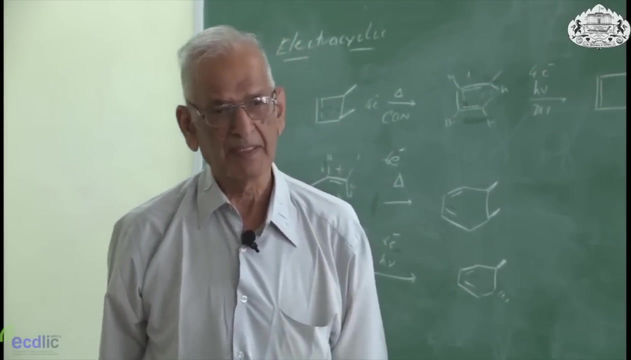 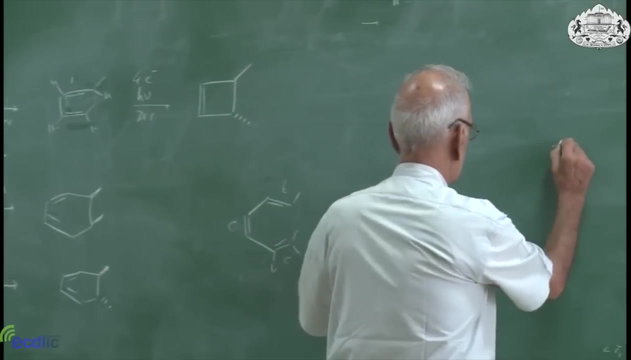 cyclic product. In this reaction, what happened? Cyclic product gave me open chain product. So in one case we went from open chain to cyclic. In the other one we went from cyclic to open chain. In a thermal reaction, you always go from laser to open chain. 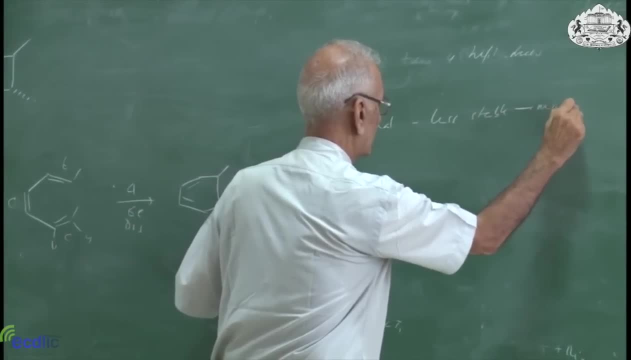 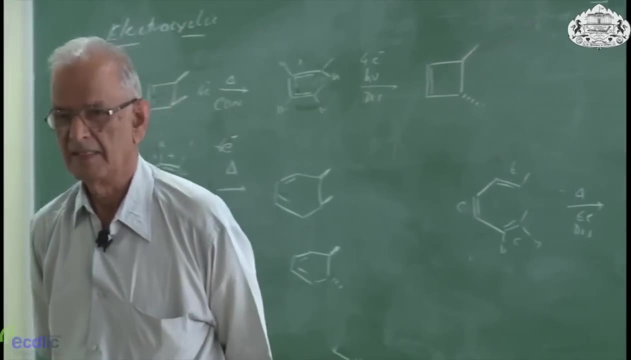 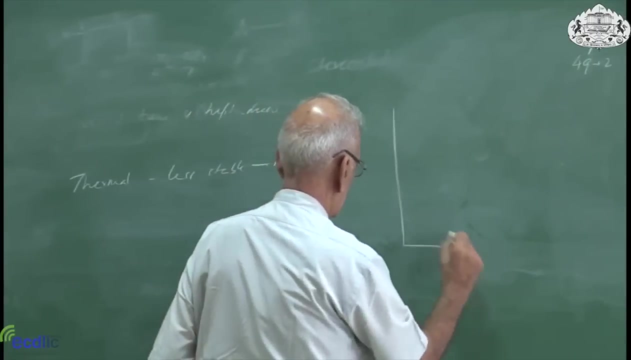 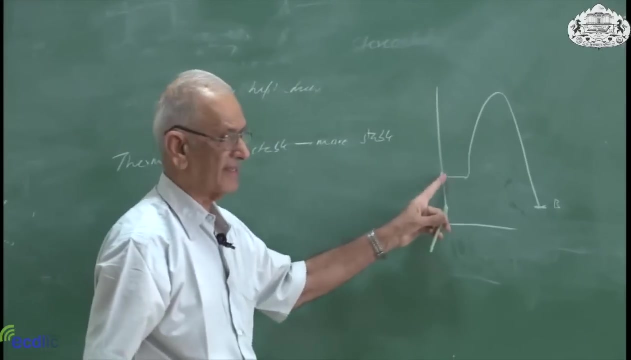 Less stable to more stable. All right, So this is your A. A goes to B, Less stable goes to more stable. What do we say For such a reaction? we say: less stable to more stable, Less stable to more stable. 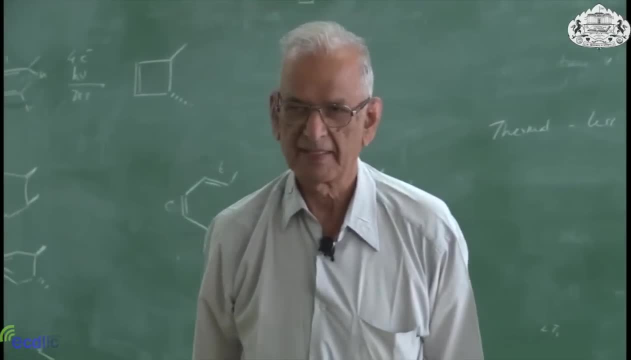 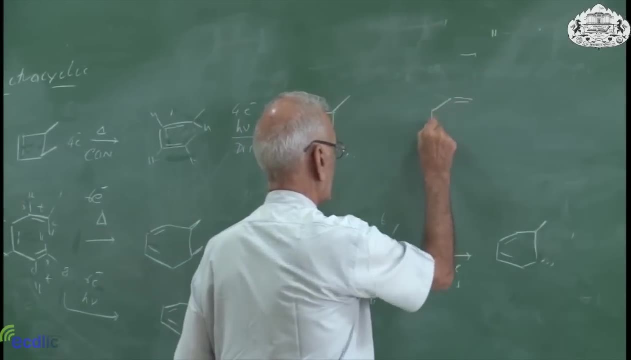 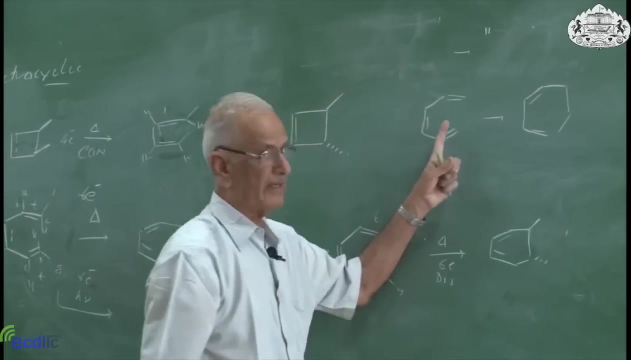 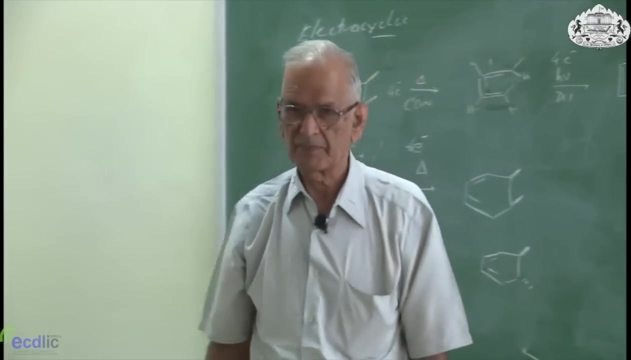 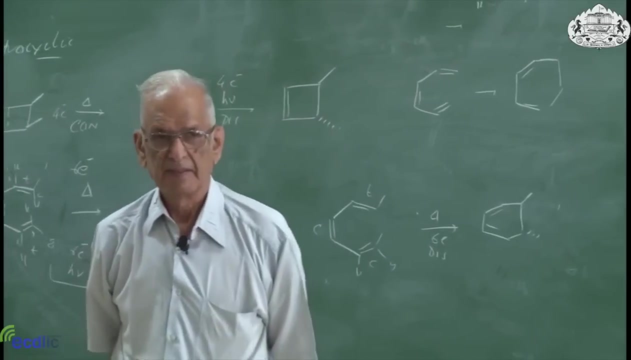 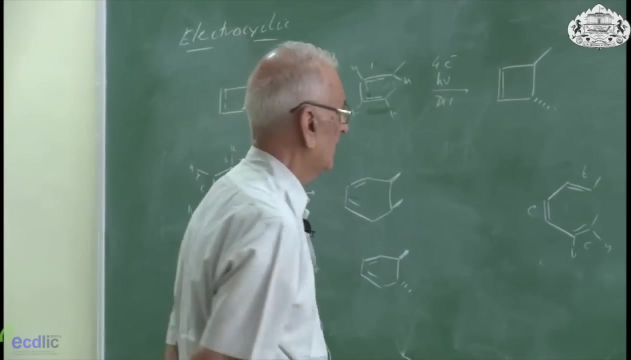 The reaction is exothermic. So we have to answer this question: Why are we going from this to this Open chain to cyclic? How many sigma bonds are there in this? Every double bond is made up of a sigma bond and a pi bond, So 1,, 2,, 3,, 4, 5 sigma bonds. 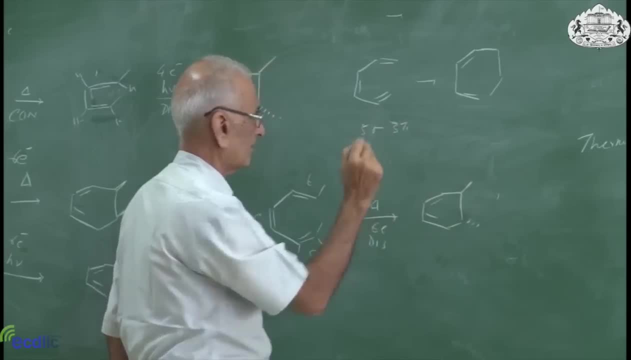 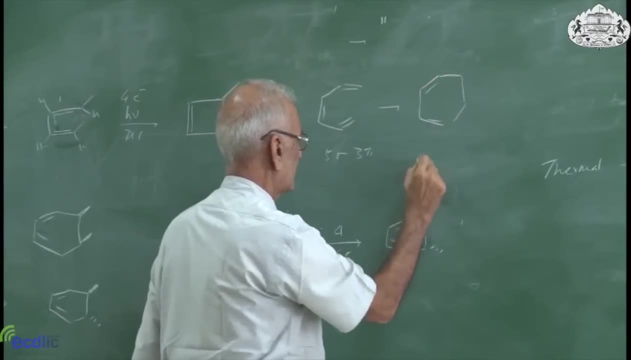 and 1,, 2,, 3, 5 bonds In my product: 1,, 2,, 3,, 4,, 5, 6 sigma bonds and 2 pi bonds. So this is my product. This is my product. 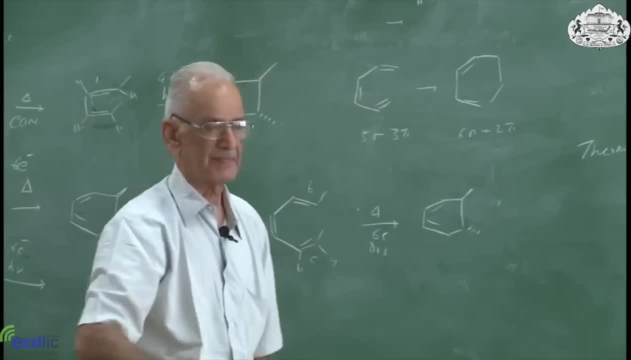 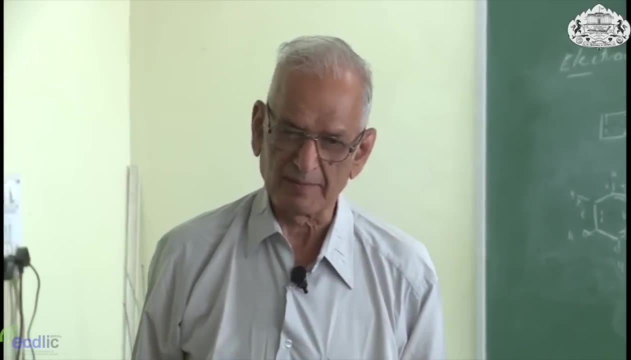 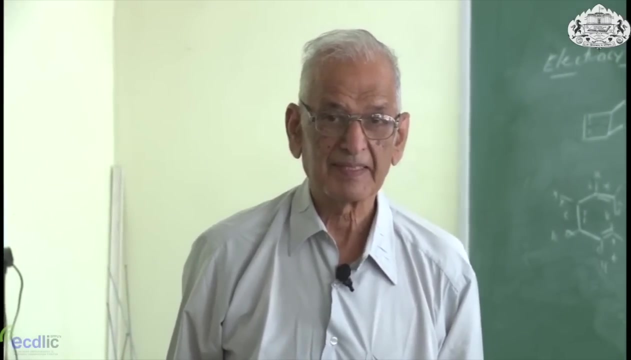 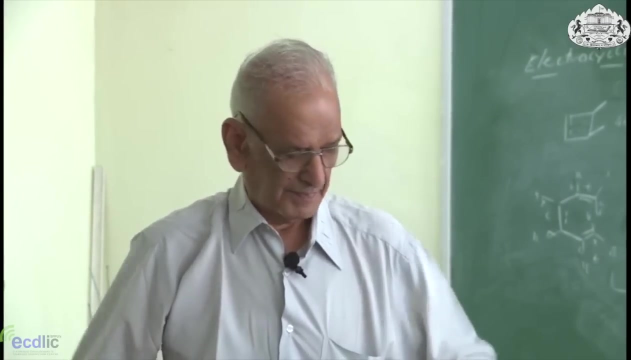 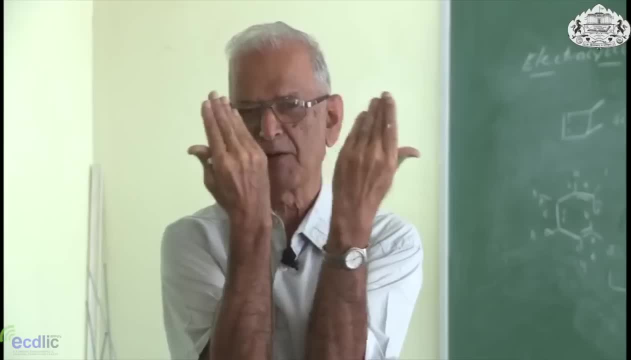 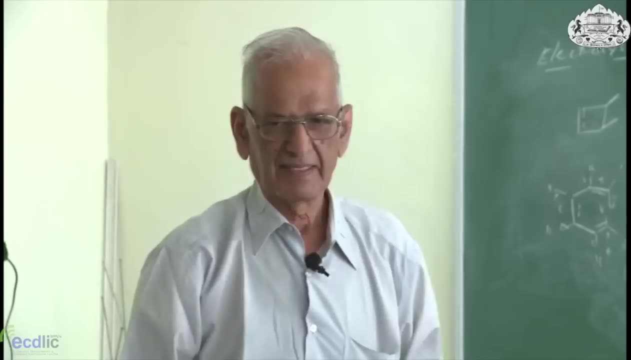 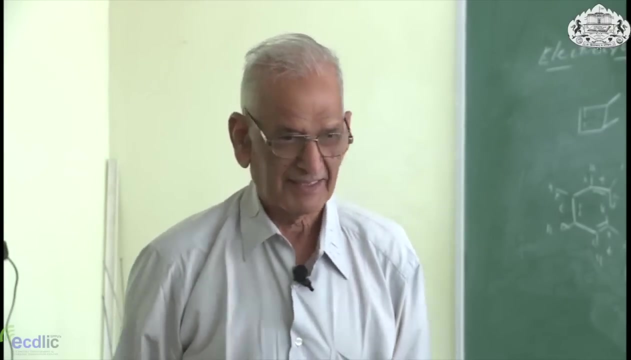 this Overlap is head on. bond is formed by lateral overlap. this is head on overlap, To which you say: you look at the compound, can you see like this, like this, all this? I do not believe it. So how? 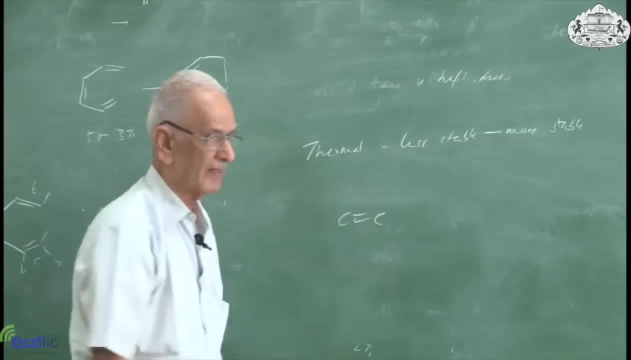 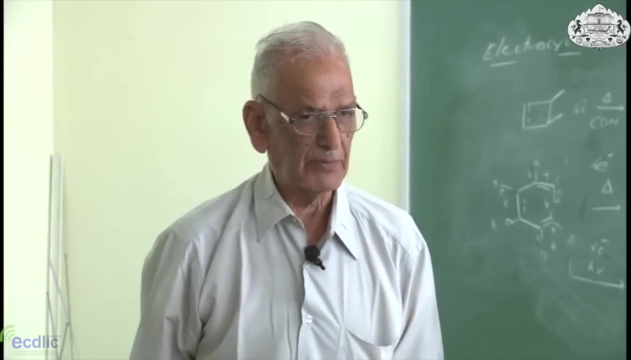 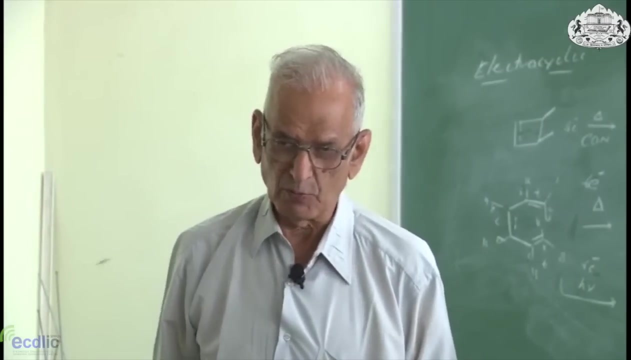 do you find out? I measure the heat of combustion. what do I mean heat of combustion? I take such a compound, burn it in the presence of oxygen. it will become carbon dioxide, hydrogen will become water. I measure that heat of combustion and from this I find carbon carbon. 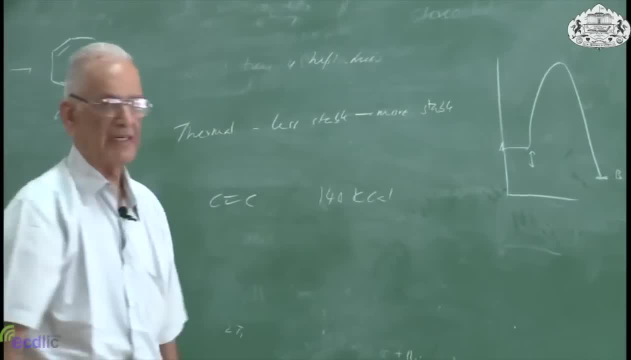 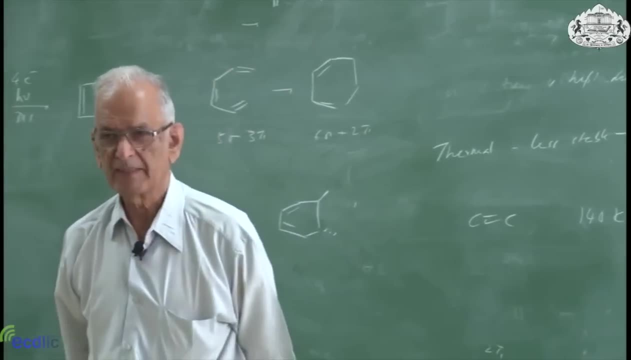 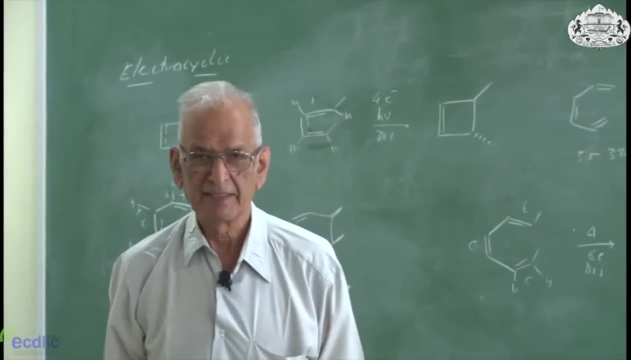 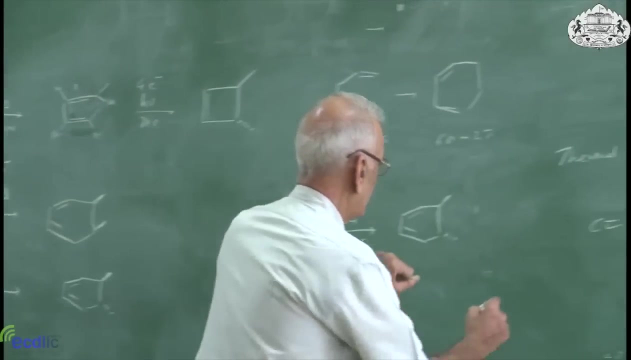 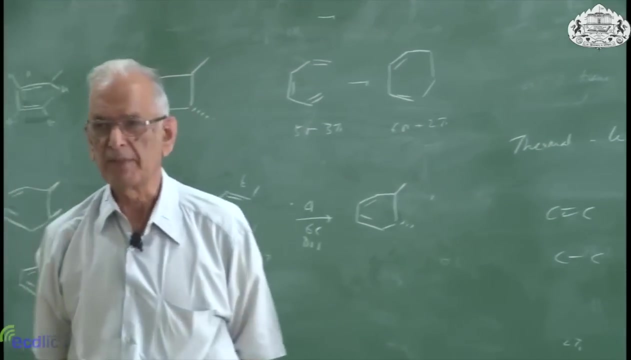 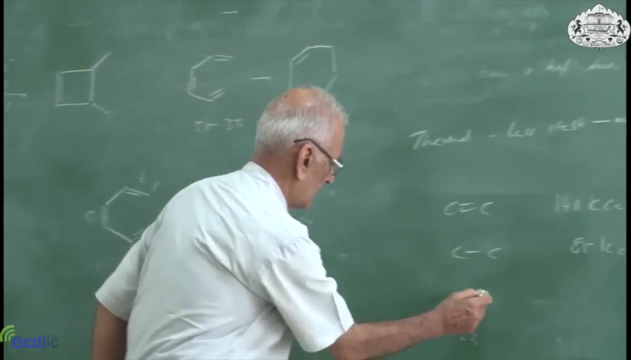 bond 140 kilo gallons. Take ethylene, burn it, you will get two molecules of carbon dioxide, two molecules of water. Take ethane, burn it, you will get two molecules of carbon dioxide, three molecules of water. and from this, energy of the carbon, carbon bond is 85 kilo. What is the energy of the? 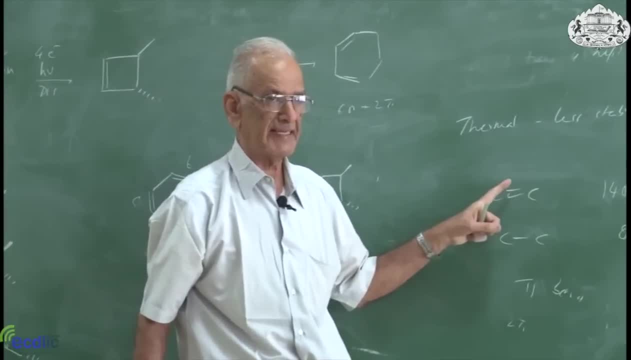 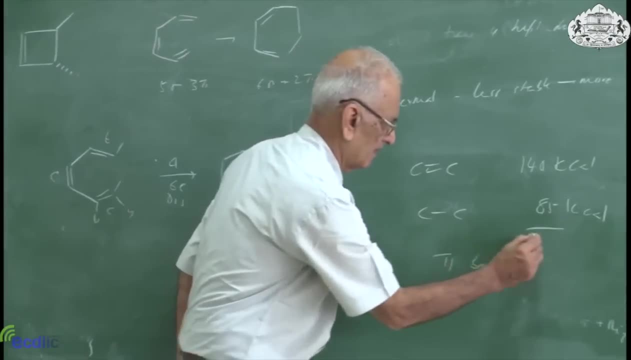 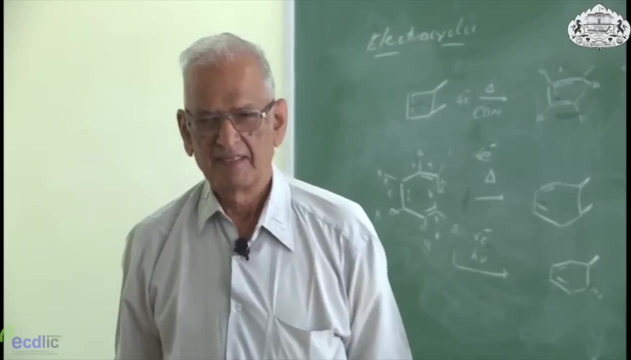 pi bond Sigma 1 pi and this is 1 sigma. So this minus this is the energy of pi bond. So pi bond has an energy of 55 kilo. So now we have experimental proof that pi bonds are less. 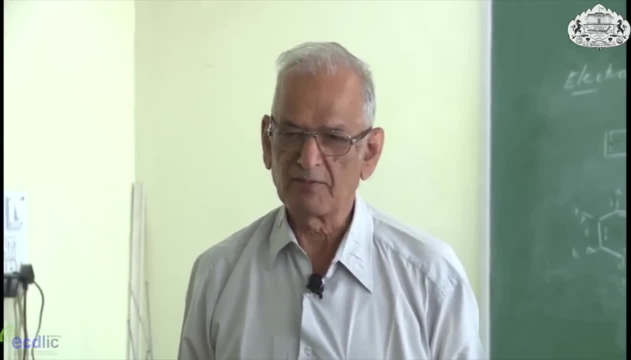 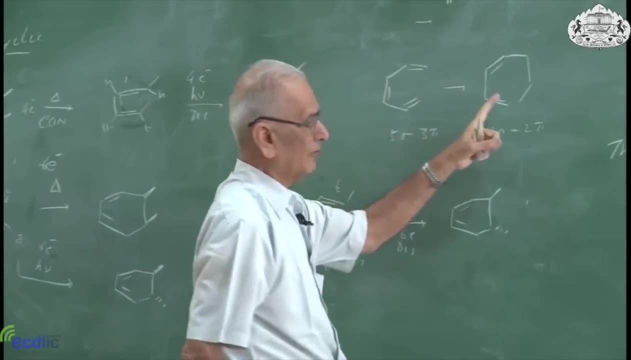 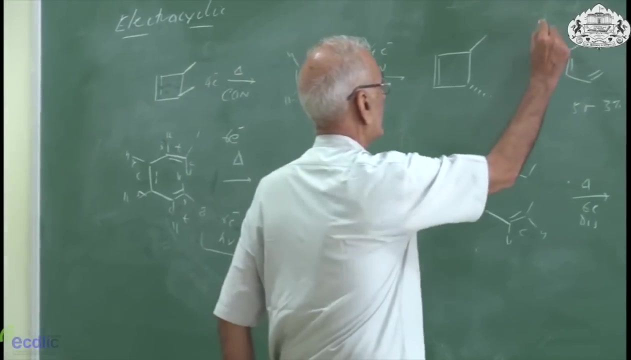 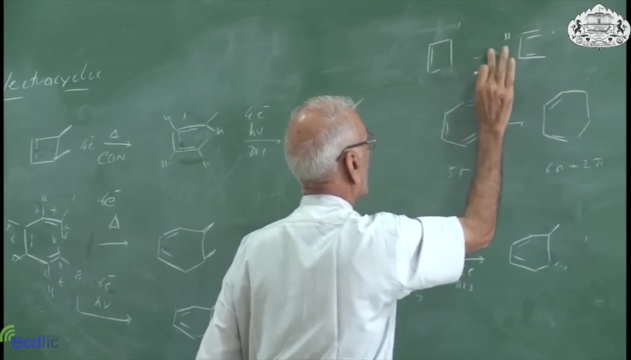 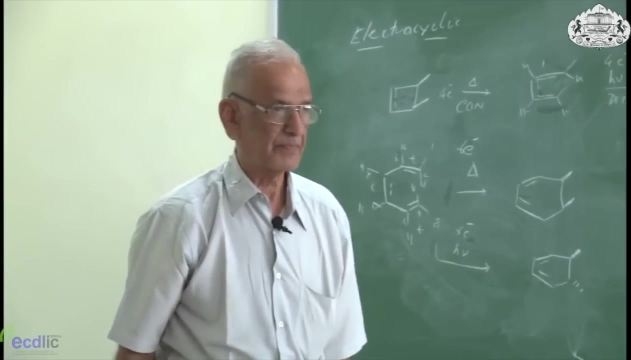 stable than sigma bond. So more sigma bond will be more favorable. So reaction going to be more favorable than sigma bond is expected. Now we look at this. How many sigma bonds are there in this starting material? 1,, 2,. 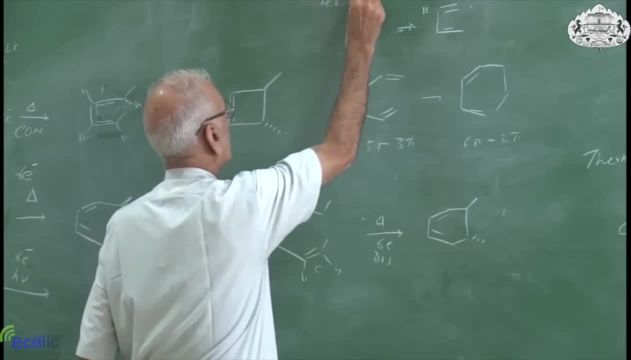 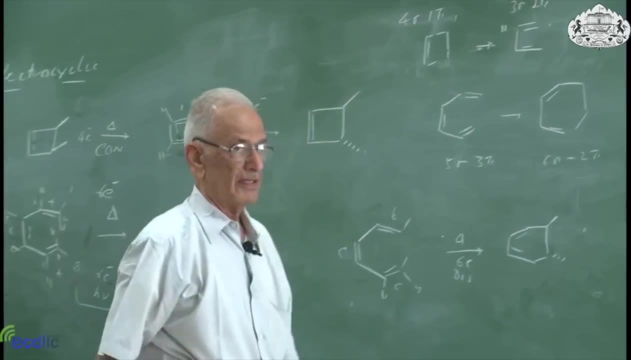 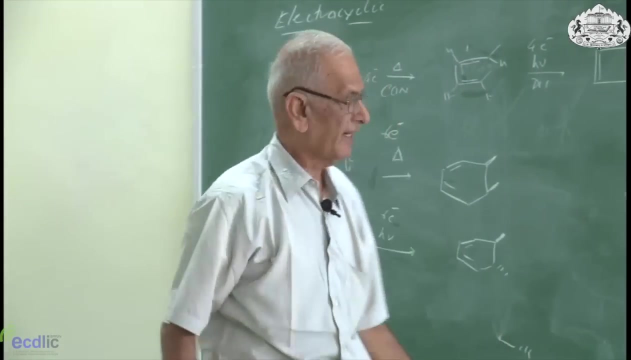 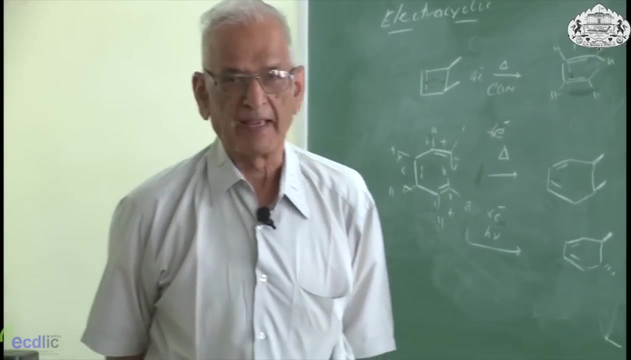 3, 4.. 4 sigma 1 pi. 1, 2, 3, 3 sigma 2 pi. So, according to what we just said, this should be more stable than this. but when we do, the reaction reaction goes from cyclic to open j, So why? 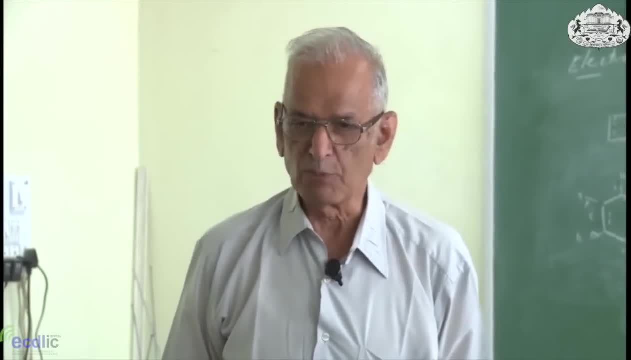 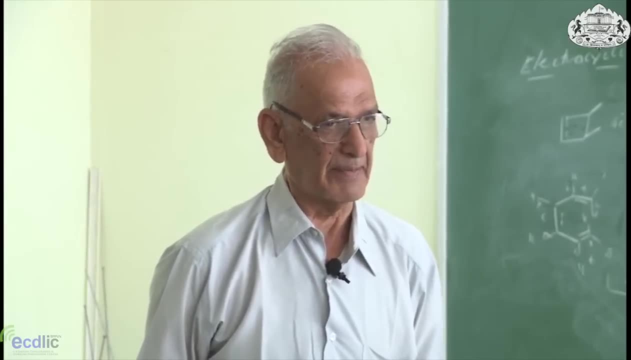 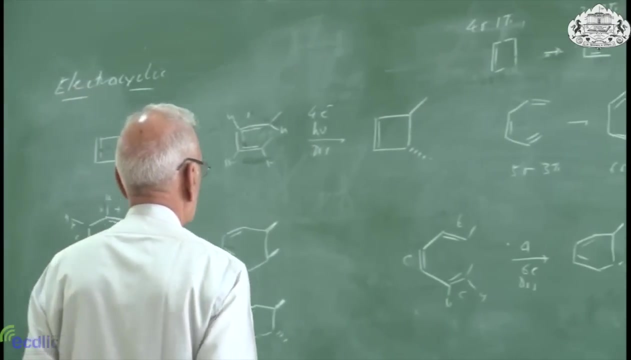 Two minutes ago for six-membered ring, we said cyclic is more stable. In this case we are saying for some reason cyclic compound is less stable. Angle strain is present in the four-membered ring. Very good, What is that angle strain If this four-membered ring? 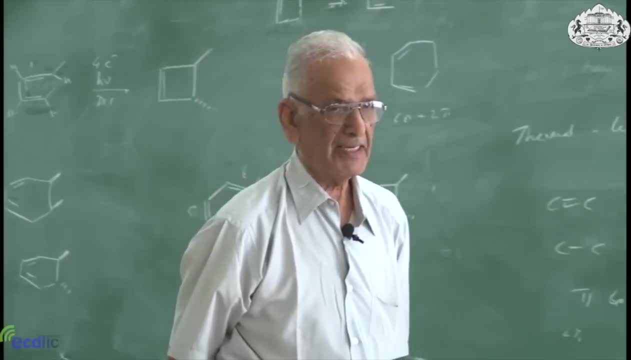 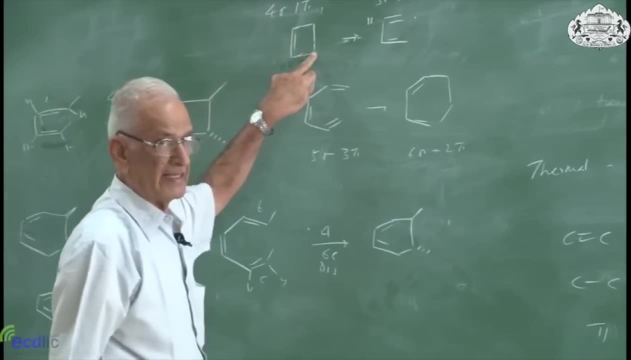 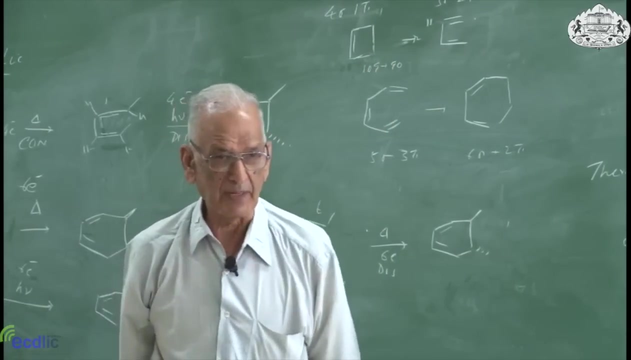 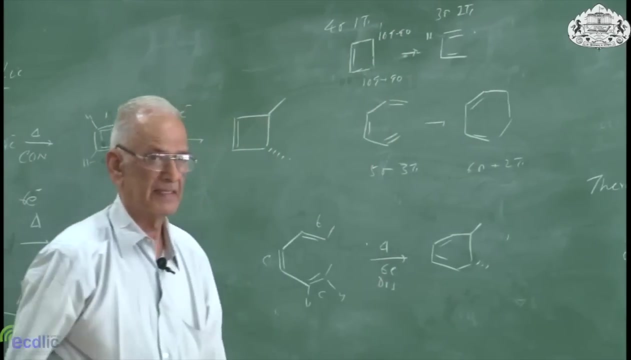 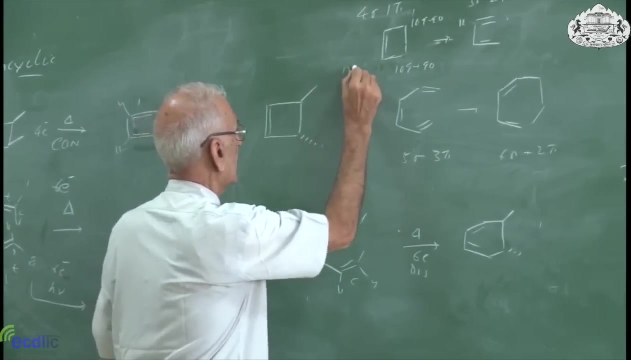 had to be planar. according to our geometry, all angles should be 90 degrees. What type of carbon is this? SP 3.. So 109 going to 90.. I am forgetting the 28.. 109 going to 90.. 109 going to 90.. What about this? This is an SP 2 carbon. So 120 going to 90.. 120. going to 90.. 109 going to 90.. So how much angle strain? 30,, 30,, 60,, 60, plus 38,, 98 degrees of strain. So, though, more sigma is more stable because of that, 98 degrees of angle strain, the four-membered 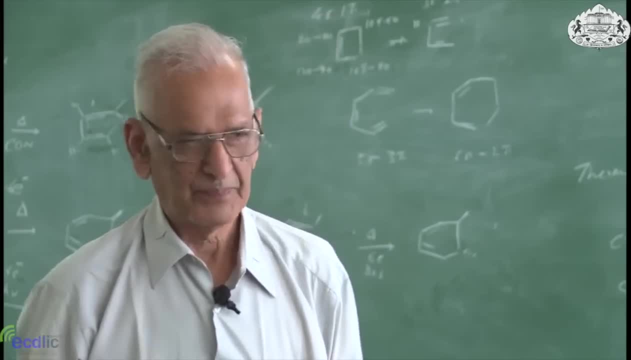 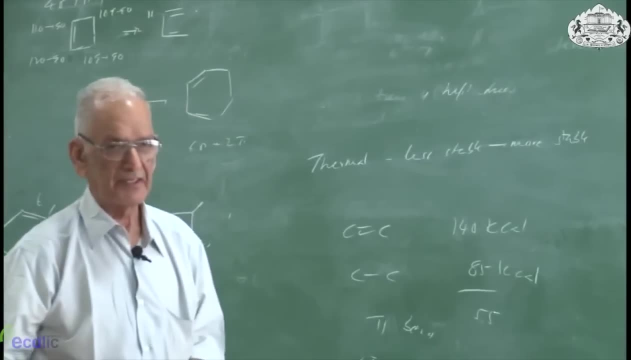 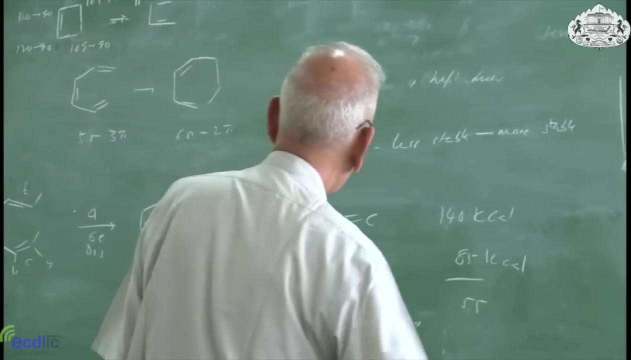 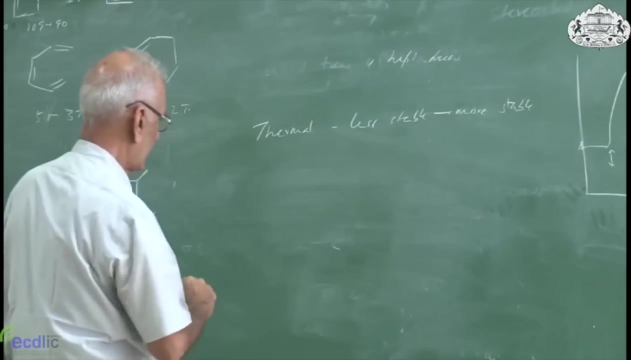 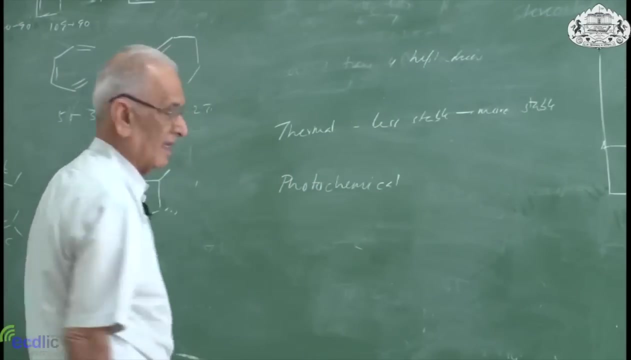 ring is unstable. We have learnt this very important principle. In a thermal reaction, you always go from less stable to more stable. Now what is our problem? In photochemical, we have a very important principle: We have to know the temperature. 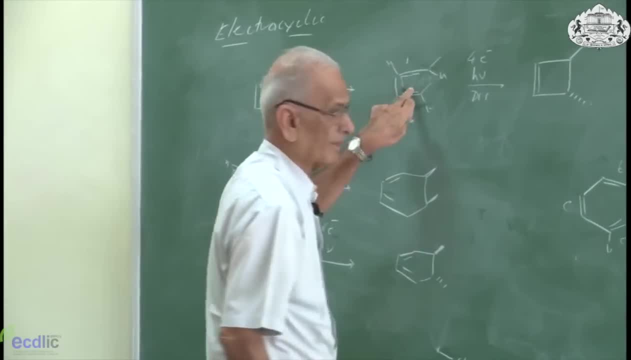 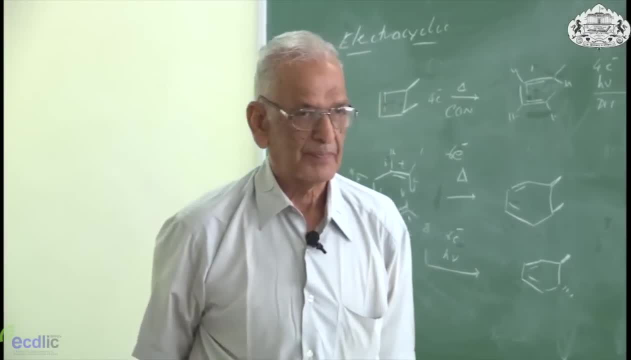 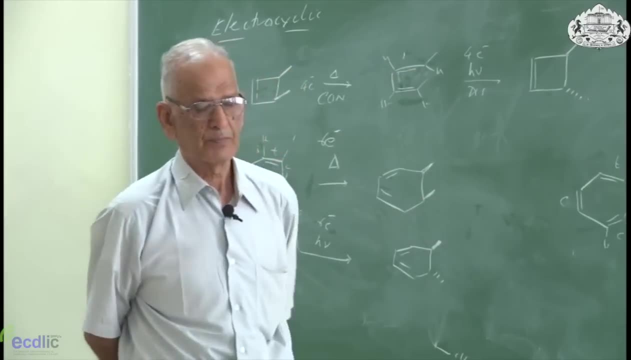 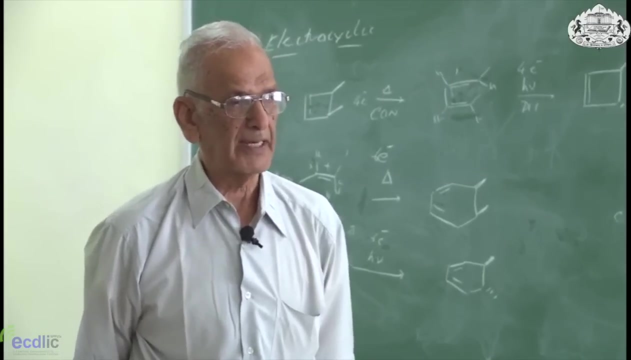 What is the principle in photochemical reaction? What is the UV of butadiene 217.. What is the UV of ethylene 185.. So butadiene absorbs at longer wavelength. So when I do photochemistry, butadiene gets excited. 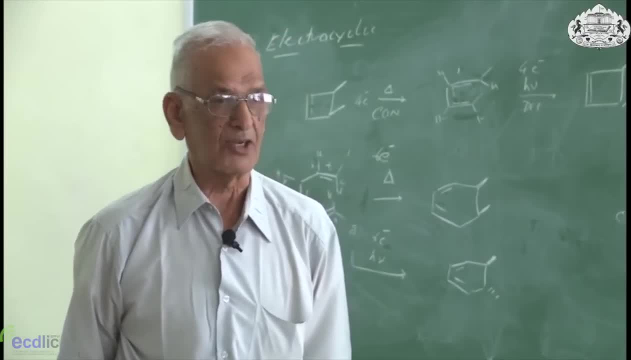 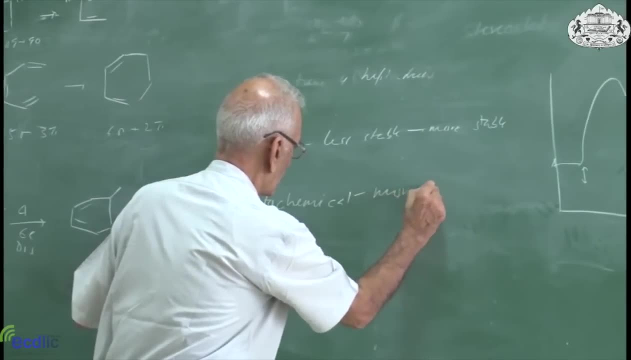 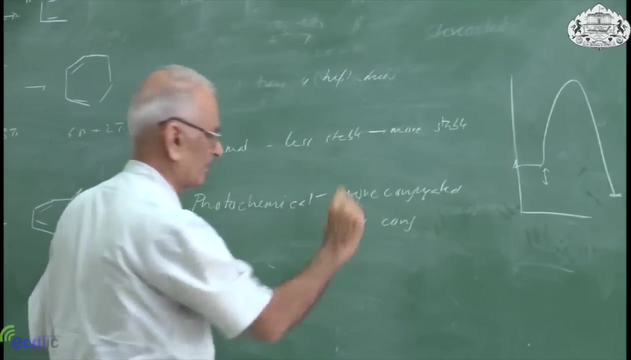 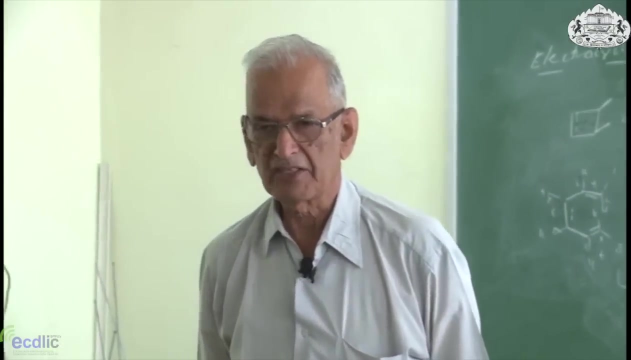 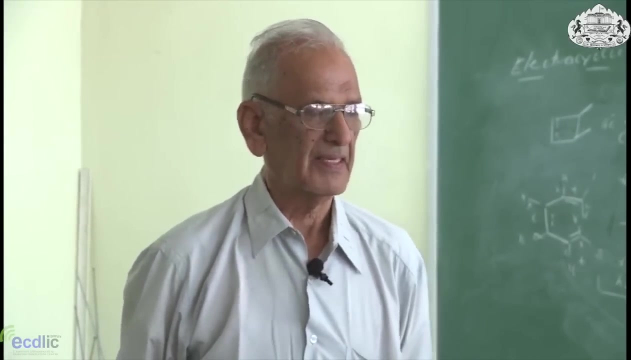 X, Y gets excited, ethylene does not get excited. So in a photochemical reaction the principle is more conjugated goes to less conjugate. In a thermal reaction you always go from less stable to more stable. In a photochemical reaction you always go from more conjugated. 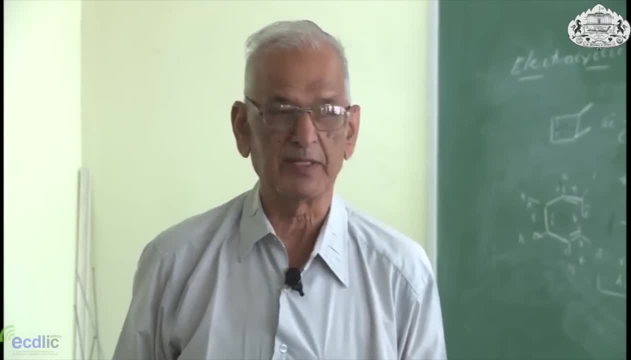 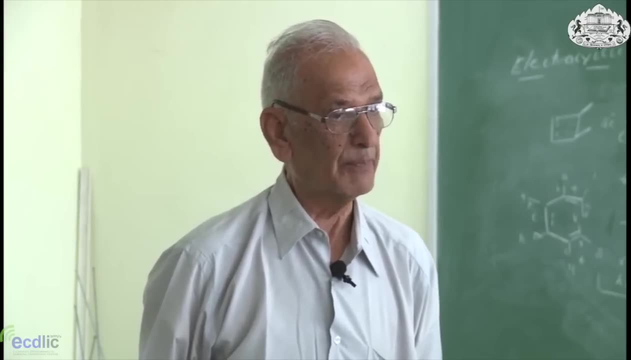 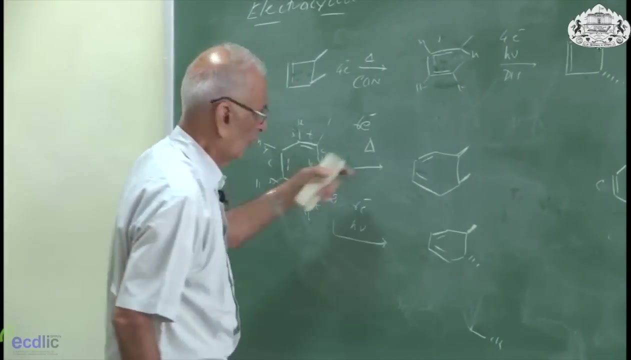 to less conjugate, even if less conjugated is less stable. That is why photochemistry is important. You can prepare compounds which are less stable, But here both went like this. Thermal also went like this, So in a thermal reaction, 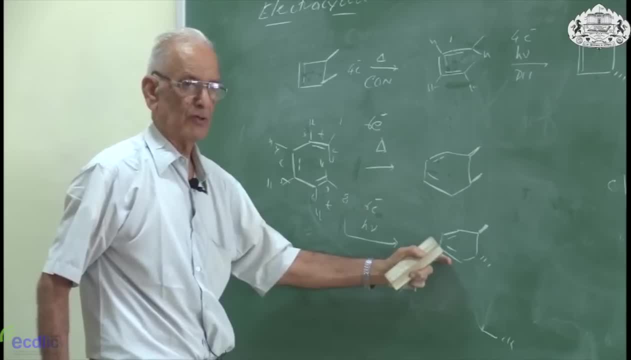 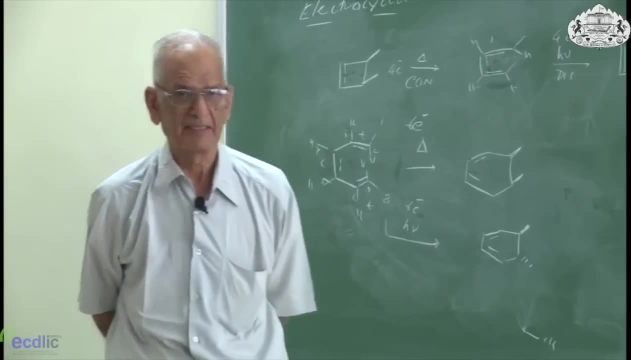 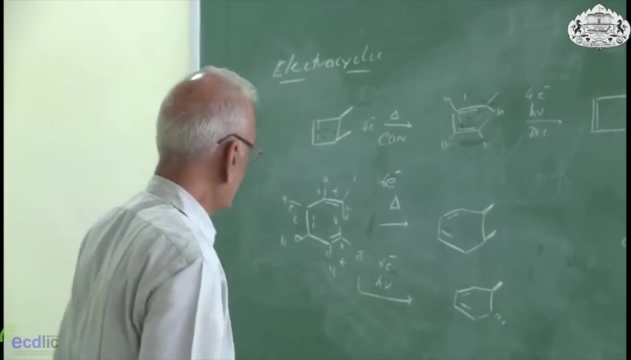 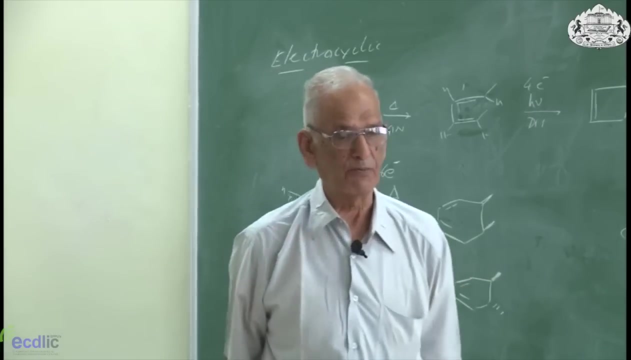 gives you ring compound. Photochemical also gave you ring compound. Why, How many double bonds? Three double bonds. Product has two double bonds. So more conjugated has gone to less conjugated In this case. less conjugated is also more stable, but that is not important. 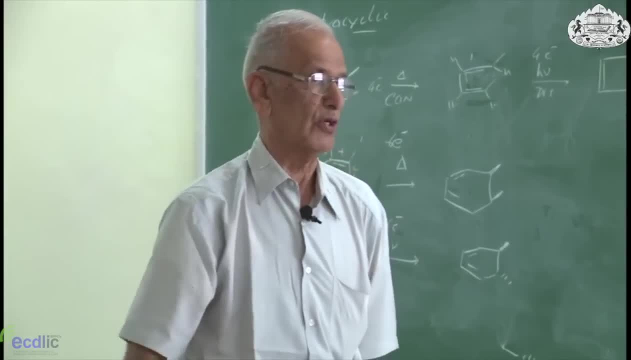 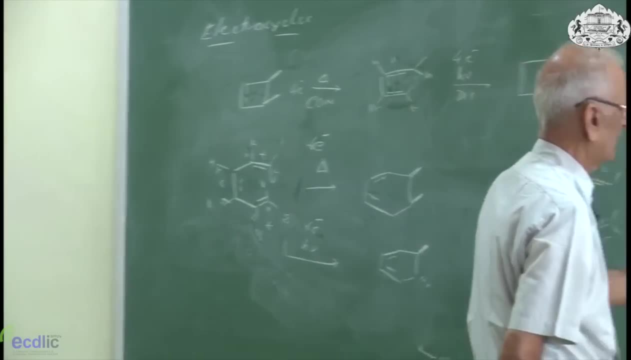 In photochemistry you always go from more conjugated to less stable. So in a thermal reaction you go from less stable to less conjugated. So two important principles that we have seen that in a thermal reaction you go from less stable to more stable In 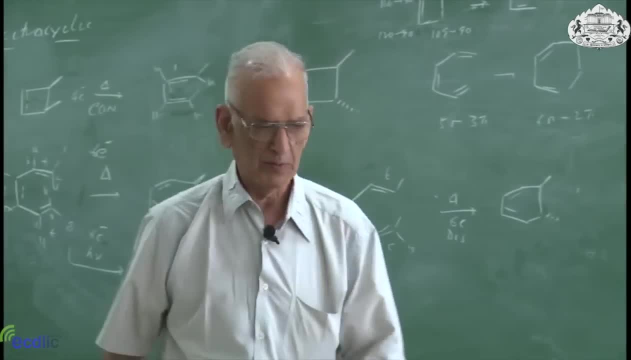 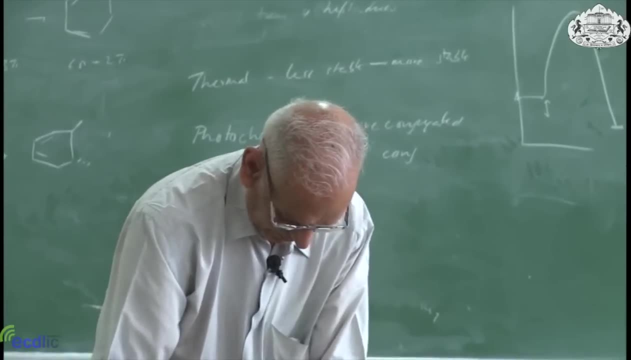 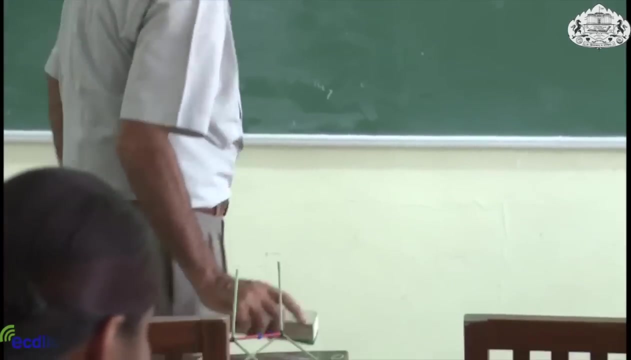 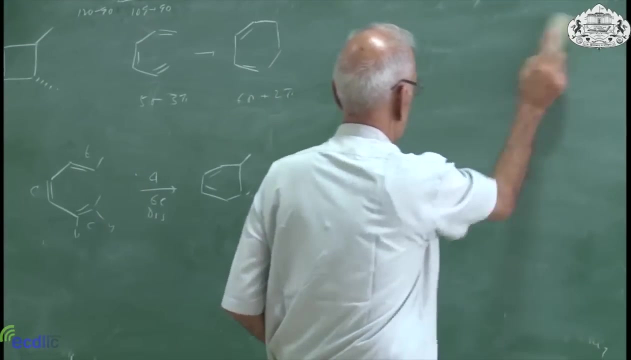 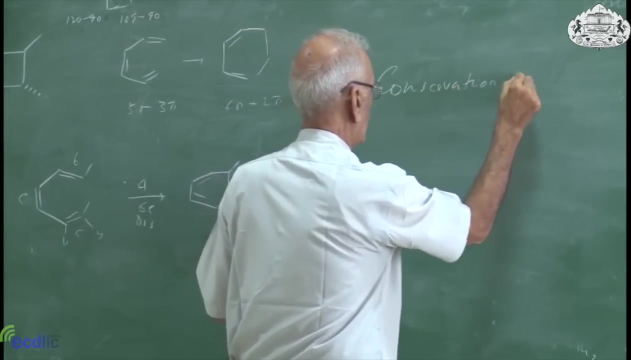 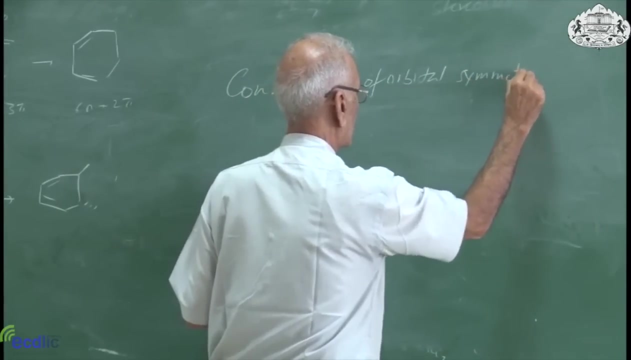 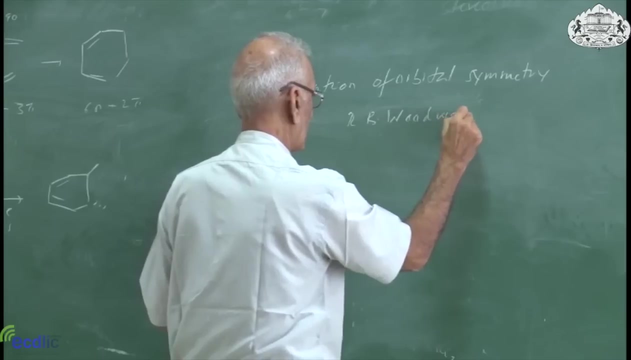 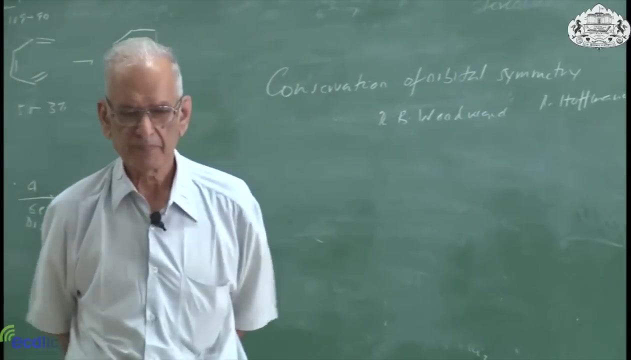 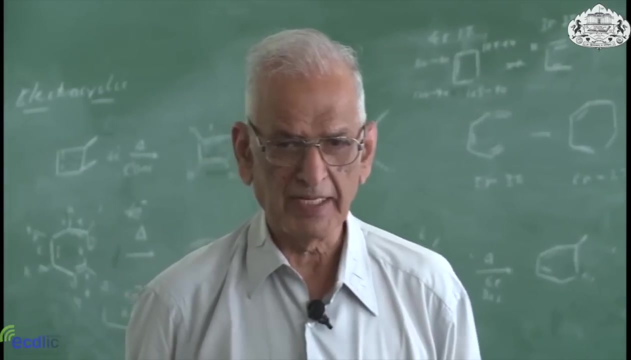 a photochemical reaction. you go from more conjugated to less conjugated. All right. What are the books you can see? Conservation of Orbital Symmetry, R B Woodward Roald Hoffman. Where have you heard this name, Woodward, apart from today? Yes, 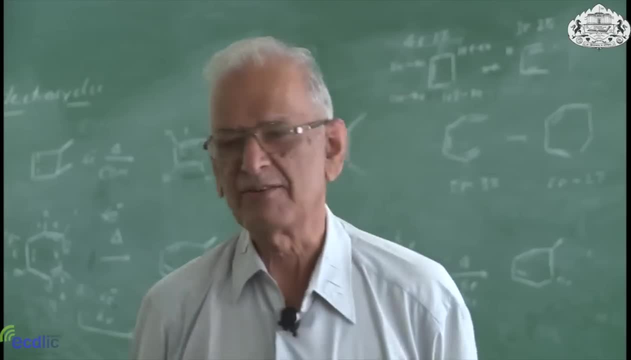 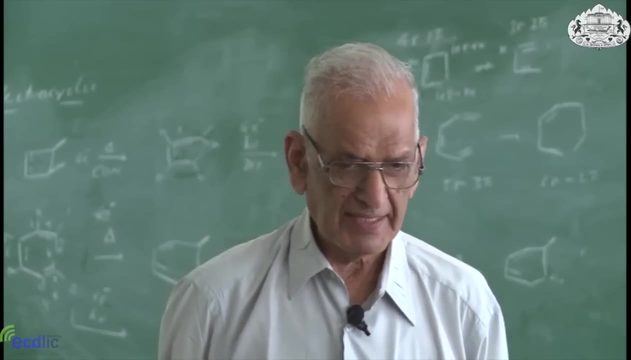 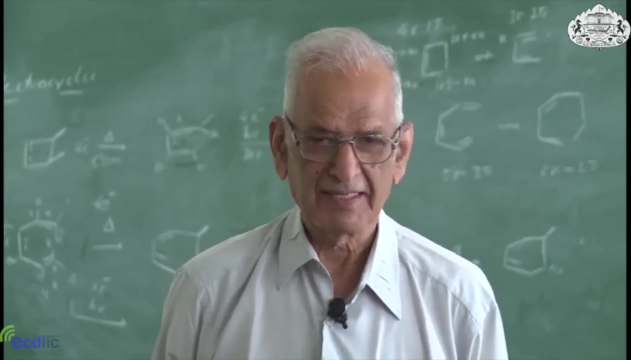 Calculation of lambda max. Calculation of lambda max- Very famous Woodward rules. What was his age when he made these rules? When he made these rules, he was 19 years old. Yes, And after 60 years, we are still teaching these rules. So now is the time for you all. 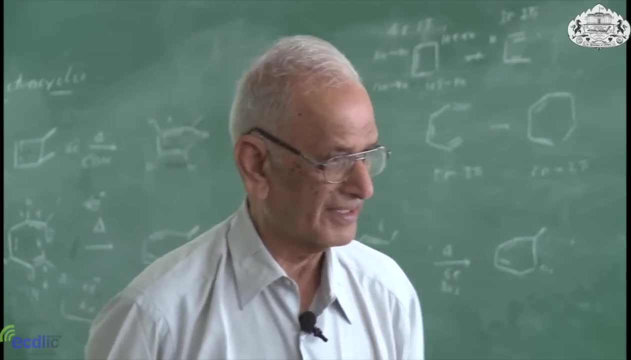 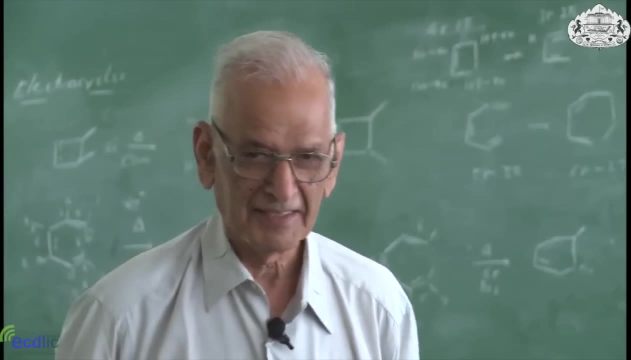 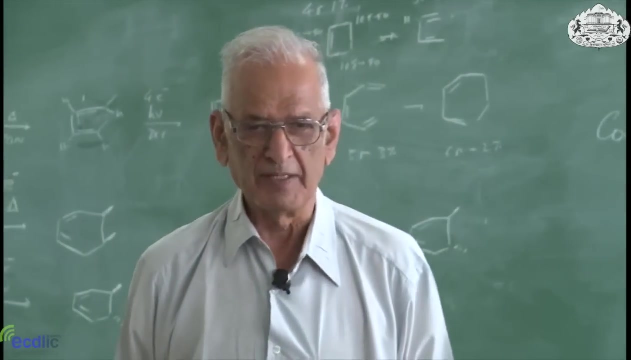 to do something great. All good things are done at young age. All old people think they are very wise, but usually that is not correct. All good science is done at the young age, all right, So better start doing now. There are lots of stories about Woodward Number. 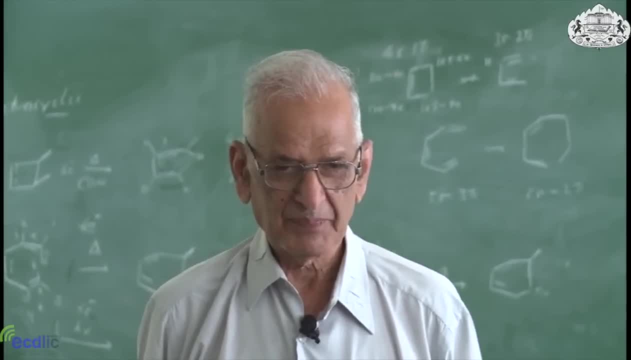 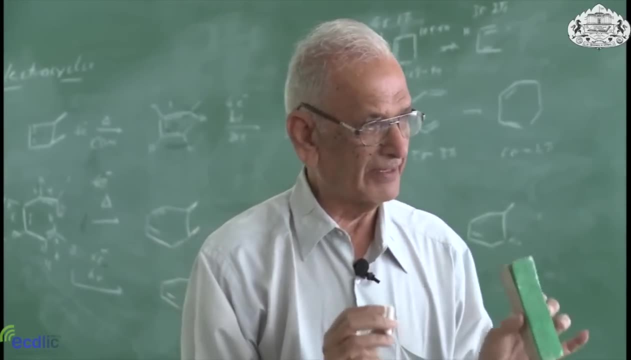 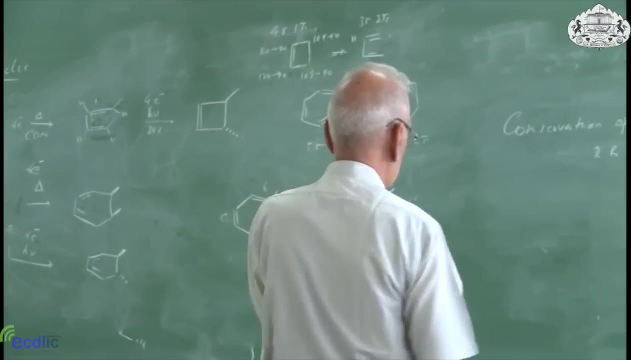 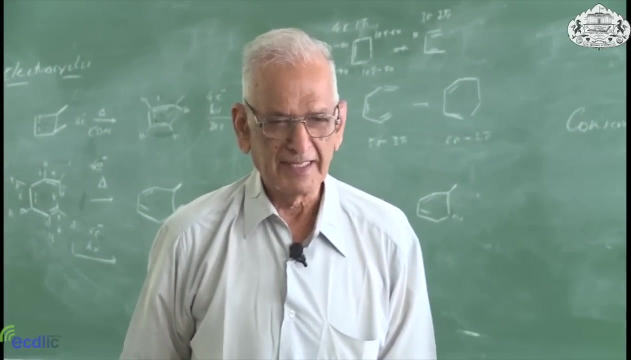 1. A Woodward lecture. being very arrogant, he brings his own chalk and his own duster. He does not believe in your chalk and your duster. Whichever country you are in, he uses his own chalk, own dust. Even on the days when everybody used slides, Woodward did not use 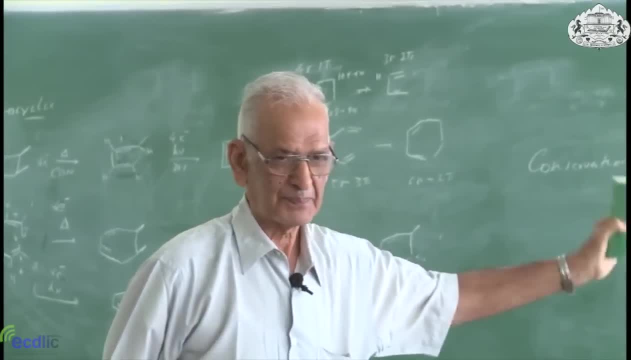 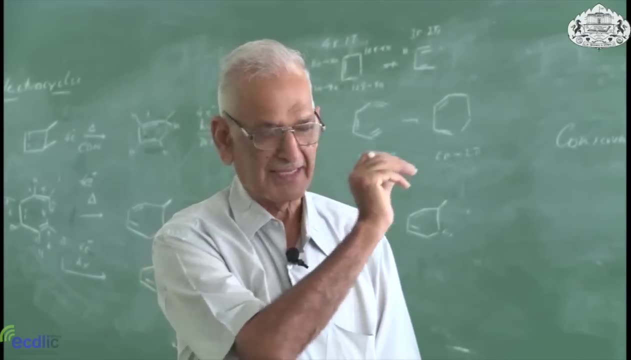 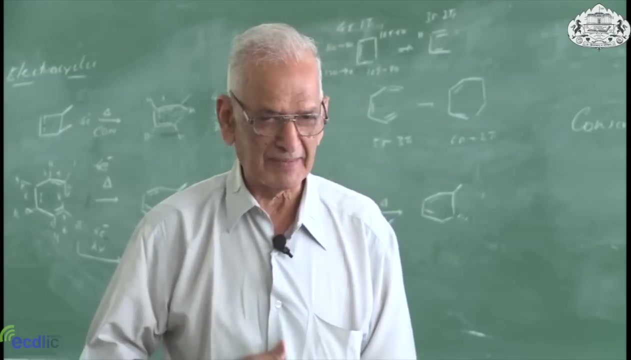 it. He started from left hand side of blackboard. His lecture is so planned that if he has a sufficiently large blackboard, his lecture ends in the right hand corner. Listening to Woodward lecture is something I mean. you are fortunate to listen to a Woodward lecture. 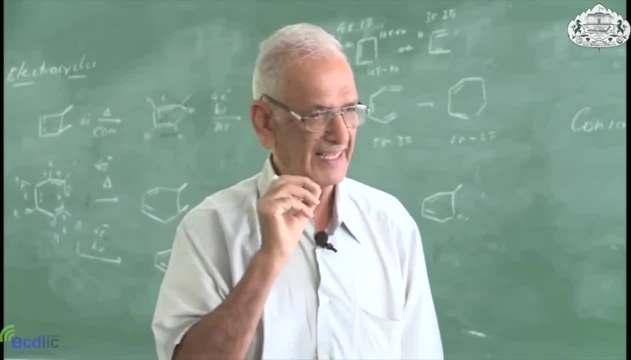 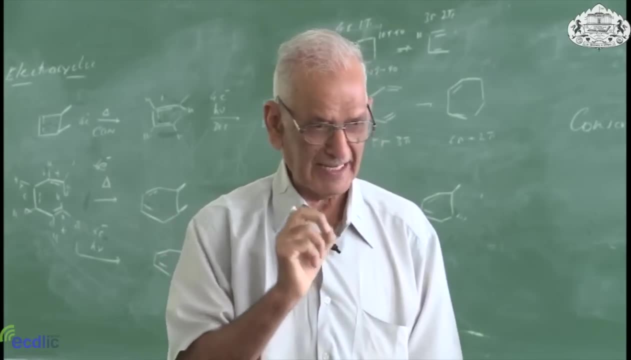 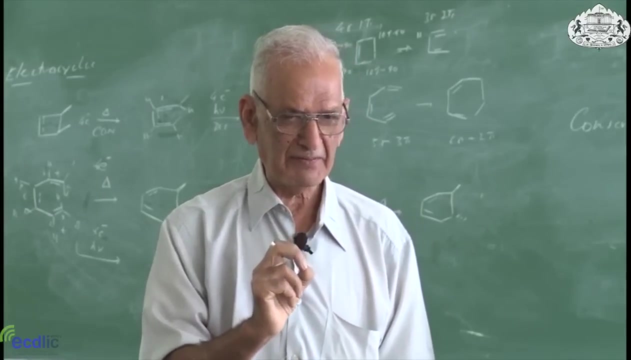 Western world is very conscious of time. When they say lecture is eleven o'clock, they are supposed to be in the class at eleven o'clock. Lecture is eleven to twelve, So lecture will start at eleven. he will stop at eleven. fifty five five minutes for questions. 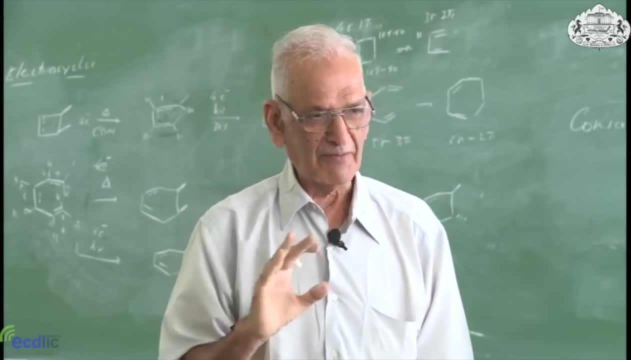 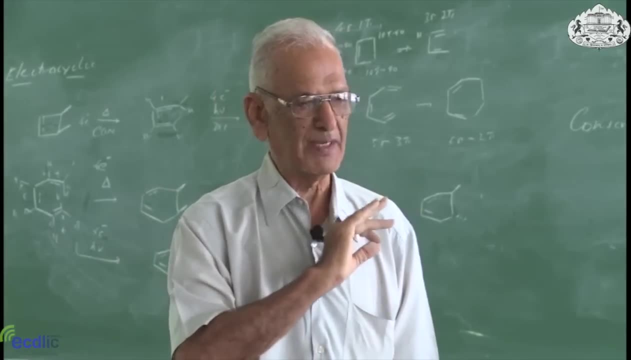 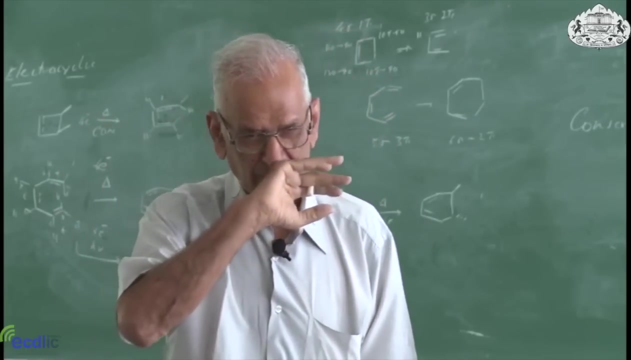 he will be out of the class at twelve. For everybody in the Western world, this is it, but Woodward was an exception. His lecture will be two p m onwards, Woodward, So he is the only person for whom No time schedule. It is said that when he was a young boy, when all American children 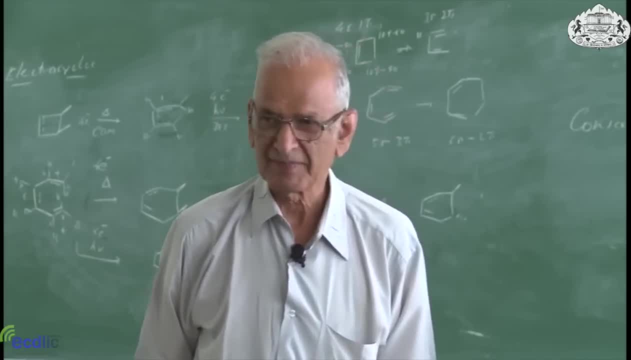 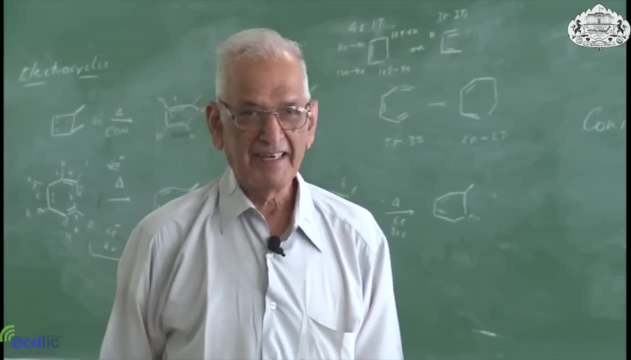 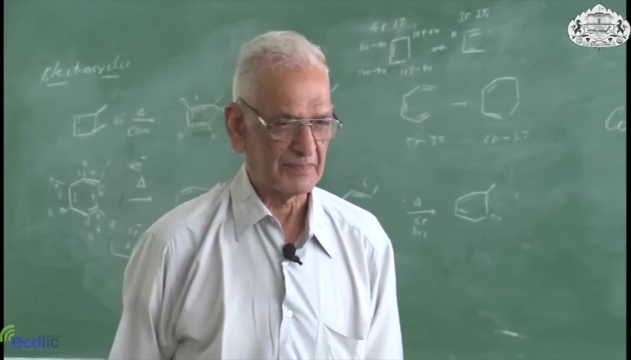 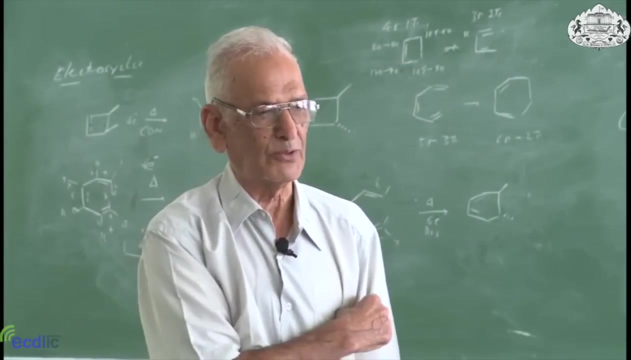 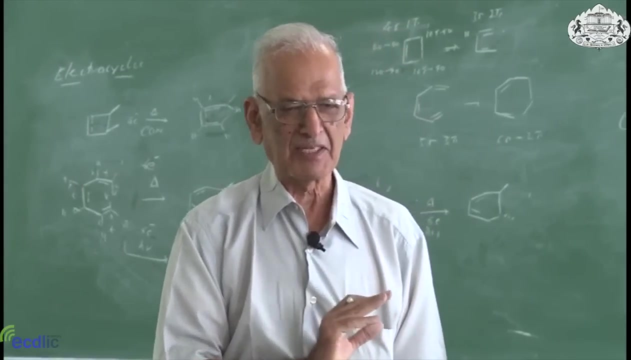 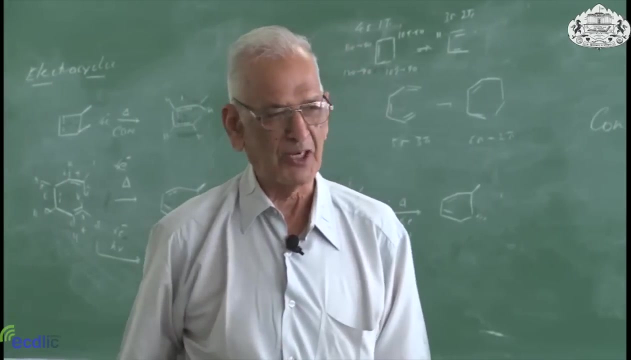 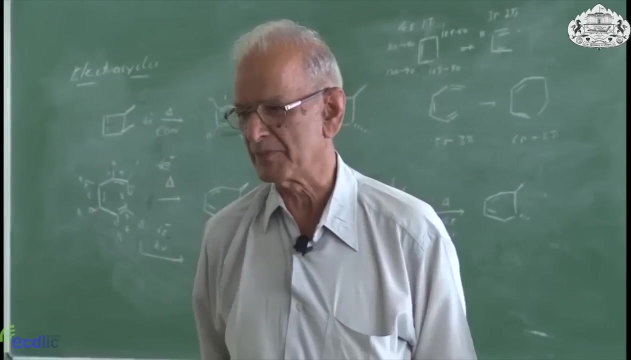 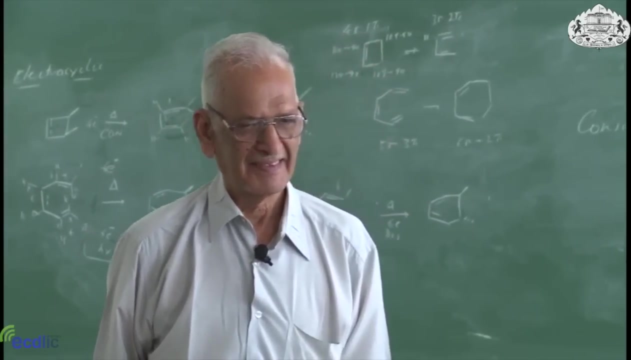 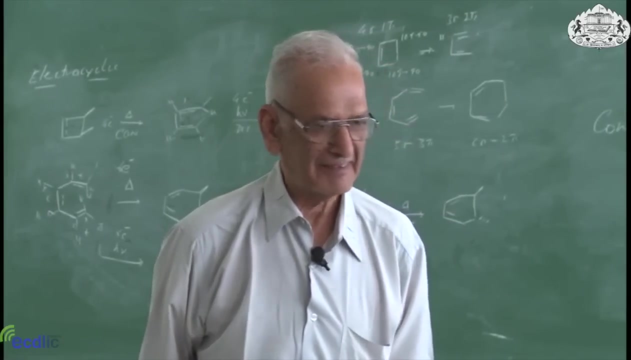 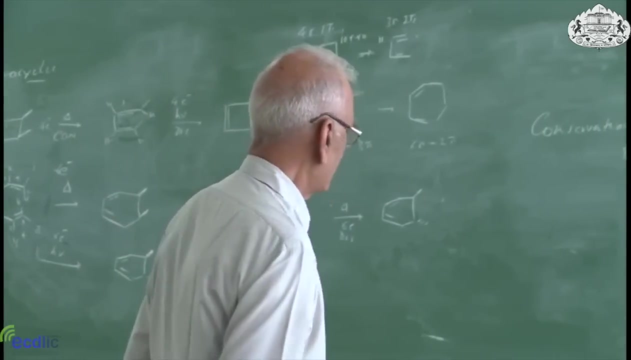 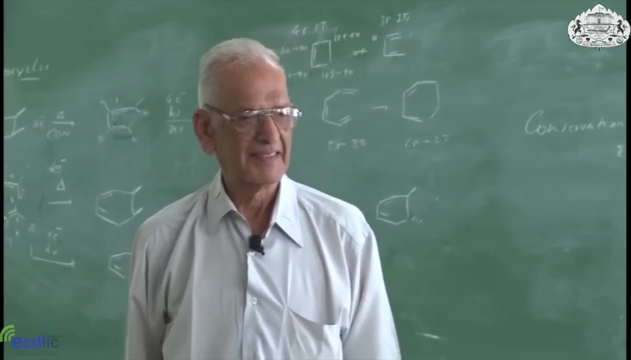 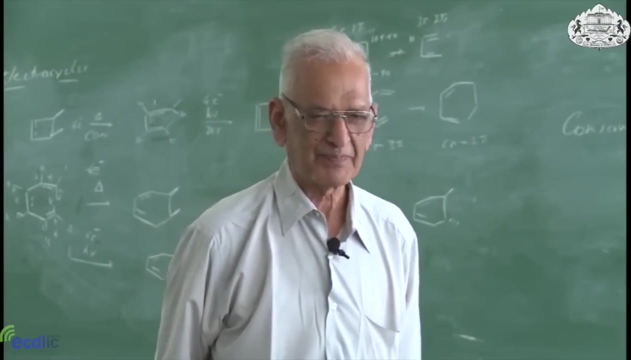 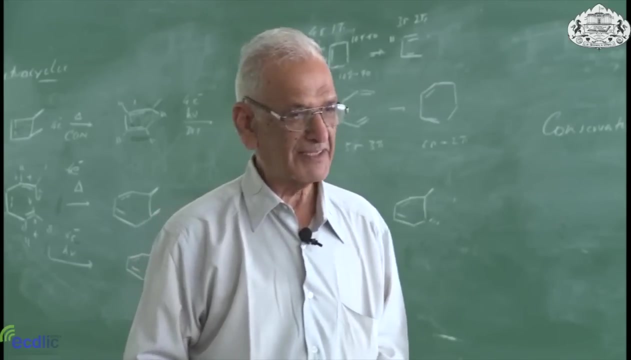 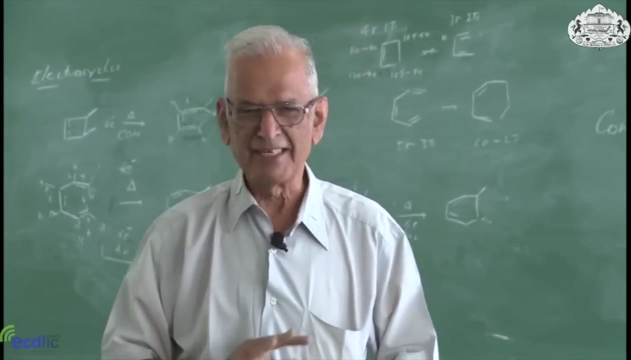 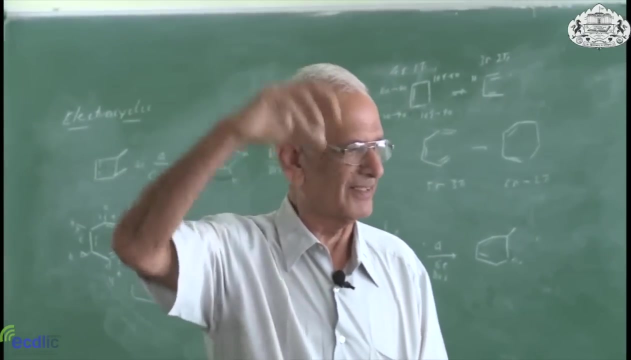 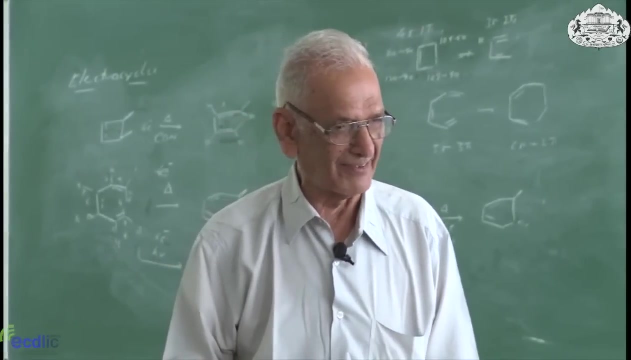 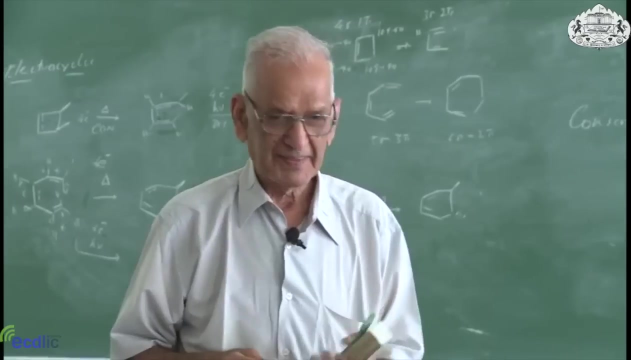 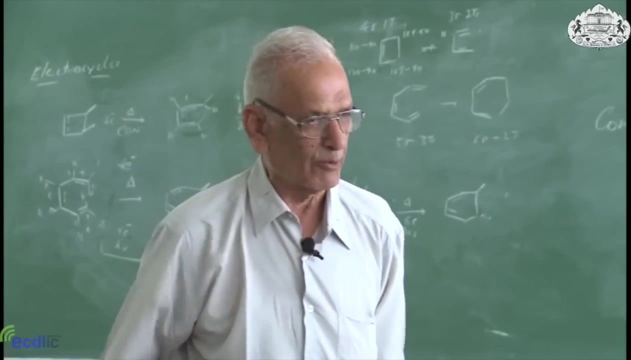 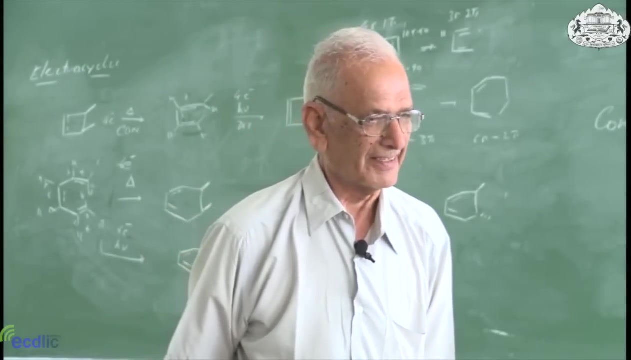 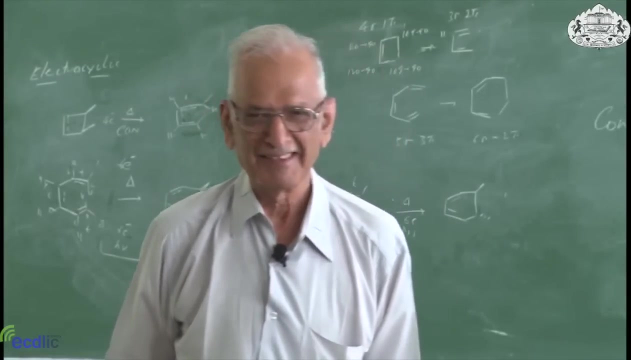 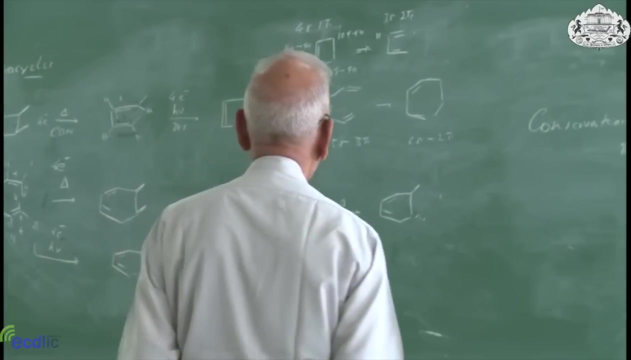 are crazy about basketball and baseball. Woodward was interested in organic chemistry even the age of six, eight, ten. End result is: in his BSC exam he failed in physics. No time schedule. but in the American system that is not the case. So that is Woodward. 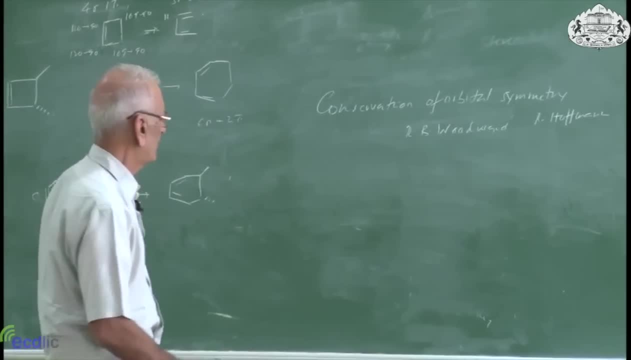 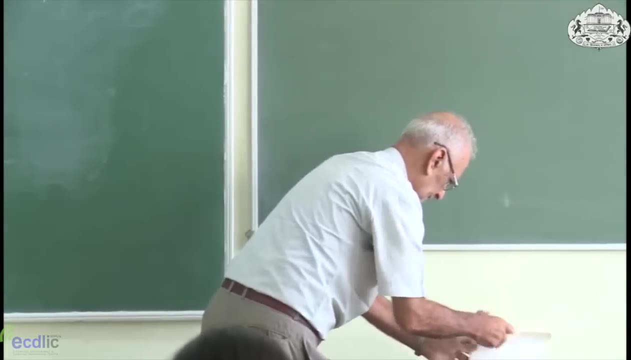 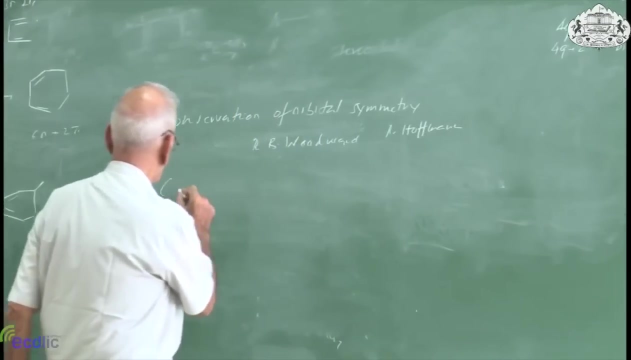 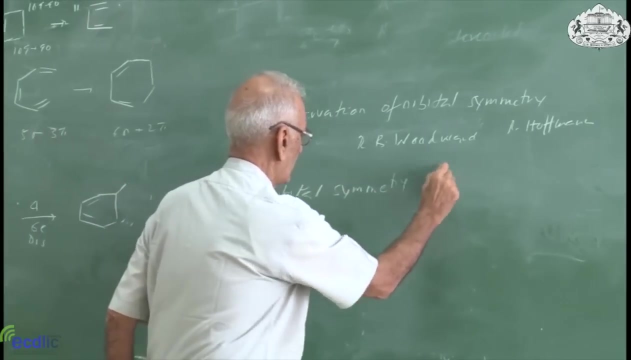 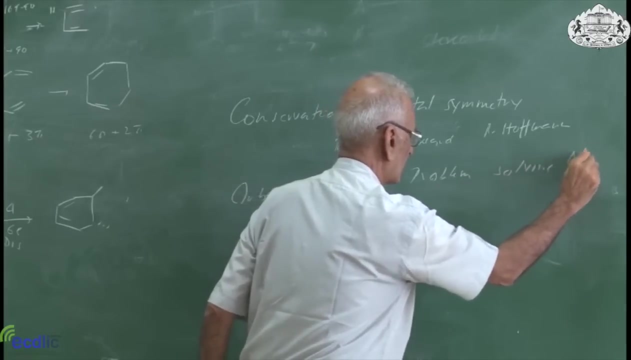 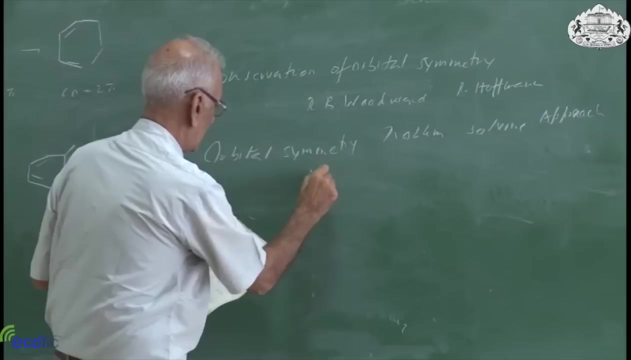 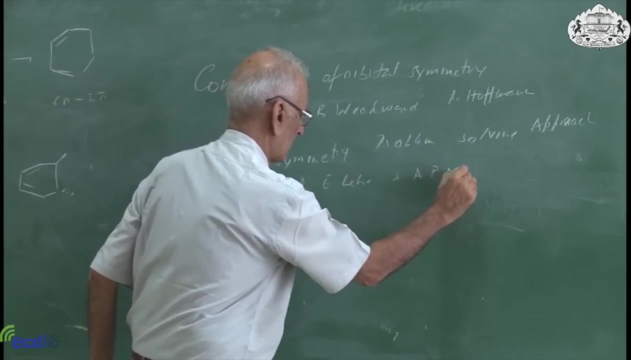 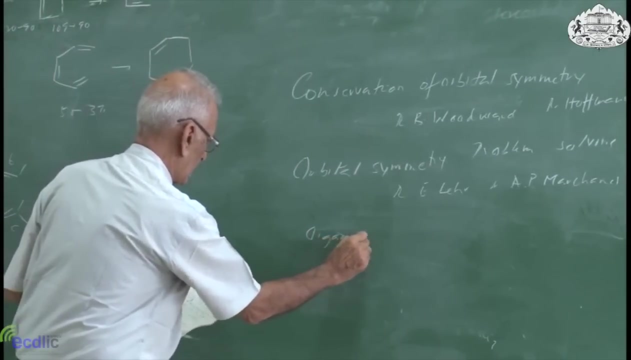 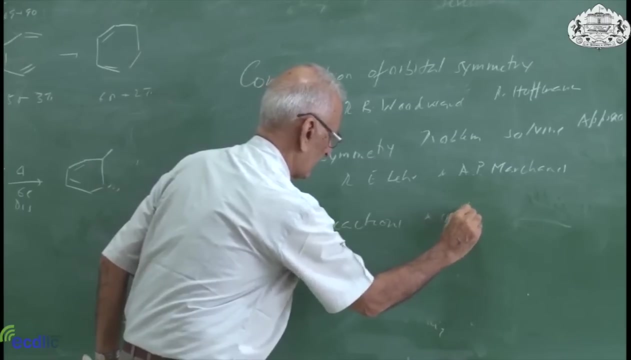 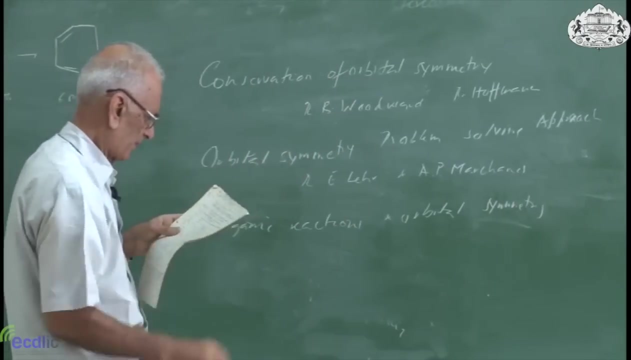 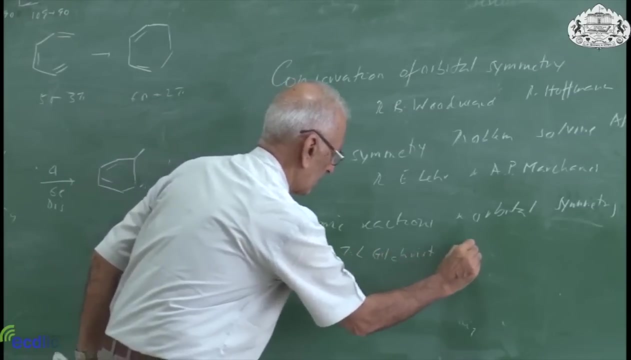 conservation of orbital symmetry. Woodward and Hoffman. Okay, Let us…. Orbital symmetry, orbital symmetry, it is an arbitrary equation. It problem solving approach: R-E layer and AP, moisture, Atmospheric reactions and orbital symmetry. T L Gilchrist, R C Storr. 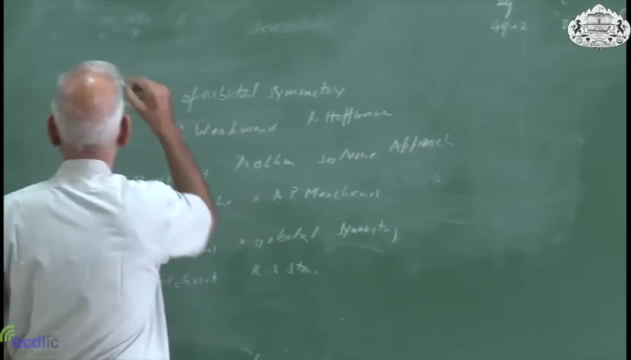 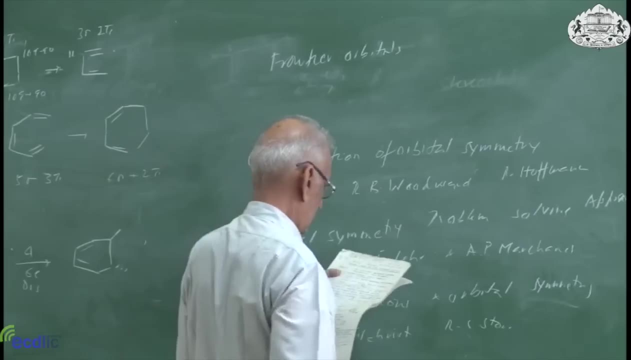 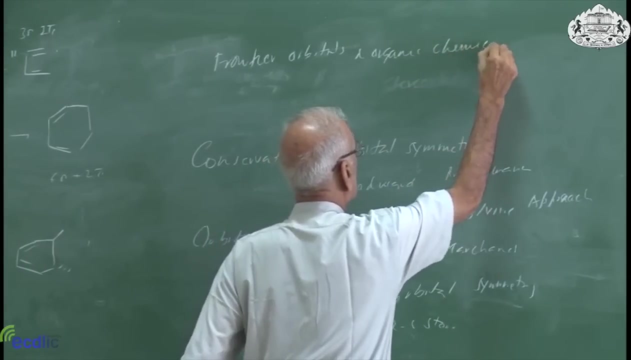 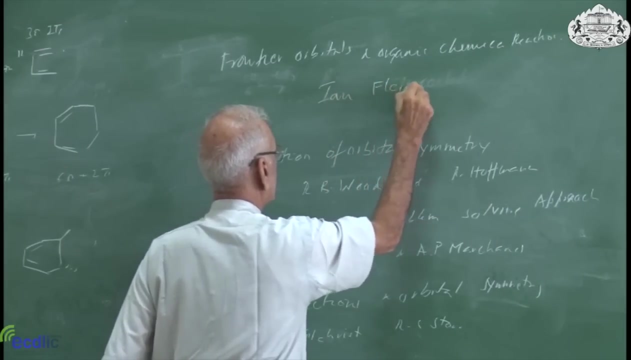 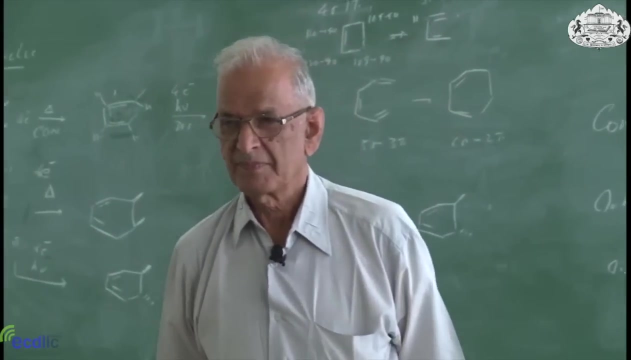 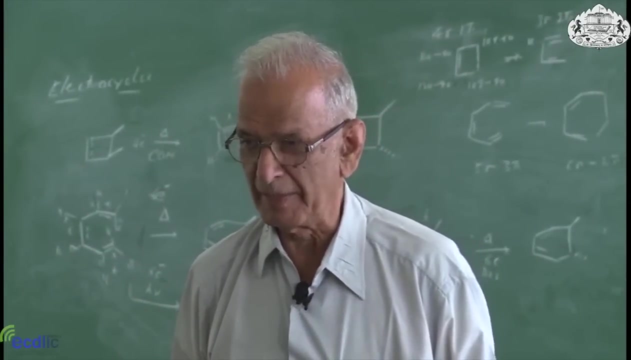 Thank you. Frontier orbitals and organic chemical reaction. Ian Fleming. You know Ian Fleming, You heard him. Do you remember Ian Fleming? All James Bond novels are written by Ian Fleming, not the same Ian Fleming. all right, That is a different Ian Fleming. 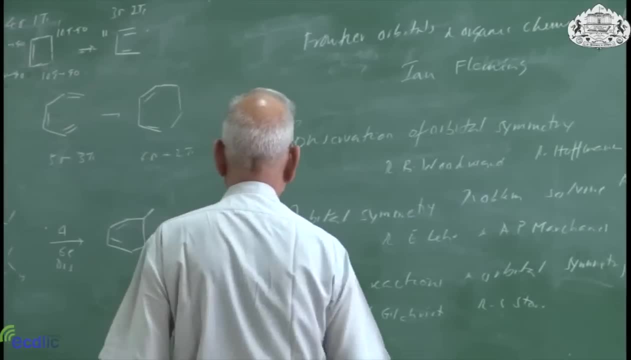 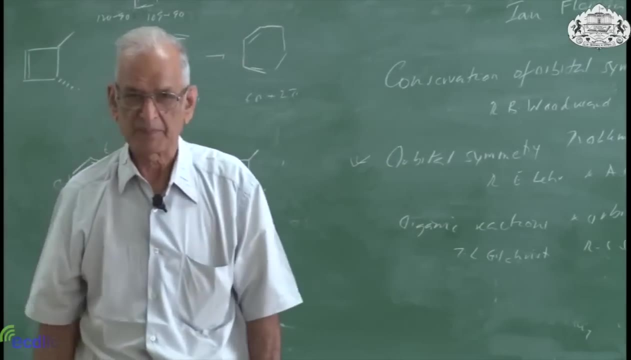 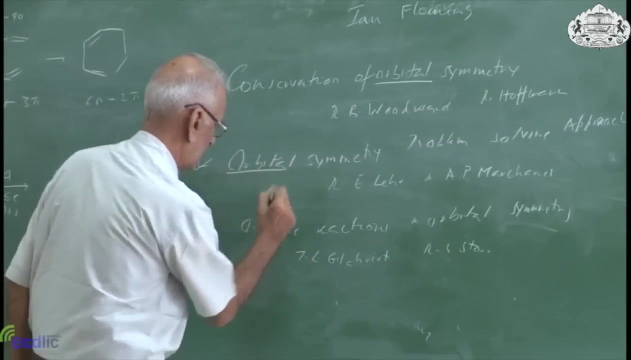 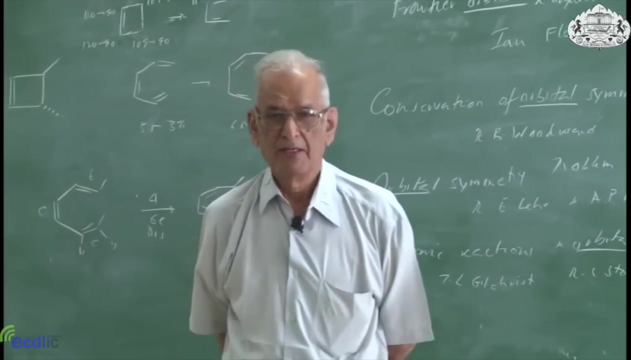 What is the purpose of writing this? We are going to choose many of the things from this book, not that we want from the others. All right, Purpose of writing this was to bring out this, All right, Thank you. So for explaining. pericyclic orbitals are very important. 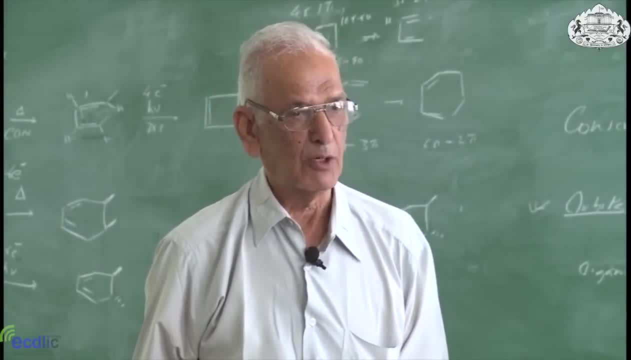 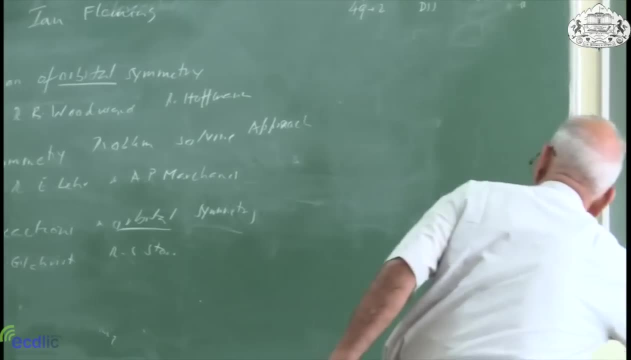 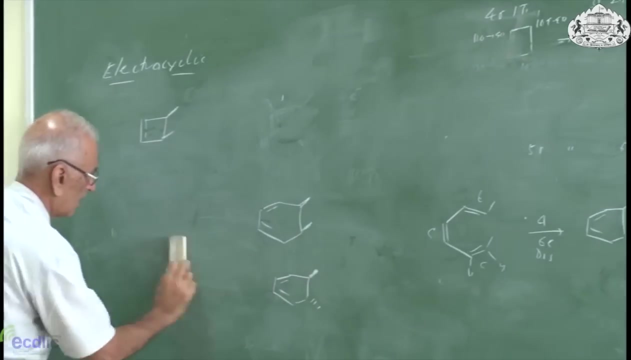 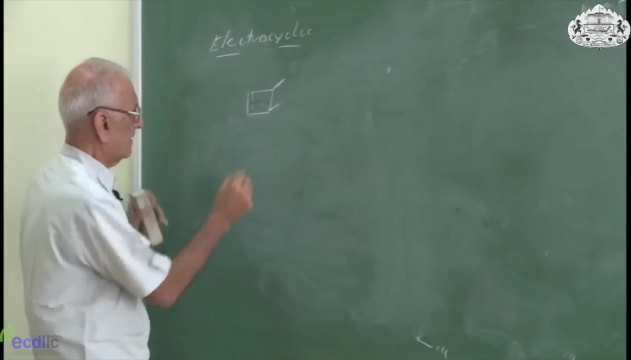 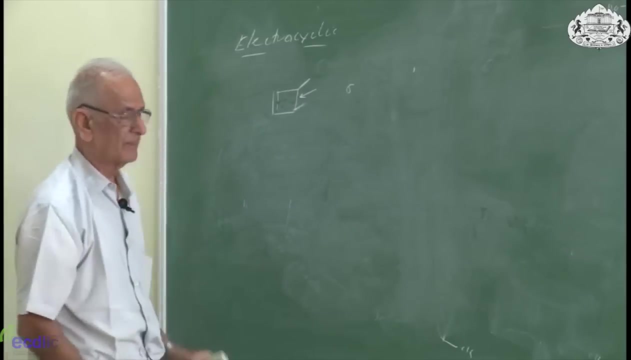 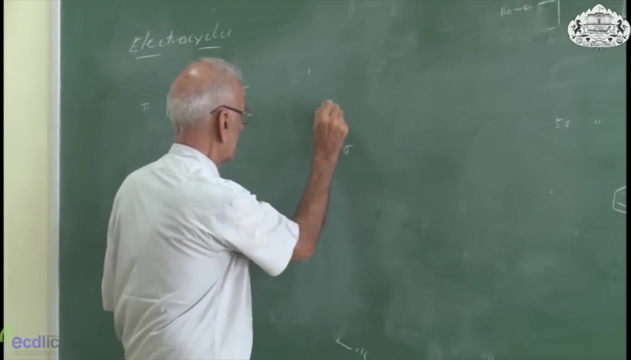 So our first job now is how to draw orbitals. Have you? Yes, Yes, Yes, Yes. So what are the reacting orbitals? This is your sigma orbital, This is your pi orbital. So, sigma pi pi star. sigma s. 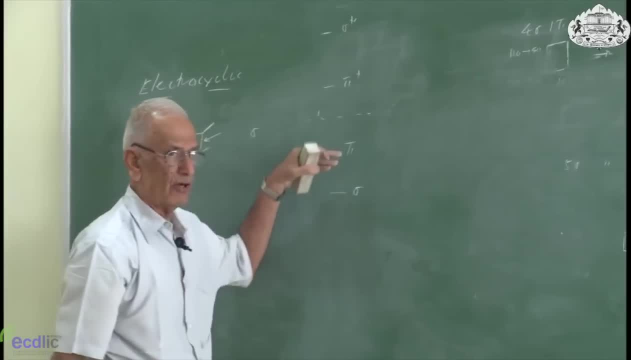 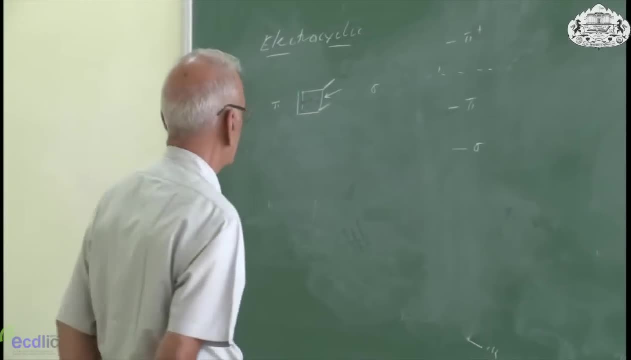 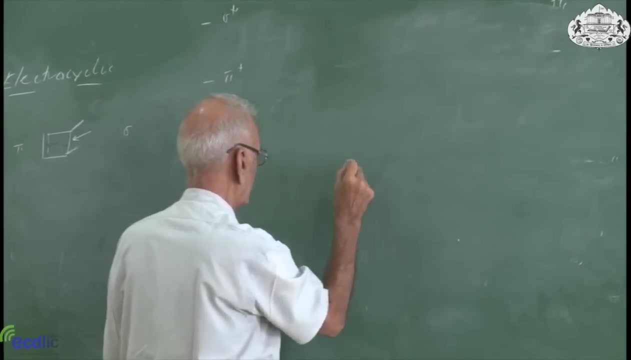 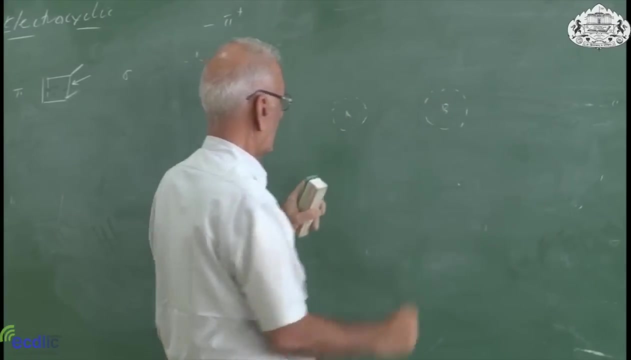 These are your bonding orbitals. In other words, these are your bonding orbitals. Now let us explain it. Take an example of the orbital sigma s bonding orbitals. these are your anti-bonding orbitals. So how can I show That is atom? 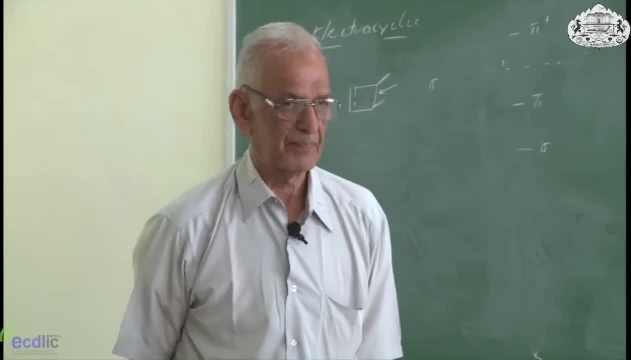 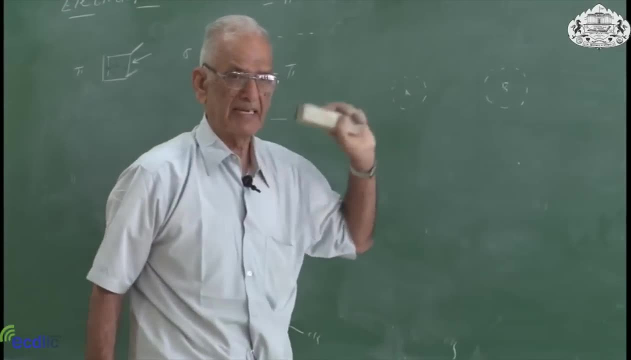 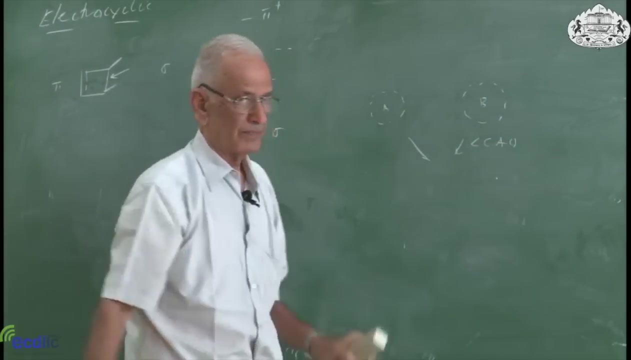 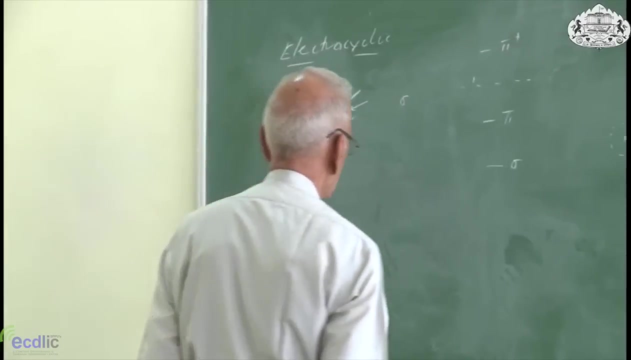 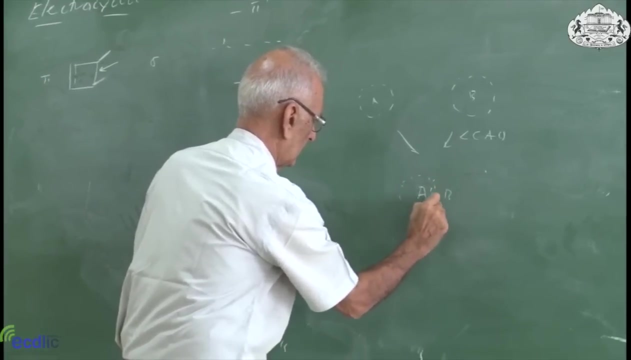 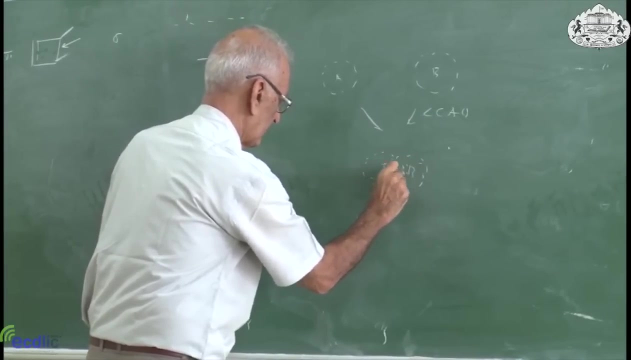 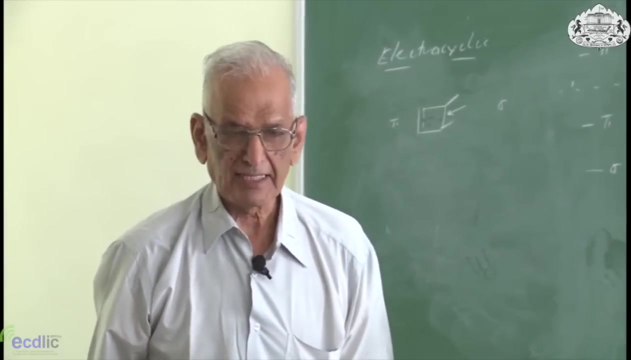 A surrounded by electron, that is, atom B surrounded by electron. Hydrogen atom combining with hydrogen atom. was that LCAO- Linear combination of atomic orbitals? LCAO- Linear combination of atomic orbitals. What are these dots supposed to show? The dots are supposed to show probability of finding. 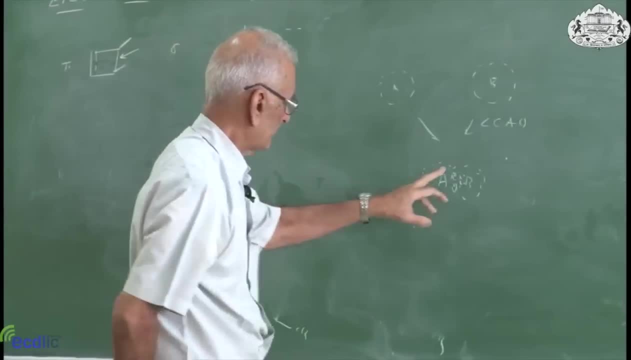 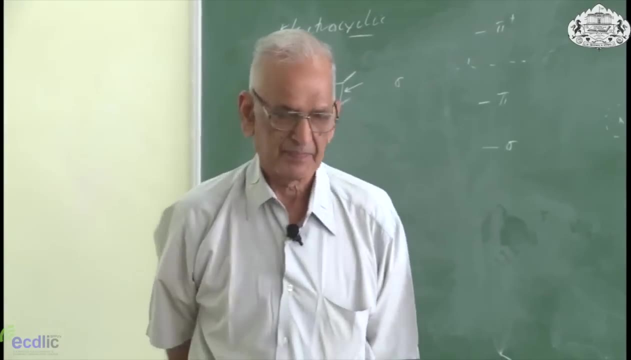 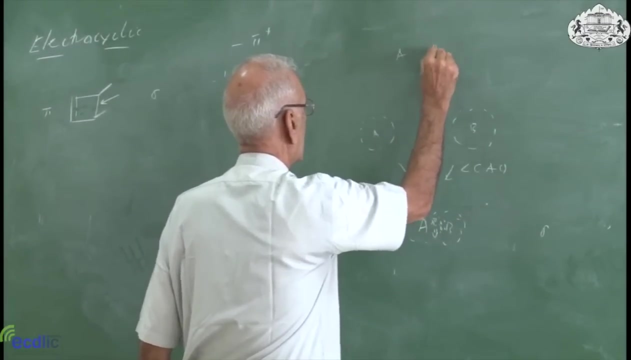 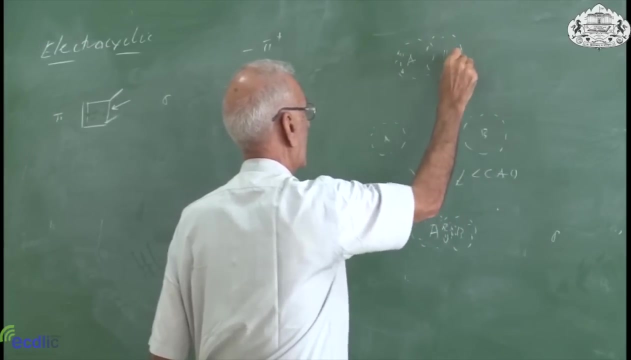 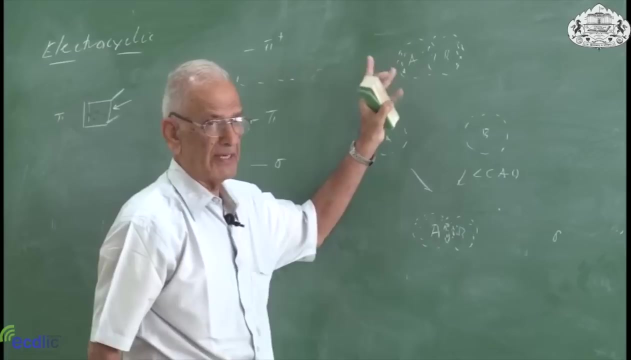 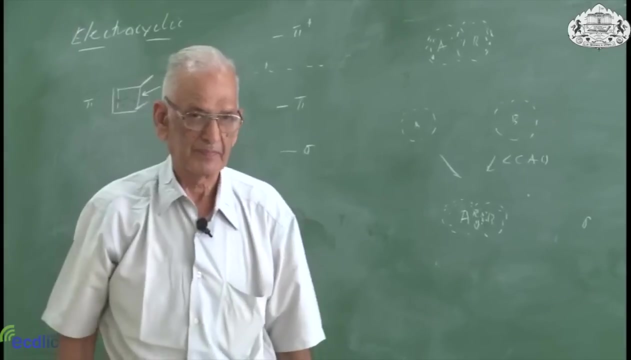 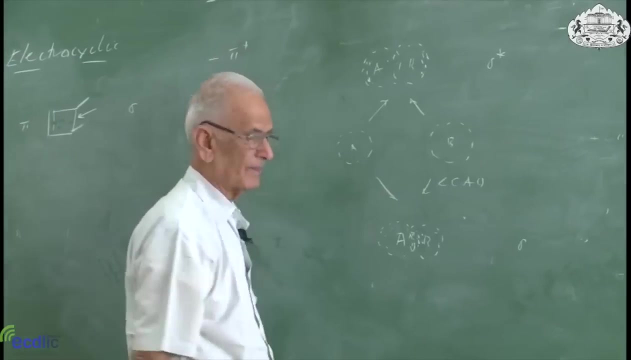 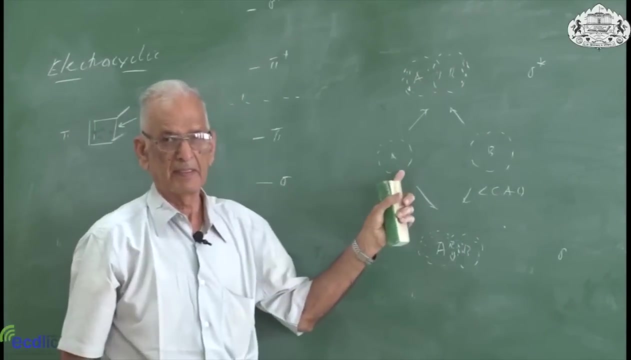 the electron. So more dots are here. Therefore, more probability of finding the electron is between A and B. This is your data, your picture in this sigma already. What are we showing? More probability of finding the electron is either here or there. This is your sigma star already. Boy meets, girl gets. 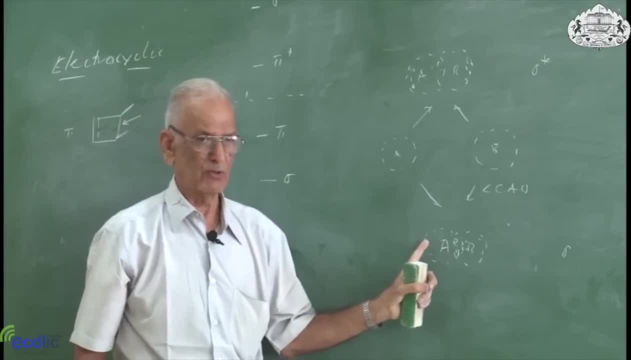 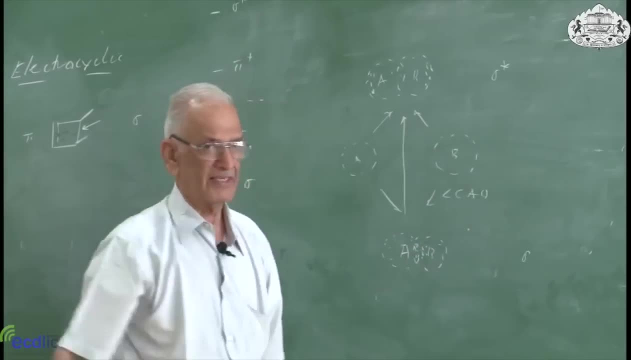 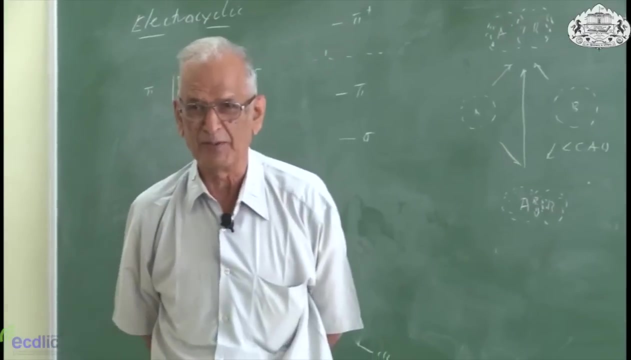 married. So what should happen? Husband should look only at wife, wife should look only at husband. Then somebody says something: I saw your husband with some other girl. Then this picture happens: Wife is looking out of one window, husband is looking out of other window. So 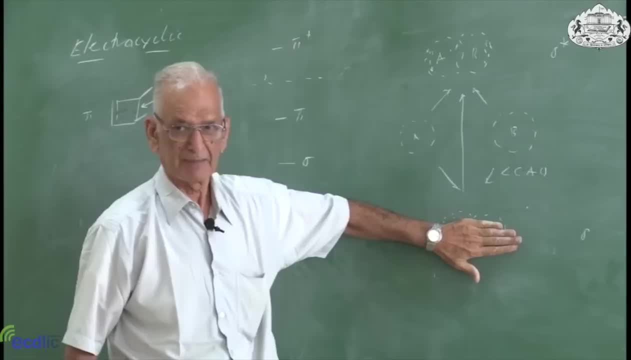 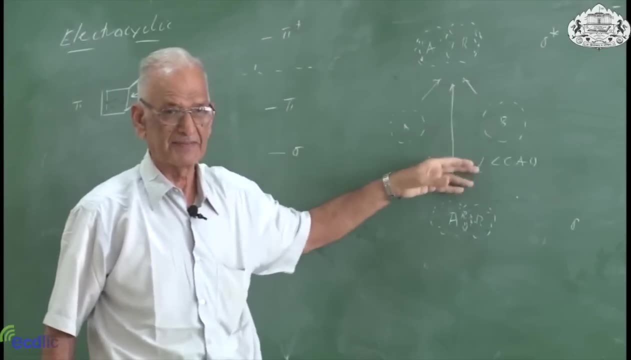 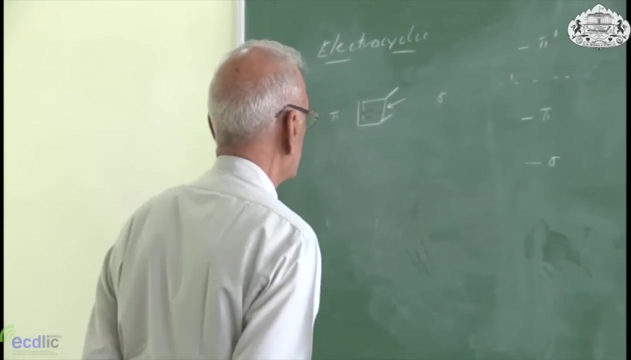 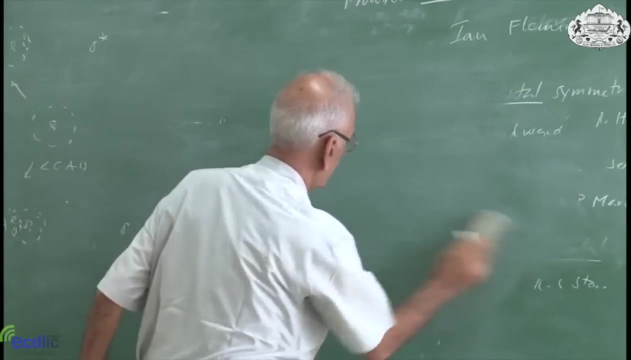 normal picture. happy picture is this bonding. An happy picture is that In molecules it comes back very quickly to ground state. With human beings it takes longer time. So that is the picture that you have. This is your signal, that is your sigma orbital and your sigma star. 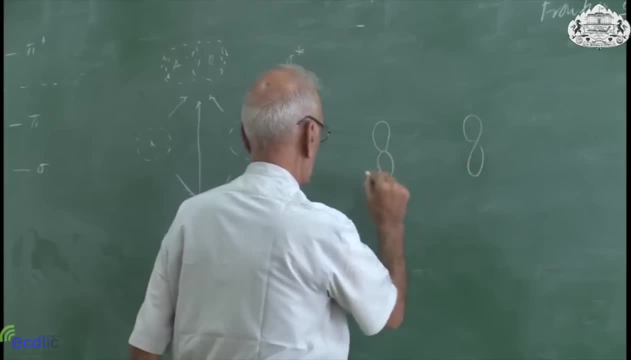 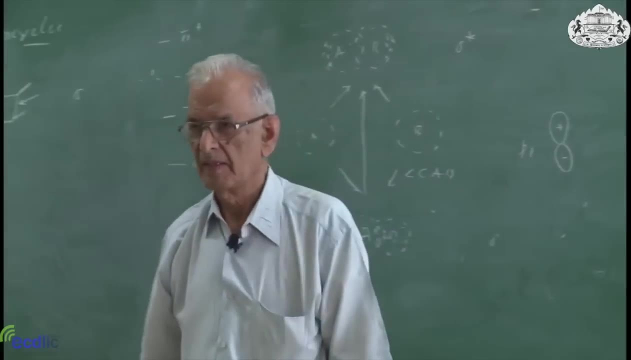 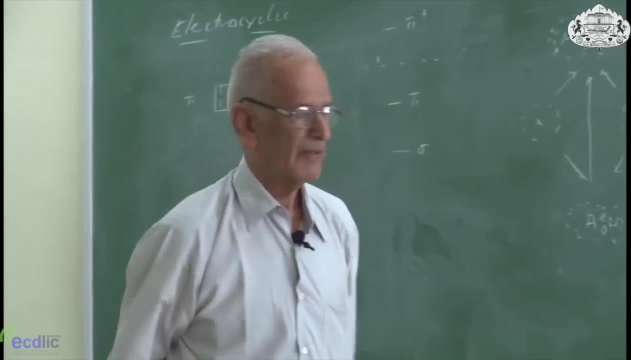 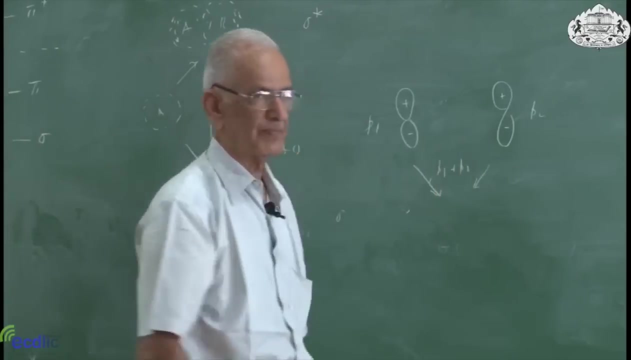 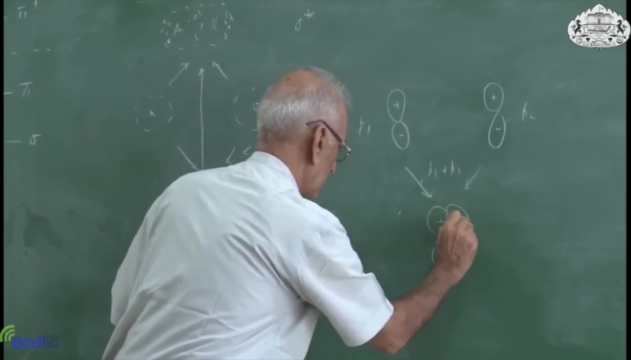 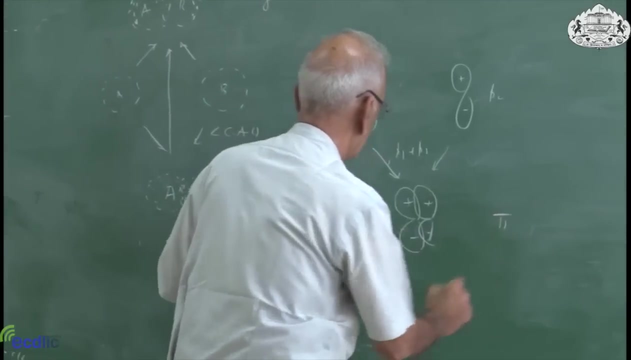 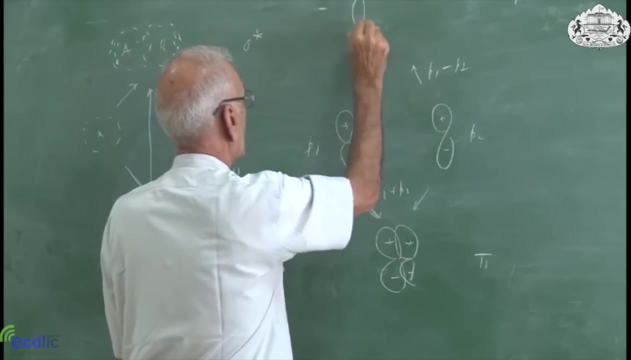 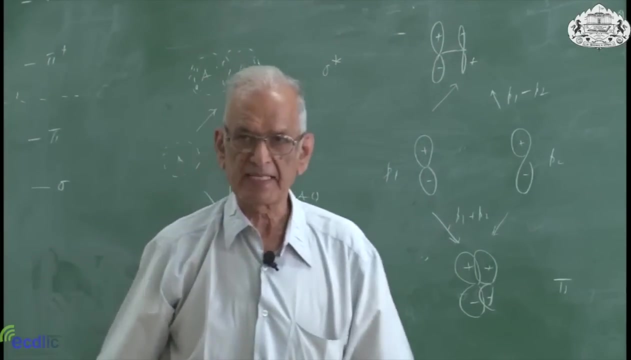 So this is your p orbital, That is your other p orbital. We can combine these orbital values: orbital p 1 plus p 2, p 1 plus p 2 means plus, plus, minus, minus. This is your phi orbital and p 1 minus p 2.. Here both pluses are on the same side, they are plus and minus. So 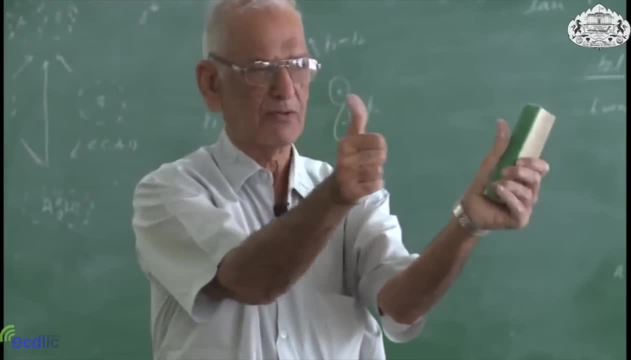 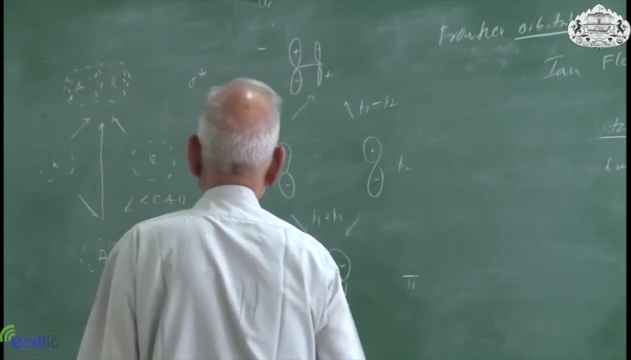 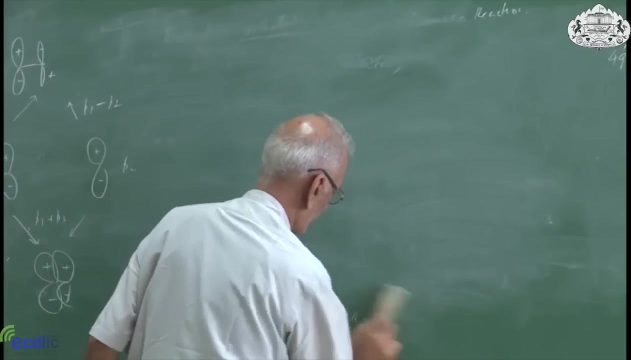 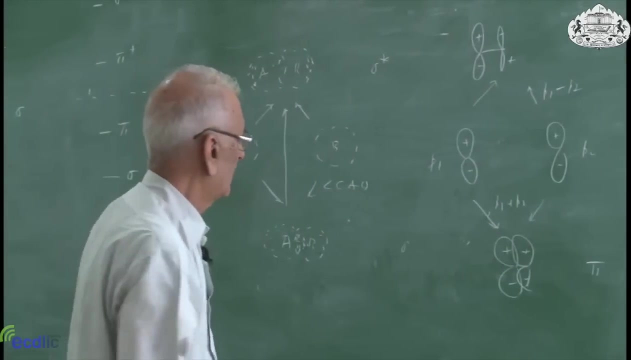 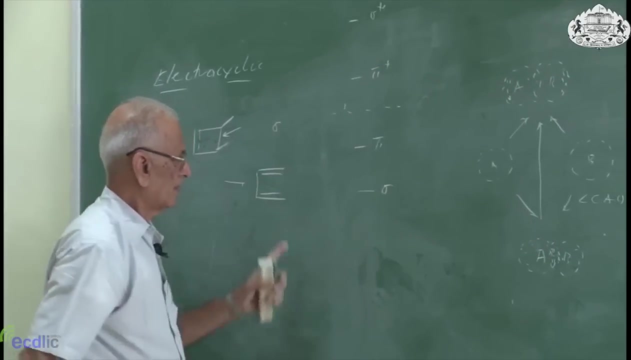 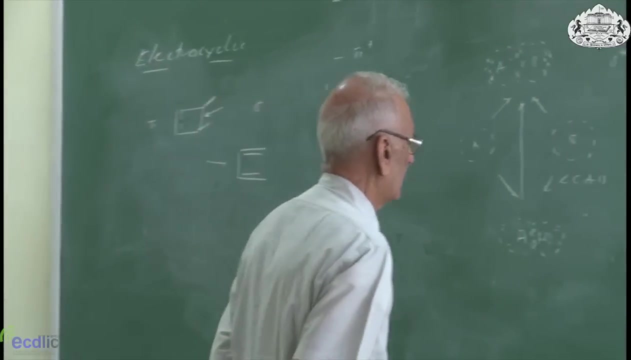 you combine them, Thumb is plus, So one combination is this. second combination: plus is combining with minus. So this is your phi orbital and phi star. Yes, So we wrote the four orbitals of cyclobutene. Now we have to write four orbitals of butadiene. 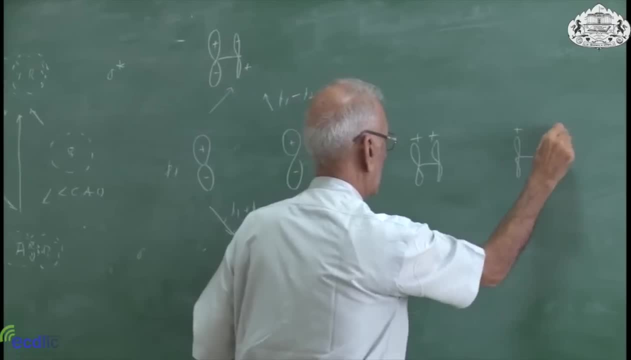 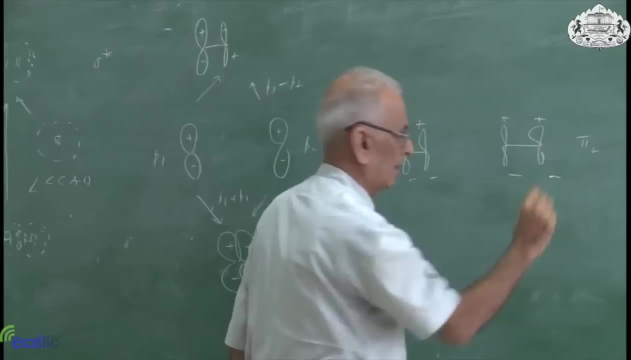 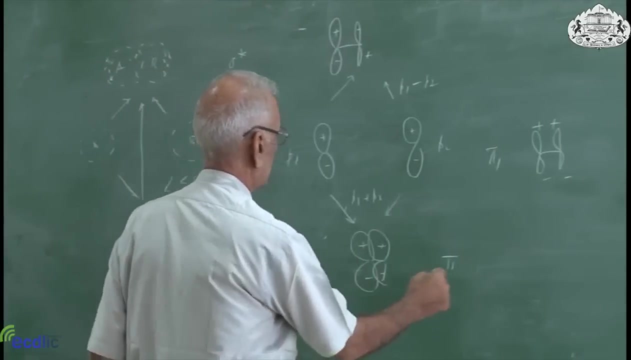 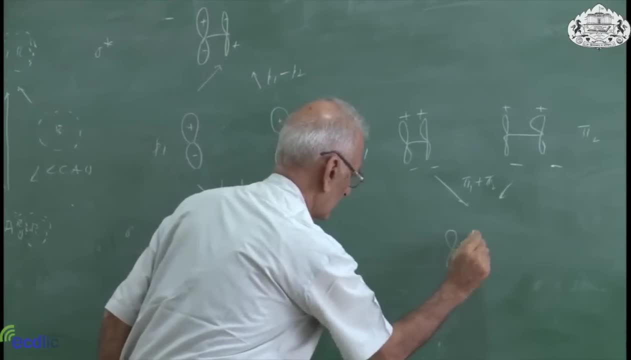 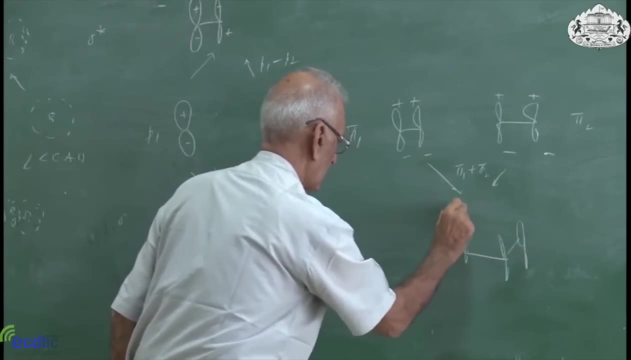 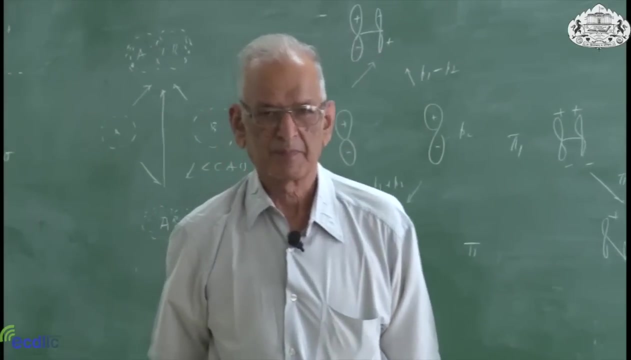 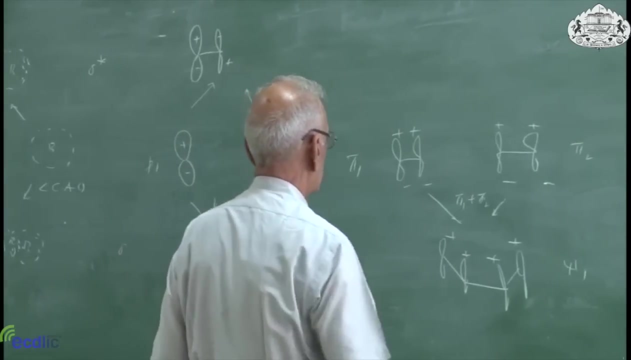 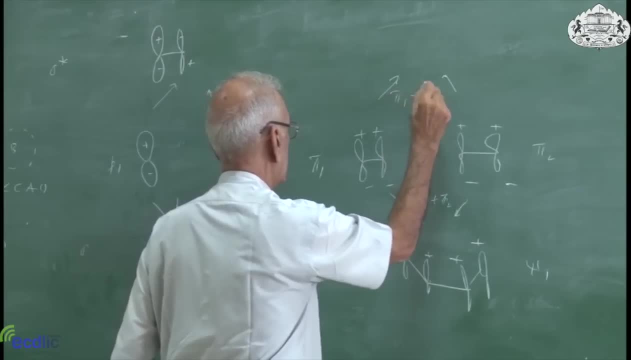 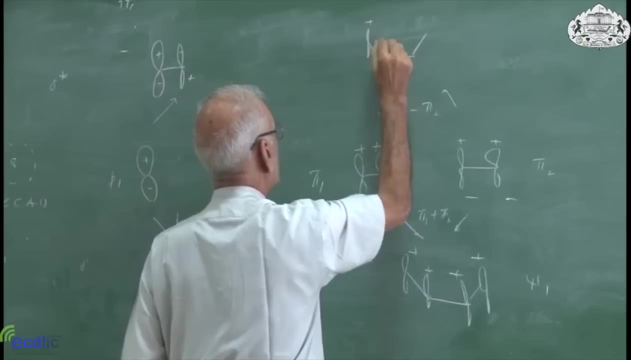 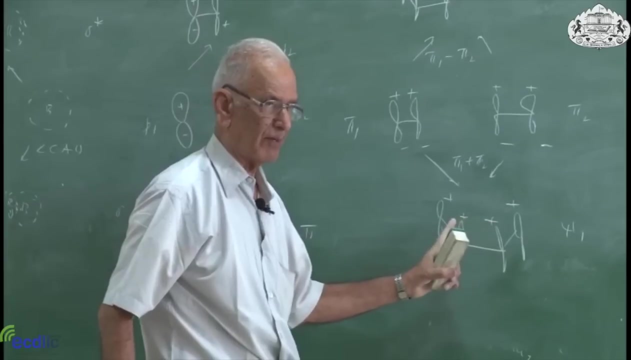 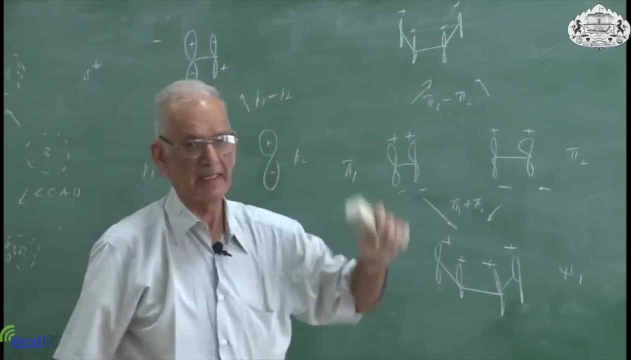 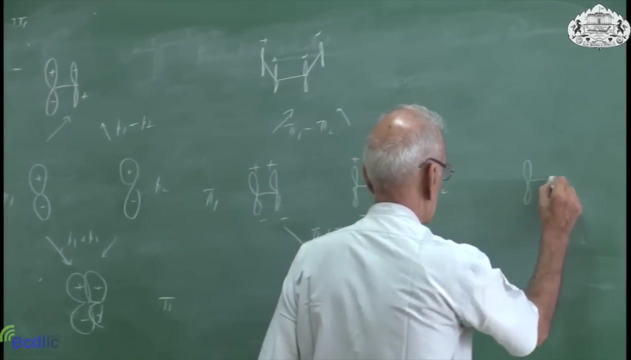 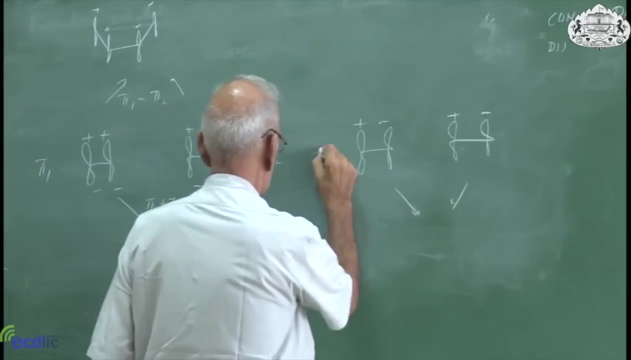 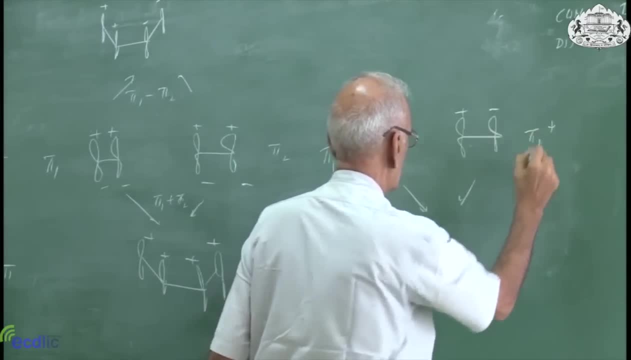 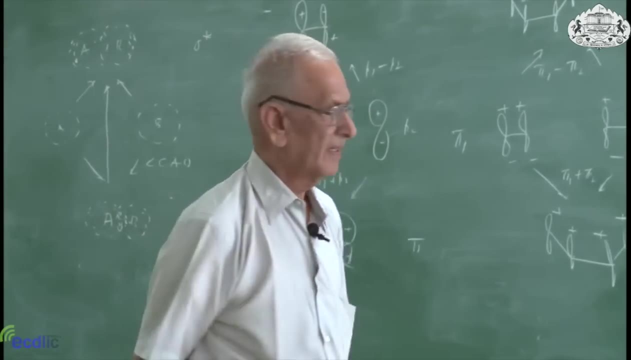 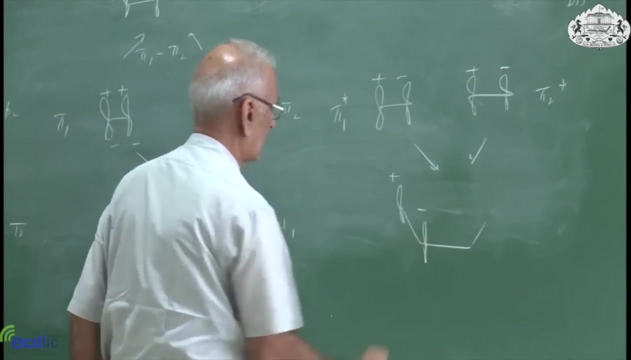 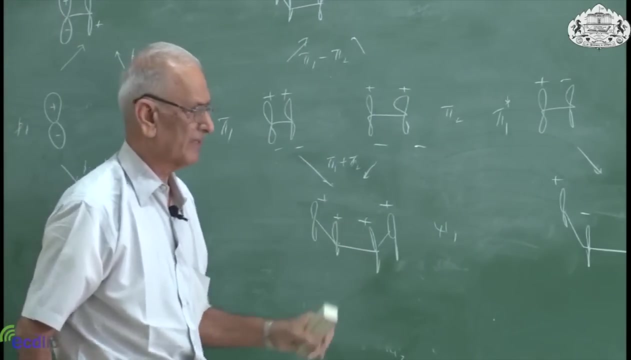 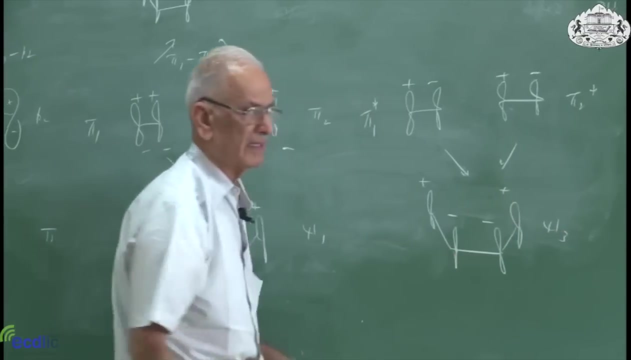 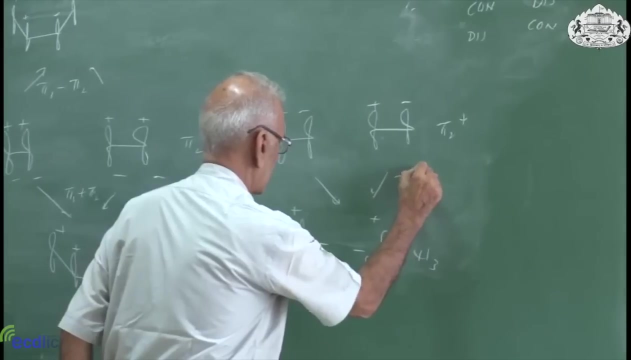 Pi 1 star, pi 2 star. what is this? These are two anti-bonding orbitals. I combine them in a positive order, In a positive manner. when it is positive, what should happen? Middle orbital should have same sign. So this is your psi 3 orbital. I combine them. pi 1 star plus pi 2 star gives 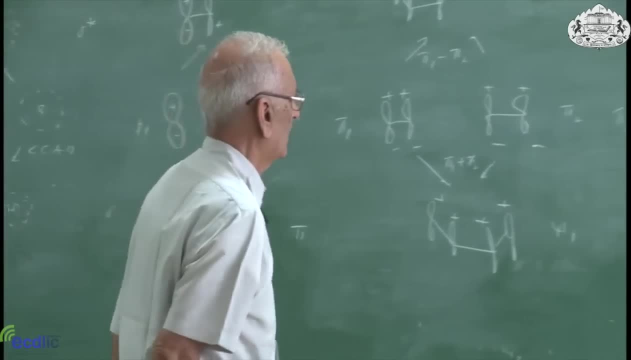 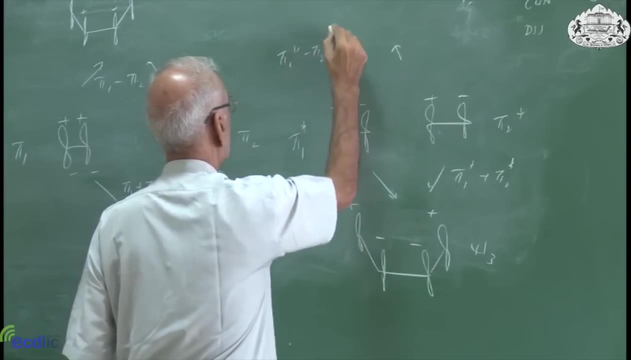 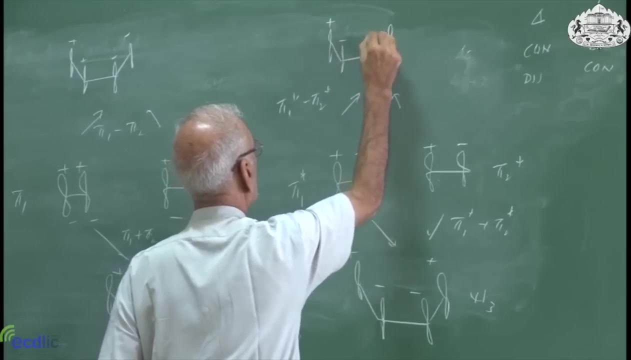 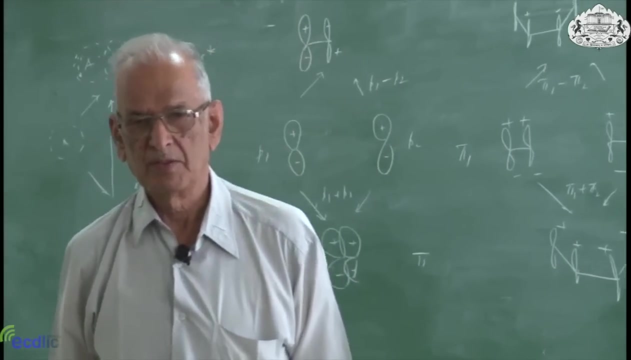 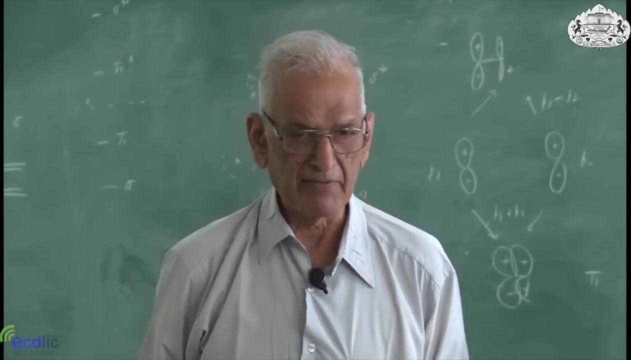 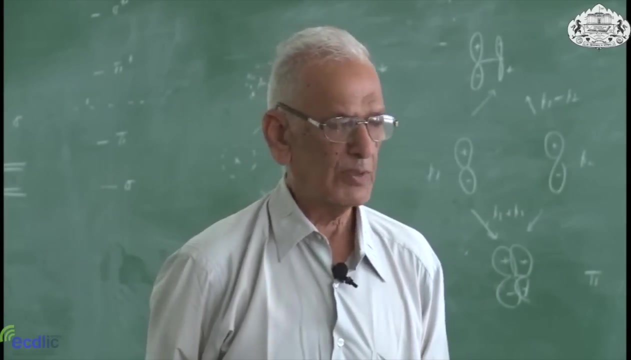 you psi 3.. And pi 1 star minus, pi 2 star, plus, minus, plus minus. So in butadiene there are going to be four orbitals: y, 1, psi 3.. 1, psi 1 will be plus, plus, plus plus. psi 2 will be plus, plus, minus, minus psi 3 will. 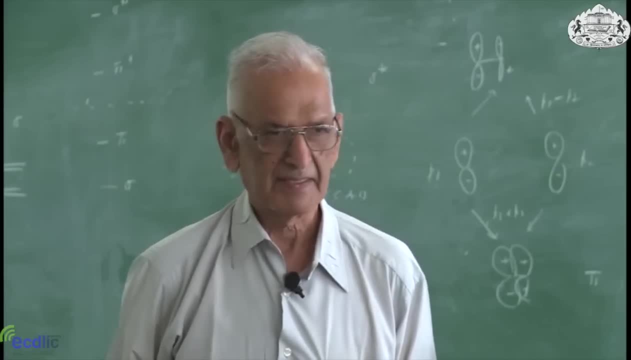 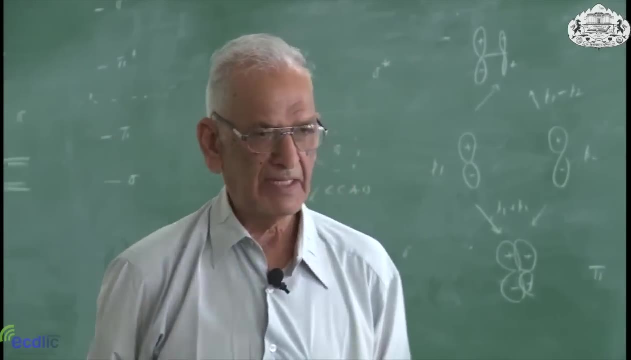 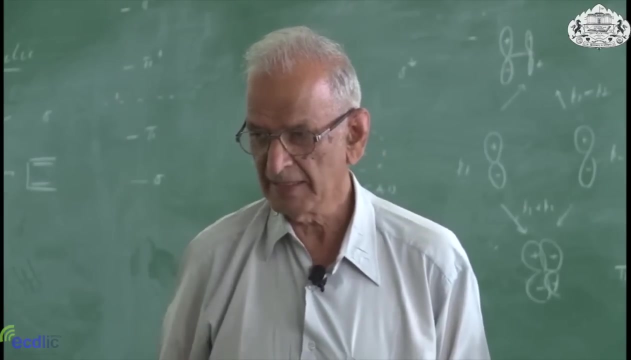 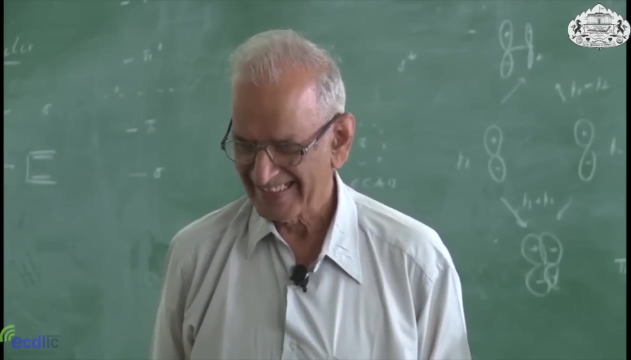 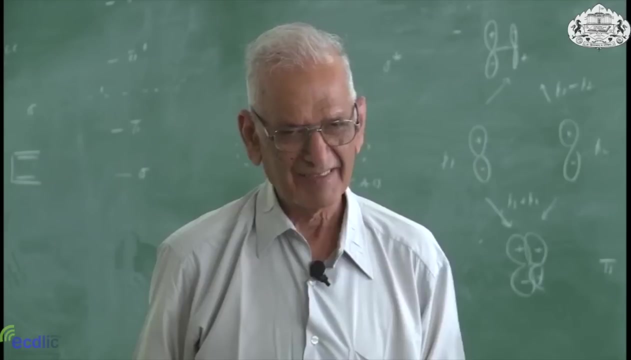 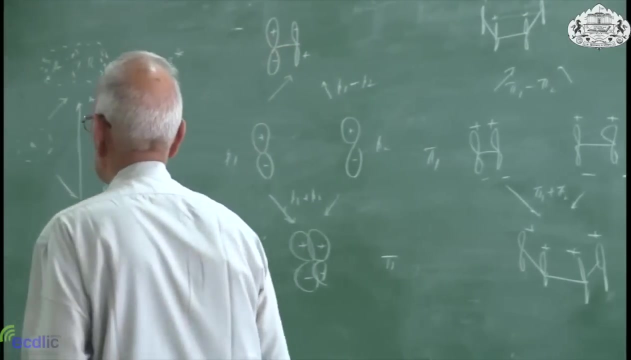 be plus, minus, minus, plus. psi 4 will be plus, minus, plus, minus. Even if you are woken in the sleep, write the four orbital of butadiene, it will come very fast. What is psi 1?, Psi 2?, Psi 3?? Very good, So both of them are in the sleep. also they can tell it all right. 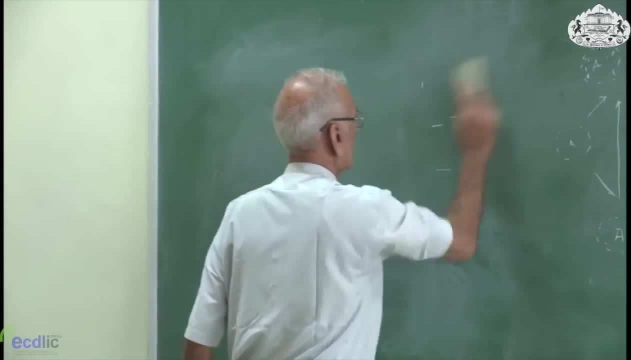 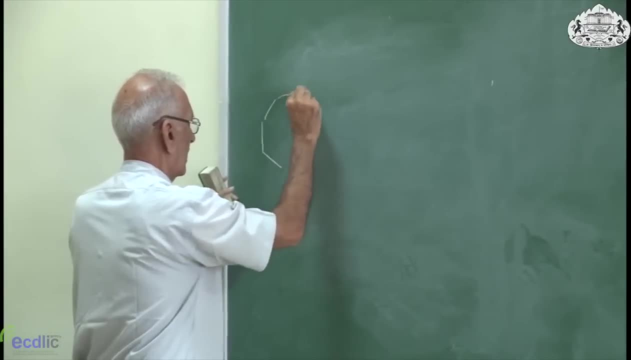 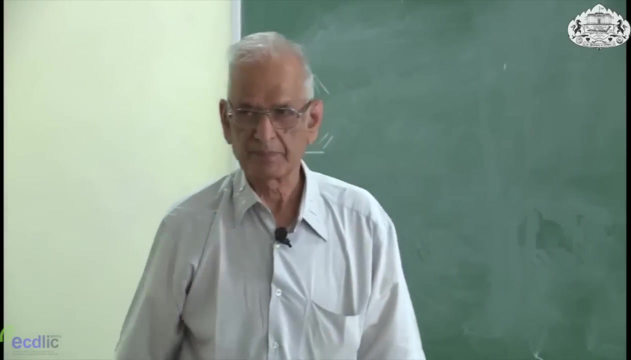 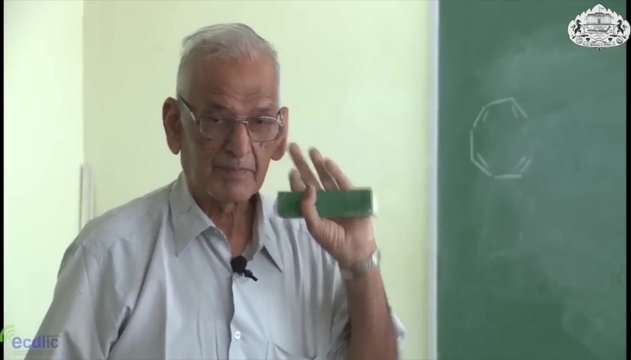 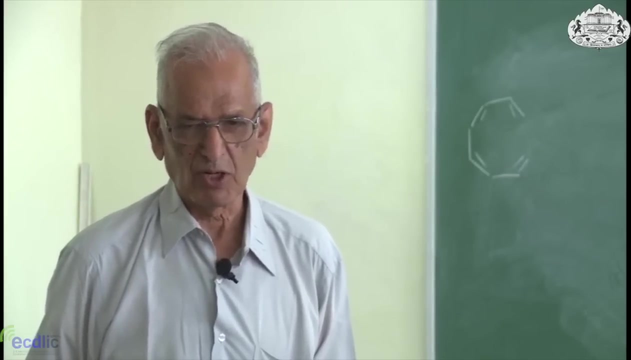 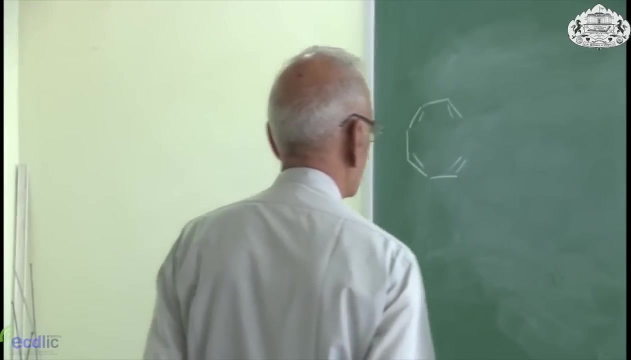 Very good. What will you call this compound? How many carbons, 8 carbons, So octa. how many double bonds? 4 double bonds, 4 octa tetraene. You want to put the numbers 1,, 3,, 5,, 7, octa tetraene. How did we make? 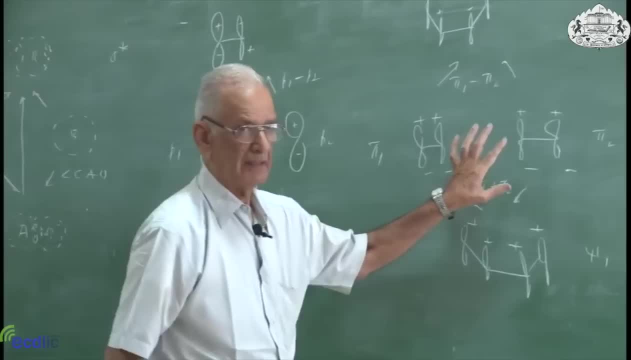 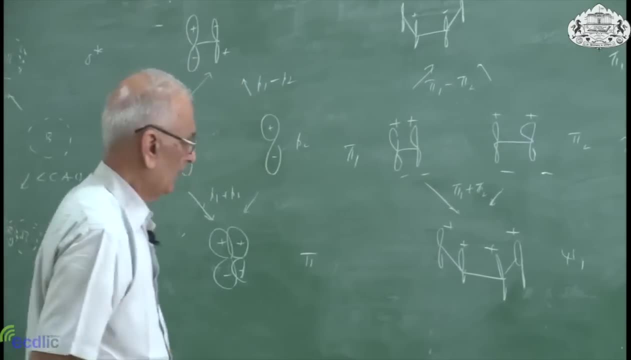 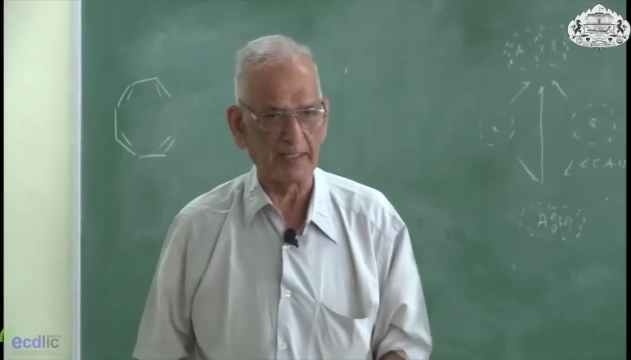 butadiene. We combined two ethylates and built this. So if I want to write how many double bonds, 4 double bonds, 4 double bonds, 4 double bonds. So it should be 8 orbitals. 4 will be bonding, 4 will be anti-bonding. 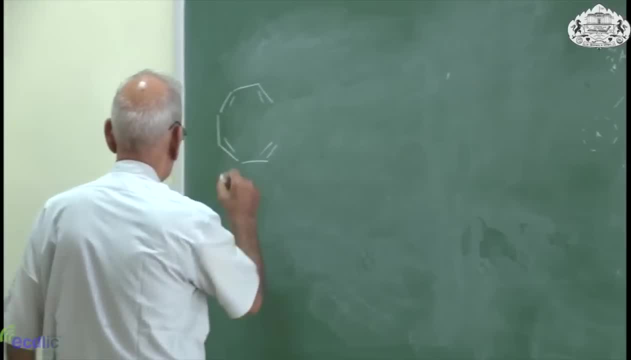 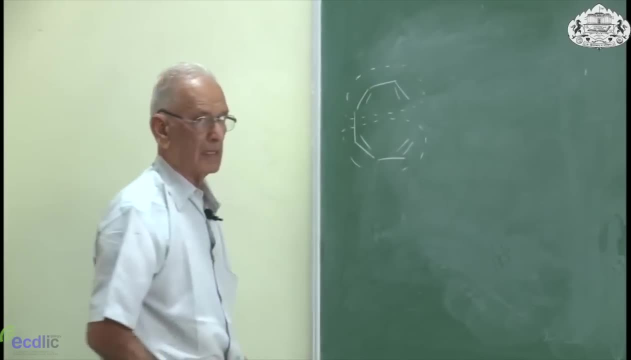 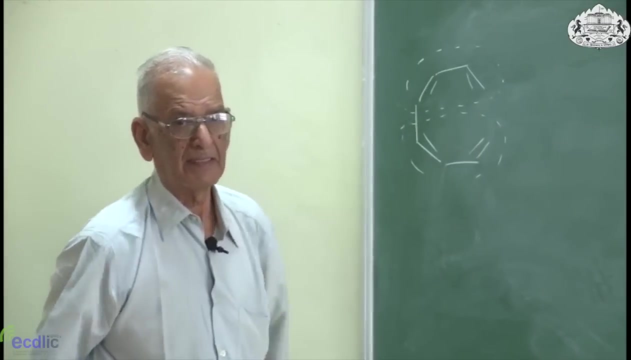 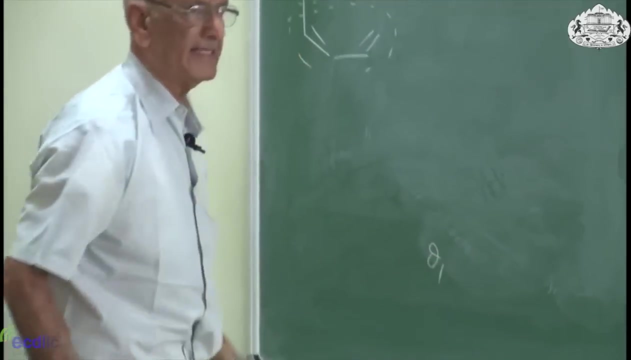 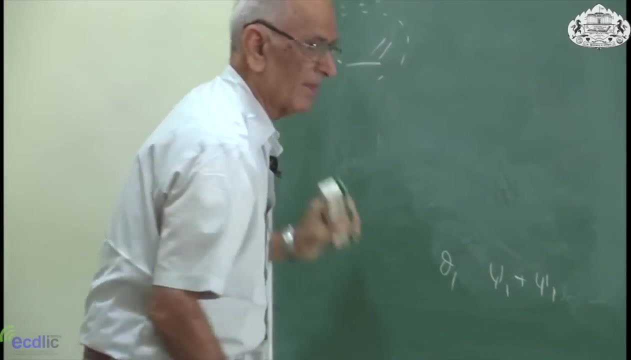 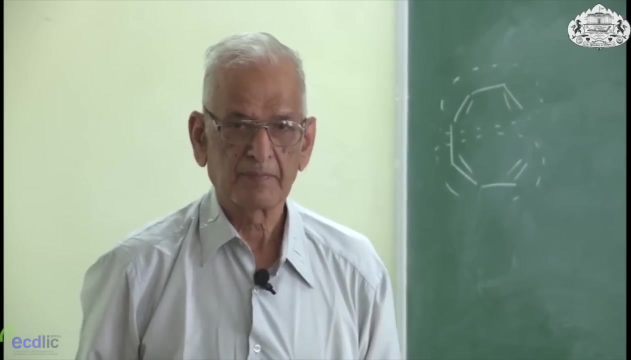 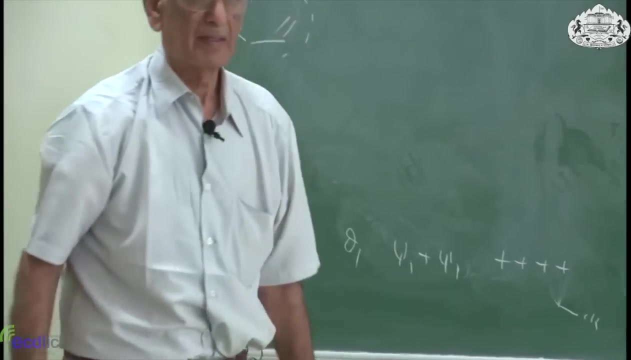 What should I combine? 1 butadiene has to be combined with another butadiene. So let us write Theta 1 orbital Psi 1 plus psi 1.. What is psi 1? Plus, plus, plus, plus, So and combination is positive. So middle orbitals must have: 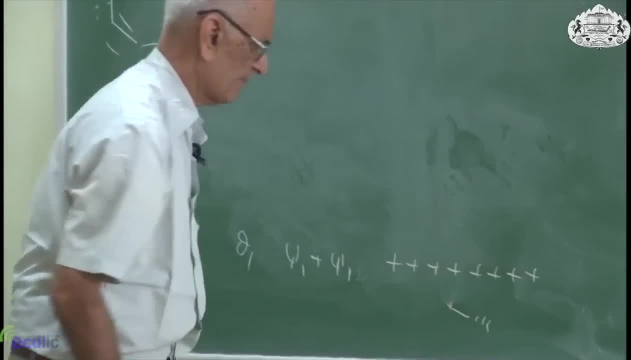 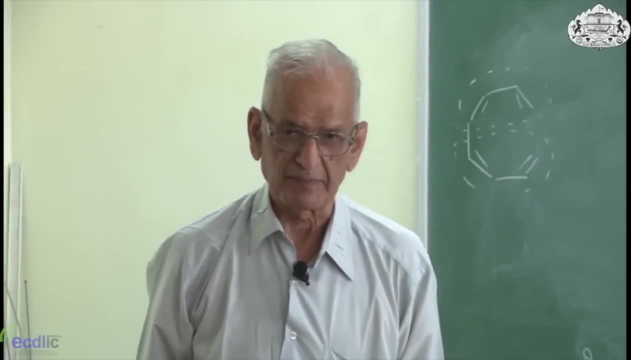 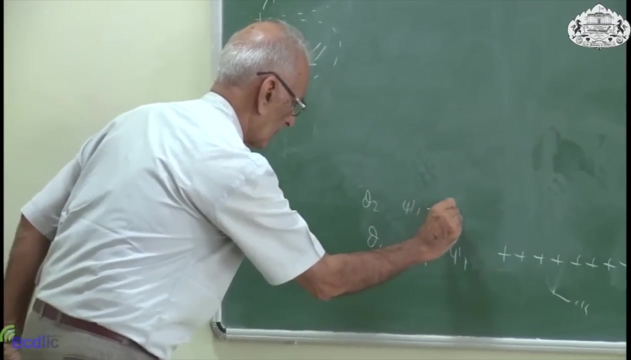 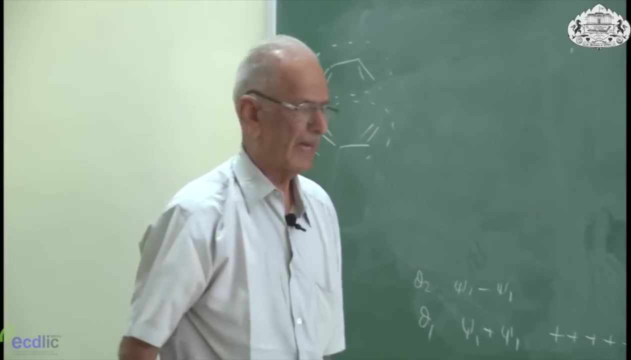 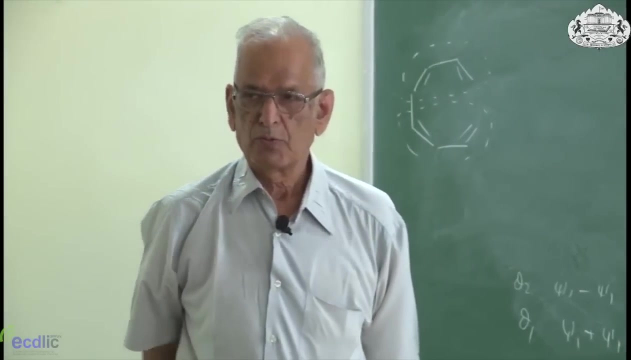 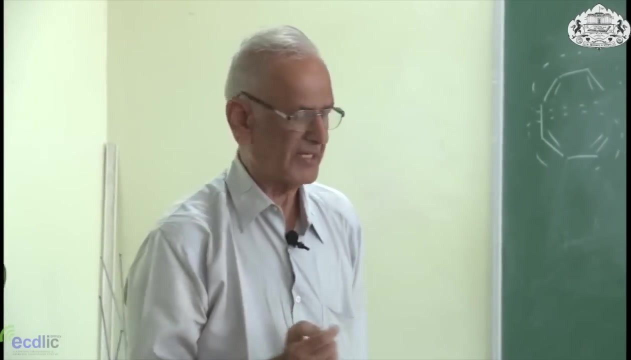 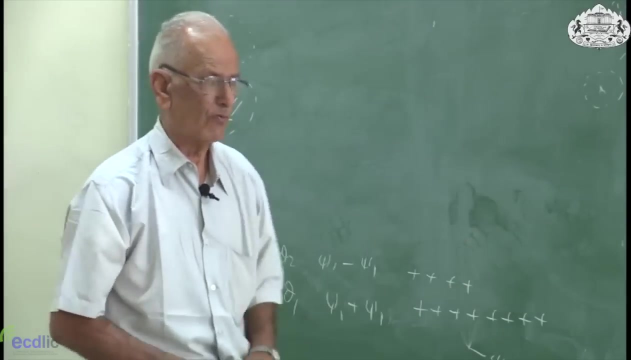 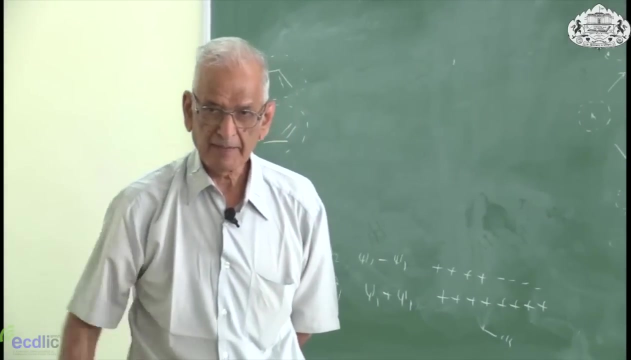 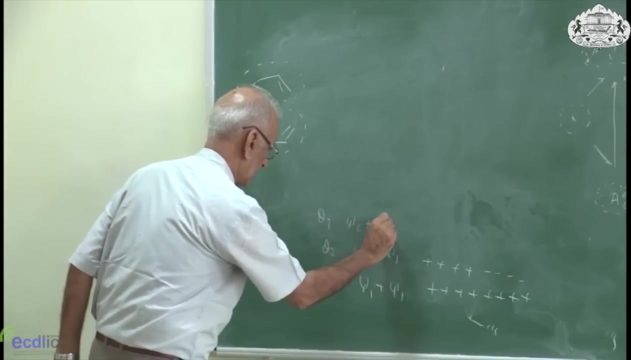 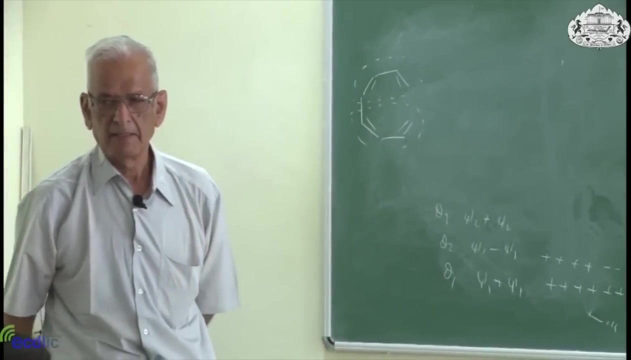 same sign. So, without mathematics, we are writing these orbitals: Psi 1 minus psi 1.. What should I write next? Middle orbital must have opposite sign. So all four pluses on this side. on that side, all four minus Yes, please. What are the signs of psi 2?? 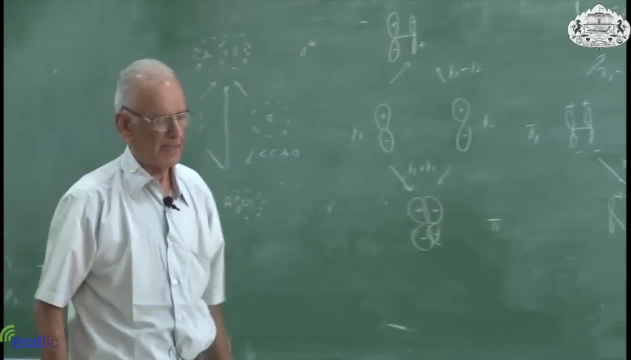 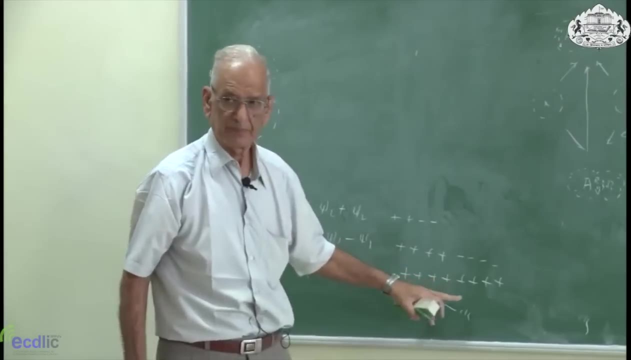 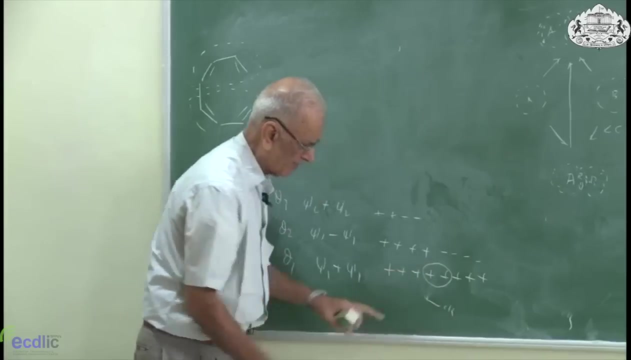 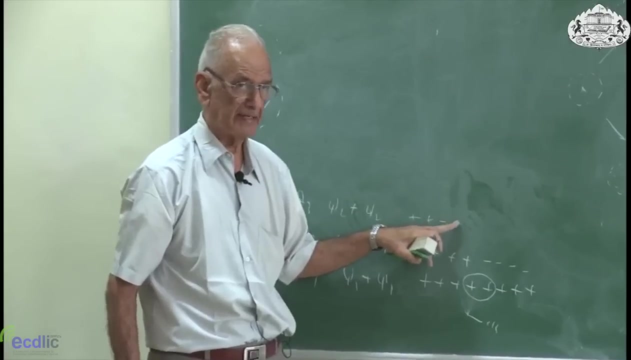 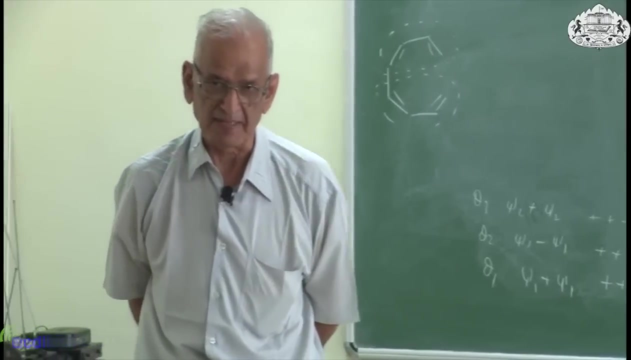 Zero, Zero, Plus, plus, minus, minus. What should I write now? When the sign is positive, these must have same sign. So what was the sign here? Minus, So minus. minus, plus, plus. 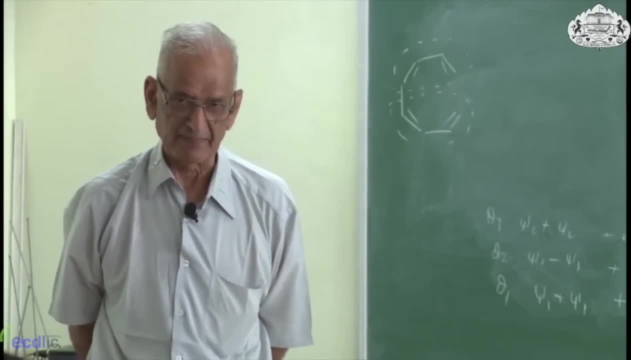 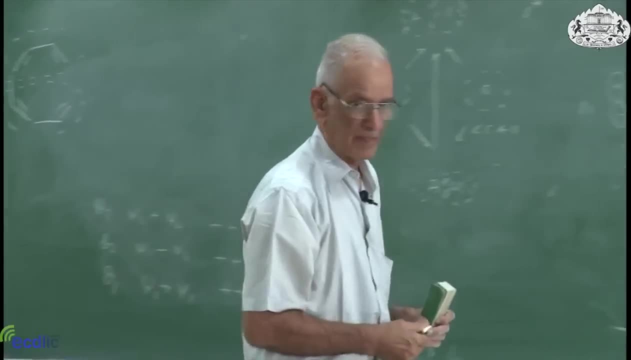 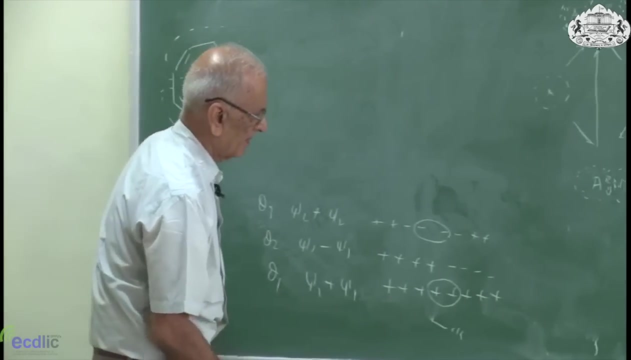 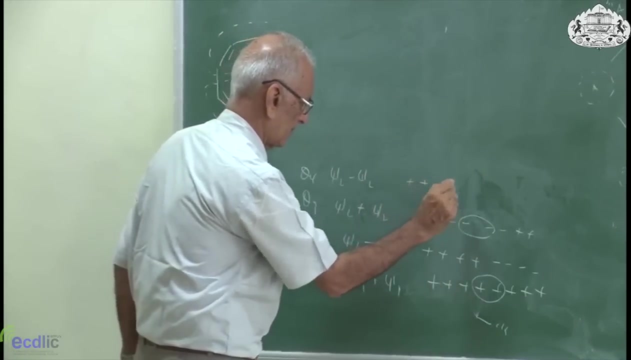 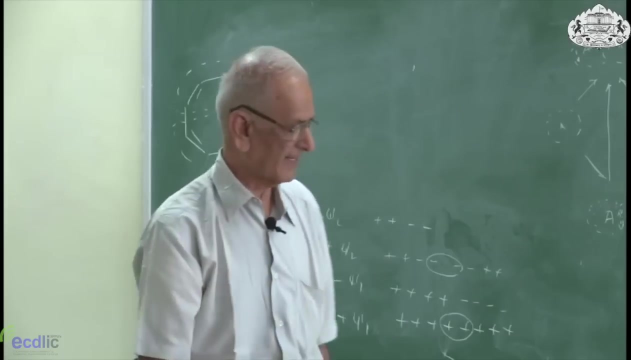 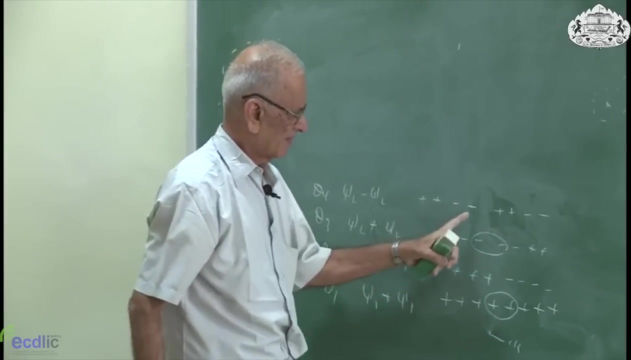 And which side The middle orbital have same sign. There you are OK: Plus plus, minus, minus. Now what Middle orbital have…? orbitals have opposite sign. Therefore this fellow must be plus, plus, plus, minus, minus. 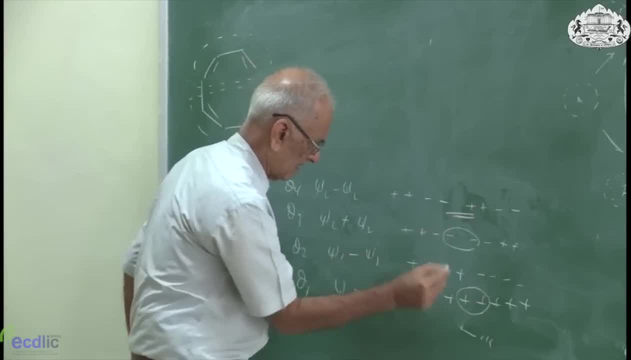 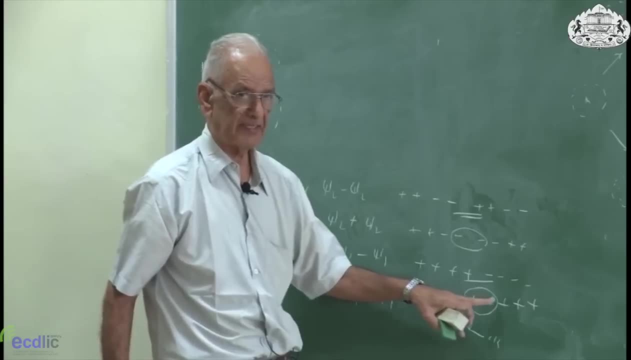 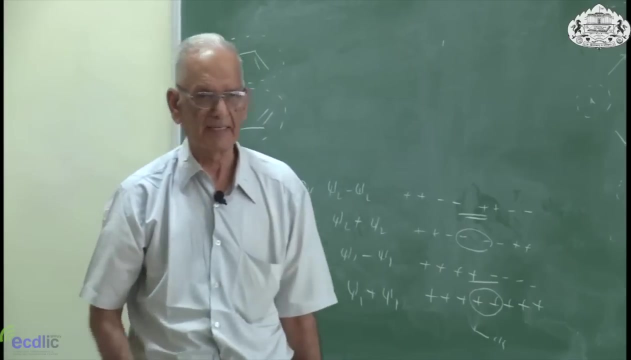 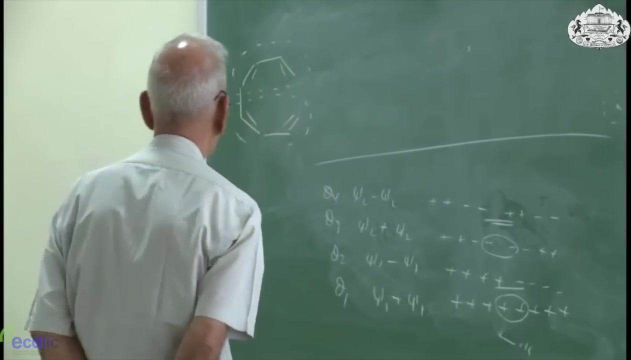 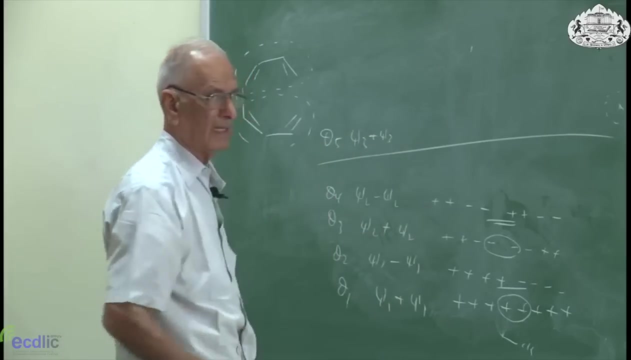 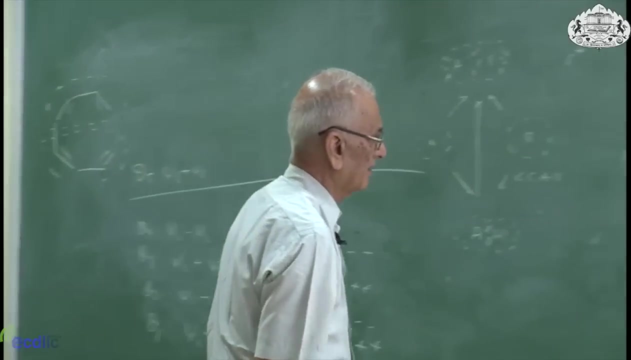 plus plus, minus, minus. When the sign is positive, middle orbitals have same sign. When the sign is negative, middle orbitals have opposite sign. So these are your four bonding orbitals. Now we are going to combine psi 3 orbitals of butadiene. What is your psi 3 orbitals? 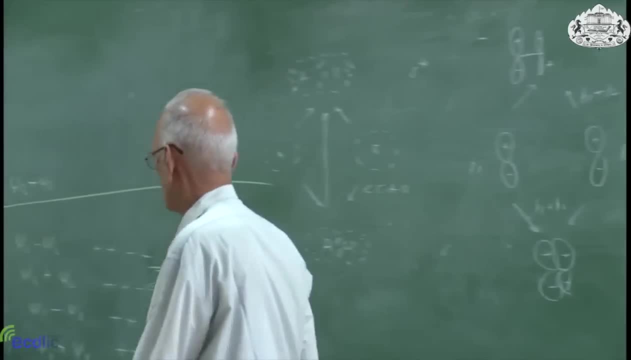 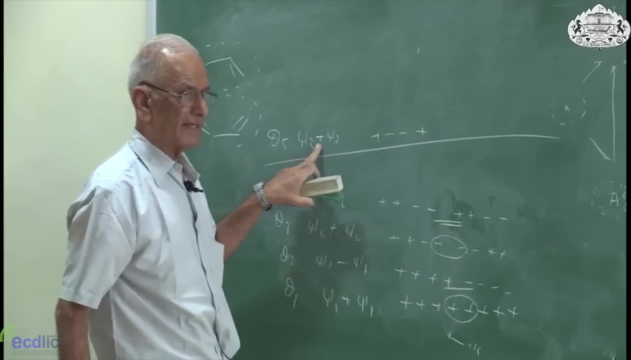 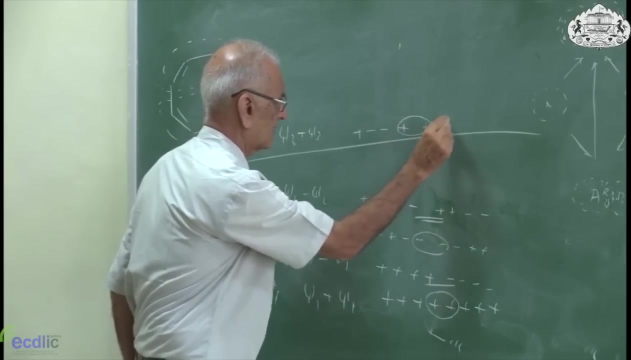 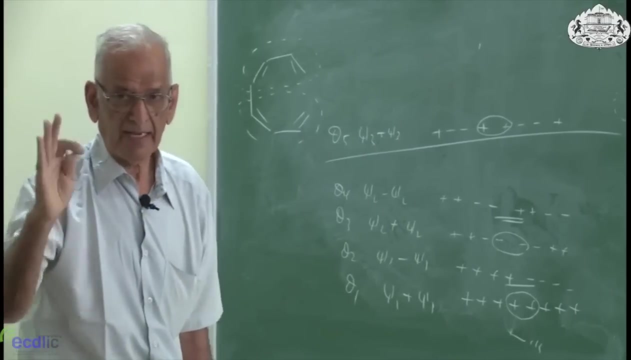 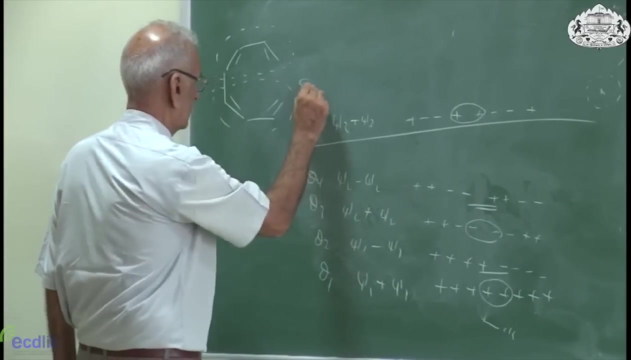 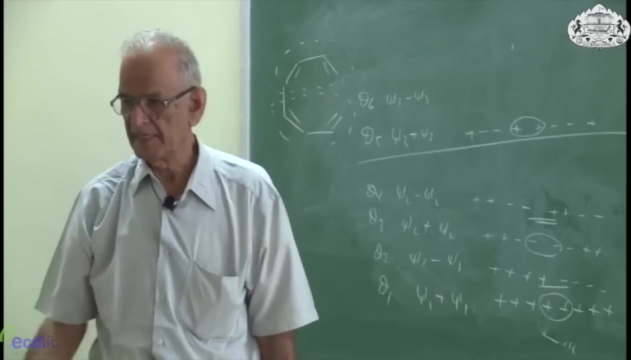 Plus, minus, minus, minus, Plus, minus, minus plus. What is the sign? Sign is positive, So middle orbitals must have same sign. So plus minus, minus, plus. If anybody has a problem, do not keep quiet. Yes, please. What should I write? 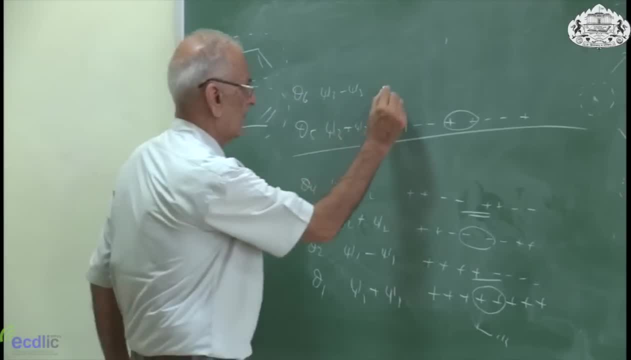 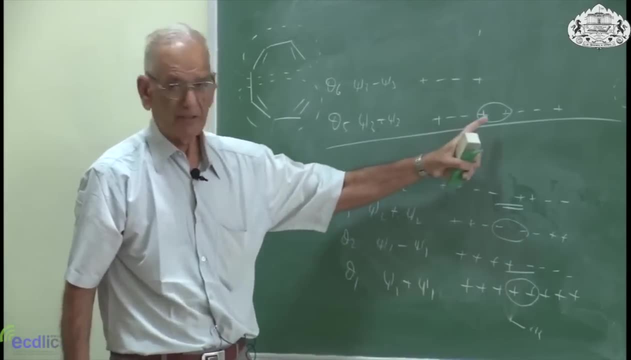 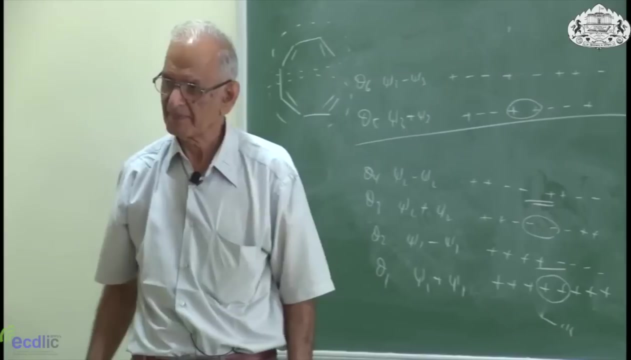 Plus, minus, minus, minus, plus, Plus, minus, minus, plus. Now, what Opposite sign? Opposite sign. So I must begin with minus, Minus, plus plus, minus, Minus, Minus, Minus, Minus, Minus. 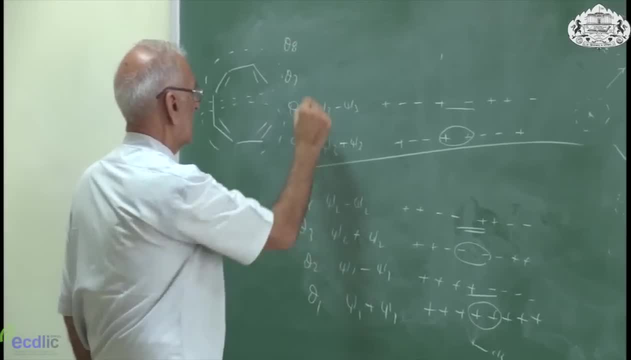 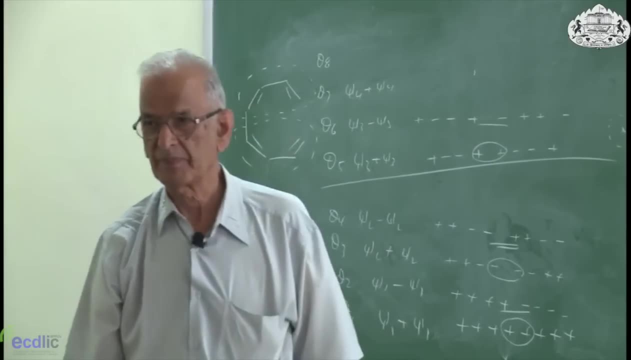 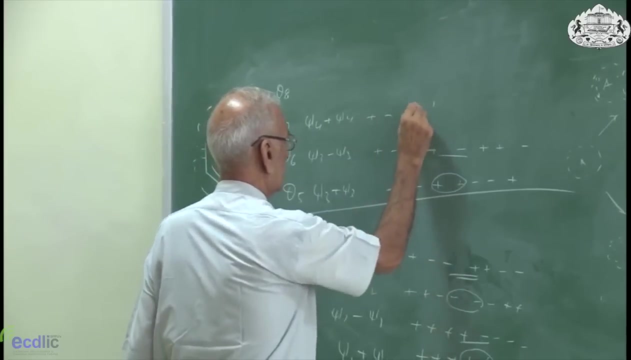 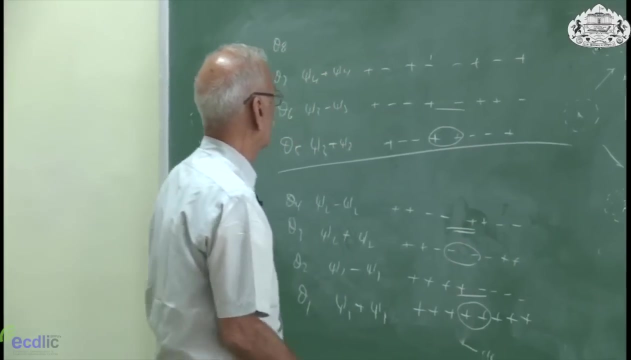 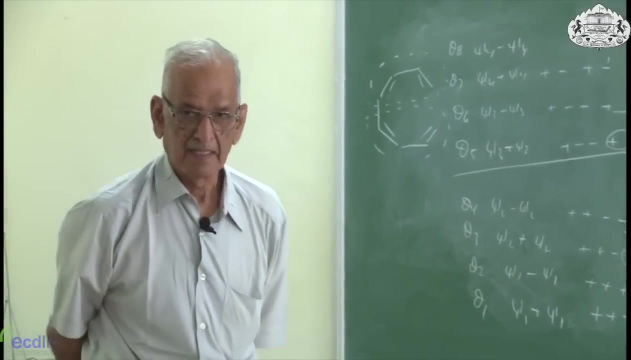 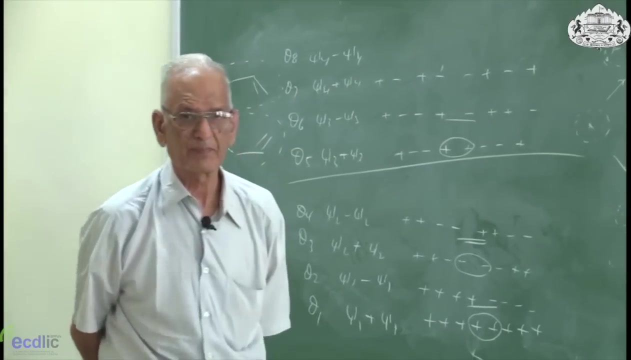 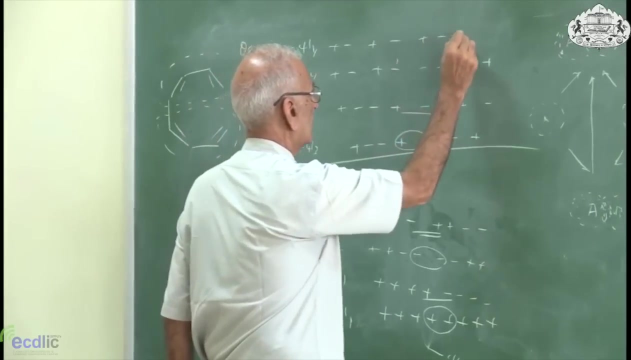 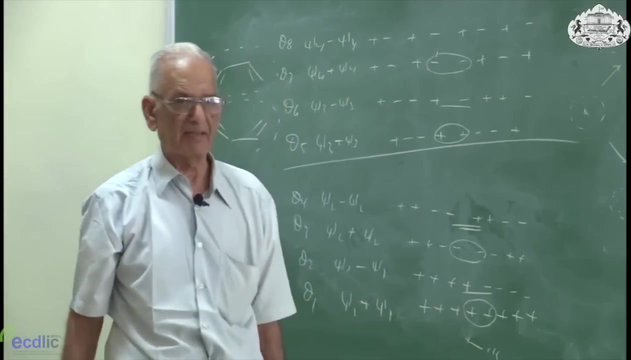 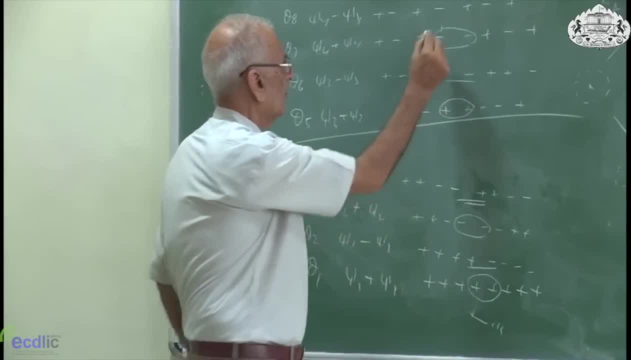 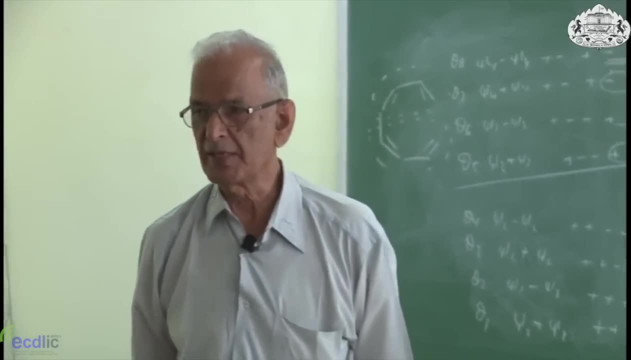 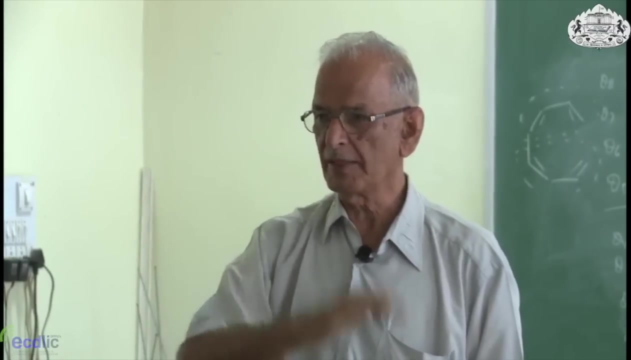 sign is positive, middle orbital have same sign. When sign is positive, middle orbital have opposite sign. So we wrote orbitals of butadiene, We wrote orbitals of ethylene, We wrote orbitals of butadiene, From butadiene we wrote octatetrine. If I ask you, write 16,. 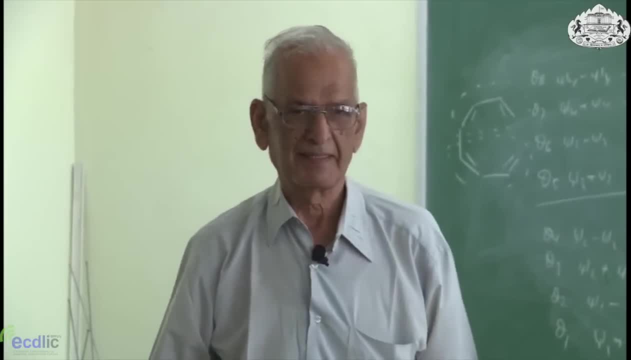 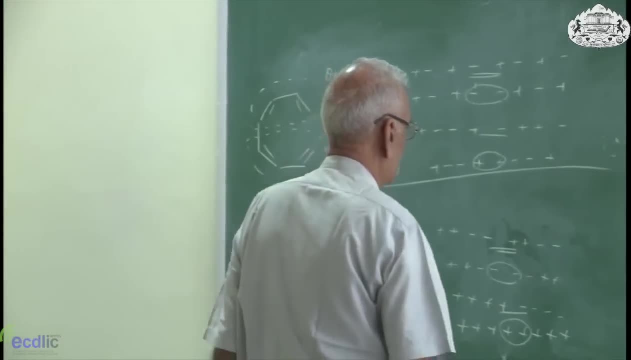 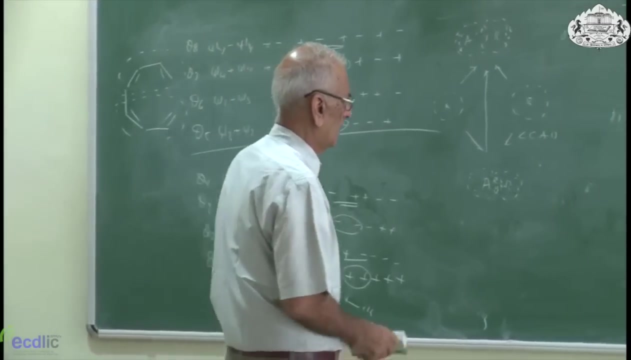 no problem, Combine these 8 orbitals, Theta 1 plus theta 1, theta 1 minus theta 1, and so on. So very easy, All right. So now we will come to our next question. What is this next question Question? 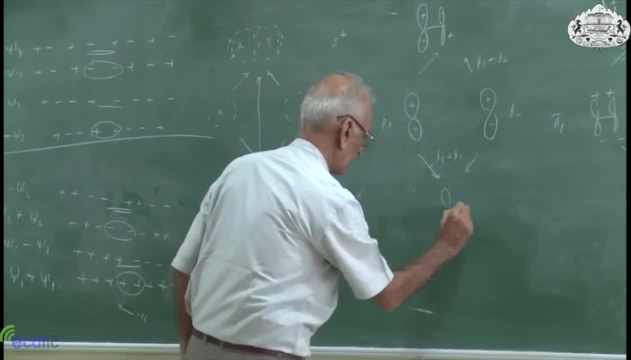 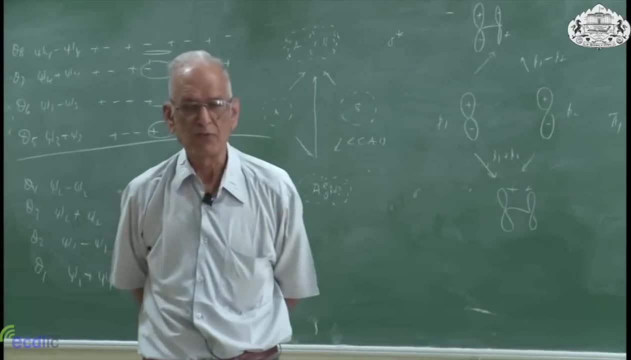 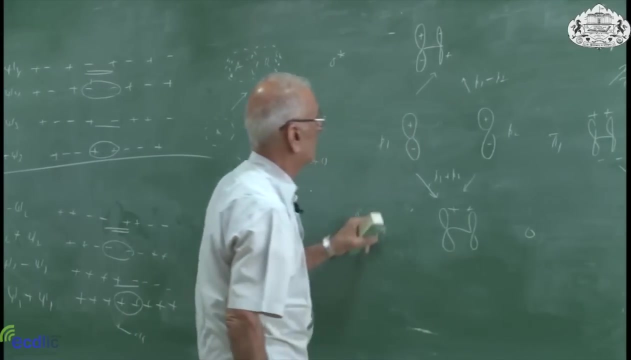 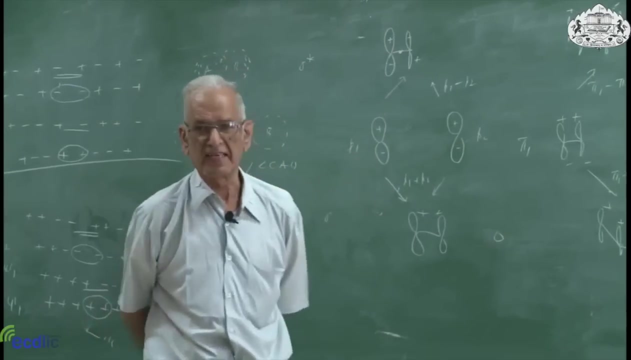 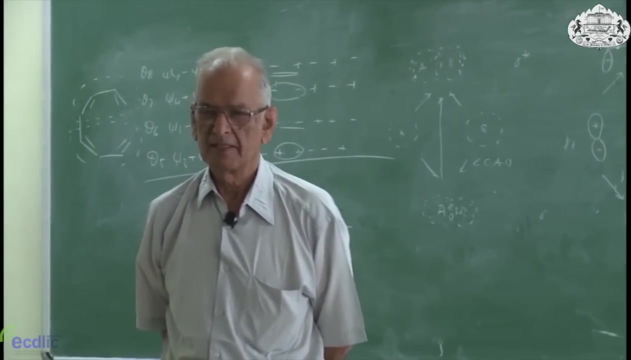 of nodes. Here there is no sign change. So first orbital has no nodes. Second orbital has 1 node. Where is that sign change? 1 sign change. So first orbital has no nodes. Second orbital has 1 node. Third orbital has 2 nodes. Fourth orbital has 3 nodes, 100 orbitals. 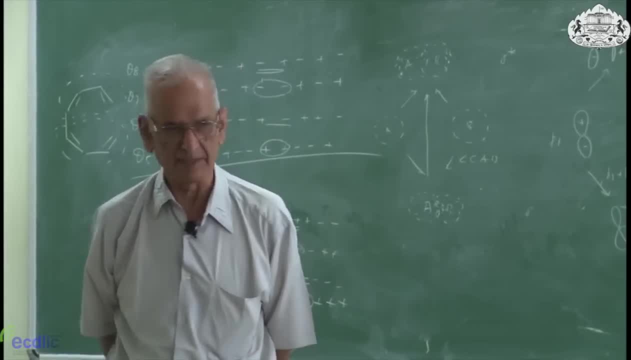 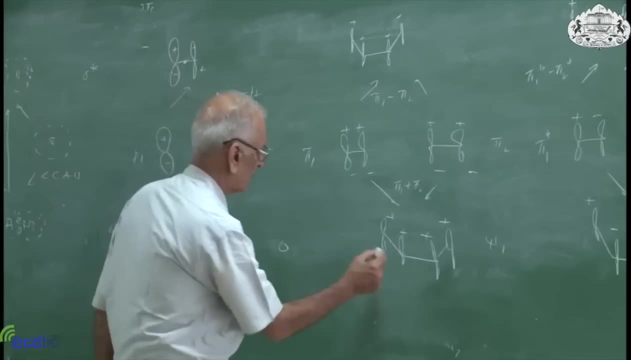 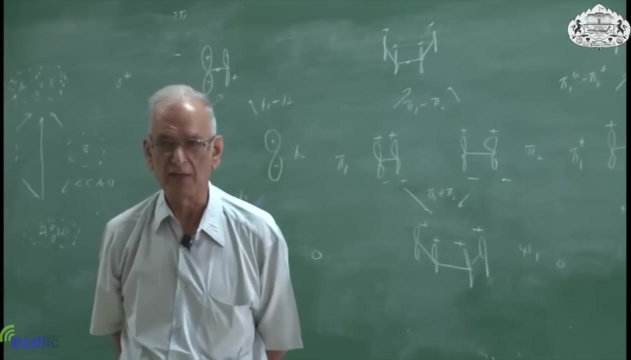 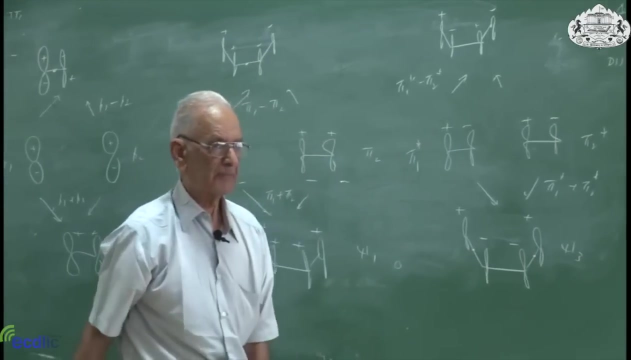 has 99 nodes, Very simple. So let us see. First orbital: How many nodes? No nodes, 0 nodes. How many is? 1., 2., 3., 4., 5. one node? second orbital has one node. third orbital: how many nodes? two nodes and the 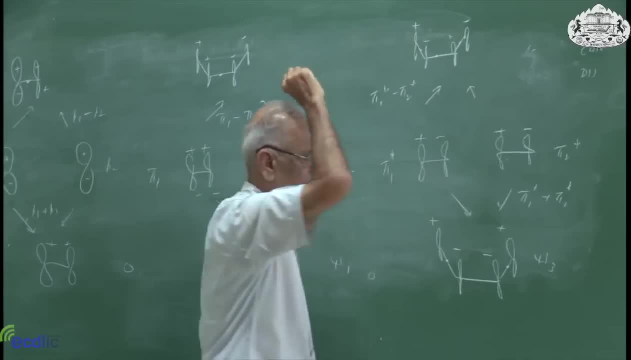 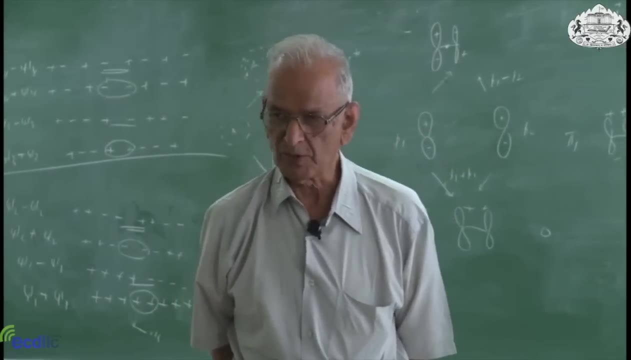 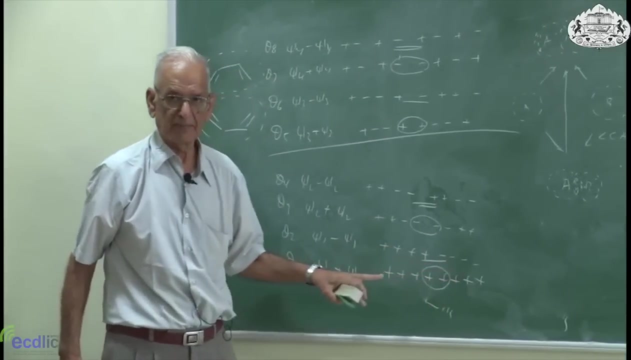 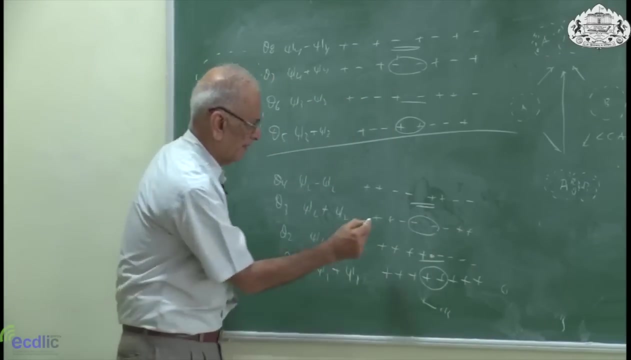 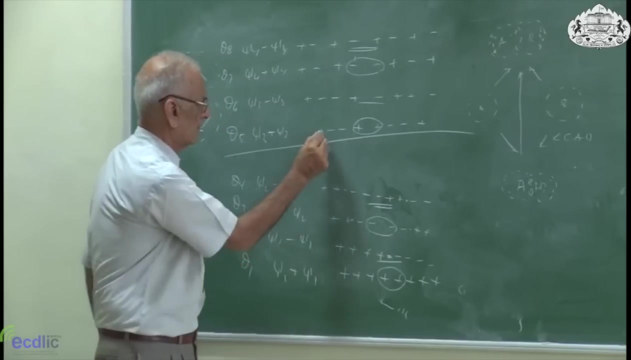 third orbital. the fourth orbital has three node, So I can use concept of nodes in order to draw orbital. Let us look at this: first orbital: no nodes. second orbital: one node. third orbital: two nodes. fourth orbital: three nodes. fifth orbital: one, two, three, four nodes. 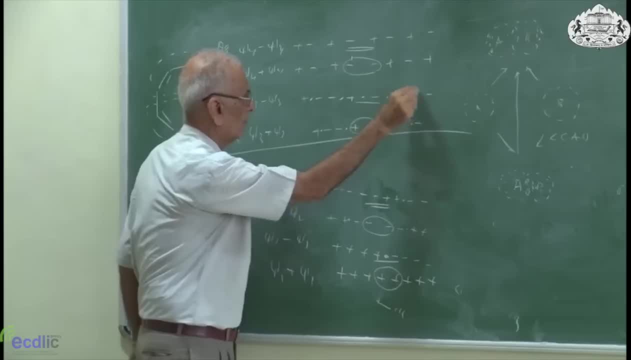 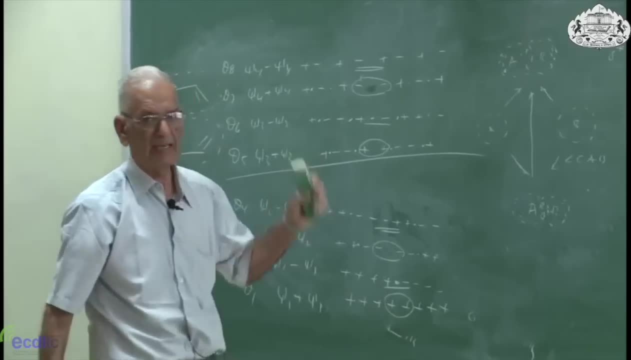 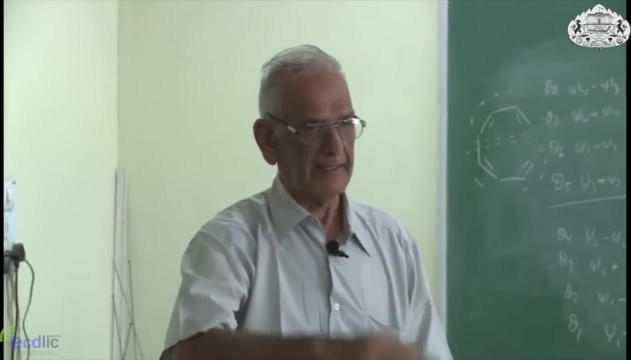 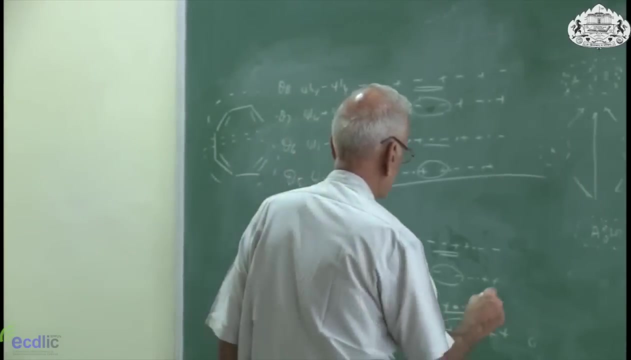 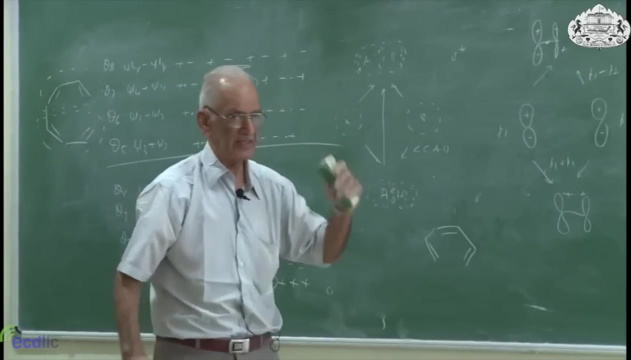 sixth orbital: one, two, three, Three, four, five nodes. one, two, three, sorry, four, five, six nodes and that will have seven nodes. So we have learnt to draw orbitals: ethylene, butadiene, octetetrine. What is our question When we go to hexatrine? 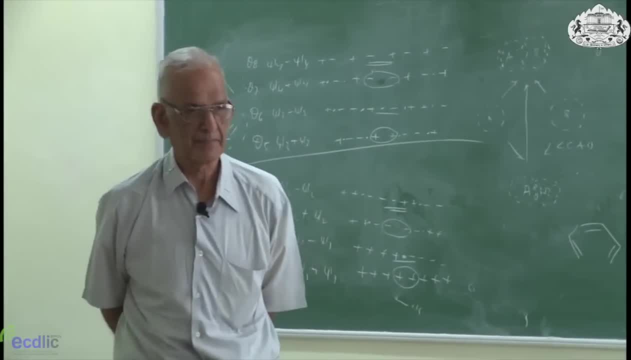 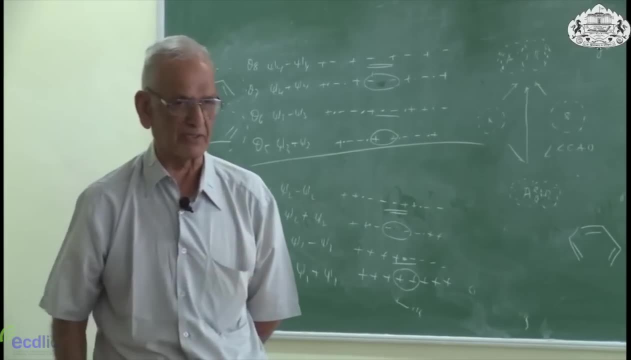 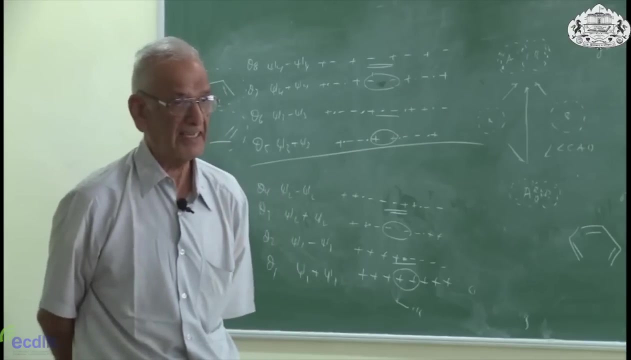 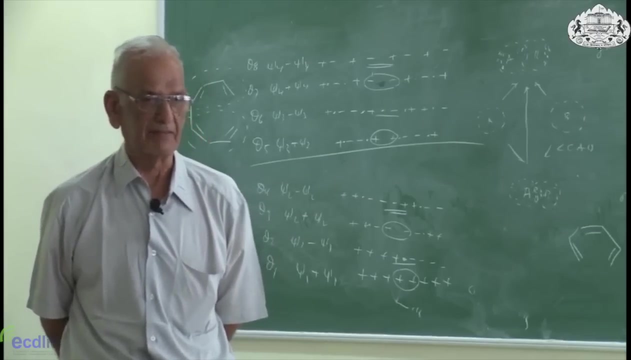 how can we combine? Ethylene was two, went to putadiene four, So combination was easy. Octetetrine four plus four. combination gave this. but for hexatrine combination will not work. So for writing the orbitals of hexatrine we will use the question of nodes. So when? 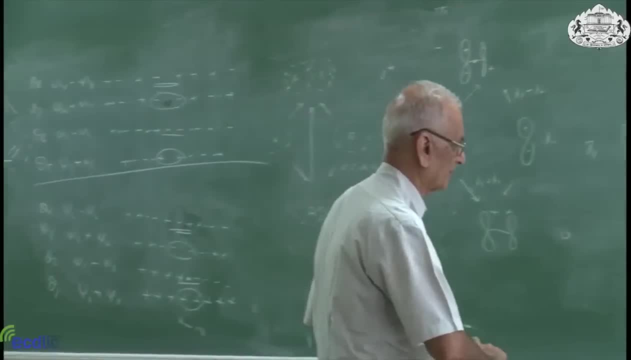 we meet next time. we will start with that. Thank you. Subtitles by the Amaraorg community.